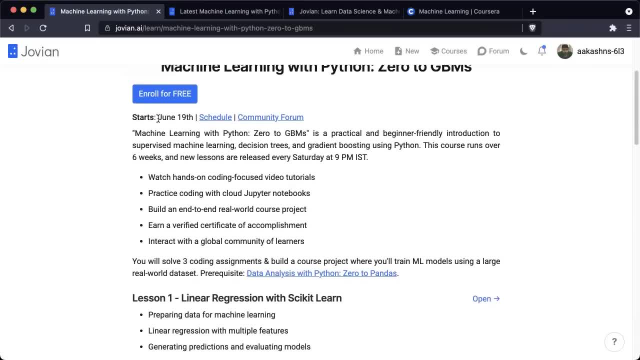 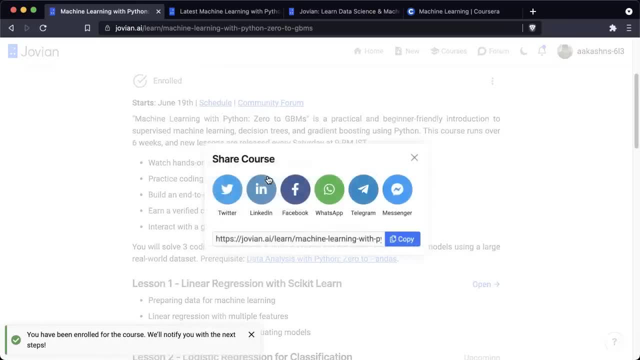 Even if you are unable to attend the course live, the first thing you should do on the course site is click the enroll button to enroll in the course. Once you're enrolled In the course, you can also invite your friends to join the course by sharing. 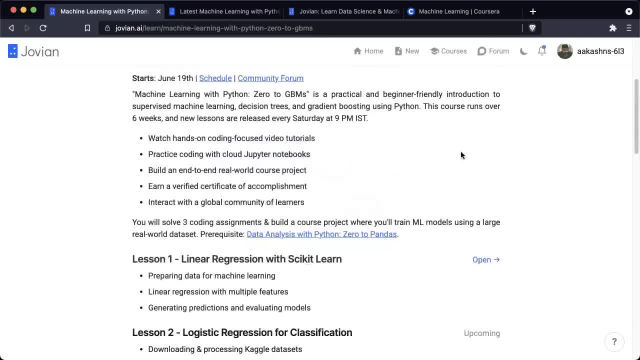 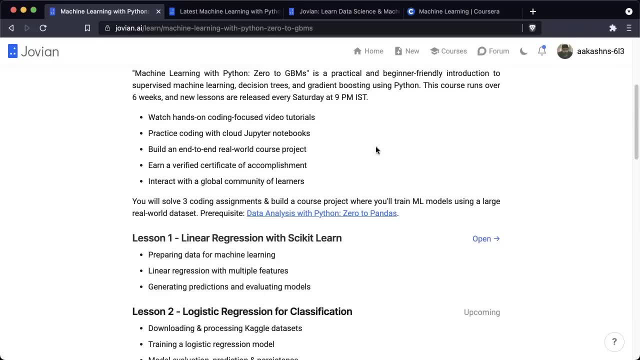 the course on any platform of your choice. So here's how the course works. every week You will watch one hands-on coding focused practical video tutorial on machine learning. Everything covered in the tutorial will be available as a Jupiter notebook which you can execute online on the cloud. 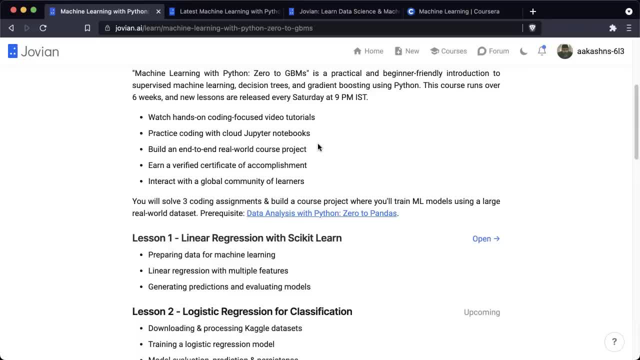 You will also solve three coding assignments and build a real world course project where you'll train machine learning models on a large real world data set. You can earn a verified certificate of accomplishment by earning a pass grade in all the assignments and the course project and you will get to interact with a global 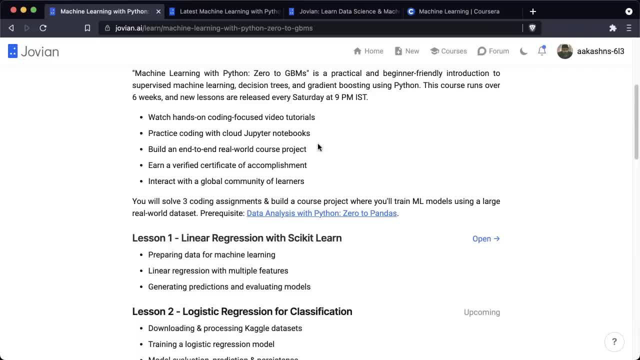 community of learners. As you participate in this course, there is a prerequisite for this course, the course data analysis with Python zero to pandas. So if you haven't taken this course already, do check this out. this is an introduction to programming with. 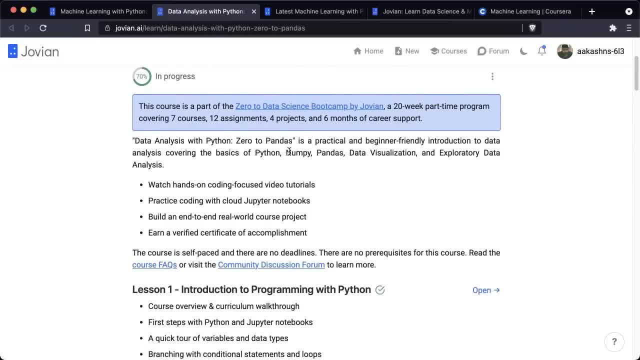 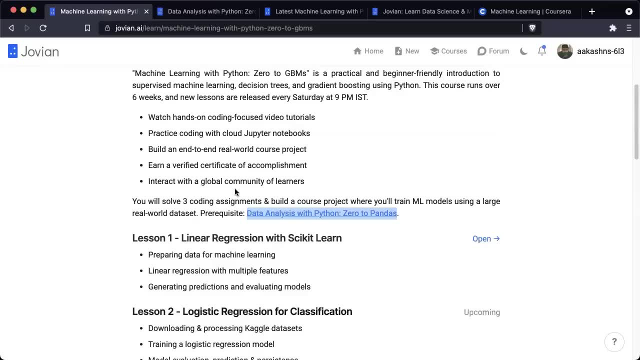 Python, and data analysis and visualization using tools like NumPy, pandas, matplotlib and seaborn. We'll be using these tools extensively during the machine learning with Python course. So before we begin, let's take a quick look at the curriculum for the course. 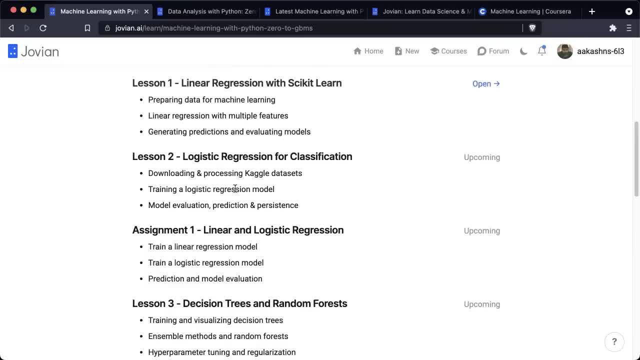 The first lesson which we'll cover today is linear regression with scikit-learn. We will talk about how we prepare data for machine learning, what a machine learning problem statement looks like. Then we'll train a linear regression model, first with One feature and then with multiple features, using scikit-learn. then we will generate. 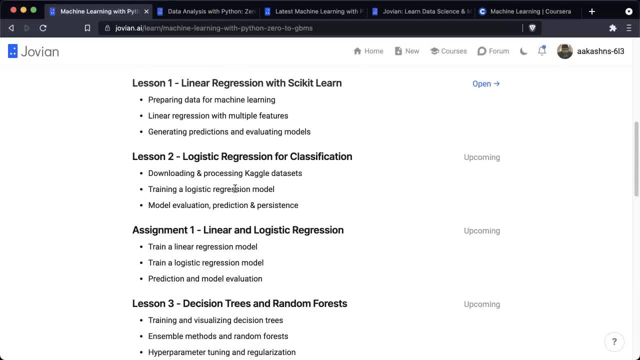 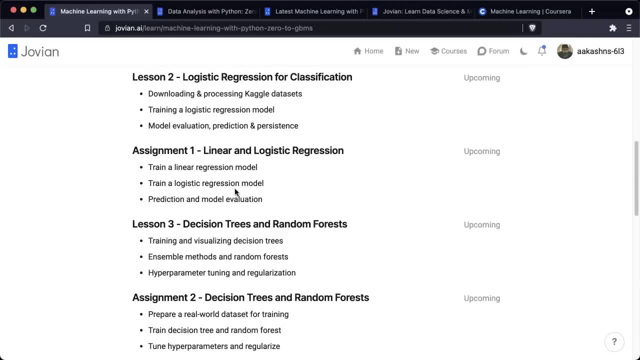 predictions and evaluate our linear regression models. Next week, we will look at logistic regression for classification problems, where we will download and process a dataset from Kaggle, an online platform for participating in data science competitions and building data science projects. We will train a logistic regression model using scikit-learn and we will look at model evaluation. 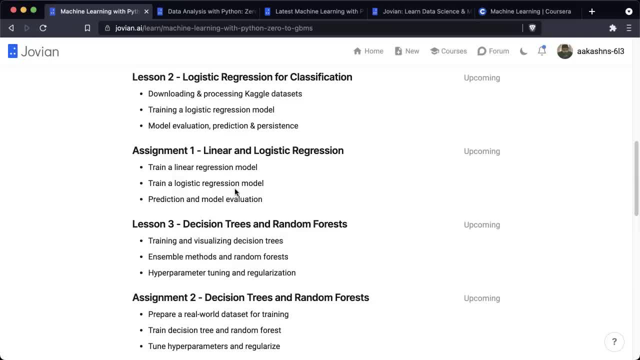 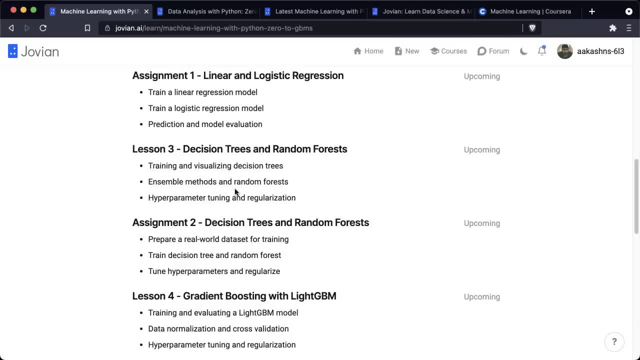 prediction and persistence. After the first two weeks, you will work on assignment one, which focuses on linear and logistic regression. You will train a linear regression model using scikit-learn. You will also train a logistic regression model using scikit-learn. 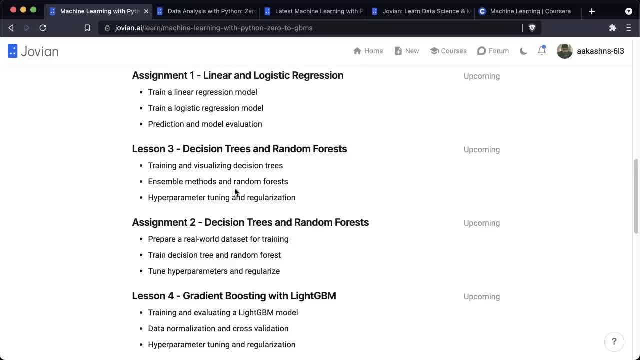 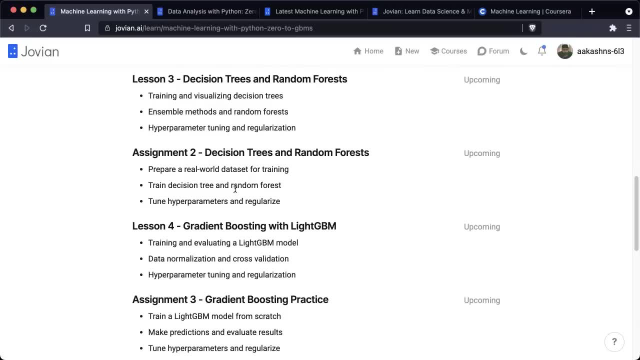 And you will use these models to make predictions and evaluate their performance. The third week will focus on decision trees and random forests. We will learn about training and visualization Of decision trees. We will learn about ensemble methods in general and apply the random forest technique in particular. 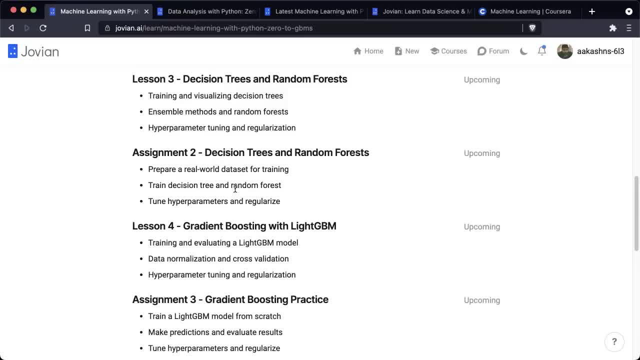 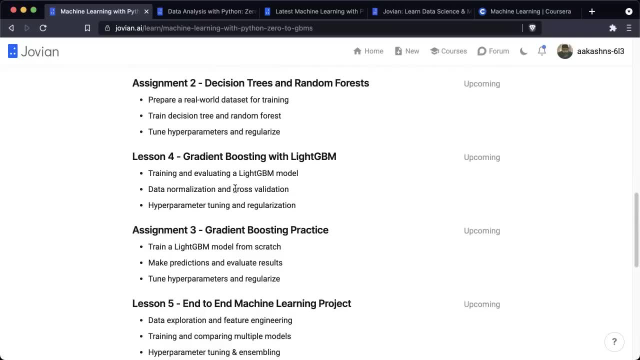 We will also look at hyper parameter tuning and regularization of machine learning models. This will be followed by an assignment on decision trees and random forest, where you will prepare a real world dataset for training, train a decision tree in a random forest and tune hyper parameters. 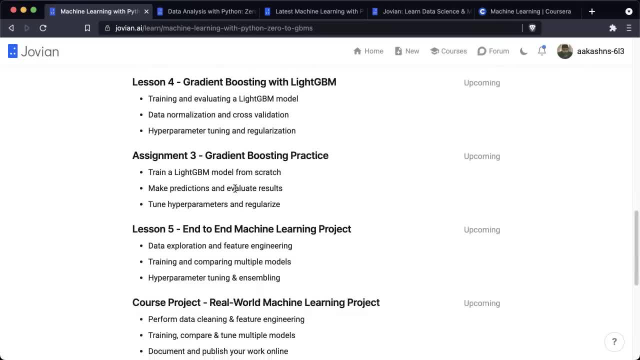 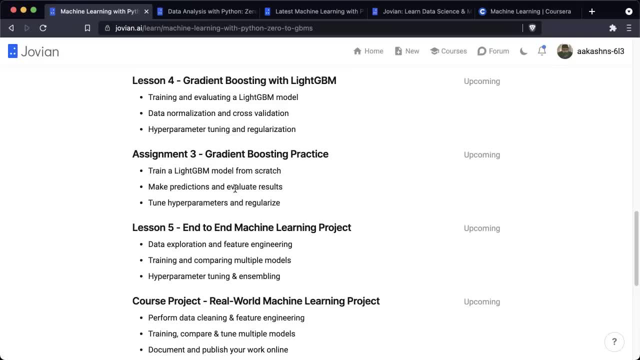 to regularize your model. The fourth week is gradient boosting with light GBM. We will train and evaluate a light GBM model. We will learn about data normalization and cross validation techniques. We will also learn about hyper parameter tuning, regularization and feature engineering. 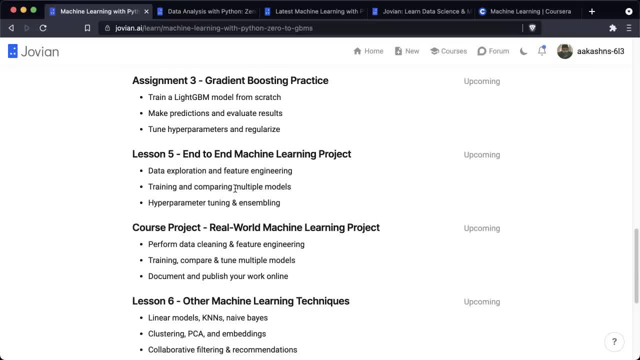 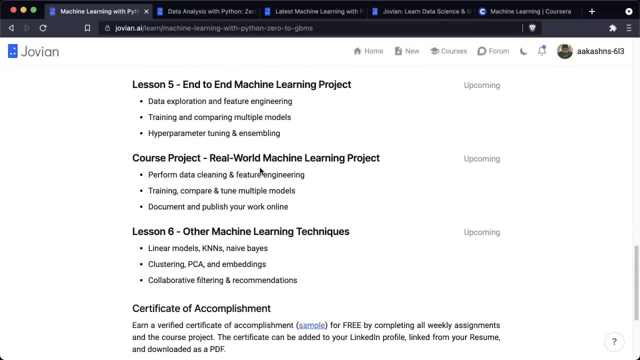 Then you will work on the third assignment, where you will train a light GBM model from scratch, make predictions, evaluate results and tune hyper parameters. The fifth week we will focus on building an end to end Machine learning project from scratch. We will take everything we've learned over the previous four weeks and apply them to a real world dataset with millions of rows of data. 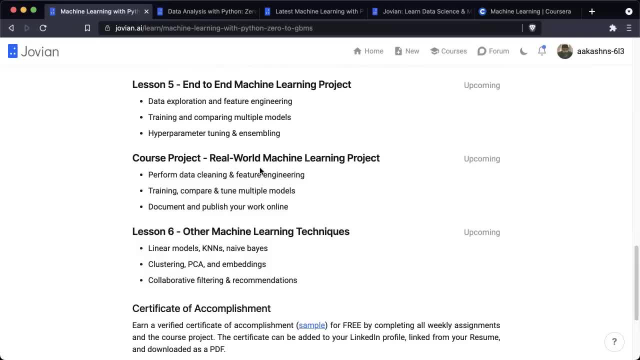 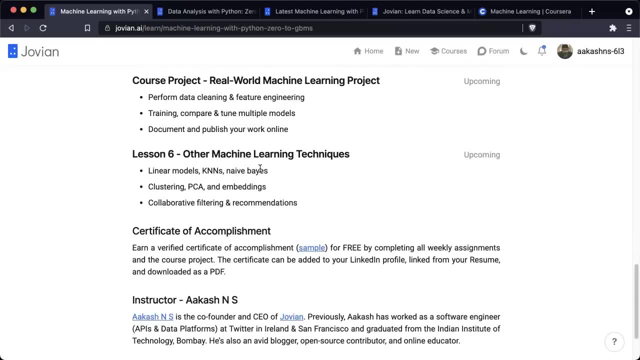 We'll start with data exploration and feature engineering. We will then train and compare multiple models. We will also tune hyper parameters and we will ensemble the results of several models. After this, you will work on a course project where you will build a real world machine learning project on your own from scratch. 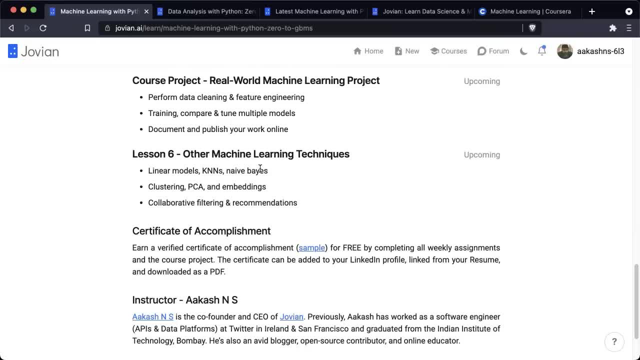 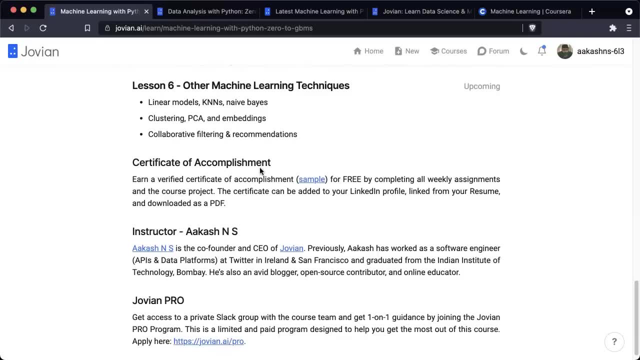 So you will perform data cleaning, feature engineering, You will train, compare and tune multiple models, and you will document and publish your work online. The sixth lesson is about other machine learning techniques, where we will have a quick overview of the entire landscape of machine learning. 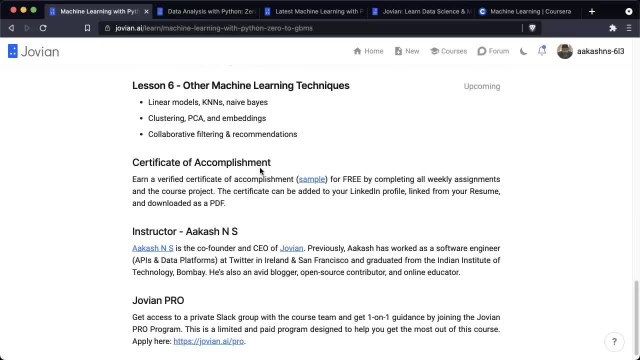 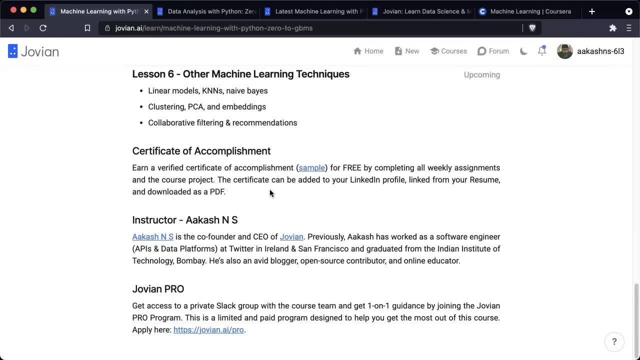 We will talk about linear models, KNNs, Naive Bayes models. We will also look at unsupervised learning techniques like clustering, PCA, embeddings, collaborative filtering and recommendations. briefly, You can earn a verified certificate of accomplishment for free by completing all weekly assignments and the course project. 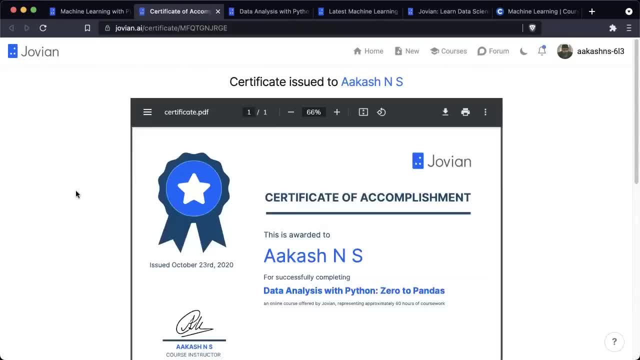 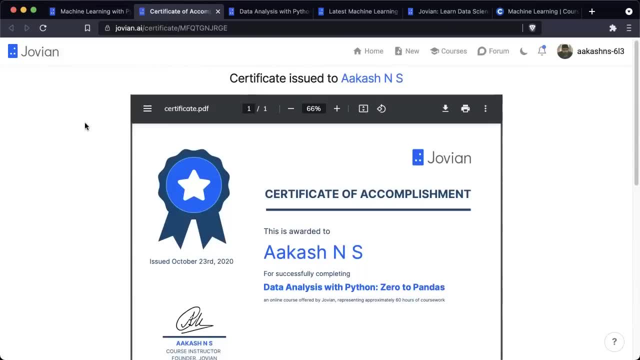 Here is a sample of what the certificate looks like. This certificate will be hosted online on your Jovian profile and you will be able to add this link on your LinkedIn profile and on your resume. You will also be able to download the certificate in PDF format. 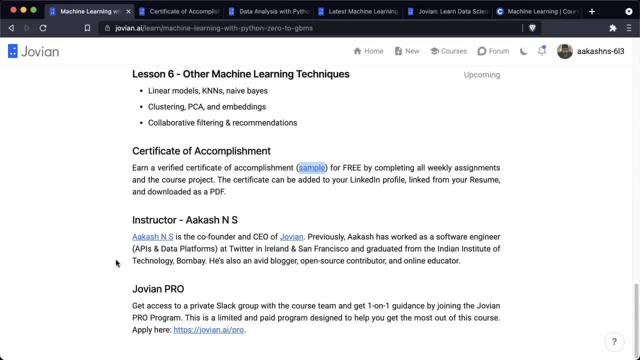 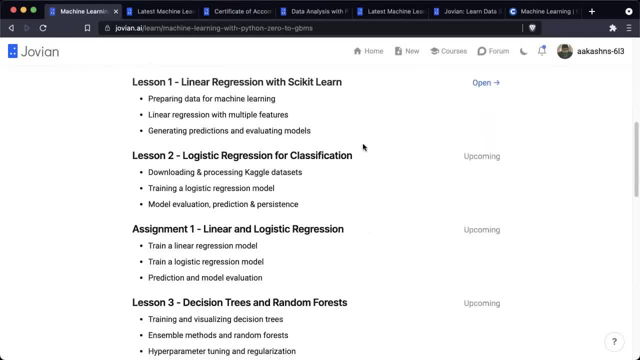 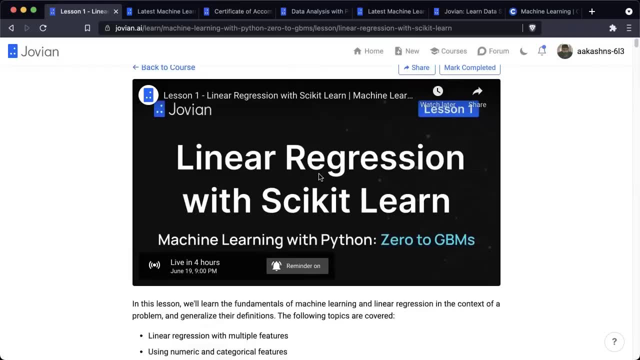 So with that, let's get started with lesson one: linear regression and scikit-learn. So I'll open up lesson one here and on this lesson page you will be able to see a recording of the lesson. You can watch this anytime. 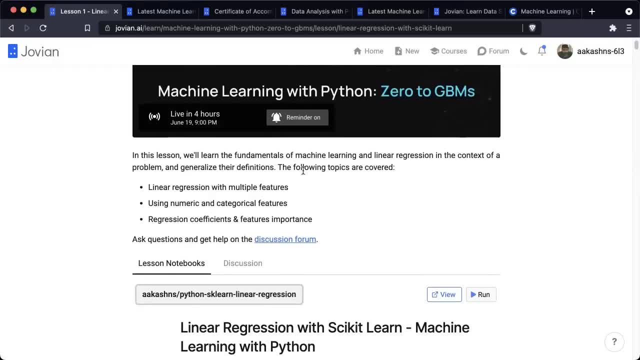 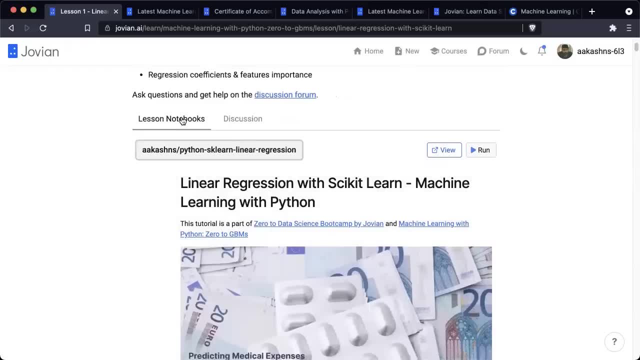 And in this lesson we learn the fundamentals of machine learning and linear regression in the context of a problem and then generalize their definitions. So all the code that we Will use in this lesson can be found in the lesson notebook section, And in the lesson notebook section you will find this Jupiter notebook. 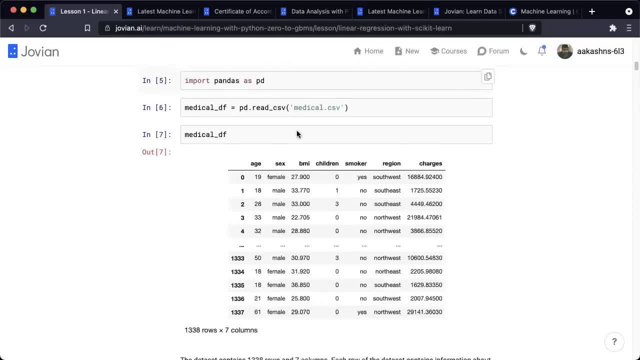 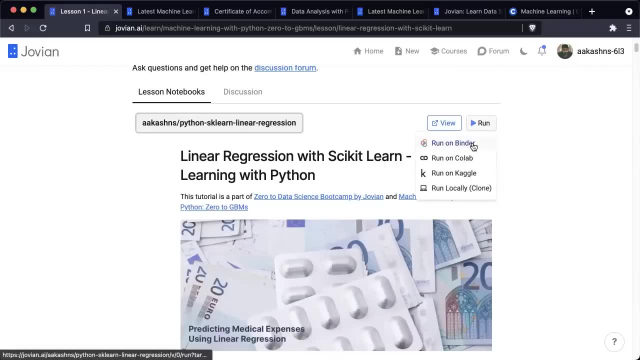 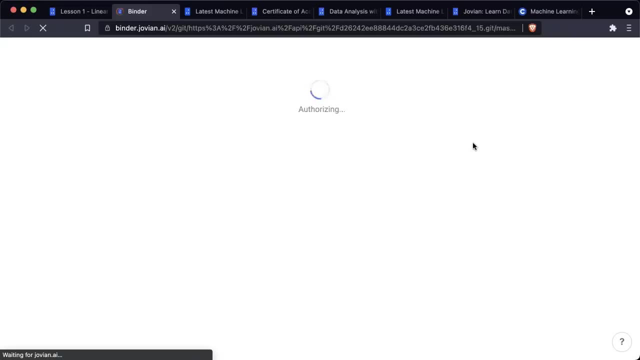 You can read the explanations in the notebook. You can see the code here, but if you would like to execute it online, just scroll up, click on the run button and select run on binder. This will take the Jupiter notebook that you were looking at on the lesson page and set up an online cloud machine for you where this Jupiter notebook will be. 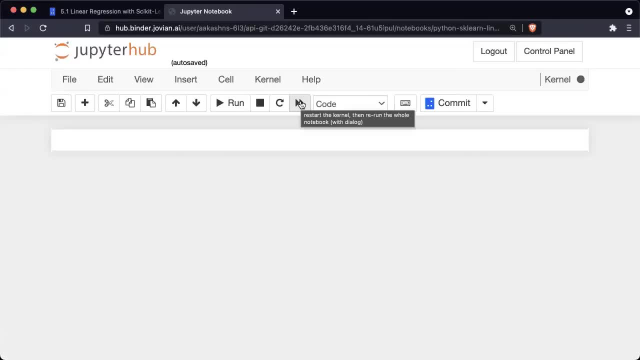 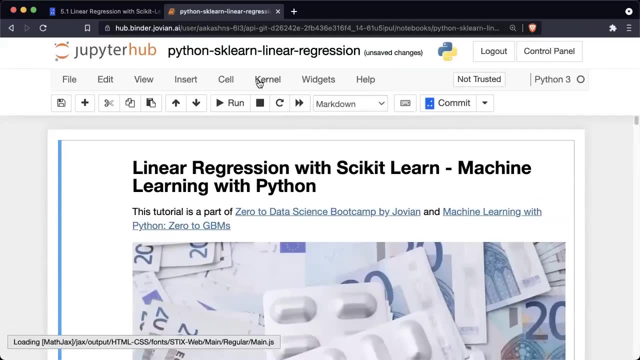 Hosted for execution. All right, It looks like we now have a Jupiter notebook running on the cloud, ready for us to edit and execute, So the first thing I like to do is click kernel restart and clear output, so that we can get all the outputs from scratch ourselves. 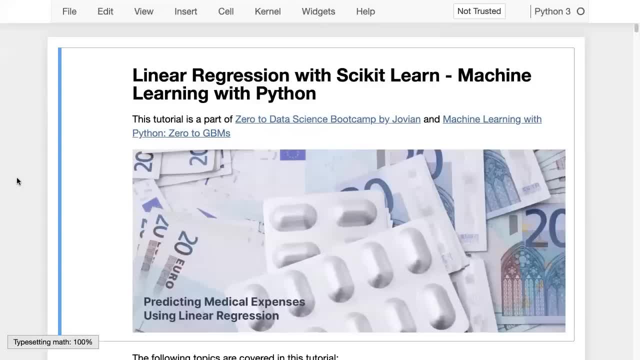 And let's just zoom in here a little bit. So the topic for today is linear regression with scikit-learn. This is the first topic We are covering in machine learning with Python. So here's an overview of what we are going to cover. today is to quick outline. 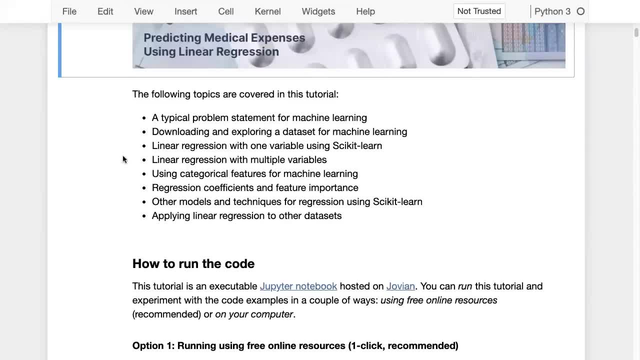 So first we'll start by stating a typical problem statement for machine learning. Then we will download and explore a dataset. Then we will perform linear regression with one variable using scikit-learn. Then we'll perform linear regression with multiple variables- and don't worry, if these terms don't make sense right now, they will by the end of this session. then we'll use categorical features. 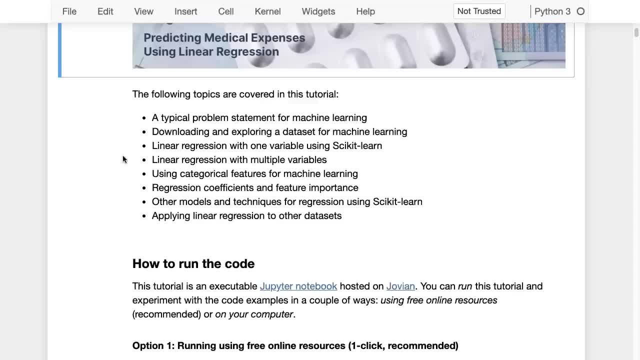 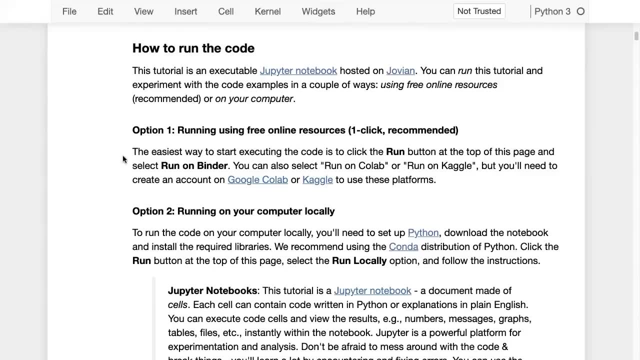 For machine learning. learn how to apply that in general, not just for linear regression. So this tutorial is an executable Jupyter notebook hosted on Jovian and you can run this online on binder or you can run this on your computer as well. 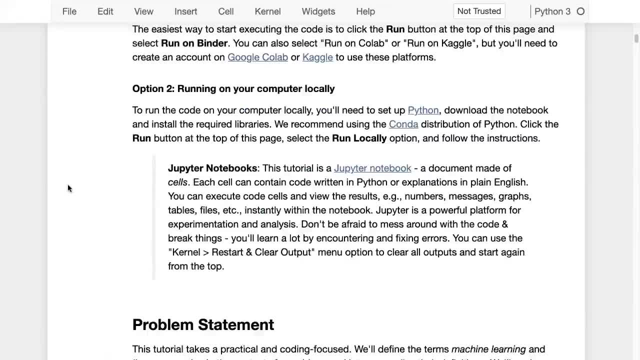 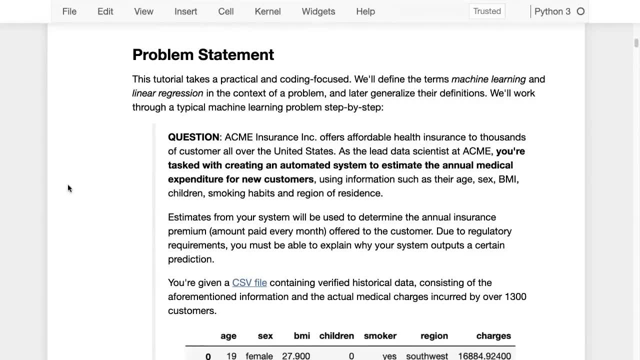 You can also run this on Google collab, and that's perfectly fine too. So here's the problem that we will solve today, and, using this problem, We will Define the terms machine learning and linear regression in the context of this problem, And then later we'll generalize their definitions. 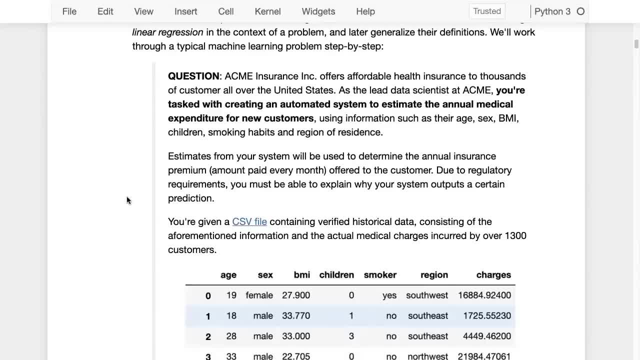 Let's read the problem carefully And then we'll think about how we can approach this problem. Acme insurance incorporated offers affordable health insurance to thousands of customers all over the United States And as the lead data scientist at Acme, you are tasked with creating an automated system to estimate the annual medical expenditure for new. 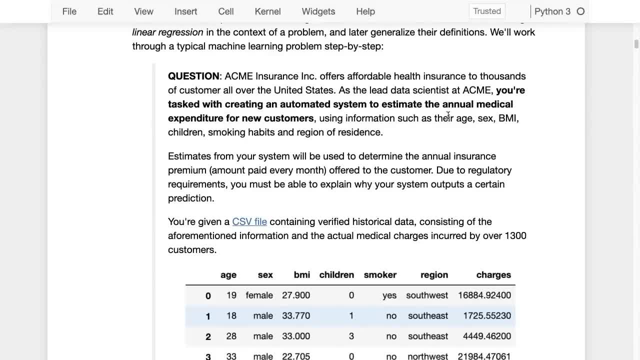 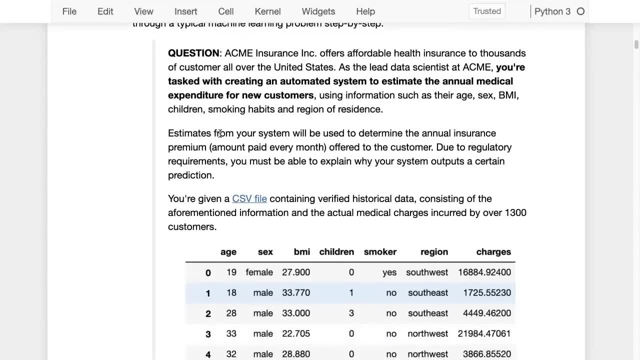 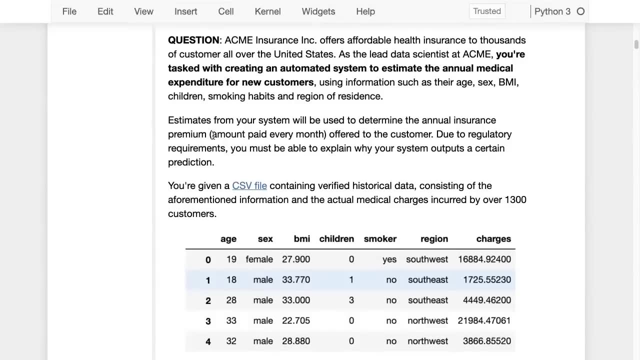 Customers using information such as their age, sex, BMI, children, smoking habits, region of residence, et cetera. Why are you asked to do that? Because estimates from your system will be used to determine the annual insurance premium, which is the amount paid every month or every year that is offered to the customer. 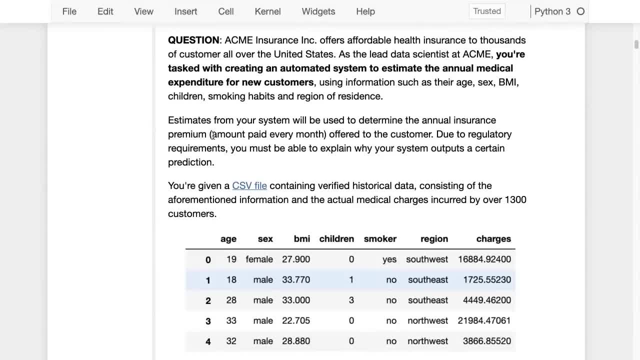 So your job is to figure out, when a new customer applies for medical insurance, based on information Like their age, sex, BMI, et cetera, how much they might incur in medical bills in an average year. if you can find that information, along with some other information, can be used to determine what you should charge the customer for insurance right. 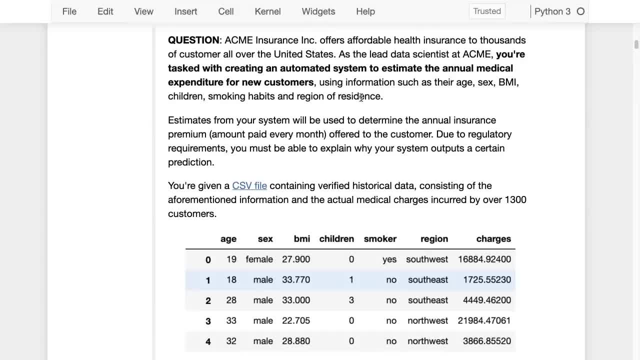 This is a typical problem that you will face, and it's a typical example of a machine learning problem where you want to replace some manual decision-making, or one Pro one For one piece of a manual decision-making process with some automation. So in this case, for example, you may need an expert who has seen customers for several decades to figure out, based on this information, what their medical information might look like. 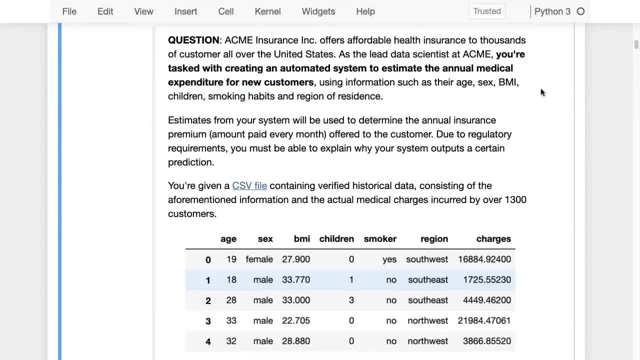 Or if you're a data scientist, you can figure that out using data, And that's what we're going to create today. You need some data to actually figure this information out, but fortunately, because Acme insurance already has thousands of Customers- 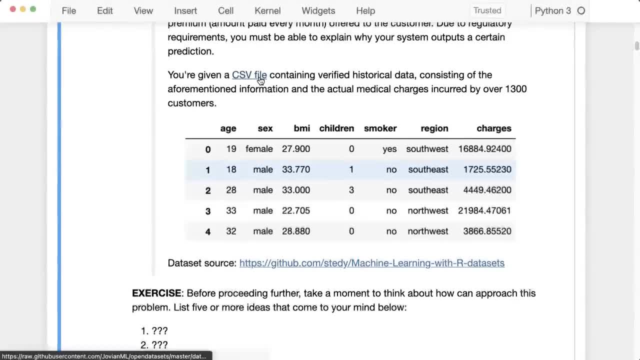 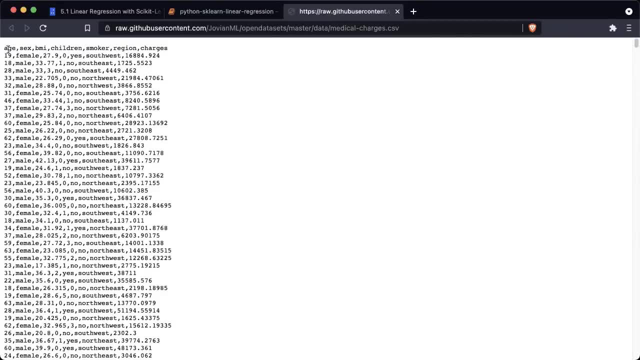 They have given you a CSV file. So here's a CSV file that your manager, or whoever is working on this project, has given you, And this CSV file contains historical data, Let's say from the past year, for over 1300 customers. you can see here. we have information like age, sex, BMI, the body mass index, number of children, whether this person is a smoker or not, which region of the country. 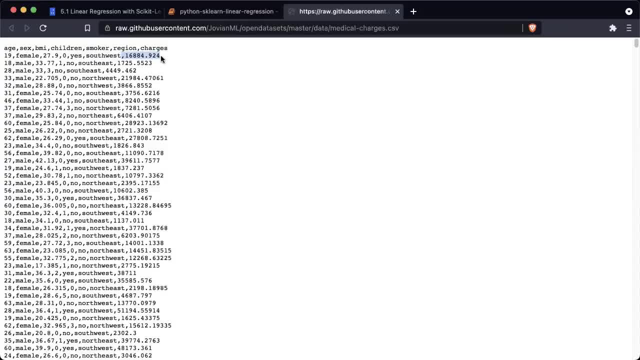 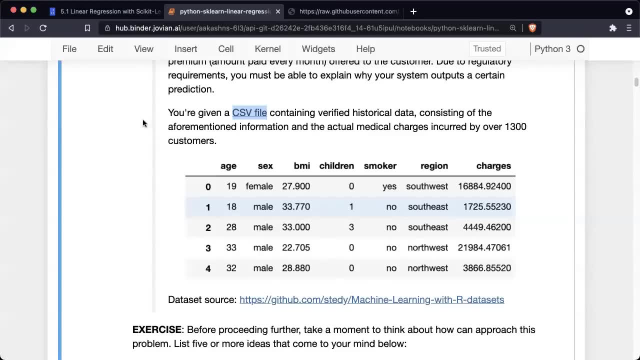 They belong to and the actual medical charges they incurred in the previous year. All right, So we have some historical data and we would want recent historical data not going too far behind, because medical charges can change due to inflation and due to other reasons as well. 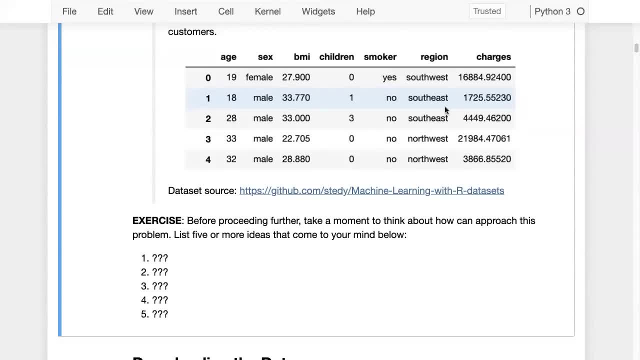 So that's the data you have, and your job is to create some kind of a system which can take this information- age, sex, BMI, children's smoker region- for a new customer And estimate what their charges are going to be over the coming year. 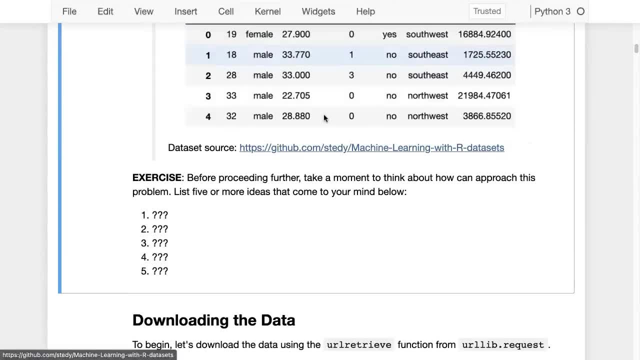 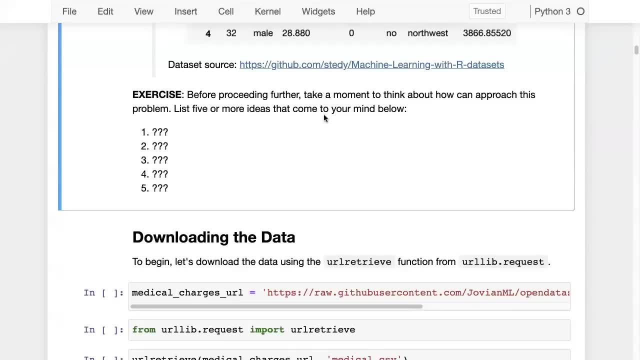 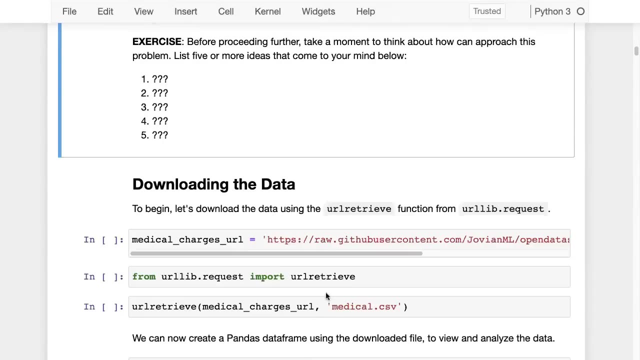 And here's a source for this dataset. This is a popular dataset that is used in machine learning. Now, before we proceed further, just take a moment to think about how you can approach this problem And, as you think through it, just post your strategy on the chat. but in the meantime, let's begin by downloading the data. 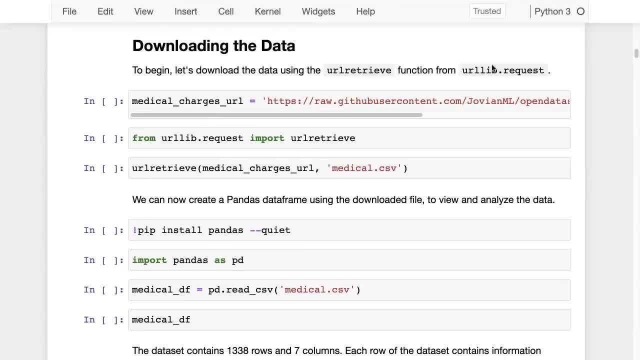 So we will Download the data using the URL retrieve function from URL lib dot request. This is a simple function that's already present in the Python standard library URL, So let's get the URL into a variable called medical charges URL and let's import from URL lib dot request from URL lib dot request the URL retrieve function. 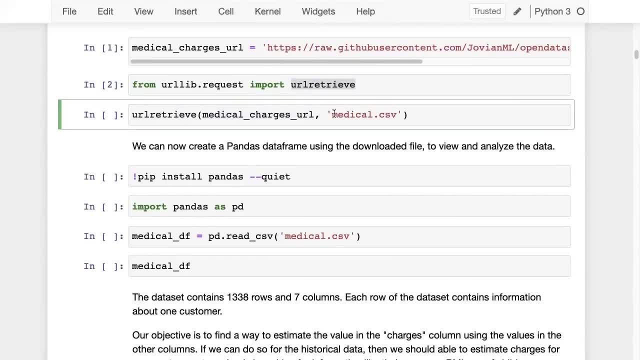 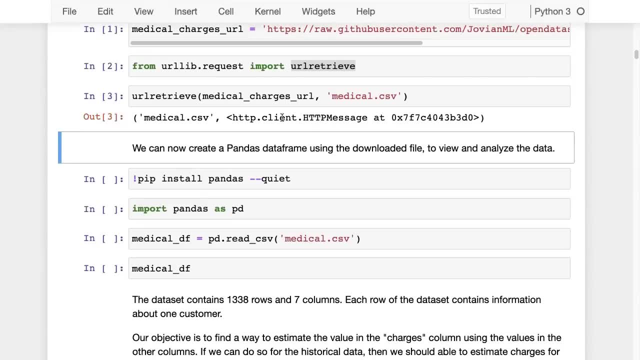 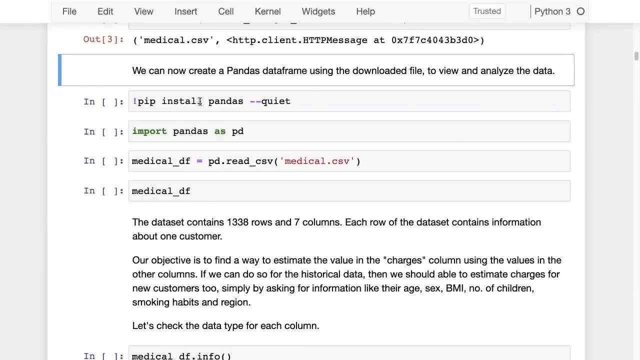 Let's call you, I will retrieve with the medical charges URL and let's download the data to this file- Medical CSV. Okay, So now we have a file- medical dot CSV- which should have the required data. next is to create a pandas data frame using the downloaded file to view and analyze the data. 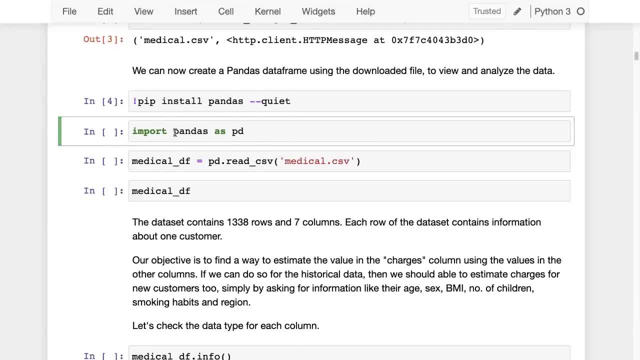 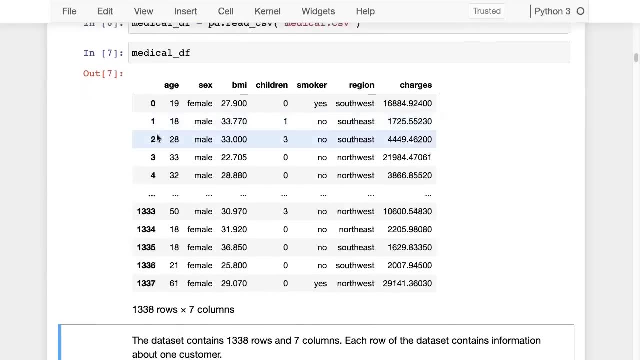 So let's install the pandas library using pip and then we import pandas using the alias PD and then we call PD dot read CSV and give it the name of the CSV file, And here we have the data frame. So the first step is to get the data into your Jupiter notebook, no matter what kind of problem you're working on, whether it is data analysis or machine learning. 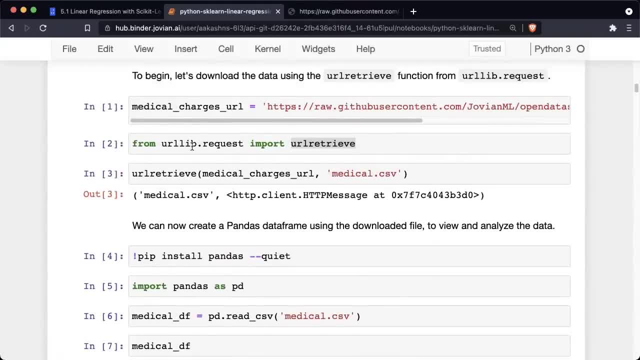 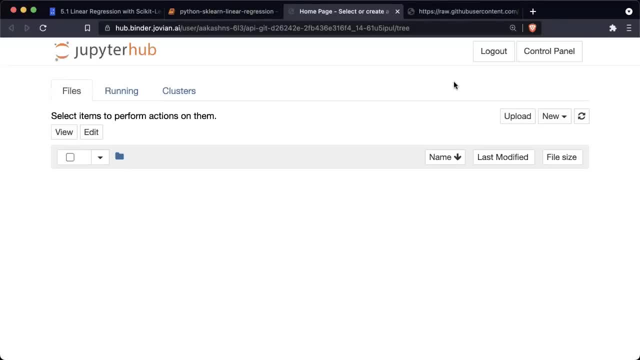 And one way to get the data is by downloading it using URL Lib. The other way to do it is you can go file open and then you can click the upload button here. You can click the upload button here and upload the file from your computer. 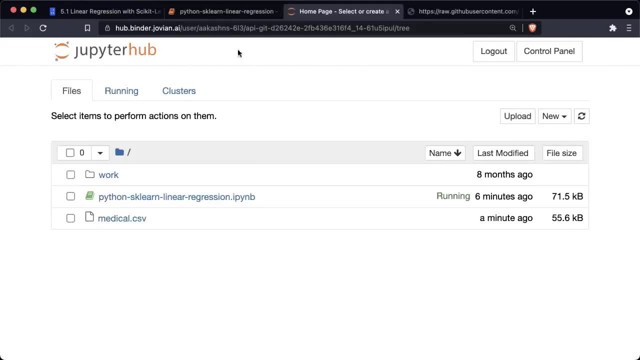 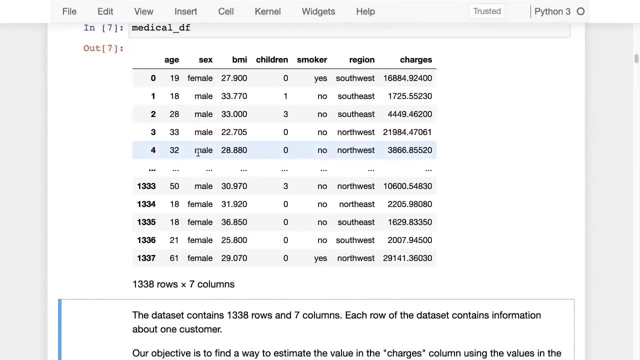 We've also looked at other Ways to download data sets, for example from Kaggle, and we will apply all of these different techniques at different points in this course. So here's the data, And this data contains 1,338 rules and seven columns. 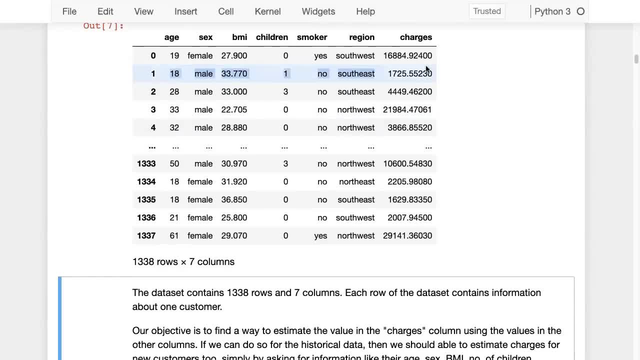 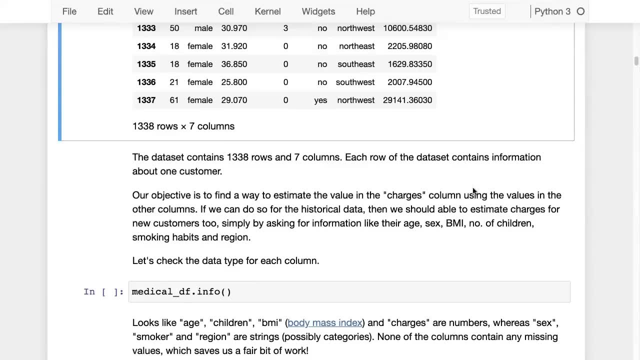 Each row of the dataset contains information about exactly one customer. Our objective is to find a way to estimate the value in the charges column using the values in the other columns. Now, if we can do so for historical data, then we should be able to estimate the charges for new customers too. 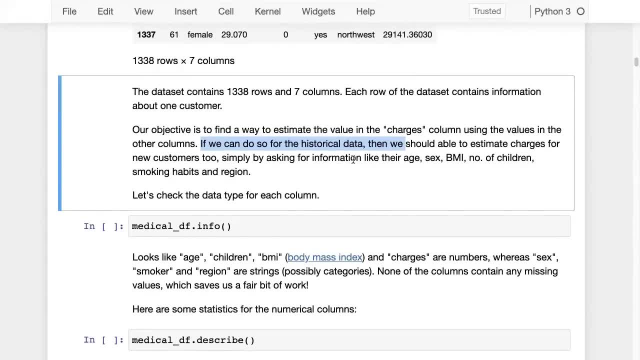 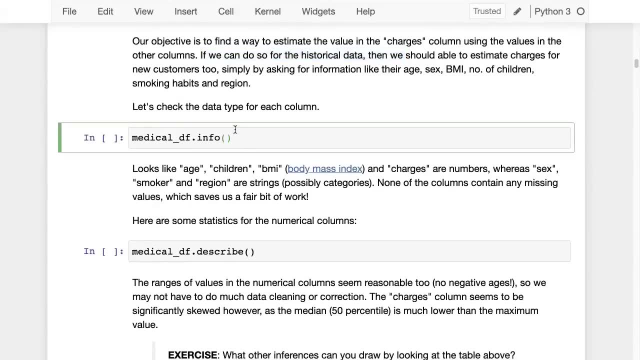 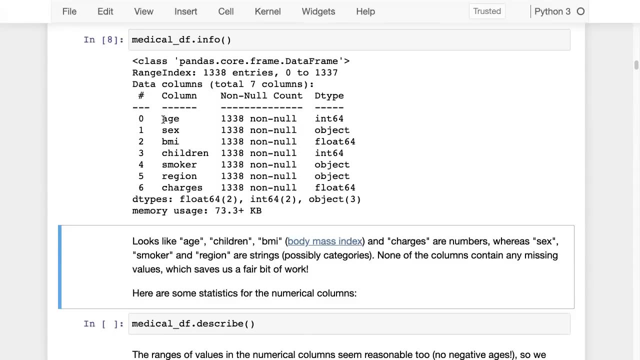 Simply by asking for their information like age, sex, BMI, et cetera, maybe in an application form. Okay, So let's first check the data type for each column. We go medical DF dot info and we have seven columns age. 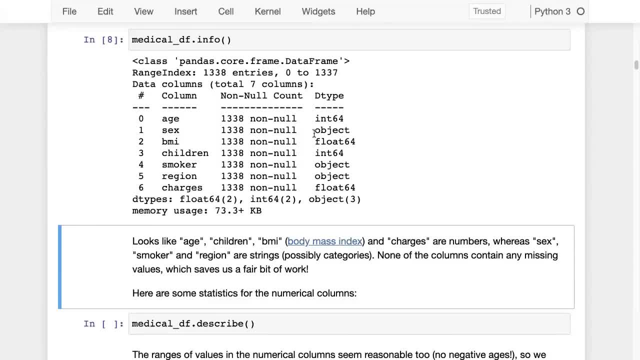 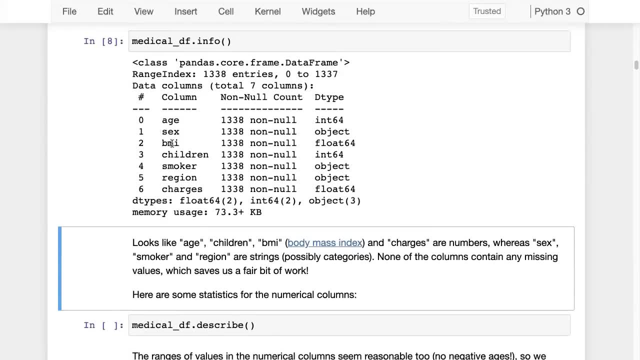 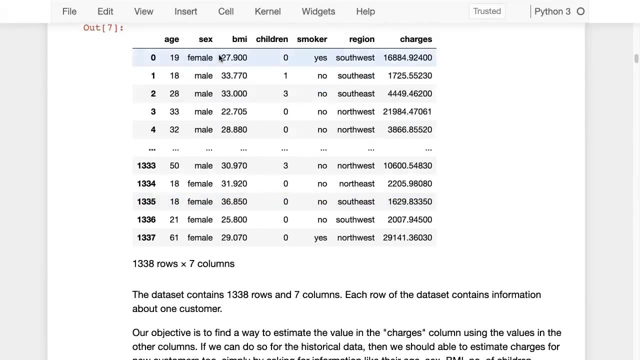 And it seems to be an integer. sex Seems to be a string, as you can see here, male and female, So actually it's more of a categorical column, but let's just call it a string for now. BMI seems to be a floating point number and you can see here in BMI we can have these decimals, each can also have decimals, but it looks like we've only collected the integer portion of the age. 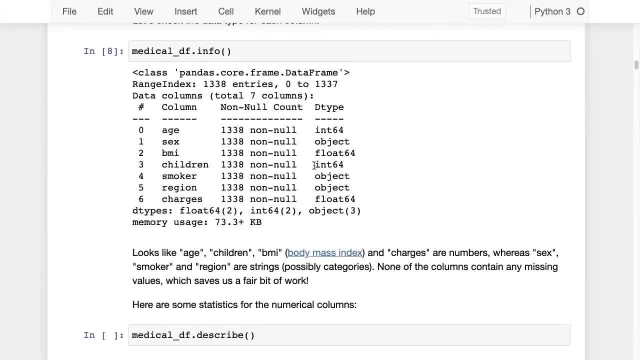 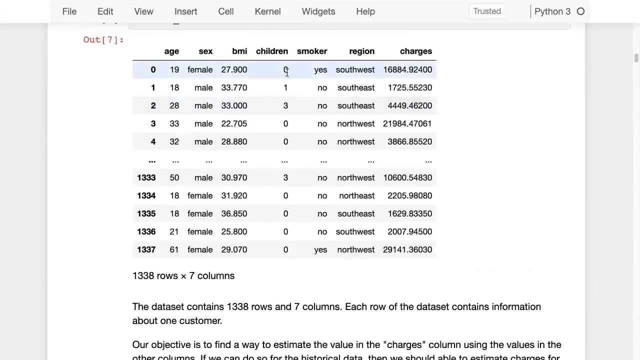 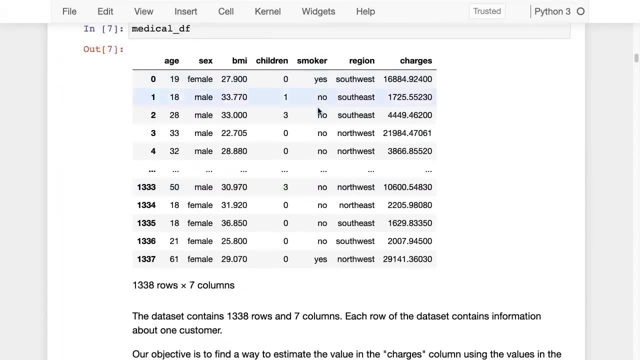 So that's what we're working with. Then we have children. This is the number of children The customer has, And this is again an integer, and typically this would be a number like zero, one, two, three. Then we have smoker, whether the person smokes or not, and this has a yes- no answer. 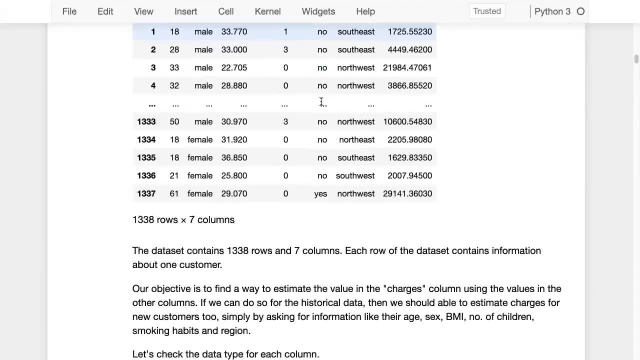 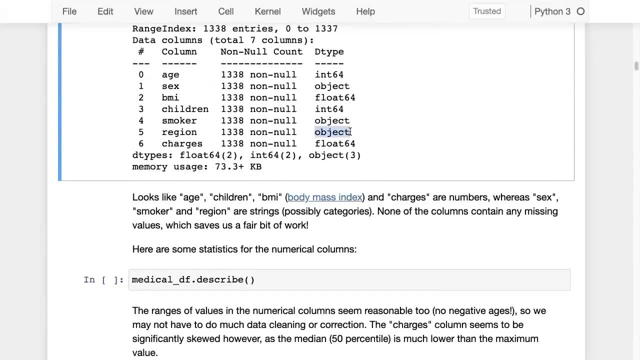 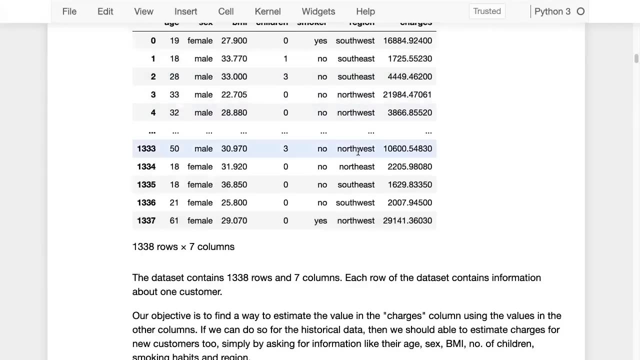 So this was probably a tick box somewhere in a form. So this is also a categorical column which we have in the form of a string right now. then we have a region, So it seems like there are different regions customers can belong to, like Southwest, Southeast, Northwest, Northeast. 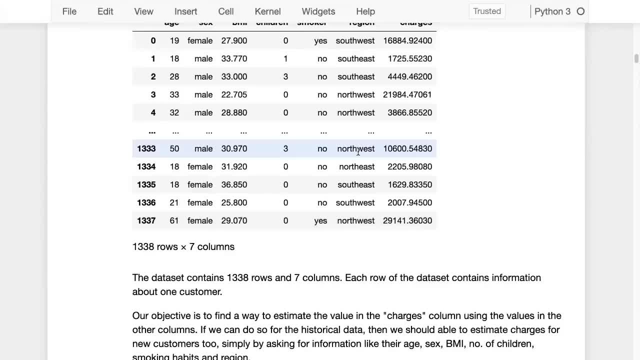 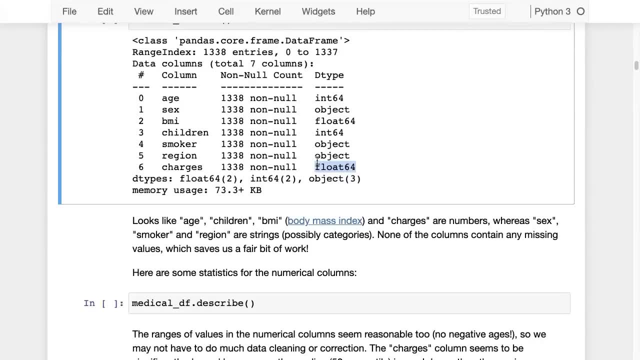 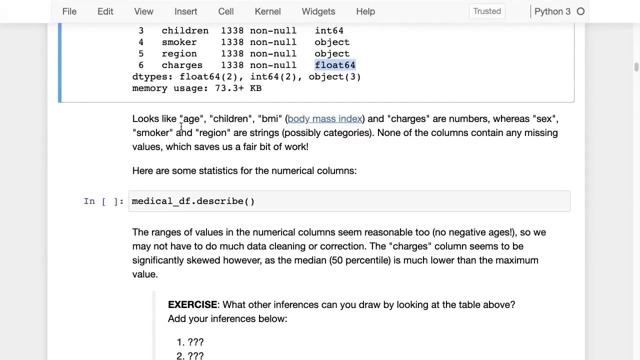 Seems like there are four of them, but we'll have to check. And finally we have the actual annual medical charges incurred by the customer. So there are numeric columns, and then there are categorical or string columns, And among the numeric there are integers and floating point numbers as well. 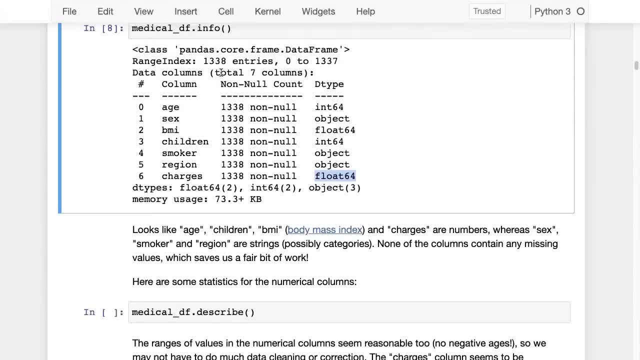 Now, one good thing here is that there are no null entries. If you see here non null count, that is one, three, three, eight, Which is also the total number of entries. So that means that there are no empty values in any columns. 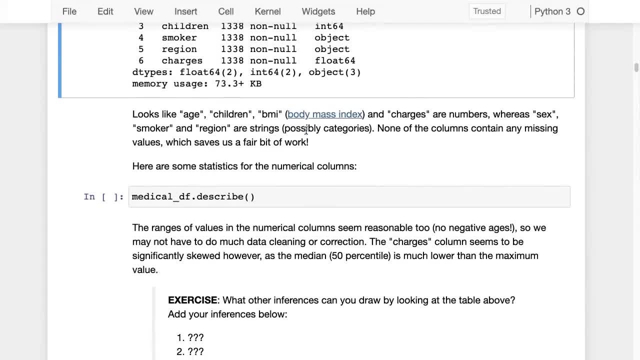 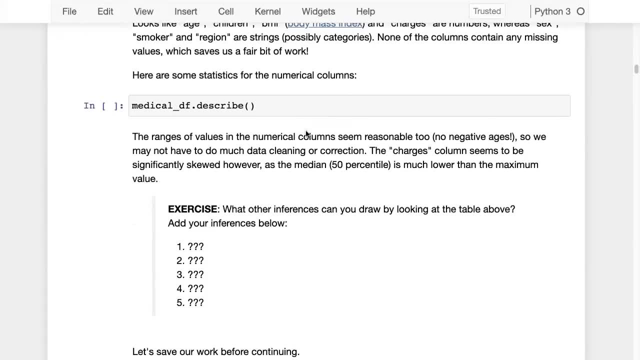 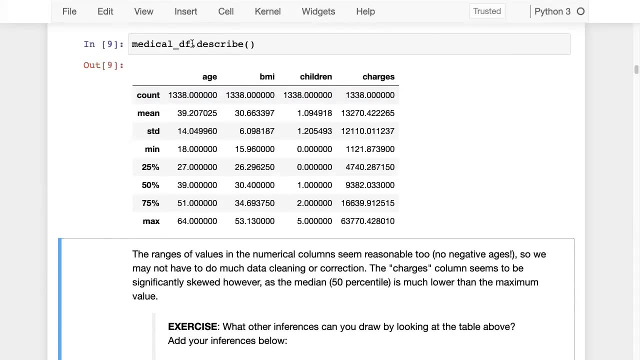 So none of the columns contain any missing values and that already saves us a fair bit of work. but don't worry, We will deal with missing values in future lessons. Next let us look at some statistics or the numerical columns. So if we call medical DF, dot describe, that is going to give us information like the count means standard deviation, minimum value. 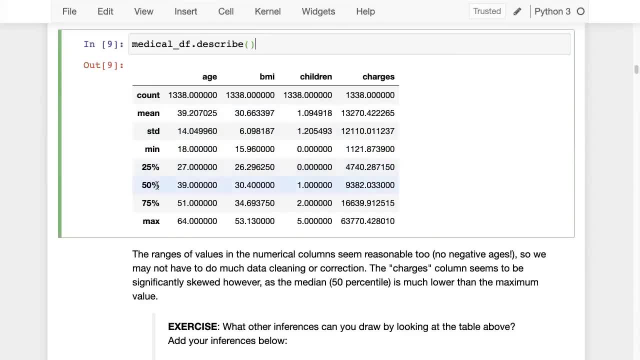 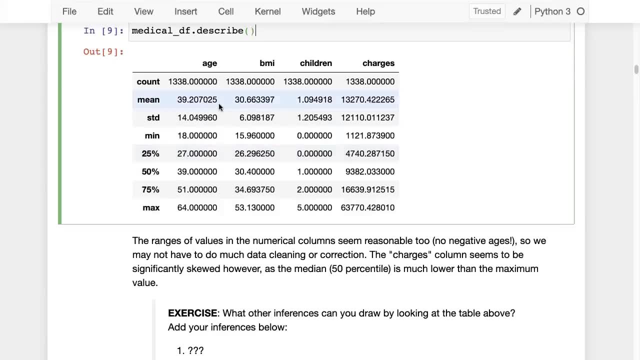 Okay, And all the percentiles, like 25 percentile, 50 percentile, which is the median, 75 percentile and the maximum. And this is always a good thing to do at the very beginning, just to see if the data, the range of data, makes sense. 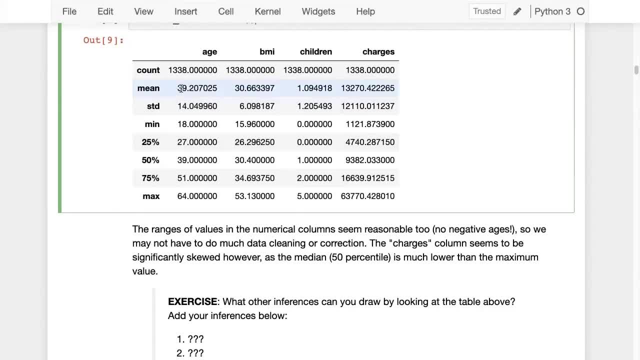 And I would say that the data makes sense. Seems like the average age is around 40. Seems like the standard deviation is 15, minimum is 18.. Maximum is 64.. Okay, We already know that 18 is the minimum age, 64 is the maximum age. They both seem reasonable. but this also tells us that perhaps the Insurance company does not take applications below the age of 18 or above the age of 64. Then we have the BMI. So with the BMI it seems like the minimum is 15.. 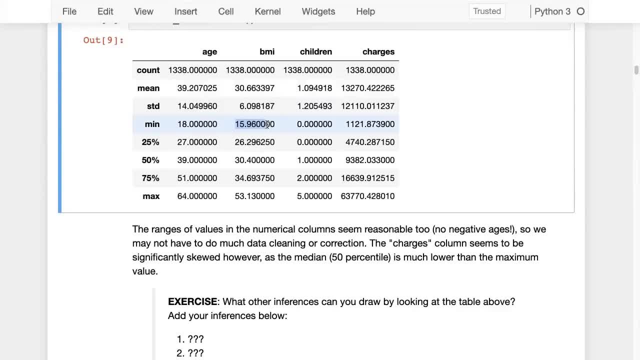 So the BMI, just to give you a sense, is the mass of a person in kilograms divided by the square of their height. So it's a ratio of mass or weight to the square of a person's height in meters. So BMI this is in the units kilograms per meter square. 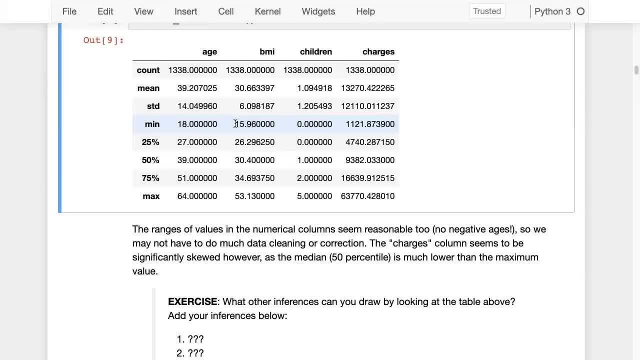 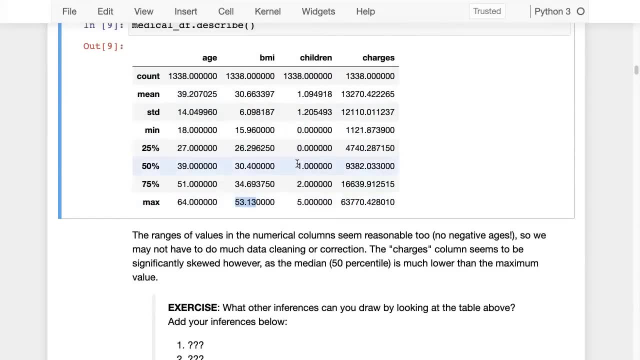 So it seems like the BMI is, the minimum is around 15.9,, six or 16.. And the maximum is around 53.. Okay, Then we have the number of children. that goes from a minimum of one to a maximum of five. Then we have them at actual medical charges, which go from a minimum of one one to one, So just a thousand dollars- this person basically did not go to the hospital at all during the year- to a maximum of $64,000.. So you can see that there is a huge. 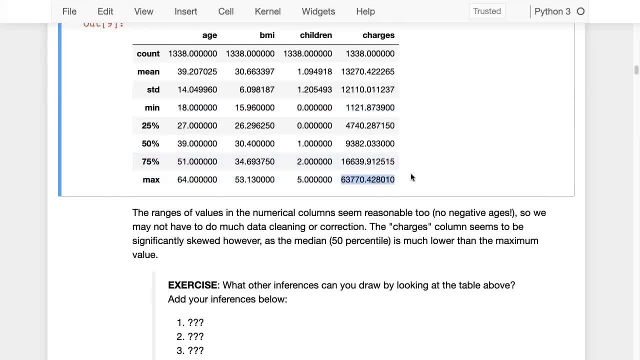 Huge Variation in the charges, from thousand to 64,000.. Not only that, you can also see that if you check the 50% mark, 50% of people have their medical charges under $10,000, or even 75% habit under $16,000. 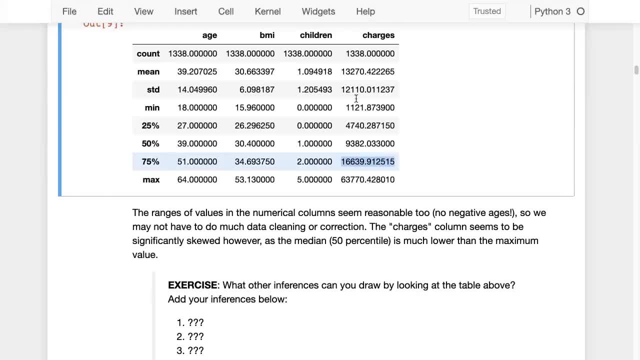 So that means there is a huge skew or there are several outliers in the charges column, And we'll see that in more detail once we study the visualizations. but even just by looking at these numbers you can tell some of these things The mean. 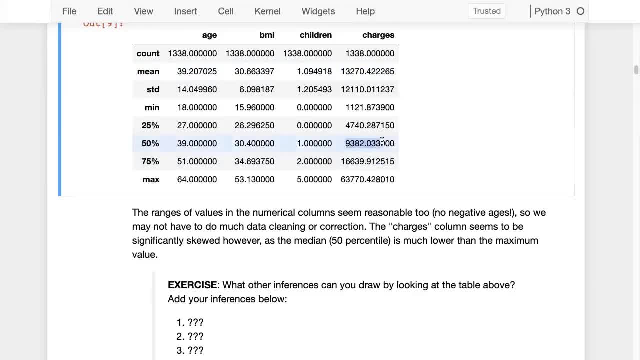 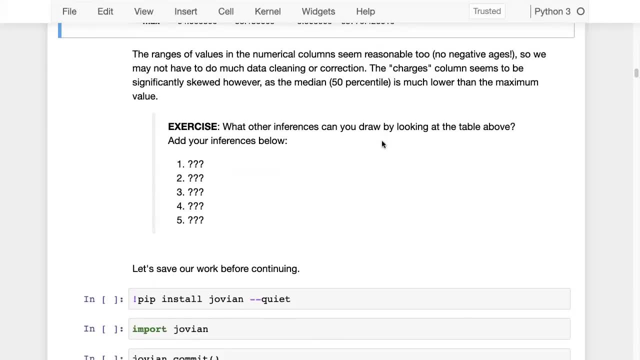 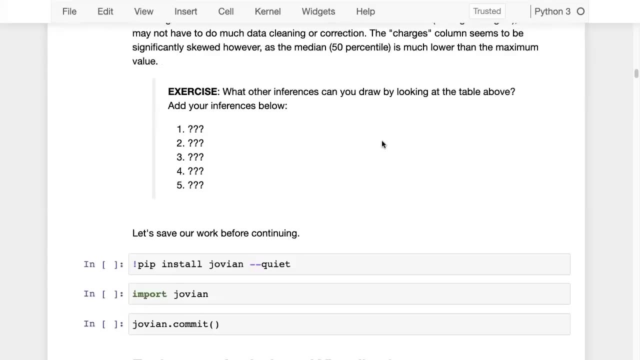 Is 13,000, but the 50% mark is 9,000. So there's a bit of a skew in the data. So this is what you should do Whenever you load up a data frame: just look at the data, just look at all these statistics and try and draw whatever inferences you can. 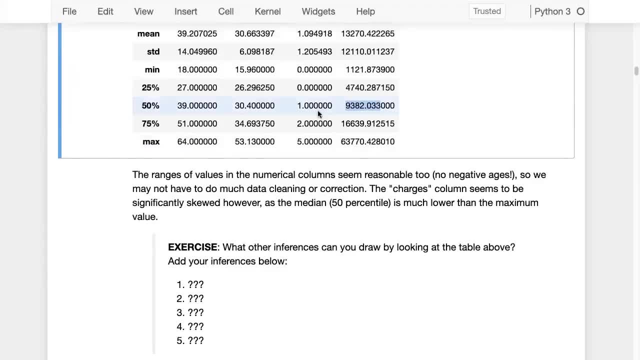 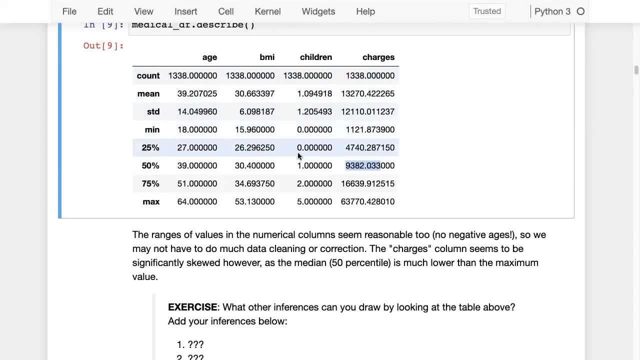 In this case, once again, there don't seem to be any incorrect values like negative ages or ages greater than 200,, let's say, or any Negative values. Everything seems nice and clean. So somebody has put together this dataset for us, made sure that it is pristine. 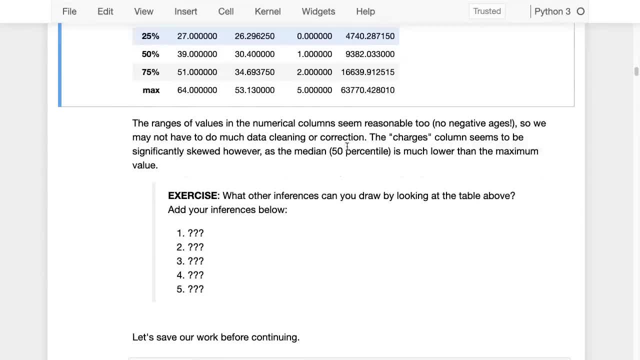 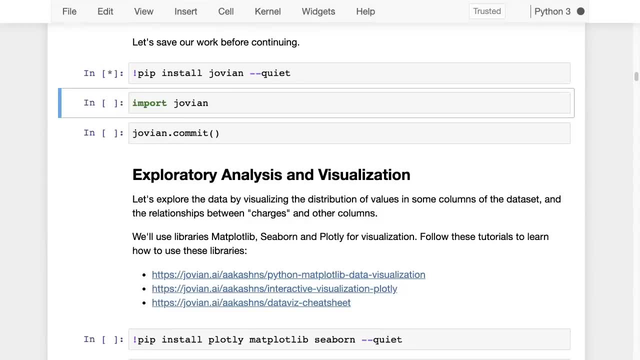 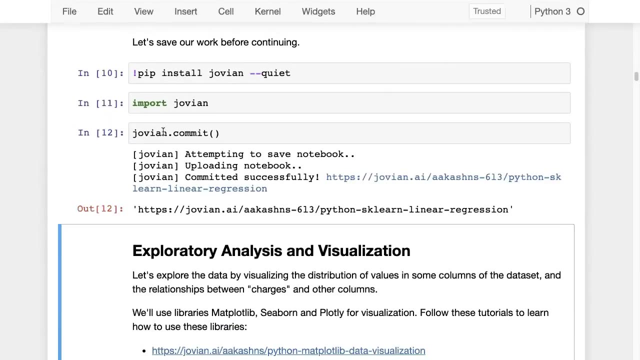 All the data is valid and there is no missing data. that makes our job a lot easier. So that was downloading the data, So let me just save my project at this point. I'm just going to import the Jovian library and click Jovian dot commit. 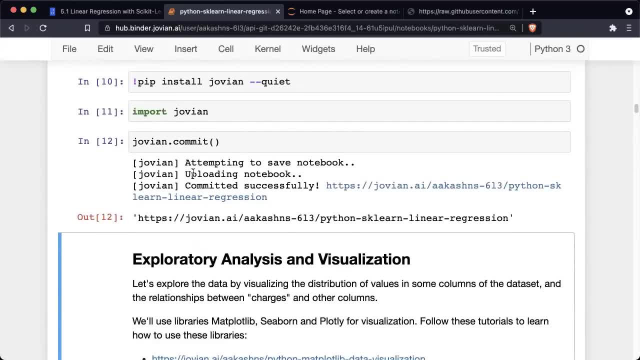 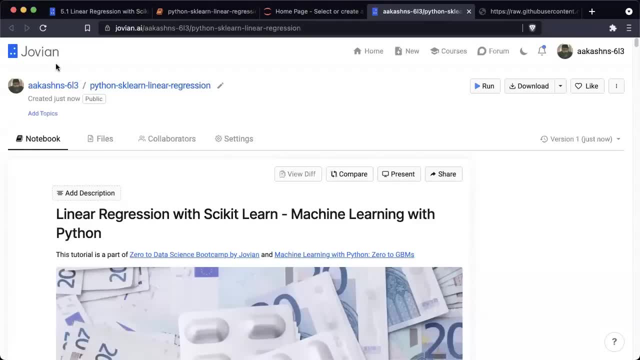 And when I run Jovian dot commit, a snapshot of this Jupiter notebook is taken and saved to my Jovian profile. So if I go to Jovian dot AI on my profile I will be able to find this notebook. So this is the notebook page where I can see the notebook again and I can run it again by clicking the run button. 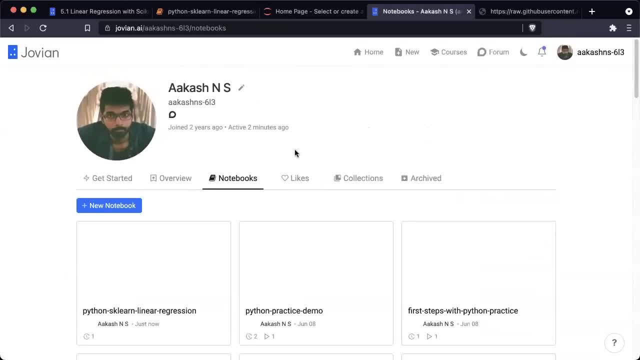 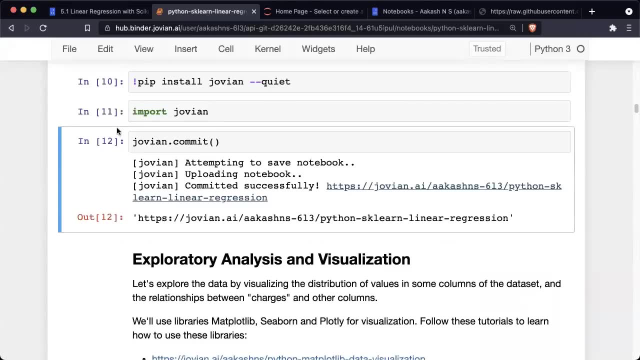 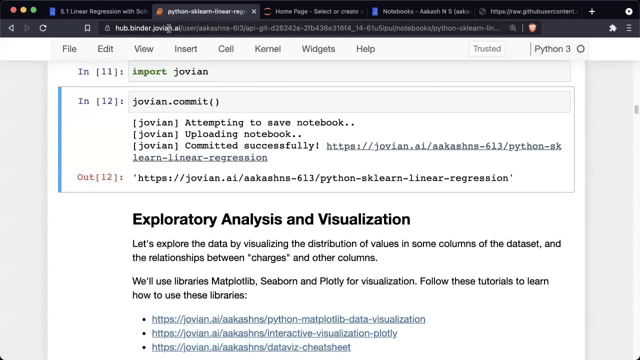 And if I go back here on my profile, under the notebooks tab, I can find the same notebook, Python, SQL and linear regression. So make sure you're saving your Notebook Book from time to time, because the binder instance will shut down if you step away from it for 10 minutes. 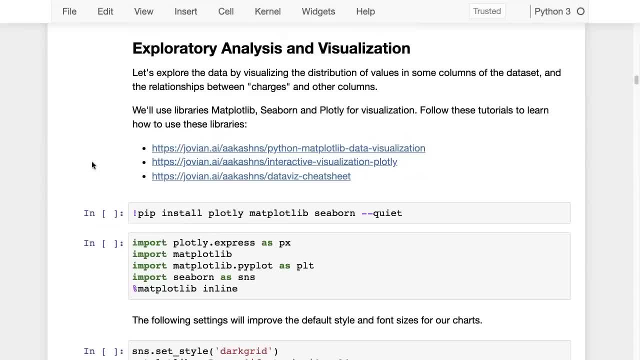 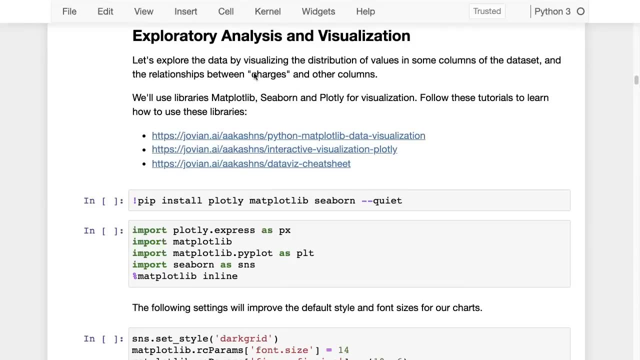 Okay. So now we've downloaded the data. So let's start by doing what we know. Let's start by just doing some exploratory analysis and visualization and let's see where that can take us. We will visualize the distributions of values in some of the columns and we will also find the relationships between the charges columns and the other. 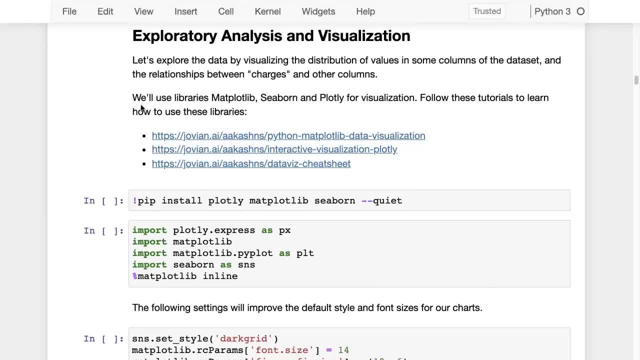 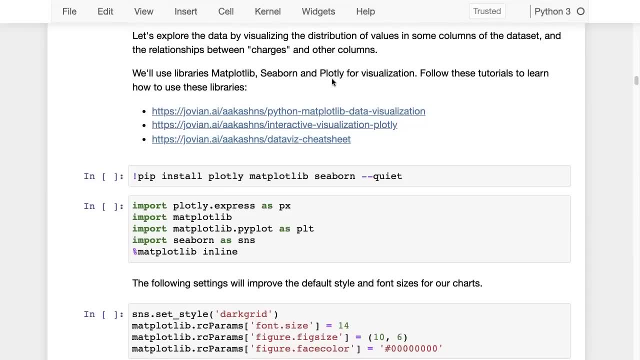 columns because we have to use the other columns to predict charges. And we will use the libraries matplotlib, seaborn and plotly for visualization. plotly specifically because it will give us some interactive charts and save us some coding. But a lot of all of these plots can be done using just matplotlib and seaborn as well. 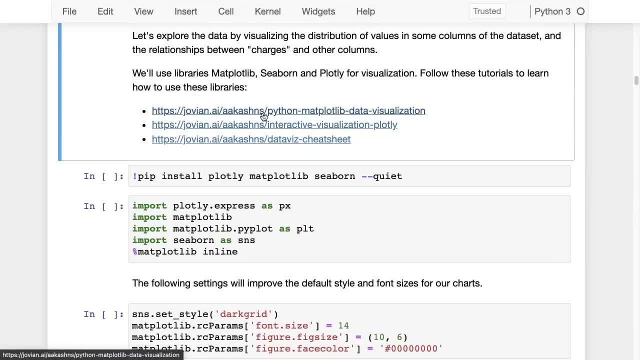 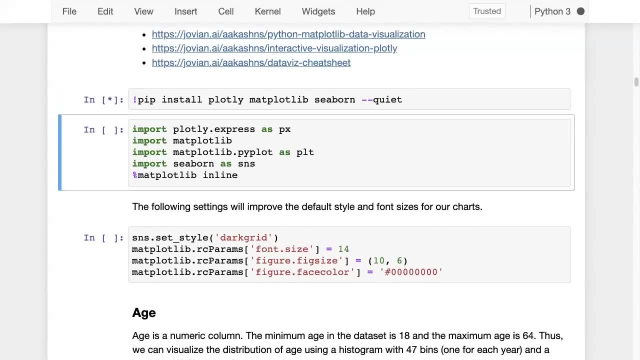 And I've linked to some tutorials here that you can check out in case you want to refresh or learn one of these libraries. So I'm going to To install these libraries, first using pip, All right, And then I'm going to import these libraries. 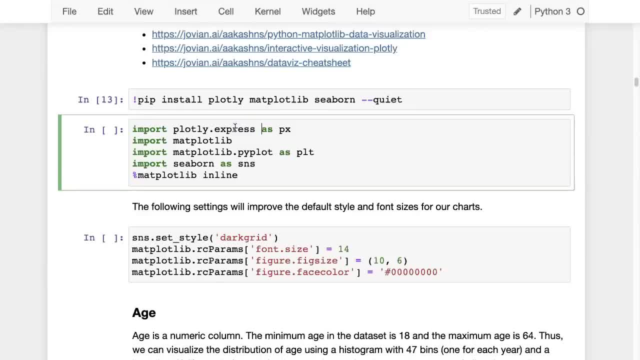 So I'm going to import plotly dot express, which is a high level API that makes it really easy to create plotly interactive charts. Then I'm going to import matplotlib and I'm going to import matplotlibpyplot as PLT. This is how typically 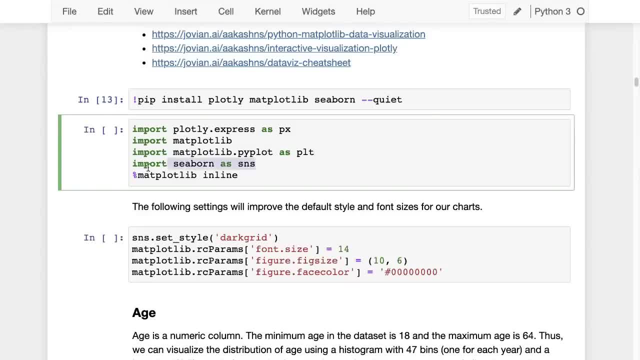 Matplotlib is imported. And finally, I'm going to import seaborn as SNS. So these are all the conventional ways in which these libraries are imported. One last thing we have is matplotlib inline. The purpose of this line is to ensure that any charts that you create, they show up as outputs within your Jupiter notebook and not as pop-ups, because when you close a pop-up, the chart goes away. 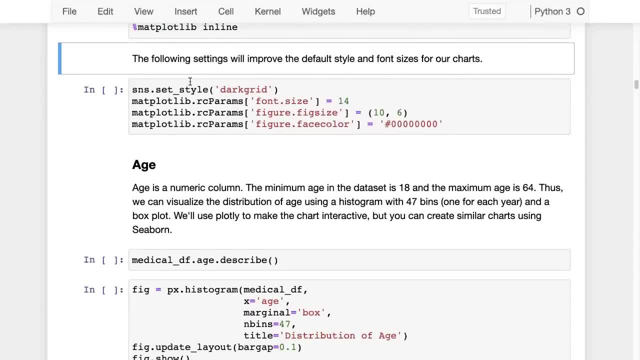 All right. So now we have imported the One other thing I'm going to do is just change some settings, which will improve the default style and the font sizes for our charts, which is going to make the font sizes a bit larger and use the dark grid style for seaborn. 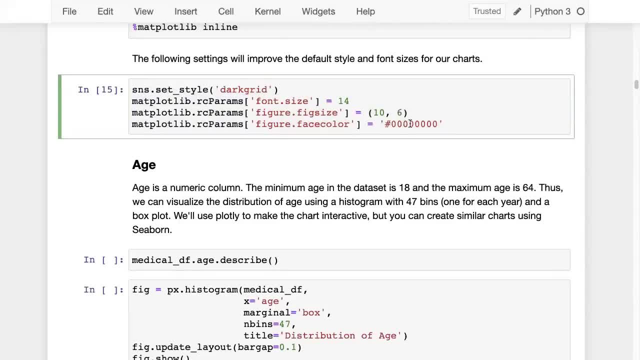 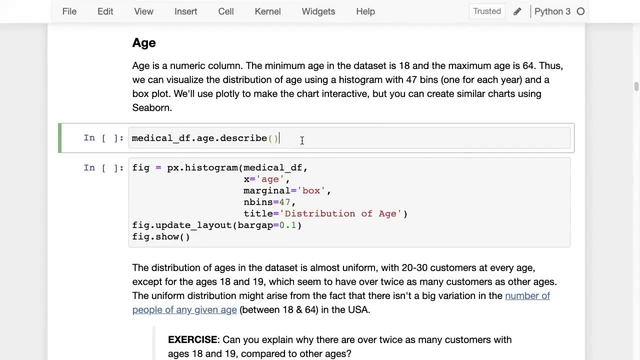 This will only apply to matplotlib and seaborn, not to plotly. Okay, Let's begin with the first column. age and age is a numeric column. The minimum age in the dataset is 18.. And the maximum age in the dataset is 64.. 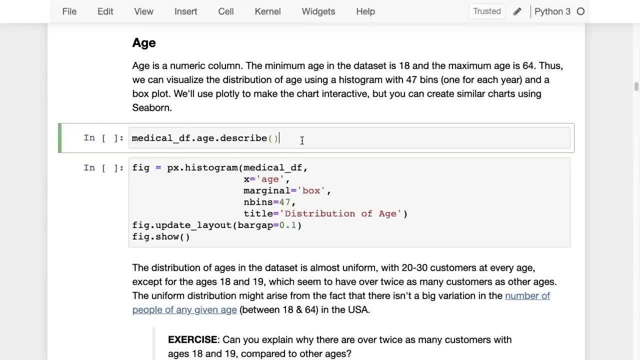 So we can visualize the distribution of age using a histogram, essentially trying to find out how many people, how many customers we have for every age from 18 to 16, four, So that means we need 64 minus 18 plus one or 47 bins, one for each year. 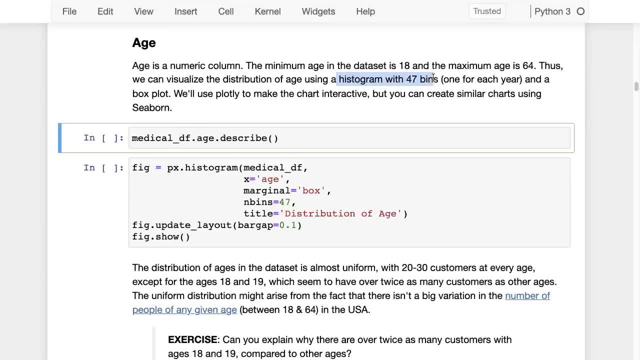 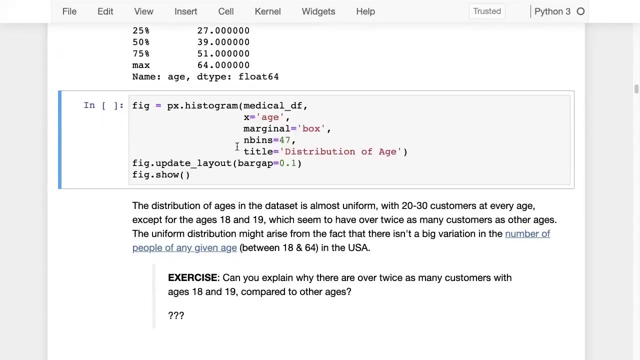 And that way we'll be able to visualize it using a histogram. Another useful plot is a box plot. A box plot is also quite useful because it tells you the minimum, the maximum, the median and all the quartiles, So that can give you a sense of the distribution, of of where the 50% point lies. and, using plotly, we can actually create both of these charts with just one line of code. 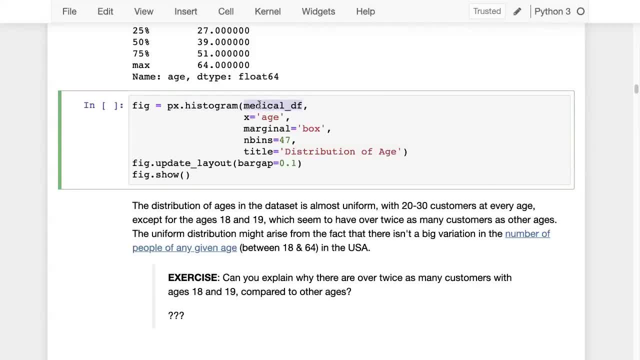 We say PX dot histogram- Okay, Okay, Pass in the medical DF data frame. And then we specify that we just want to use the age on the X axis and we want to use 47 bins and we want to give the charter title: distribution of age. 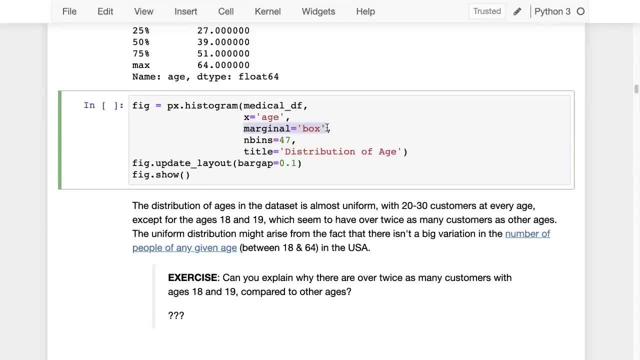 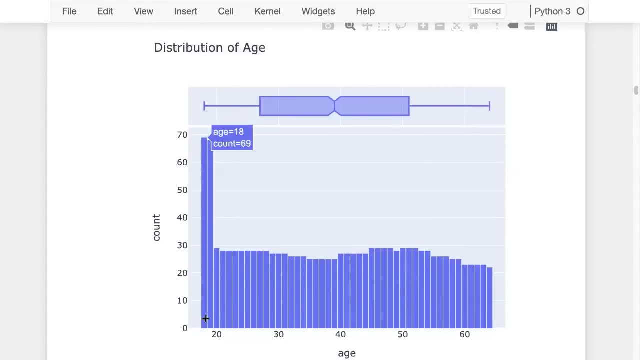 Now, by adding this marginal equals box parameter, plotly will also plot a box plot right above the histogram for us. So here's what the distribution of age looks Like. you can see here at the age of 18, we have 69 customers at the age of 19.. 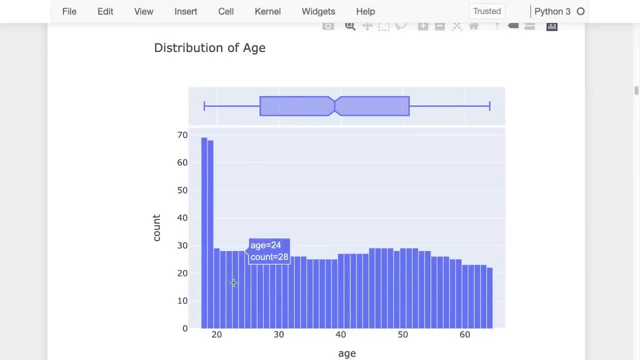 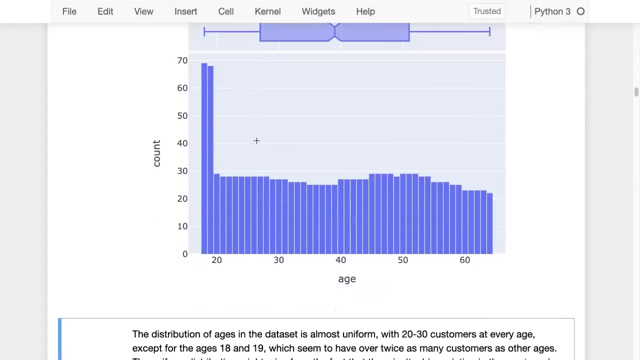 We have 68. Then we have anywhere from 20 to 30 customers at every age- seems like a lot of people here- in the range of 40 to 50. And then here we have the highest age, which is 64, and nobody beyond the age of 64, it's a nice uniform distribution, almost. if you just ignore these two values, you can see that the midpoint is around. 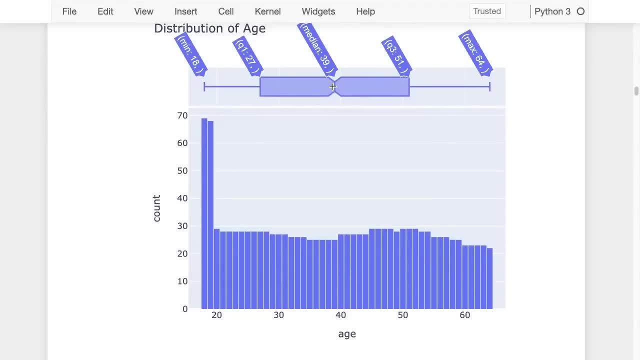 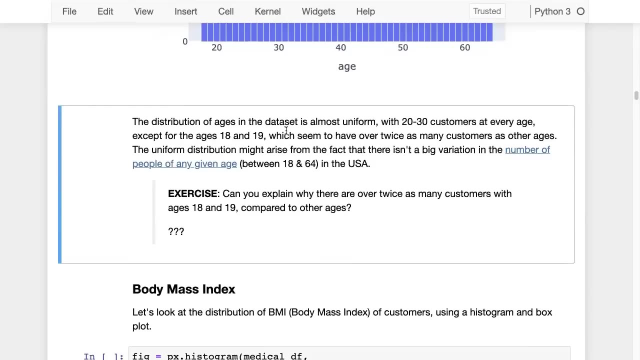 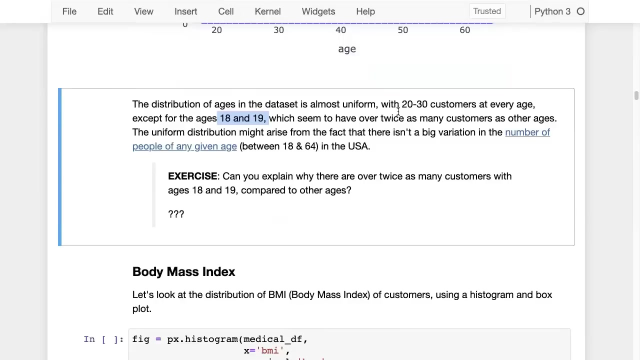 Okay, 39, and the quarters are also equally balanced on each side. So the distribution of ages in the dataset is almost uniform, with 20 to 30 customers for every age, except for the ages of 18 and 19,, which seemed to have over twice as many customers compared to other ages. 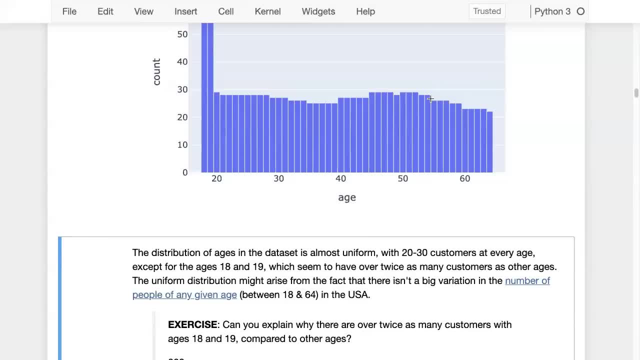 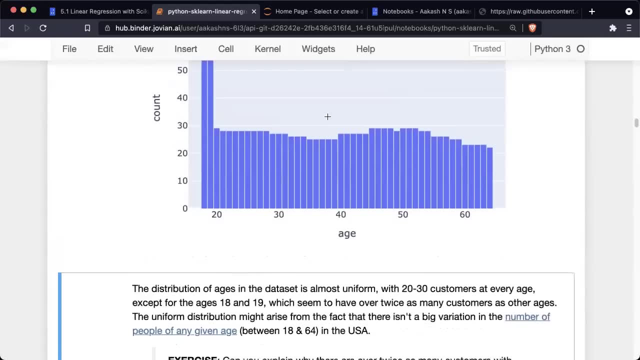 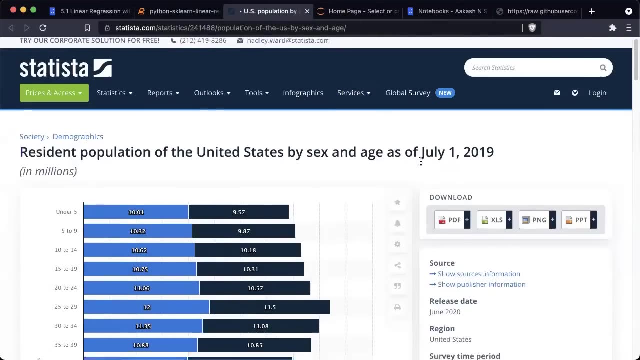 Now to explain this piece. the uniform distribution Might simply arise from the fact that there is not a big variation in the number of people at any given age, between 18 and 64 in the United States, For example. if we open up this other chart that's available online, this tells you the population and different age ranges. 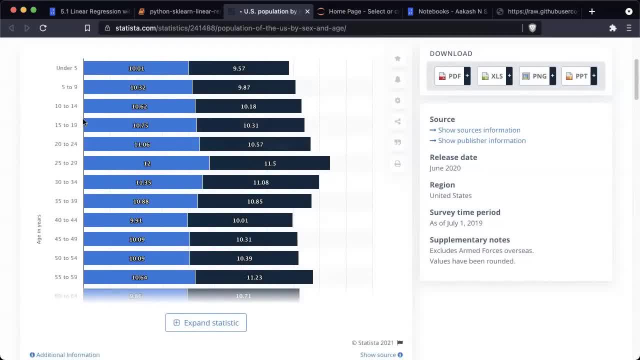 So you can see here 15 to 19,, 20 to 24,, 25 to 29.. So it seems like the split across male and female, but the overall population you can clearly see across different age groups is Fairly similar. 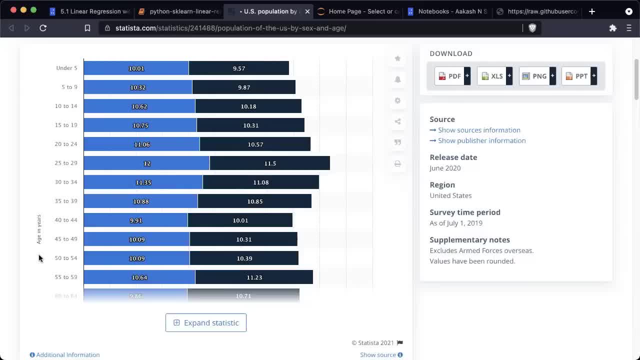 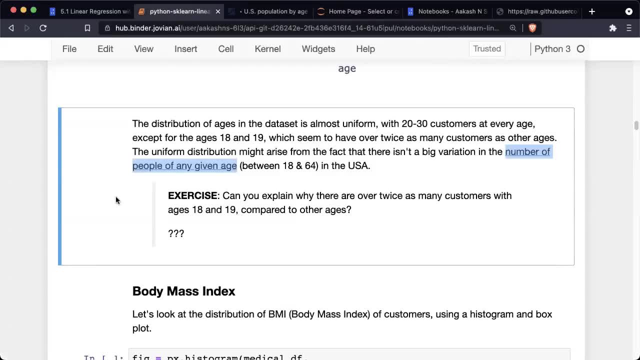 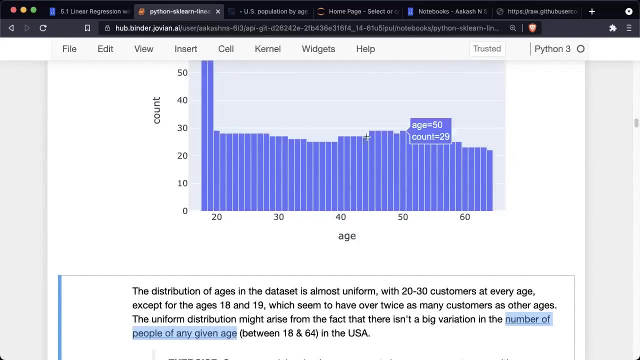 And you can assume that there is a certain percentage of people, a certain percentage of population, that takes their insurance from Acme insurance incorporated. So that's why you see this kind of a distribution which reflects the overall population. This is always something that you should check whenever you have a dataset. does the data you have reflect the distribution of the overall population or not? 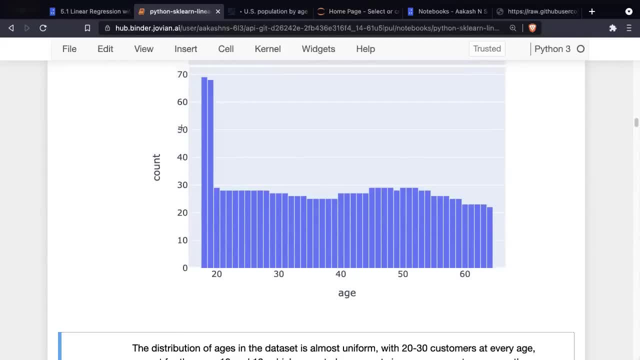 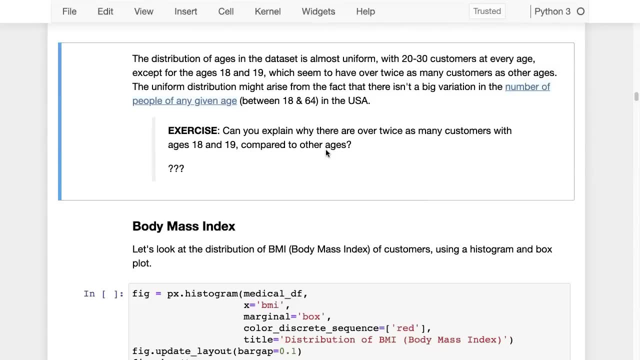 Well, in this case, in one case- it does not, And I will let you figure out why this might be the case. Can you explain why there are over twice as many customers with the ages 18 and 19 compared to other ages? 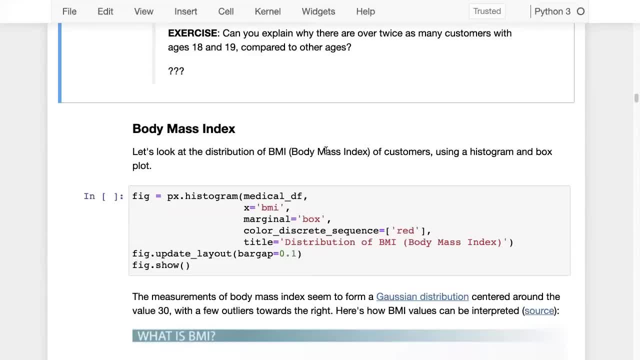 If I had to guess, I would probably guess that maybe Acme insurance is offering a lower insurance premium If you sign up before the age of 20, that could be one reason, and also because maybe 18 is the legal age for you to be able to get insurance. At least from this company. So a lot of people, as soon as they turn 18, get the insurance. That could be one of the other reasons, but neither of these we can assume. we would have to then go and verify if this is indeed the case. 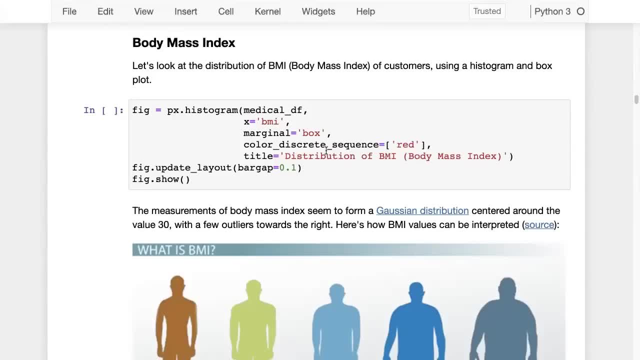 Maybe even look at some industry averages If we can find some reports online. Okay, So that was the distribution of age. It was mostly uniform, with a couple of Years where we had twice as many people. Next, let's look at the distribution of body mass index. 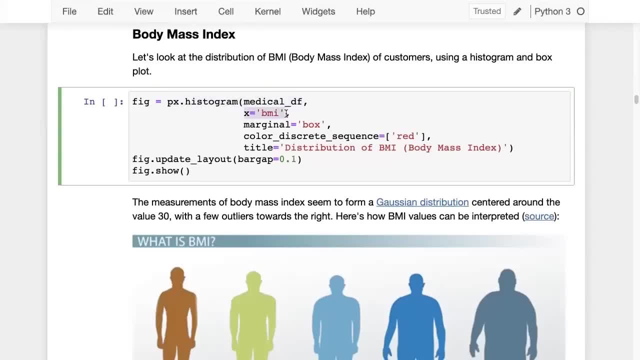 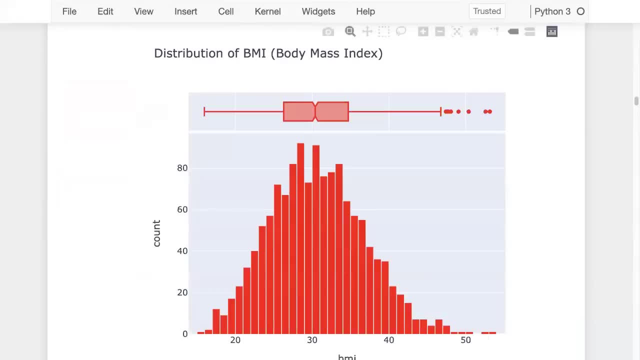 Once again, we are going to create a histogram of the body mass index, and this time we're going to use the red color and we're going to have a box spot once again. So here is a distribution of the body mass index and this looks very different. 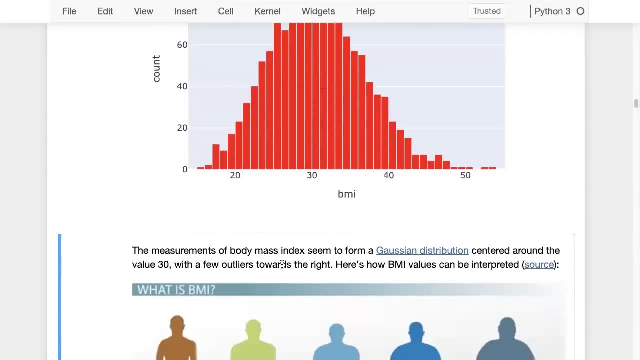 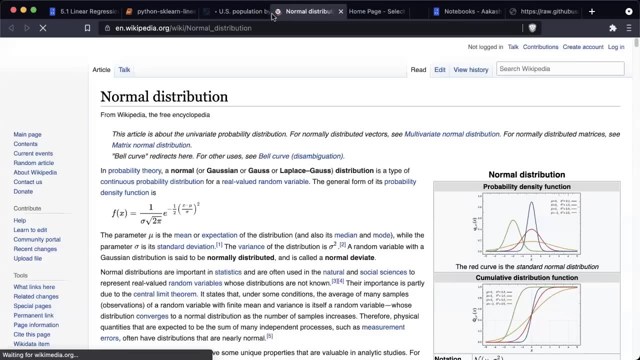 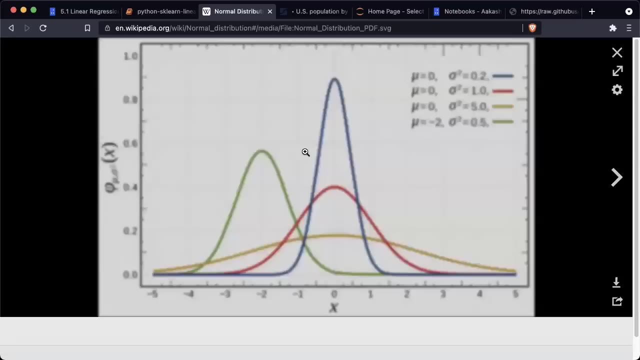 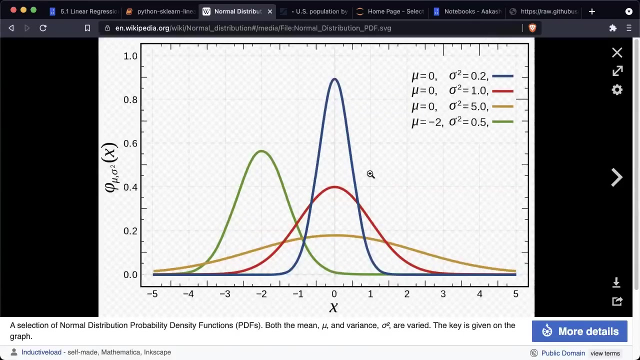 It seems like it is distributed according to a Gaussian Distribution, or what is also called a normal distribution. Here's what a normal distribution looks like. So if you have a certain population of data, yeah, this is the one. So if you have a certain population of data where most of the values are centered around a single value, the what is called the mean, and then you have a decreasing probability as you go away from that mean, that's called a normal or Gaussian distribution. 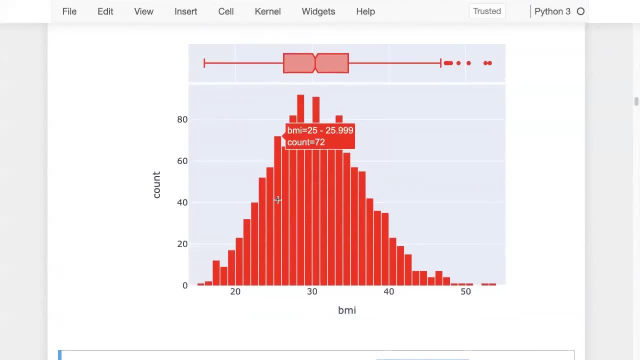 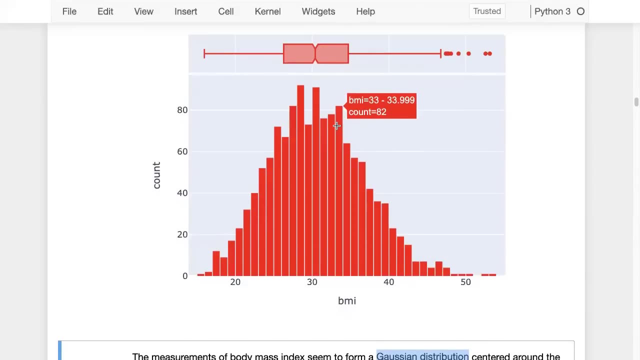 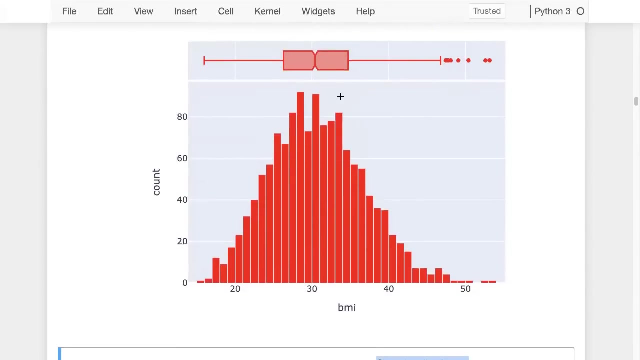 Right, And this is exactly what is visible here. Why is this Gaussian and why is the previous one normal? I let you think about that, but what we can notice here with BMI is that most people have a BMI, or a body mass index, around 30, maybe in the range of 25 to 35. 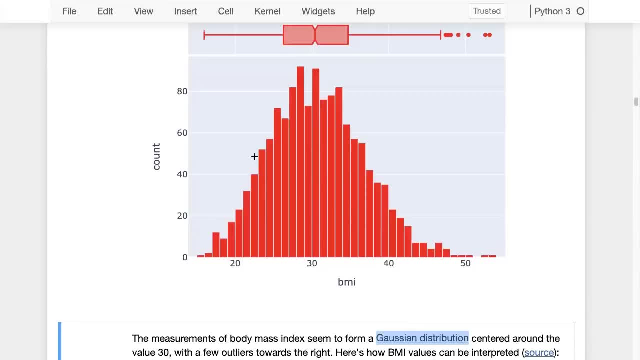 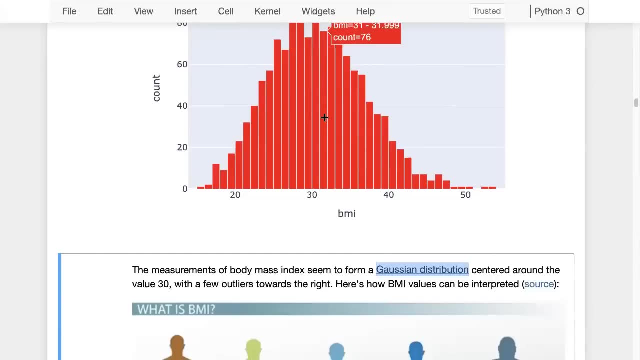 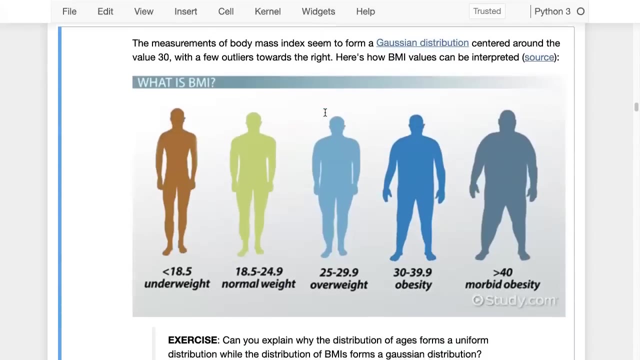 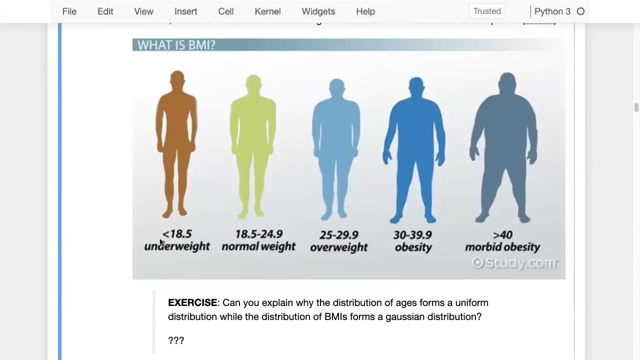 And then, as you get further away, fewer people seem to have that BMI. So 25 to 35,, roughly speaking, might represent the average human In terms of the ratio of weight to height, and here's how you can interpret body mass index values, or this is how that typically interpreted: less than 18.5 is considered underweight. 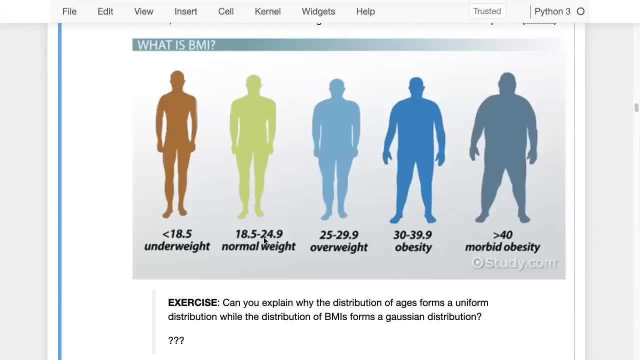 And then 18.5 to 24.9 is considered normal to overweight is well, 25 to 29.9 is considered overweight, slightly more than 30,. 30 to 39 is considered obese and greater, Then 40 is considered morbid obesity. 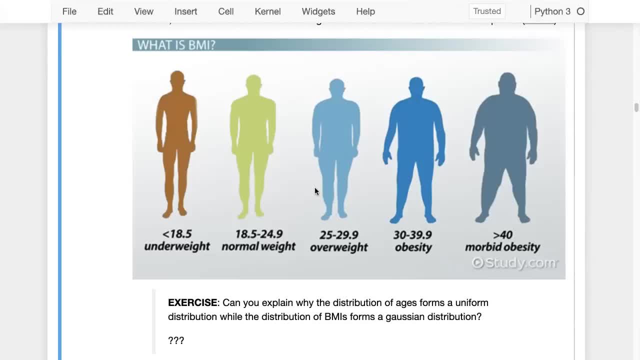 Now, this is an important factor from the health perspective. Typically, people are expected to be in the normal to overweight range. If they're underweight, then they are more susceptible to certain diseases, And if they are obese, or even morbidly obese, then they are more susceptible to certain illnesses as well. 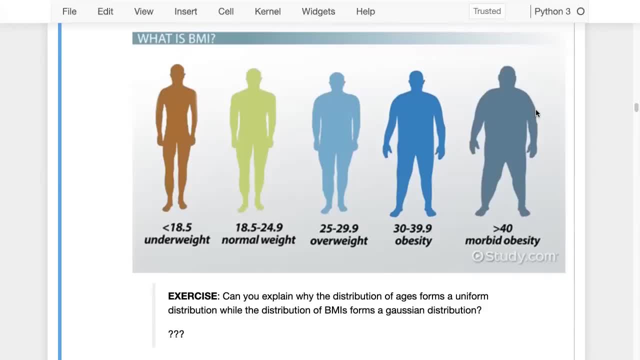 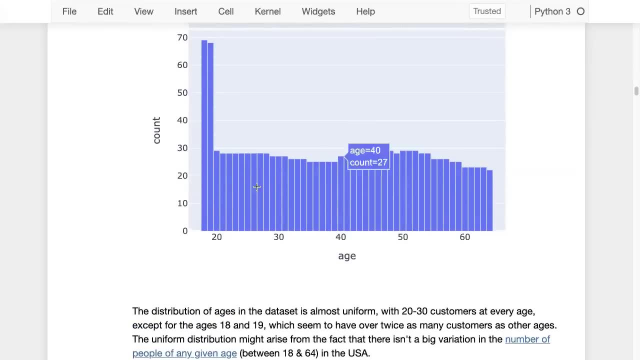 And this is why this is one important piece of information that is requested in your, In short, This form. So, as we perform this analysis, as you see, with age, you can see with age that there may be a certain relationship between age and the medical charges, and you can try and guess what that relationship might be. 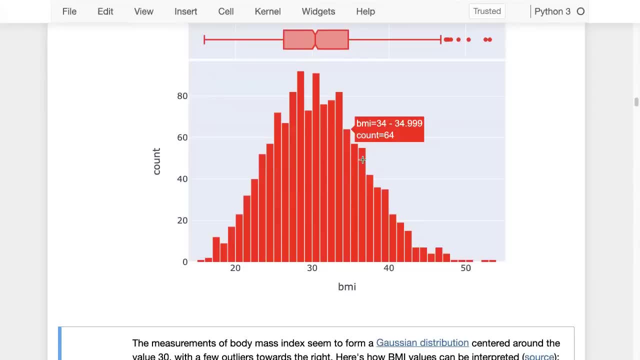 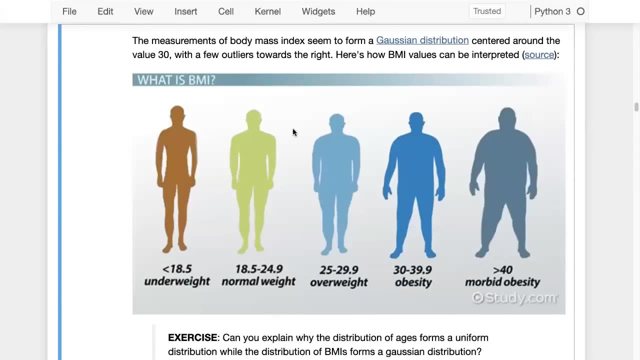 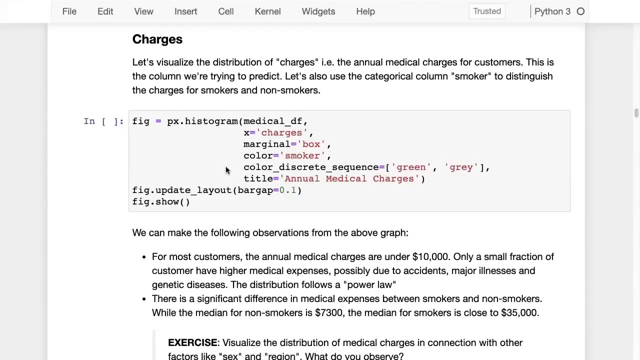 And then there may be a certain relationship between BMI and medical charges as well. with BMI, I'm guessing somewhere in between might be lower medical charges. If you're to either extreme, maybe you will have a higher medical charges. Okay, Now let's look at the most important column, the distribution of charges. 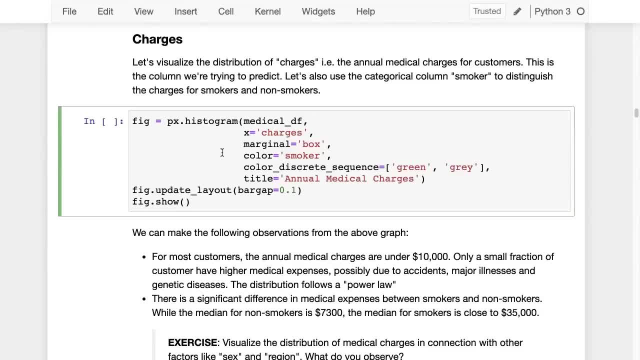 And before I look at the distribution, do you want to take a guess on what the distribution of charges is going to look like? Just think about it. We've already seen the description, We've already seen the statistics for it. So here we are creating a histogram, once again P X dot histogram, and we have a medical data frame, the DA, the data frame on the X axis. 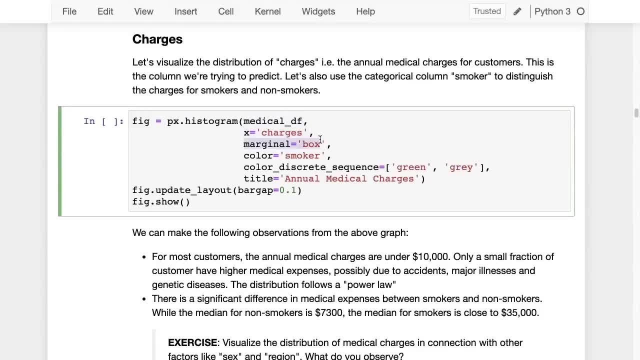 We want to show charges, Okay, Okay, And we also want to show a box plot above the histogram, and then we want to set the title to annual medical charges. but we have another important section here. This is called smoker. So what we're doing is we want to split the histogram of charges for smoker versus not non-smoker. 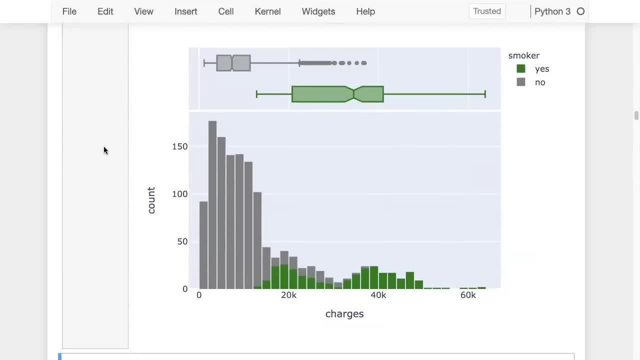 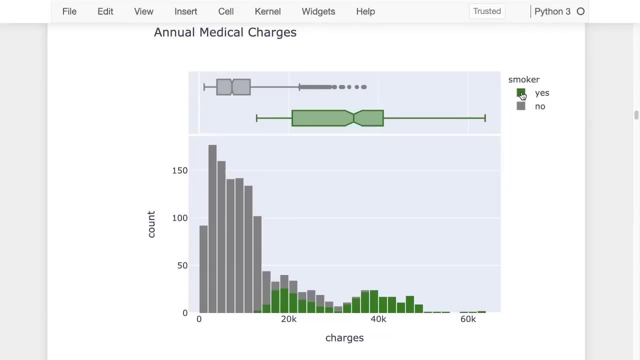 So we have a column smoker and we are going to use that to split the data, And here's what that gives us. Green represents people who have responded yes to smoker and no gray represents people who have not responded Yes to smoker. 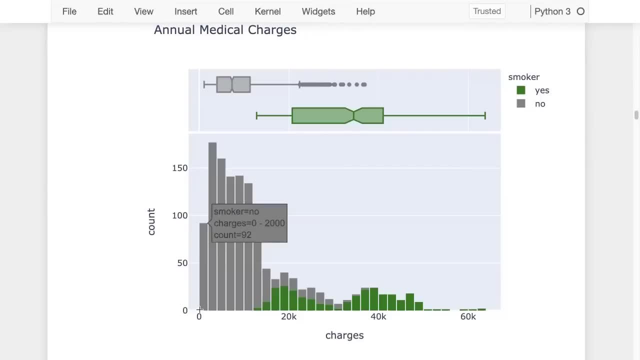 So you can see here that People who are not smokers seem to have lower medical and lower annual medical charges. In fact, most people in general overall seem to fall in the maybe like 5,000.. What is this? A 2002.. $15,000 expense category. So most people are spending between 2000 to $15,000, not more than that, which is not a very high expense. And then there are some people who need to spend a lot every year, And there is a stark difference between people who smoke and people who do not. It seems like 50%. the median for non-smokers is 7,300 and the medium for smokers seems to be 34,000.. Now It's not entirely clear If this is because they are smokers, if it is just generally true that you will have a higher medical if you smoke regularly, or is it that more people who smoke are taking life insurance and maybe fewer people who smoke or do not smoke are taking life insurance? 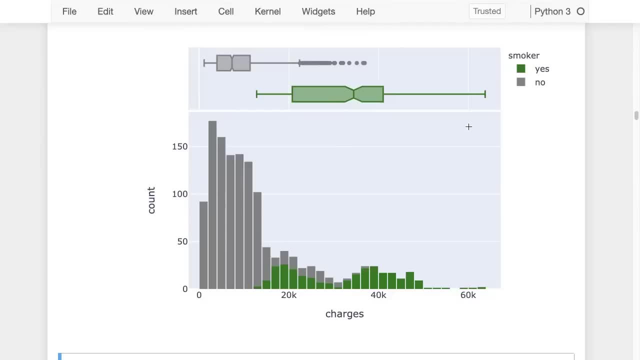 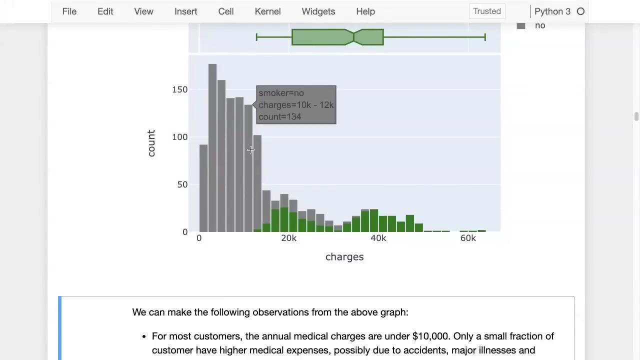 So we don't know what this means. All we know is that people have responded Yes To smoker seem to have a higher median medical expense. Okay, But in general you can see that this follows the exponential distribution, Or a, more appropriately, this is called the power law. 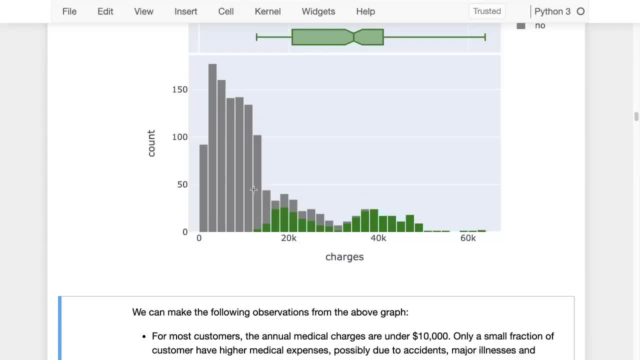 So in the power law what happens is you have a lot of people along the smaller numbers, You have a lot of people which who have a very low expense, and then you can see this exponential decrease in the medical charges. And if you were to separate out smokers and non-smokers and plot them separately, so you would see that for non-smokers you have this exponential decay and maybe for smokers you have that as well. but it seems like there are two. 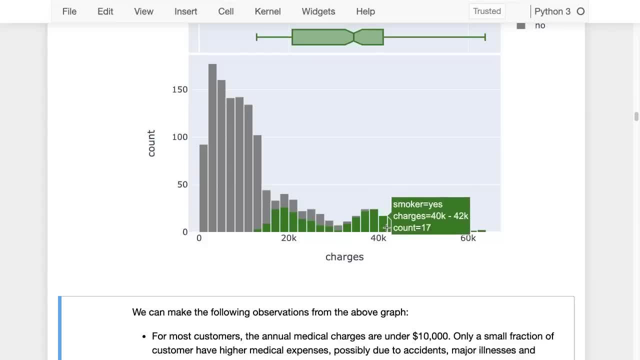 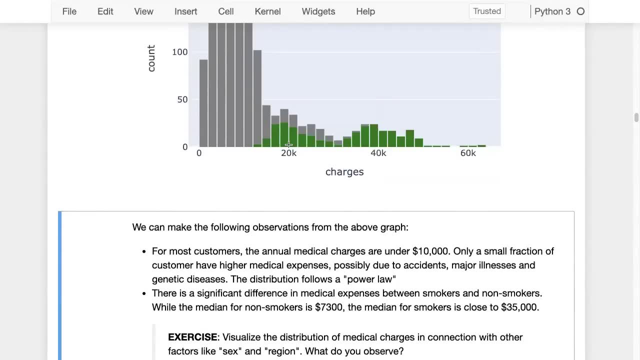 Sections. Maybe this is just general smokers and this is maybe smokers with some ailments, right? So there is something to discover here Why we're seeing this kind of a pattern. Maybe do we need another category of like light smokers and heavy smokers. 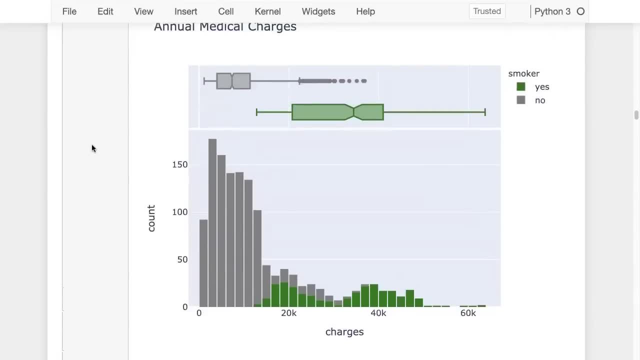 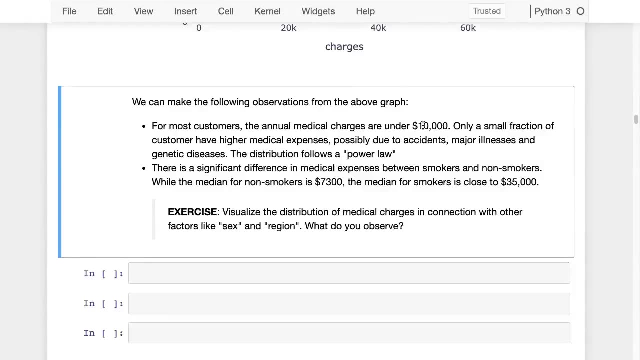 We might need to look into this, but at the very least we're already starting to observe some trends that the charges have, that for most customers, the annual medical charges are under 10,000, $14,000, and only a small fraction of customers have higher medical expenses. 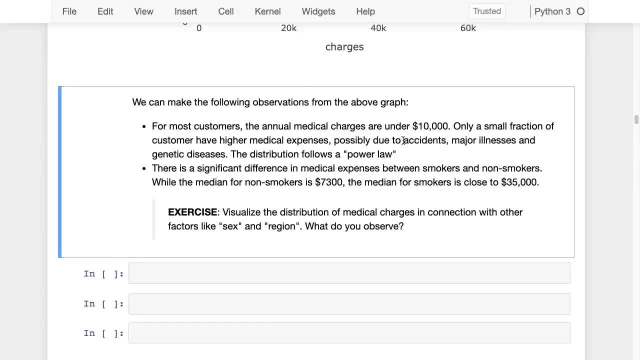 Okay, Possibly due to accidents, major illnesses or genetic diseases. And this is what happens. Most of the population is healthy. Most of the population probably does not need to go to a hospital every year, maybe except for a few checkups- regular checkups- but some people unfortunately either have accidents or major illnesses or genetic diseases. right, 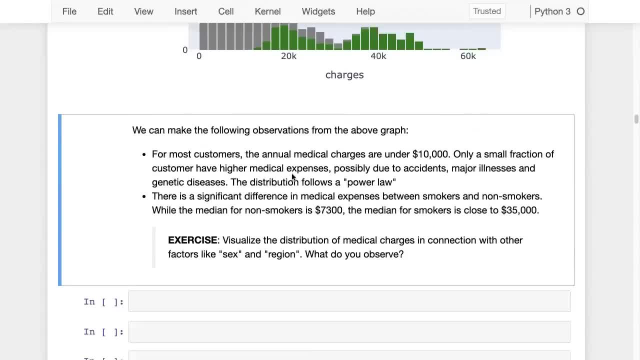 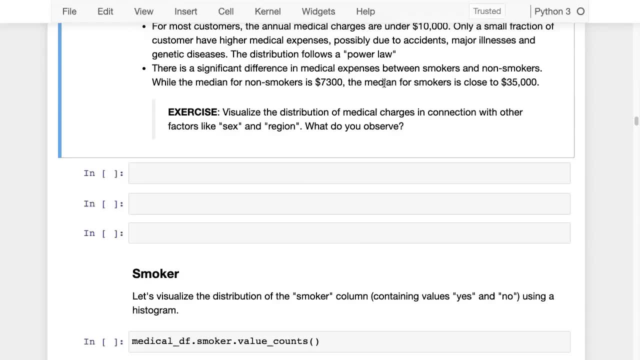 So that's why they may incur a higher medical expense. And the second is that there is a significant difference In medical expenses between smokers and non-smokers. while the median for smoke non-smokers is 7,300.. The median for smokers is close to 35,000.. 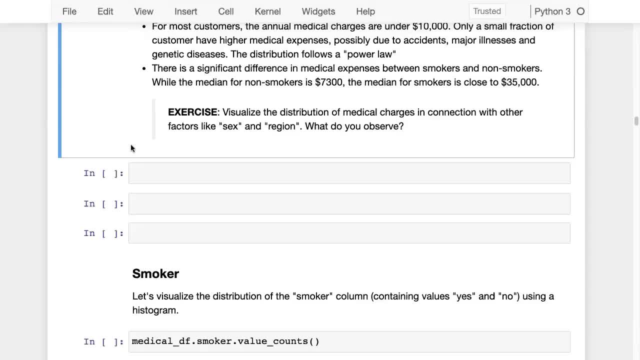 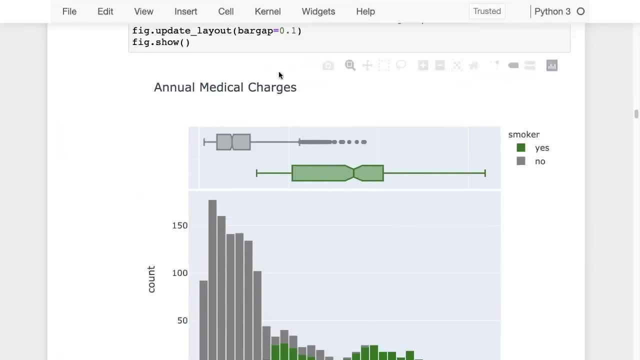 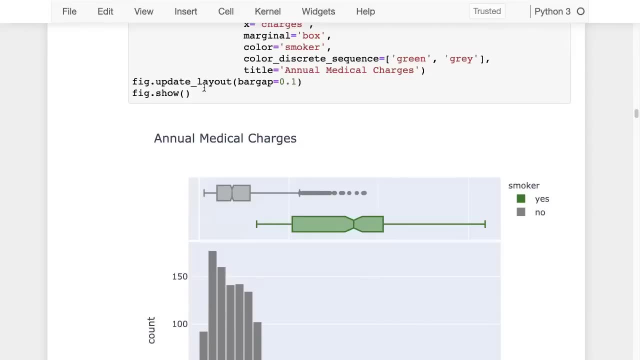 Okay, So next up here's an exercise for you: visualize the distribution of medical charges in connection with some other factors like sex and region. So maybe replace this by sex and replace this by region and see if you see it See Similar disparity across males and females or across different regions. 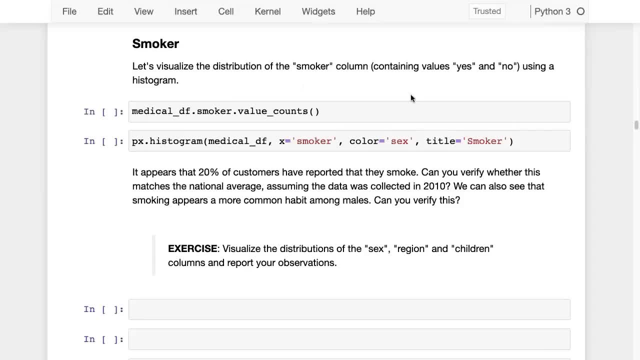 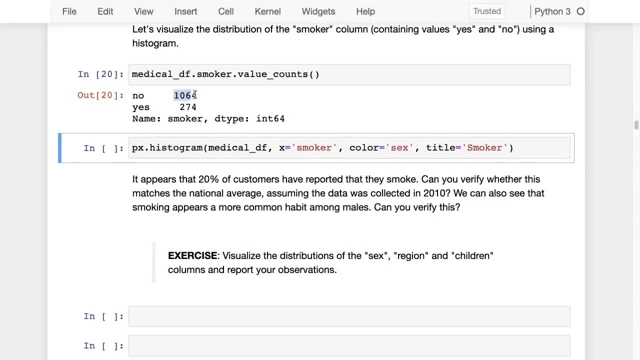 Okay, So while we're talking about the smoker column, let's try and visualize the distribution there. So let's just see how many examples we have for each. So it seems like out of the 1300 or so people we have, thousand or so have responded no for smoker and around 274 have responded. 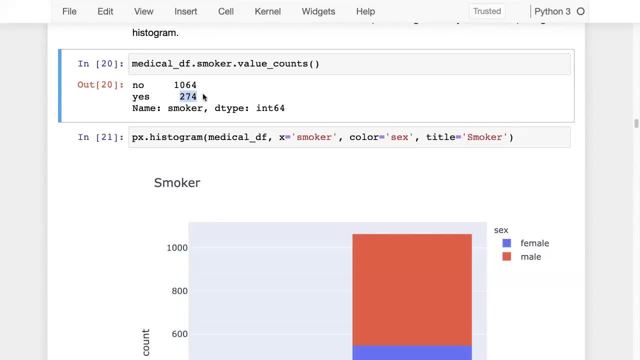 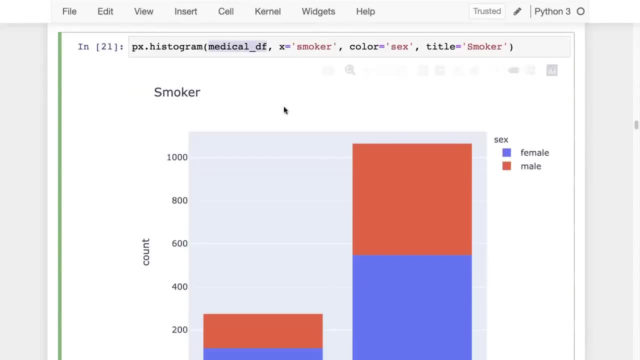 Yes, So about 20% of the customers are smokers and we can visualize this using a histogram as well. So we say PX dot histogram, we pass in the data frame for X on the X column, We have smoker, and let's break down the visualization by sex, this time. 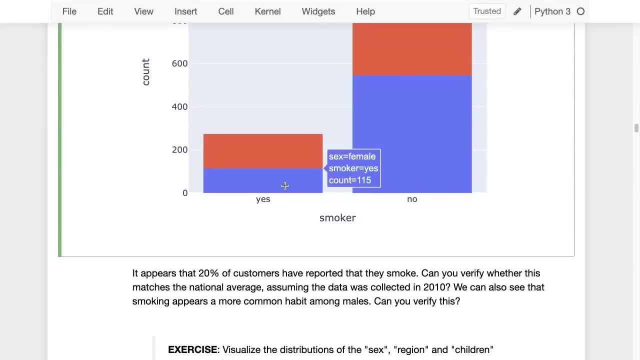 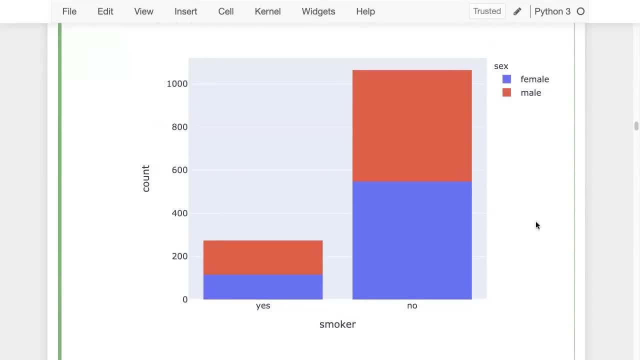 So here you can see that yes represents people who've responded Yes To smoker, And that number seems to be in total about two, 68 or so- and no represents people have responded No. but this is also broken down by sex. 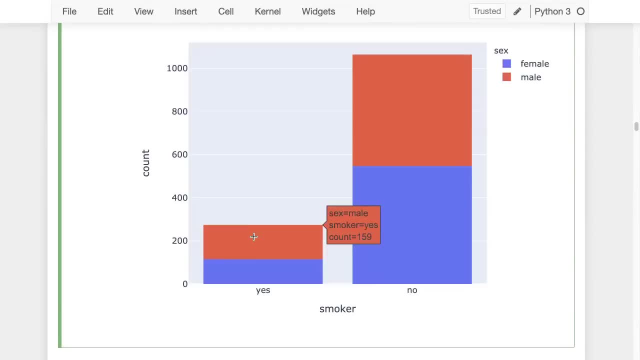 So you can see that about Yeah, 115 females said yes And one 59 meals. on the other hand, 517 meals said no And five 47 females. So it seems that smoking is more common among meals, and this is something that you should try and verify. 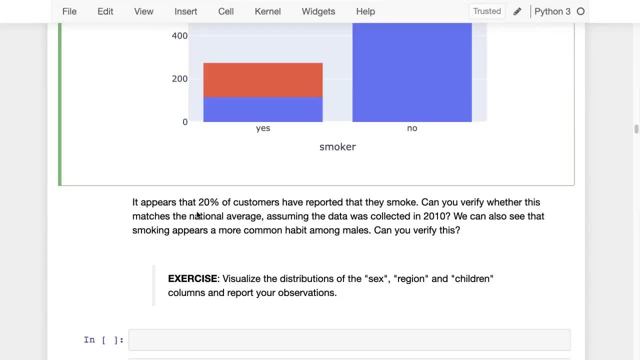 This is something that you should try and verify, And similarly, it also seems like 20% of the customers have reported that they smoke, So this is also again something that you should try and verify, See if this matches with the national average and you can assume that the data was collected in 2010.. 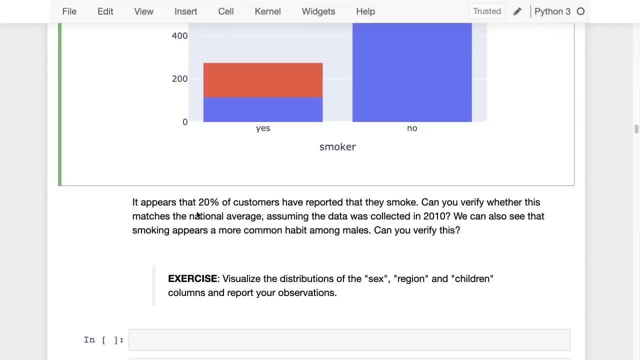 This dataset has been around for about 10 years Now. the reason you should verify these things as you're performing this analysis, And the reason you should perform this analysis in the first place, is to understand if the distribution of the data that you have matches the distribution of the population itself. right, 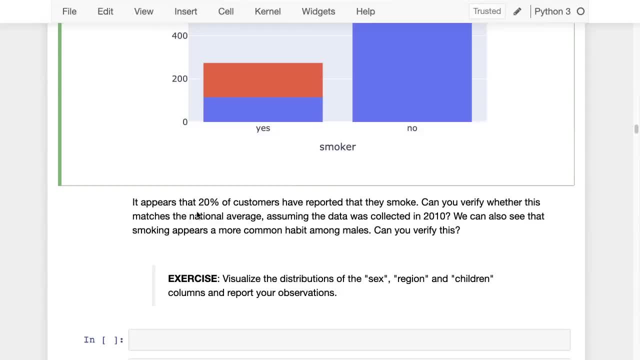 If your data contains 90% smokers But in the general, In the general population, there are only about 10% smokers, Then any analysis that you do or any model that you build will be wrong, because it will be built under the assumption that 90% of the inputs that are coming to the model are going to have, yes, in smokers. 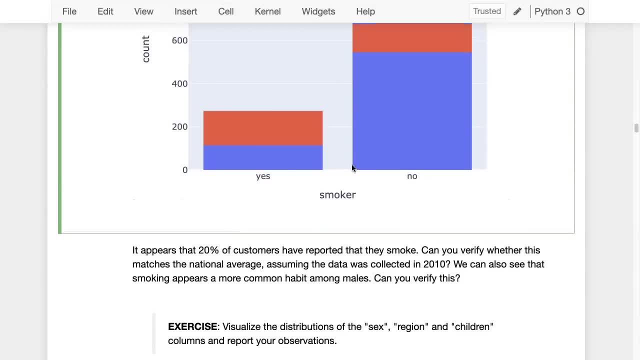 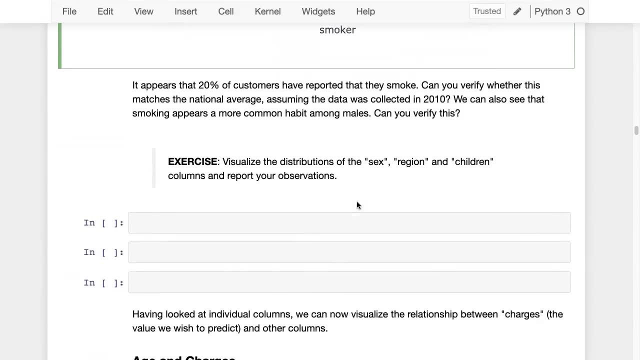 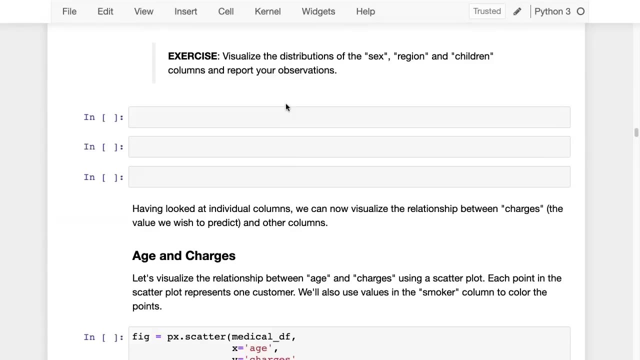 So that's why, wherever you're building a model, make sure that the distributions of each column match the distributions of the populations where the model will be applied. Okay, So with that, we've looked at the individual columns. You can also try and visualize the distribution of sex, region and children and report your observations. 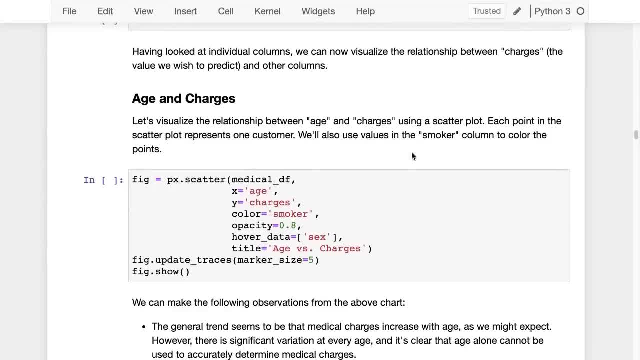 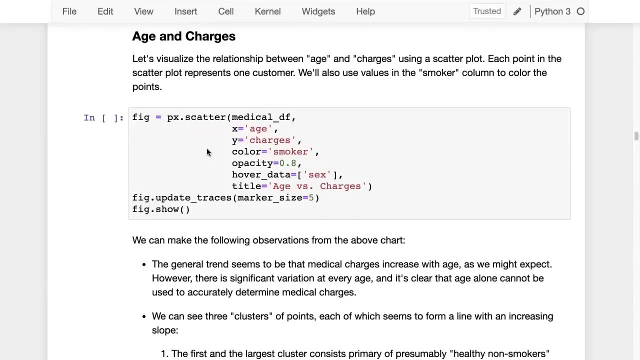 Okay, So now, having looked at some individual columns, we can now visualize the relationship between charges, which is the value that we wish to predict, and the other columns. I would guess that age would be one of the- Okay, Most important factors in determining your medical expenses. 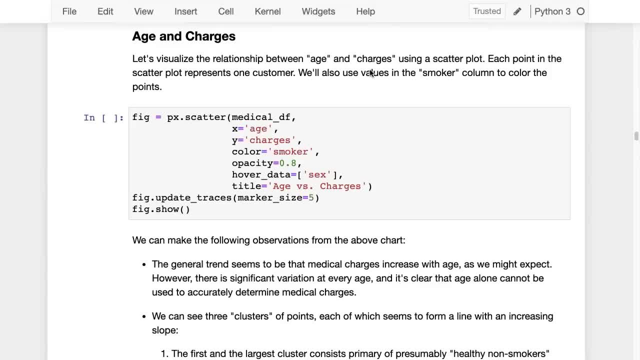 So let's visualize the relationship between age and charges using a scatter plot. So we use PX dot scatter, We pass in the data frame medical DF. We pass in the data frame medical DF and on the X axis we want to show the age. on the Y axis, 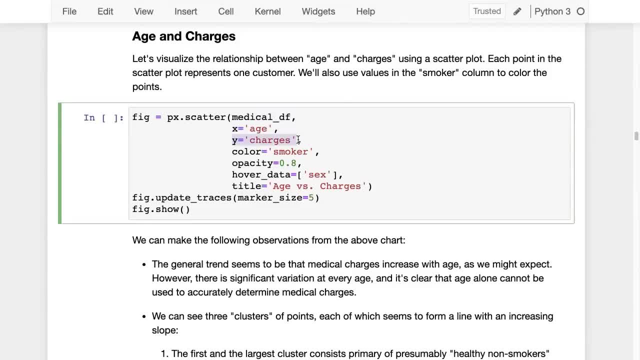 We want to show the charges And we will show Oh single point on the chart for each customer. Now, whenever you have a Scott scatterplot, you should also use the opportunity to maybe add some color. So maybe let's color the points based on whether the person is smoker or not. 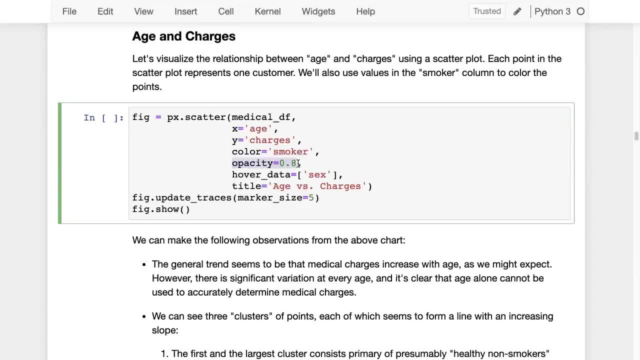 And let us just set the opacity of points to 0.8, because we have over a thousand customers, So we may have some overlapping points. So, just so that we're able to better see the data, let's just reduce the opacity A little bit of the points. and, Miley, we're just setting a title as well. 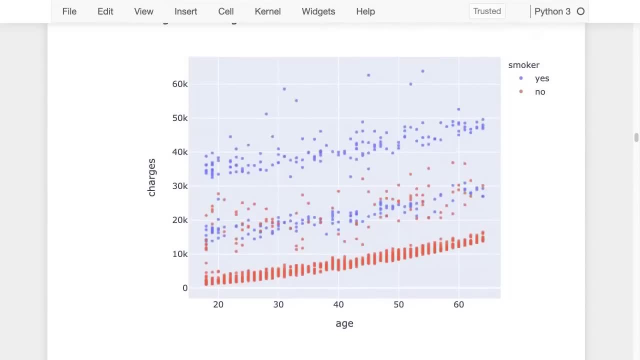 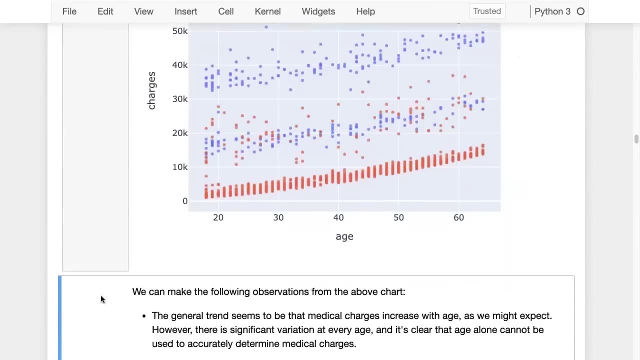 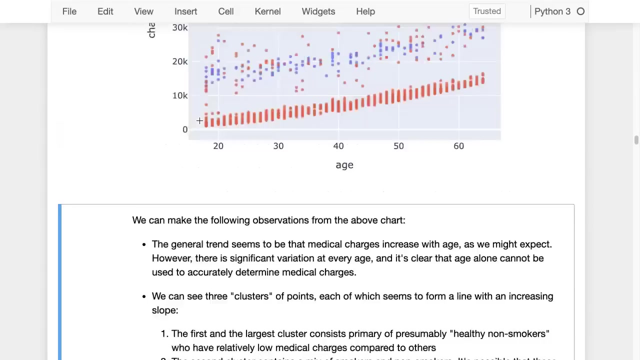 Okay, So now we have this chart and this looks very interesting. I can see three clear clusters here. Here's what I can see. I can see three clear clusters of points, and each of which seems to form a line with an increasing slope. 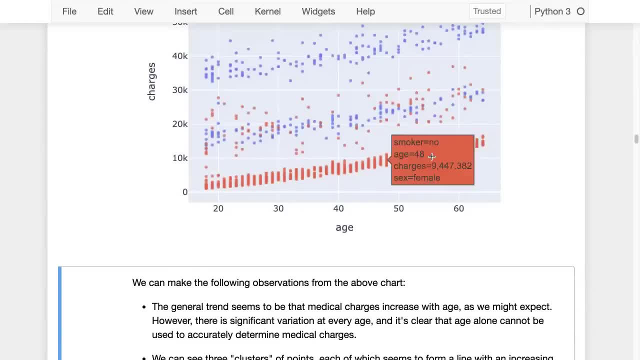 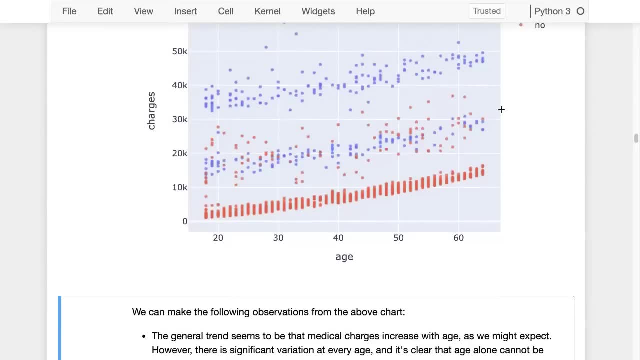 You can see that this seems to roughly lie. Okay, In a line. of course it goes up and down, but roughly. you can see a linear trend here. And then you have the second cluster, which also seems to have a somewhat linear trend as increasing with age. 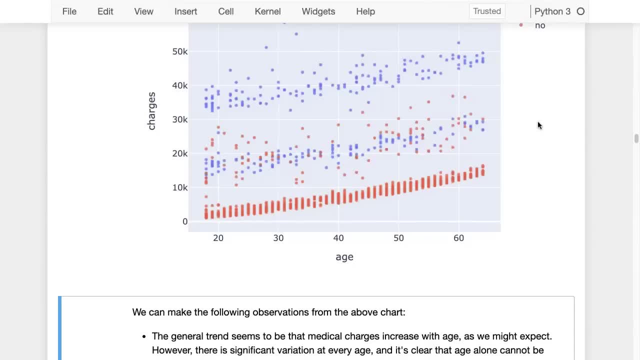 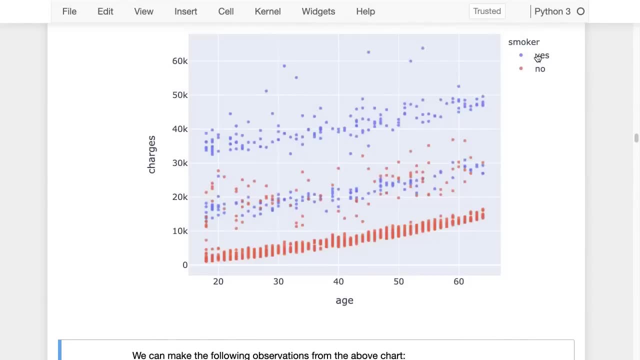 But if you look carefully, you have a mix of smokers and non-smokers in this cluster. It's possible that this is actually two different clusters which just happened to fall in a similar place. For example, if I turn off smoker, this is what we get. 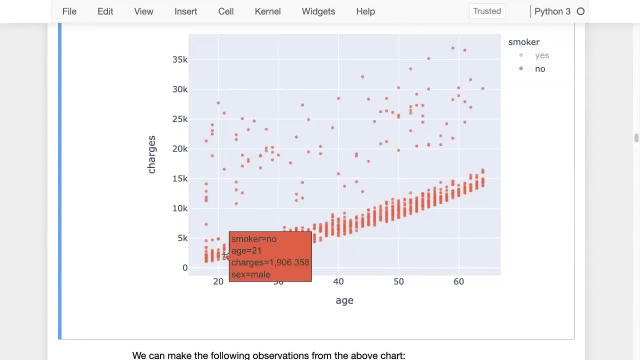 So it seems like among non-smokers, most people incur a fairly low medical expense that goes from zero to 5,000 at age 18 and goes up to 13 to 15,000 at age 64. But then there are some- as we said, there are maybe five- 10% of people who unfortunately, due to accidents, genetic ailments or major illnesses, have to spend a lot more. 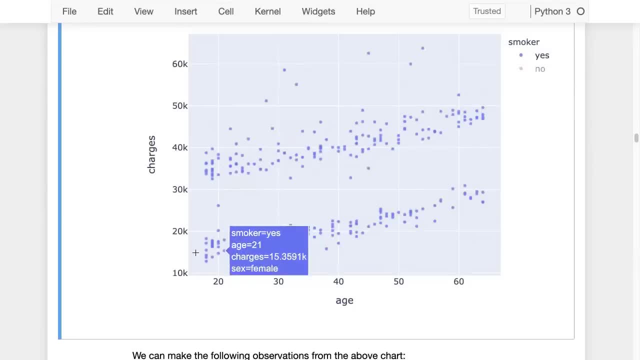 And then there's probably A similar trend here for smokers. You can see, here this is seems to be the baseline. So probably if you're just smoking, you don't have any other ailments. This is where you are, And then here you have another group of people. 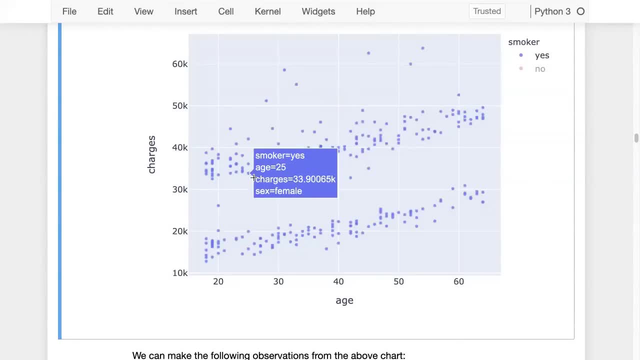 So it's possible that these are people who are smokers and have ailments or, as there was one suggestion, maybe it is a combination of being a smoker and also being obese. So it's possible that is, that could be the reason for this. 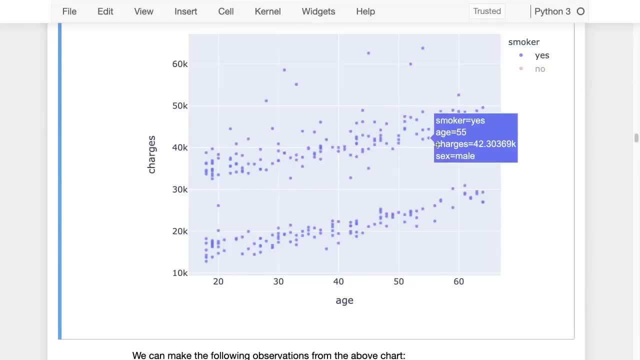 So it's worth investigating. but you can see here there are two Clear sections. Maybe you need a smoker and a heavy smoker section. Maybe that makes a big difference. Maybe a, two cigarettes a day doesn't make a difference, but 20 does. 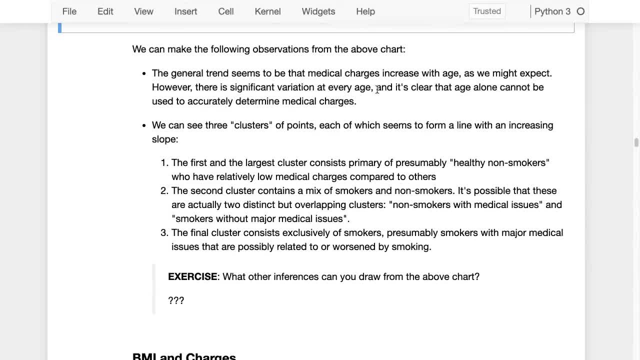 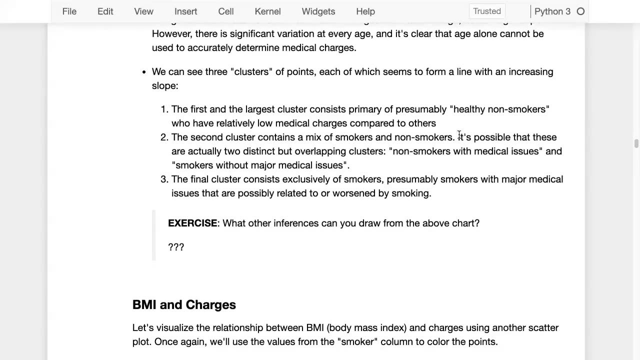 So all of these interesting tents here, and that's what we've summarized here, And this is a general thing that you should do in your exploratory analysis: Whenever you observe a trend, summarize it and try to offer some explanation, And you can mention clearly that there are certain hypotheses, like we're using the terms, like it's possible, which means that this is something to be. 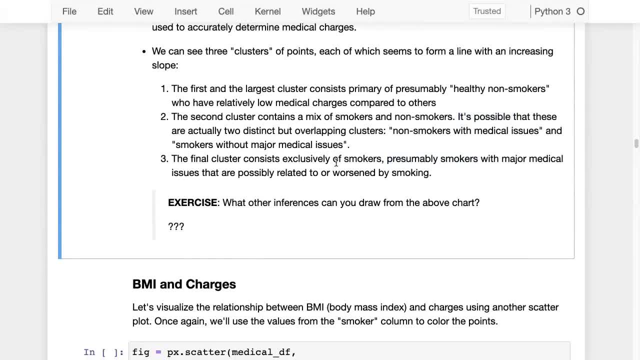 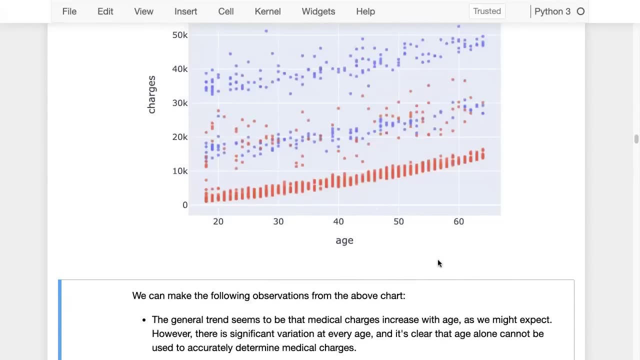 Verified and then presumably, which means that, okay, you have one cluster for smokers and one clusters for smokers with medical issues, or it could be smokers who are also obese. So we don't know. We'll have to study this, We'll have to dig deeper and try and figure it out. 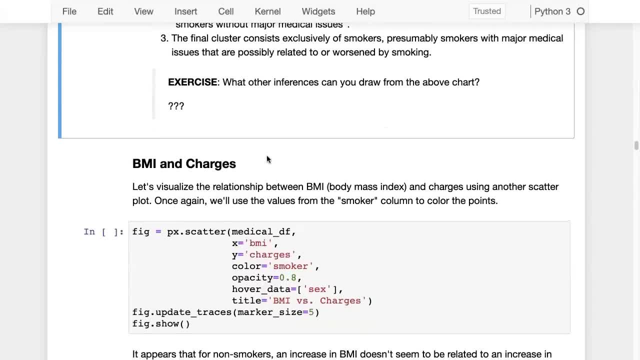 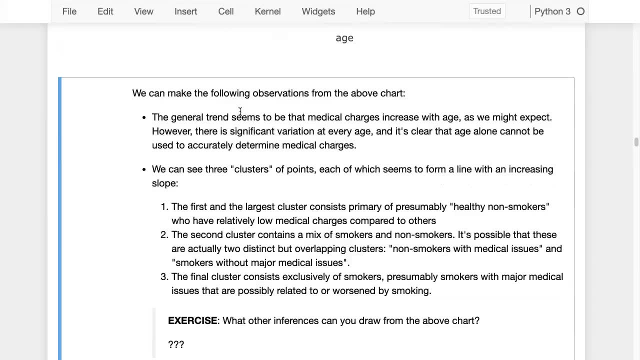 So I'll leave that as an exercise for you. And there are definitely more inferences that you can draw from the above chart, So I'll let you draw that as well. For example, what percentage of people lie outside the? No So this: how many people lie in this region and how many people lie outside? 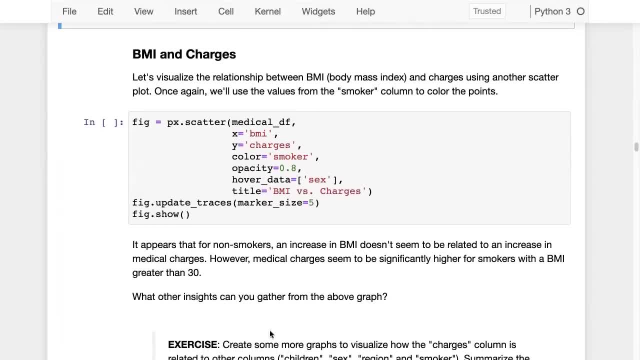 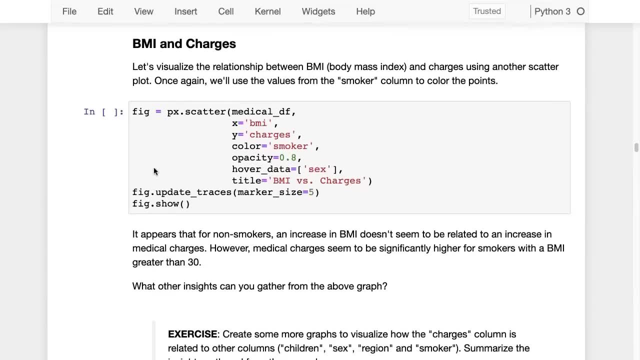 What are the number of outliers? Okay, Let's look at BMI. This seems to- this seems again to be an important factor. So let's visualize the relationship between body mass index and charges using another scatter plot. Once again, we will use PX dot scatter on the X axis. 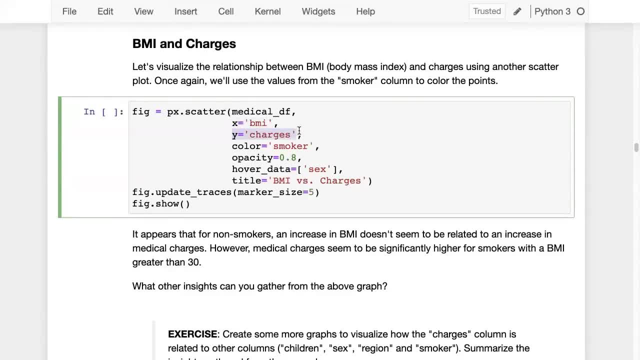 This time we will use BMI. on the Y axis, We will use charges and we will color the points once again using the smoker column and we will set the opacity to 0.8 and we will set on hover. We'll also show the sex so that when you hover over a point you have some more information and we set a title for the chart. 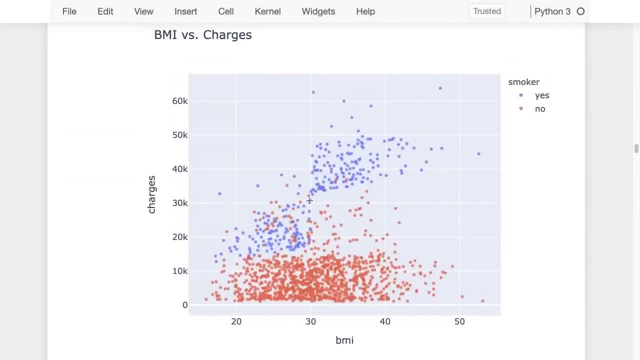 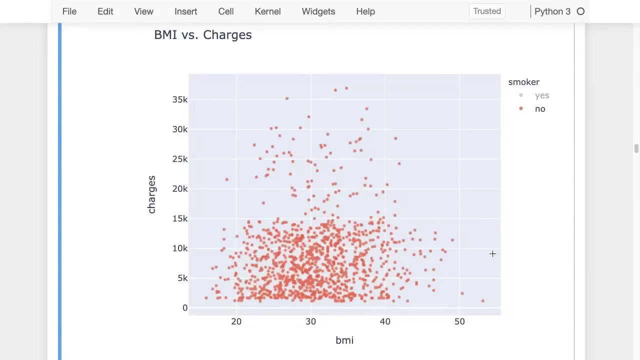 So here's what the chart looks like, And now you can see that the picture is starting to get a little clearer. So if you see here, if I turn Yes, you can see that there seems to be no real relationship between BMI and medical charges. 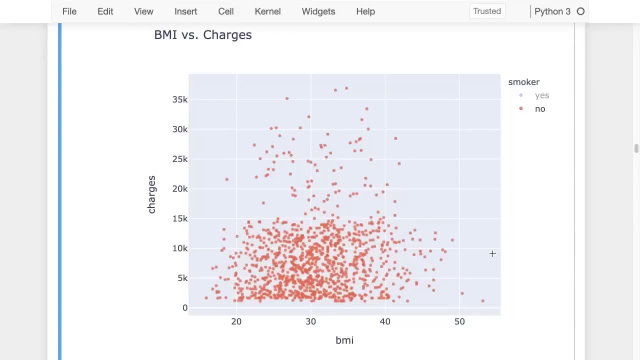 Maybe BMI is a flawed metric, Maybe it doesn't really make sense. You can see here that you have numbers all over the place And, if anything, you have some outliers here somewhere in between in the 20 to 40 range, not beyond 50 or not below 20, but that could also be because there are very few people below 20 or beyond 40.. But once you add in this, Or if you just look at the smokers, you can start to see a trend here. So it seems like there are two major clusters: below the BMI of 30, your medical charges stay low in about the 30 K range. below the 30 K range and above 30, then they seem to increase. smoking combined with obesity. 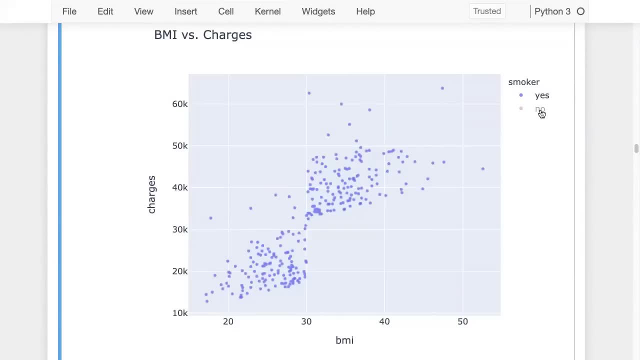 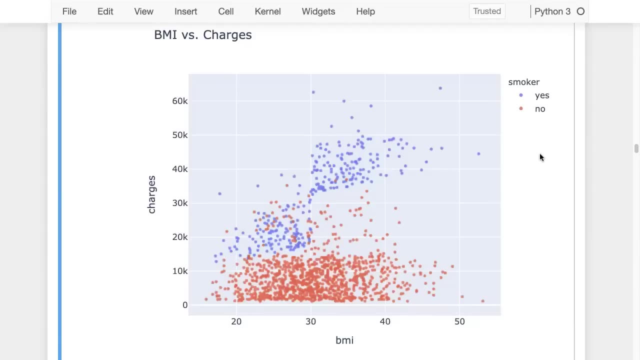 It may appear. It might seem that this might be a bad condition to be in. So this requires more investigation, but we're already starting to Uncover more information. at this point, If you have doubts, you should probably reach out to somebody in the company, somebody who actually has some expertise in the field, and ask them if this is indeed the case. 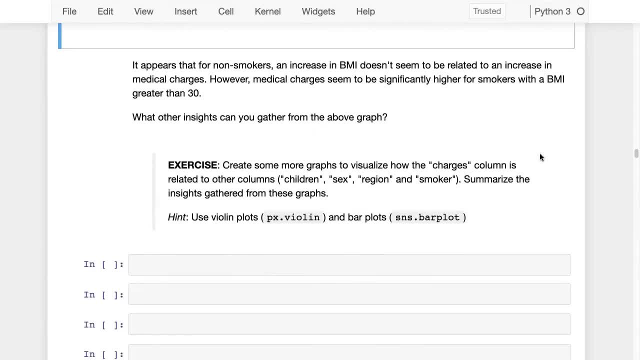 And all of these things are going to be important because the model that you build- you will have to explain why it gives the predictions that it does a lot of times, because there are regulatory requirements. There are regulatory requirements in healthcare, There are regulatory requirements in finance and a bunch of other domains as well. 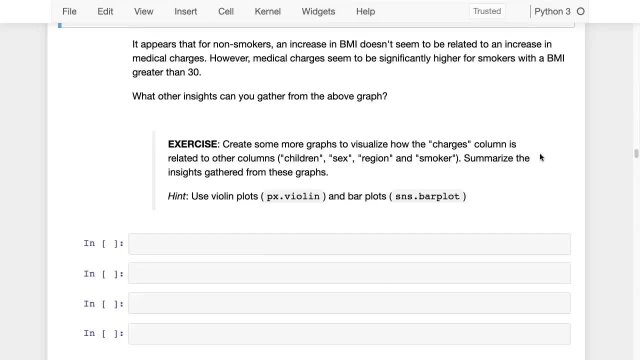 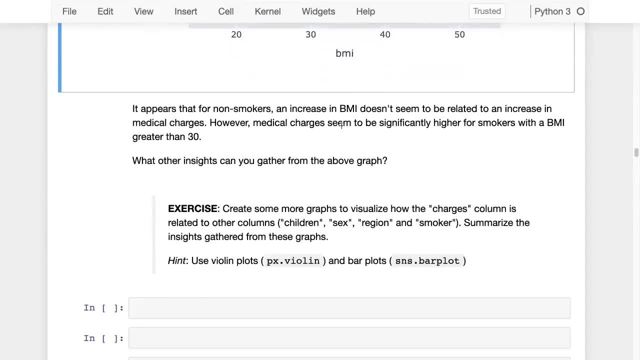 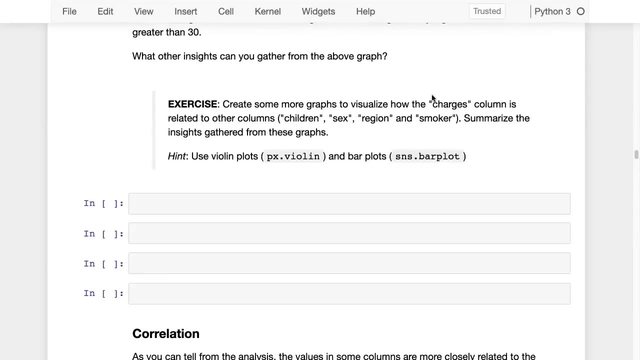 So that's why understanding these relationships is important. What other insights can you gather? Just try and see if you can gather some other insights from this graph and try and create some more graphs to visualize how the charges column is related to other columns, For example, charges against children. 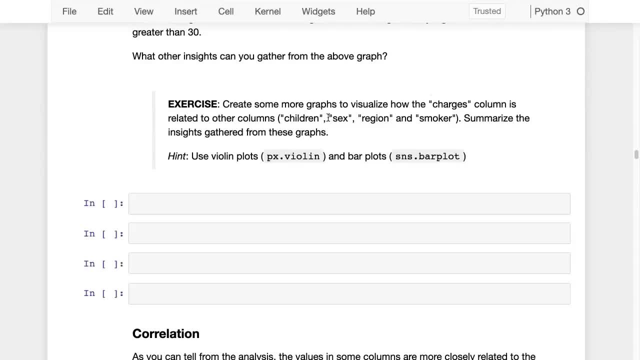 Do you see that there is a general increase in charges when you have more children or charges with sex? Do you see that there is a difference between males and females? Maybe compare with region and maybe directly compare with smoker. Maybe just look at the. 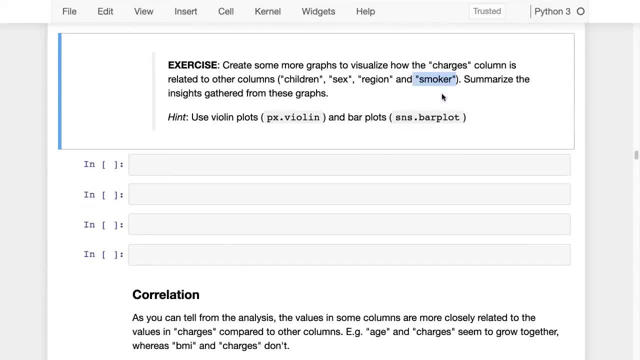 Average charges for smokers and the average charges for non-smokers. Here's a hint for you: You might want to use the violin plot for some of these. For example, if you do PX, dot, scatter, medical, DF, and on the X axis you put children and on the Y axis you put charges, 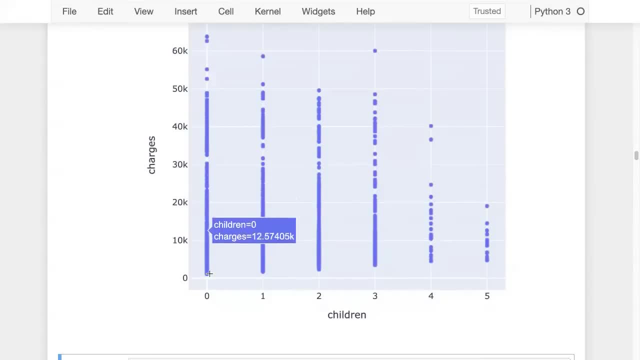 There's a problem here. You can't really tell much because The value of children Is not continuous. It goes from zero to one, to three, to four to five. So we don't know if there are five points here or 50 points or 500.. 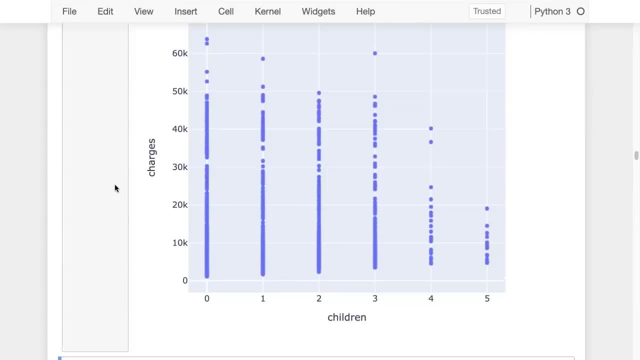 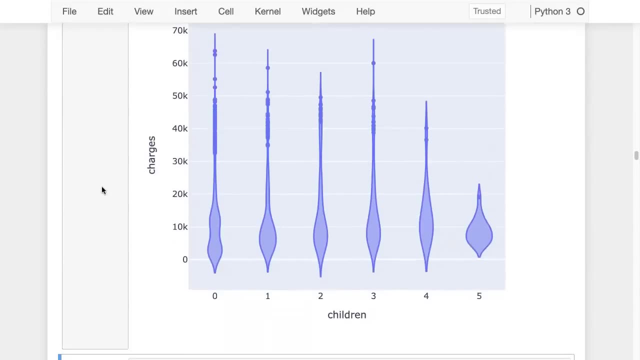 It's very hard to tell because they're all on top of each other. So if you just change scatter to violin- and if you've ever wondered why a violin chart is useful, Now you'll see- just change it to violin, Now you can see that you also have this. 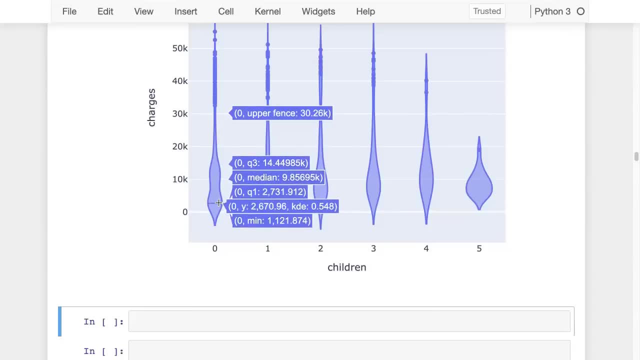 Wait for this chart. The width tells you how many values lie here relatively. So it seems Like you have a bunch of values here, a bunch of values here, and then you have all these outliers And now you can observe a general thing. 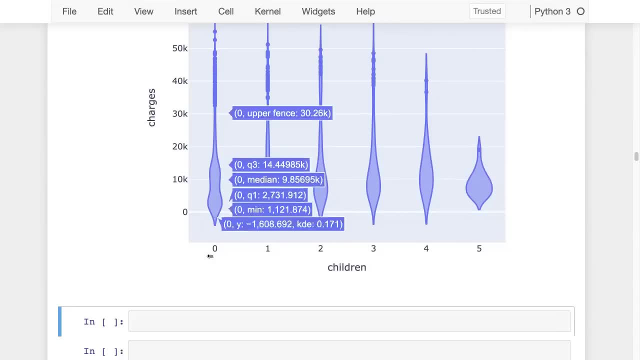 You can see that the bulk of values shift up as we go, with the number of children increasing. as the number of children increases, the potential medical costs seem to slightly increase, Not by a lot, because there are many people who have a very low medical cost. 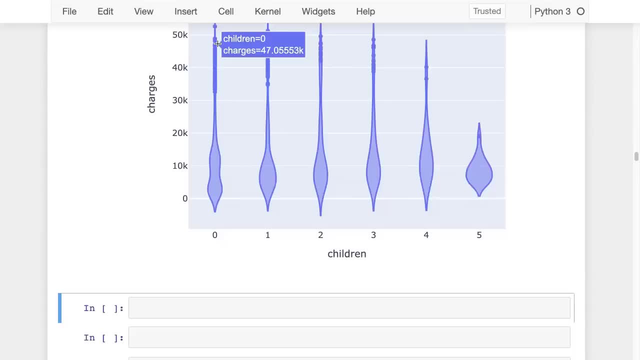 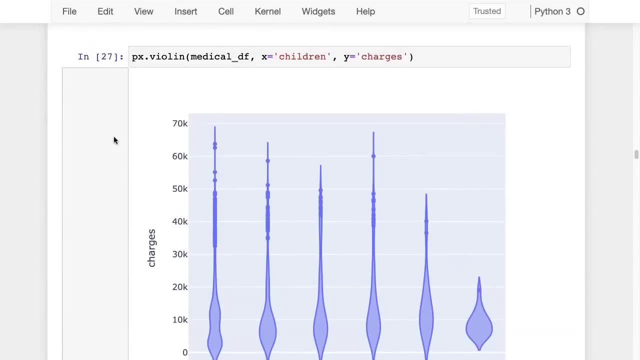 Despite having four children. there are many people who have a very high medical costs without despite having high children, despite having zero children. Okay, But there is some sort of a trend here, a very weak trend, but a trend nevertheless, Okay. 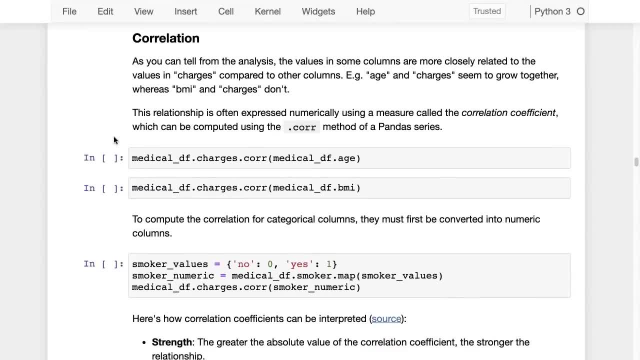 So, as you can tell from the analysis, the values in some columns are more closely related to the values in charges compared to other columns. For example, age and charges seem to grow together and BMI and charges don't. So the relationship between two columns on whether they grow together or not. 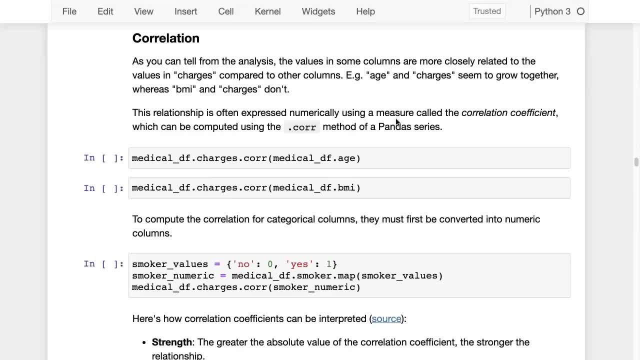 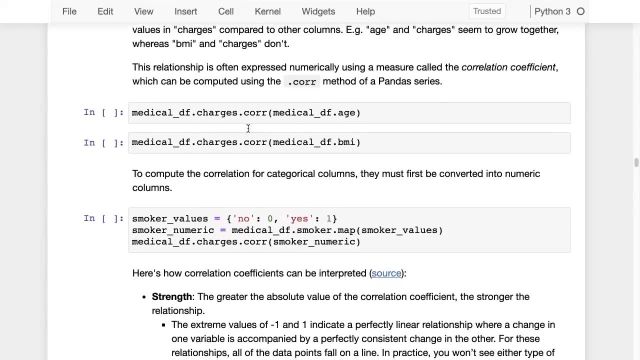 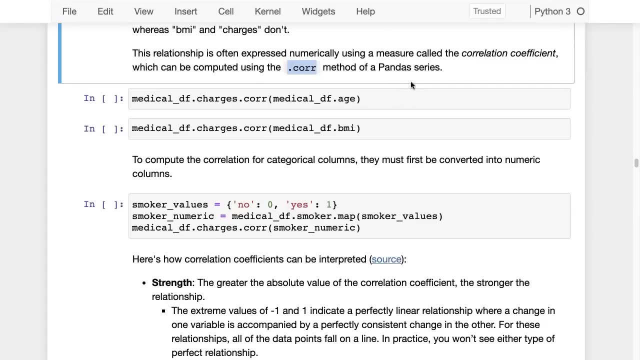 Okay, It's often expressed numerically using a measure called the correlation coefficient, and there's a certain formula for it And there's a certain meaning it has. but first let's just see how to compute the correlation coefficient. The correlation coefficient can be computed using the dot C O R R or dot core method of a Panda series. 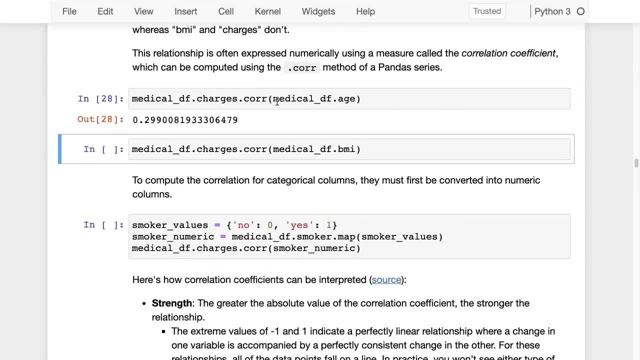 So if we say medical DF, dot charges, dot core, medical DF dot age, So we want to compute the correlation between charges and age and it seems like the correlation is 0.29.. Okay, And we'll see what that means in just a second. 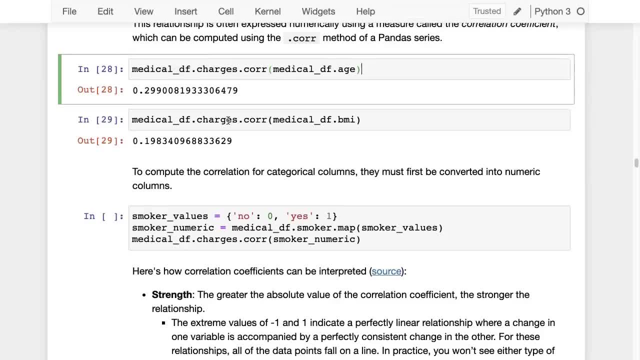 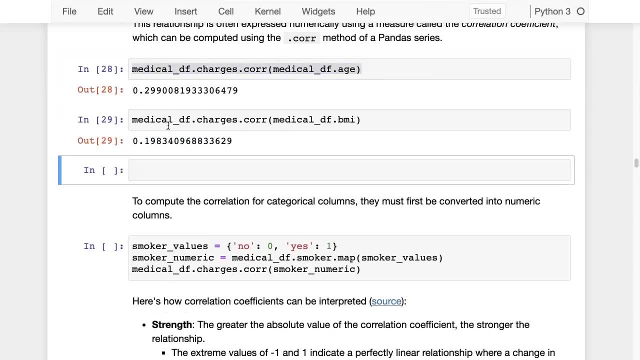 And then if you want to compute the correlation between the medical charges and the BMI, it seems like the correlation here is 0.19.. So there's definitely a higher correlation between age and charges than there is between BMI and charges. And maybe let's also compare children. 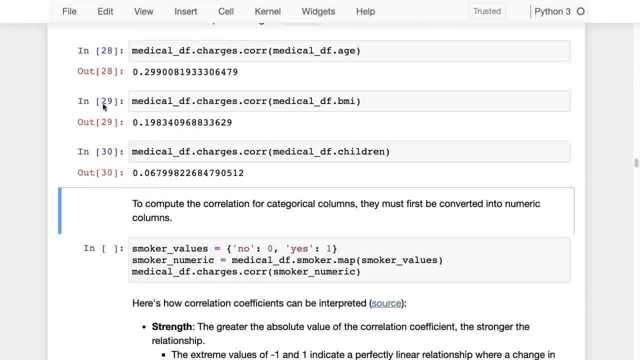 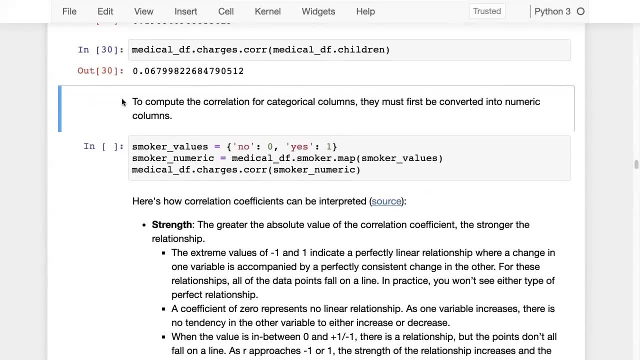 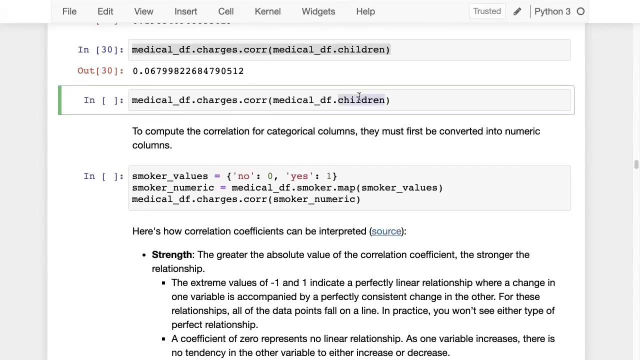 So with children there seems to be an even lower correlation than the BMI. Okay, So that's how you compute correlation between columns, And you can also compute correlation for categorical columns. It won't work directly, At least I believe it won't. medical DF dot smoker. 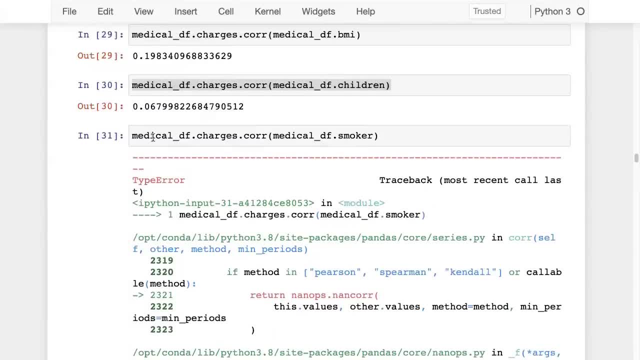 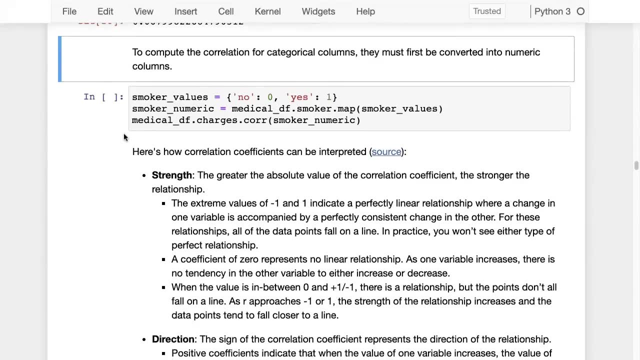 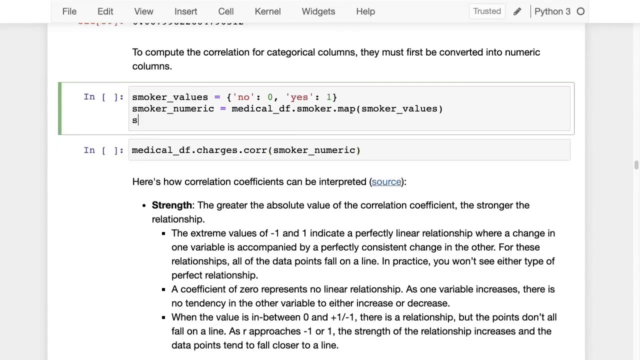 It won't work directly because you need numeric data to compute the correlation. So what do you need to first do is convert your categorical data into numeric data. So here's what I'm going to do: I am going to create a new series called smoker numeric. 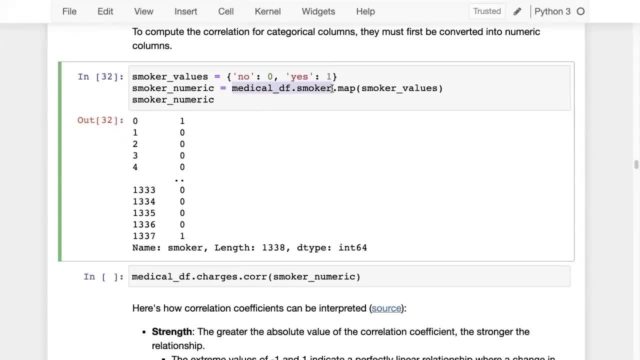 And how are we going to do that? We're going to take medical DF dot smoker and we're going to call dot map on it. So dot map takes either a function or a dictionary and it applies it to every value. So here we've supplied a dictionary- no dictionary- which converts no into zero and yes into one. 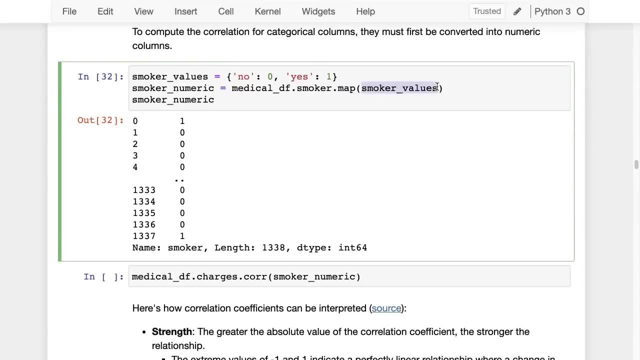 So when you call medical DF, dot, smoker, dot map, smoker values, then it, Wherever you have a no, that's going to convert to zero. wherever you have a yes, that's going to convert to one. So this is a very useful technique whenever you want to quickly convert some categories into numbers. 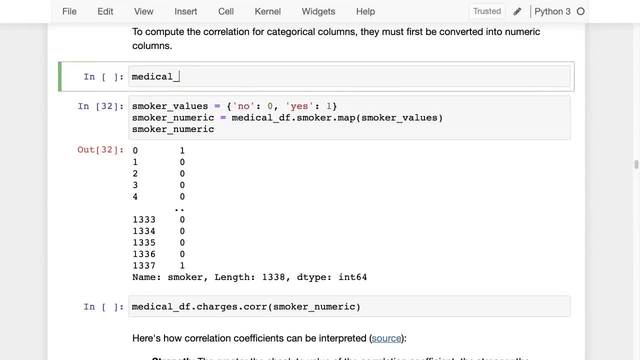 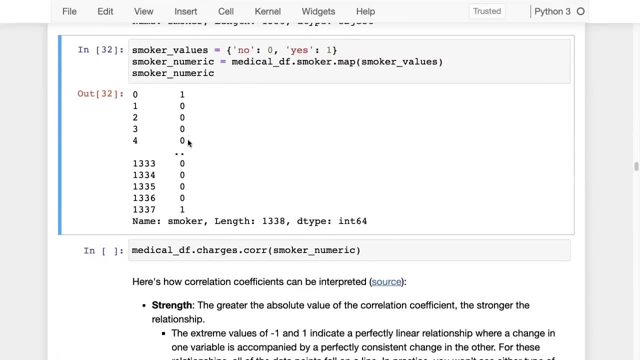 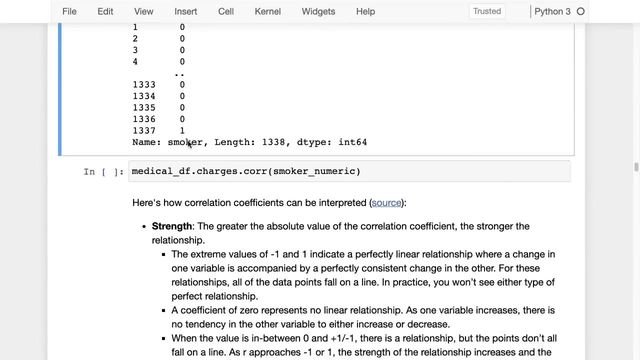 Let's, and let's compare that. Let's see medical DF, Not smoker Yep. So you have yes, no, no, no, And you have 1, 0, 0, 0.. Okay, Okay, Now, once it is converted, 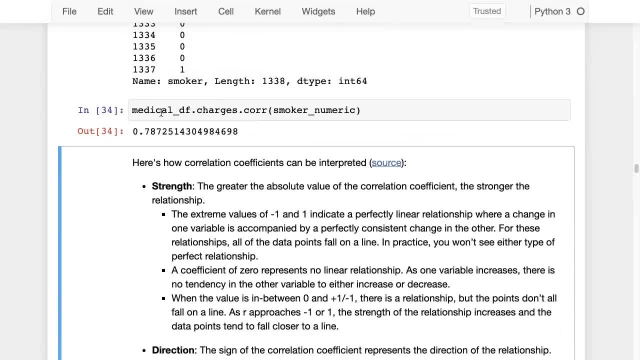 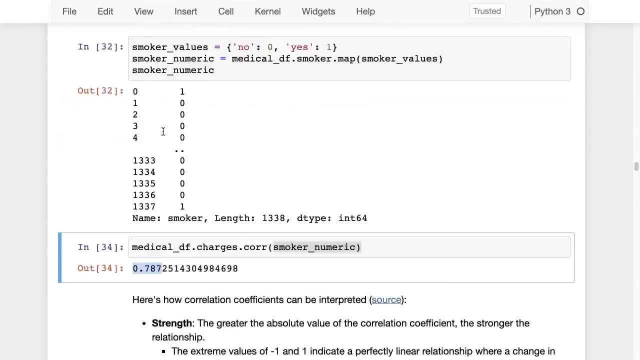 Okay, Okay, Into a number. you can then compute the correlation. So you see: medical DF, dot charges, dot correlation, smoker, numeric, and that has a coalition of 0.7, 8, 7.. So now you can start to see the trend: 0.7, 8, 7 for smoker, probably the highest correlation. 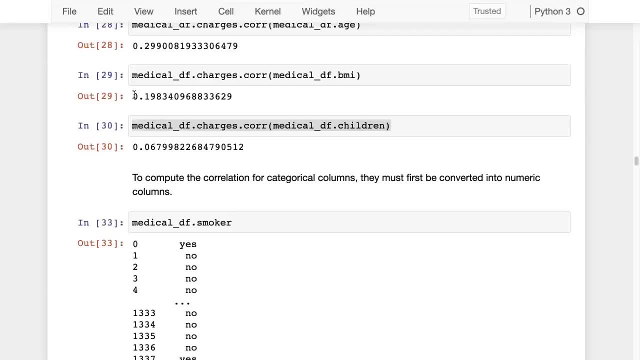 Then you have with age: 0.2, 9,, 9.. Then you have a charges: 0.1, 9,. and then you have with children: 0.0, 6,. and then there are some other categorical columns as well. 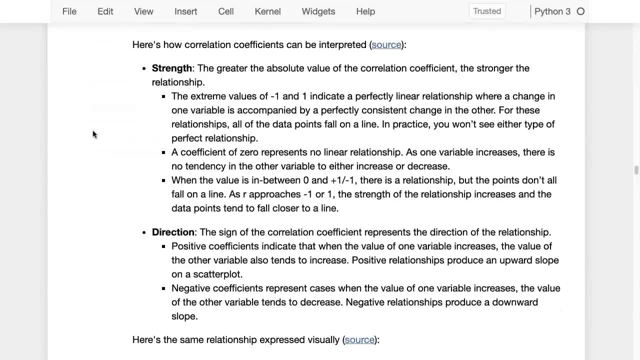 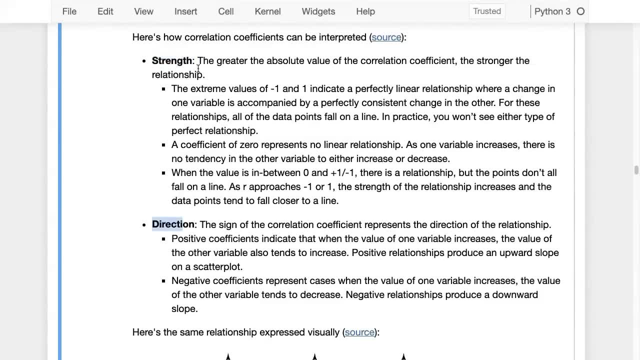 So we're not just, we're not done yet. So here's how the correlation Coefficient is interpreted. It indicates two things: It indicates strength and it indicates the direction. So the greater the absolute value of the correlation coefficient, the stronger is the relationship, which means that if you have an extreme value, like minus one or one and one is pretty much the highest value that you can get. 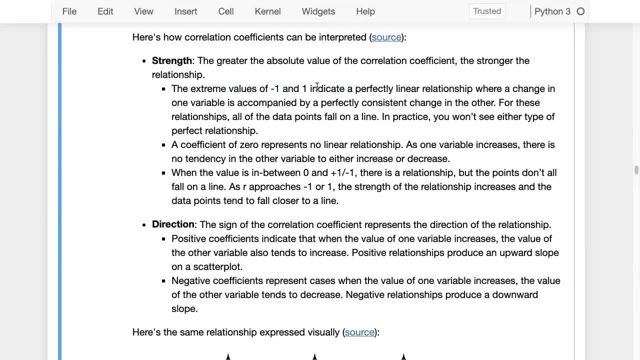 You cannot get something higher than one or lower than minus one. that indicates a perfectly linear relationship where a change in one variable is accompanied by a perfect, consistent change in the other way, Which means essentially that these points lie on a line and there's a geometric interpretation here. 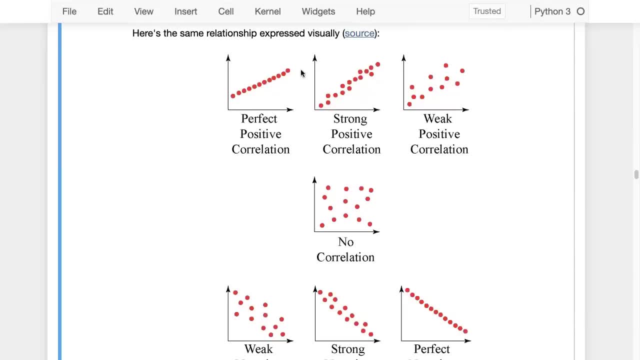 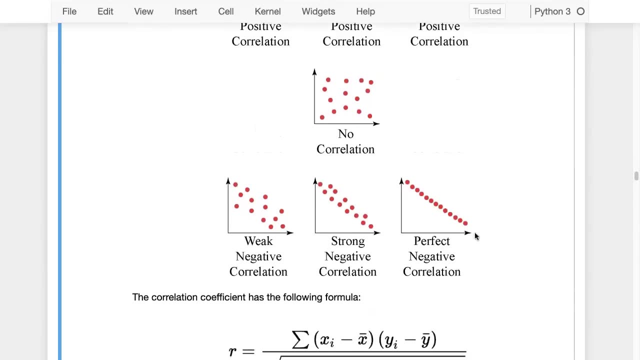 So if you have X and Y- let's say age and charges- and you saw this kind of a graph, that would mean perfect correlation, correlation of one. This would be positive correlation. And if you had a chart like this where it was a line but one increase in one led to decrease in the other, that would be a perfect negative correlation close to minus one. but you generally have something in between. 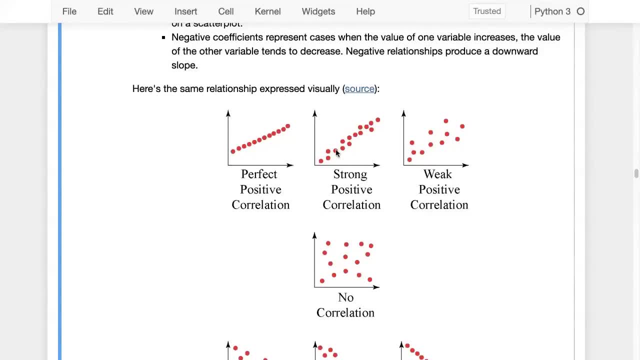 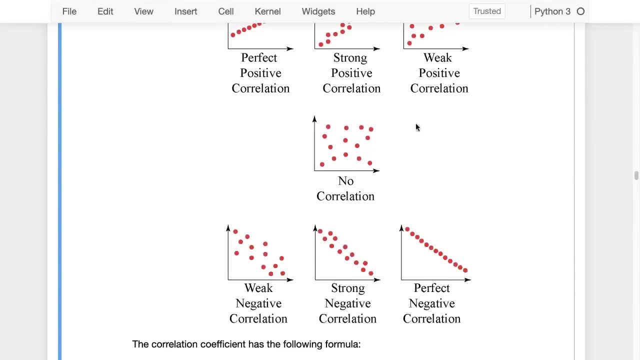 You have like a strong positive Correlation, where these points are distributed around the line, or a week positive correlation where there is a week trained of some kind, or no correlation at all where points are all over the place. or you can have a weak negative or strong negative correlation. 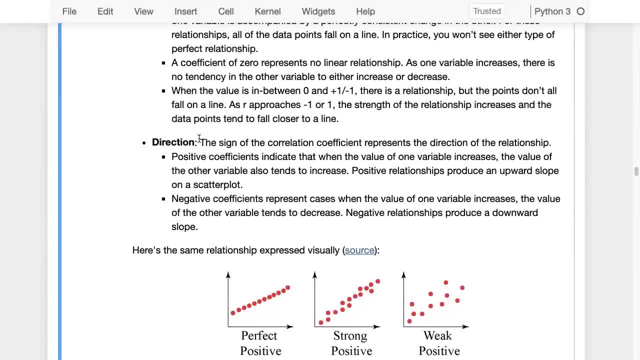 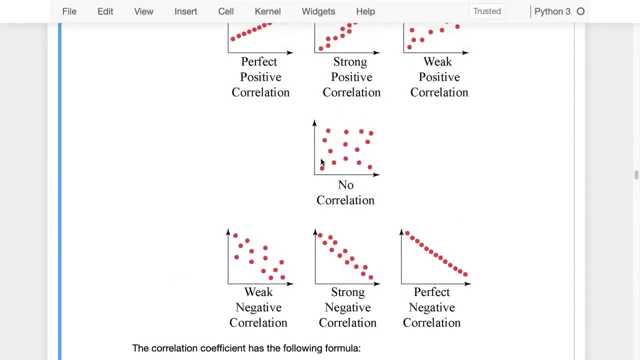 Right. So that's the direction. the sign of the correlation coefficients represents the direction of the relationship. If it's positive, then you have an increasing relationship. If it's negative, then you have a decreasing relationship. If the correlation coefficient is very close to zero, then you have practically no. 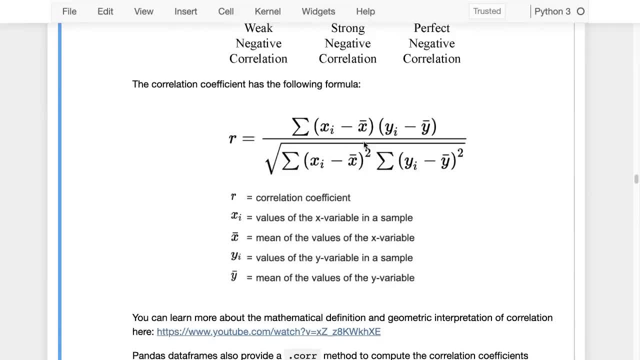 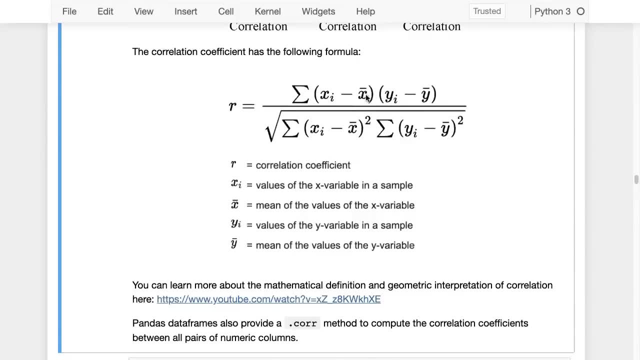 Correlation, Okay, And the correlation coefficient has a formula and you can check out this formula. This is simply the sum of X minus the mean of X, Y minus the mean of Y added up, divided by a square root of some other quantity. 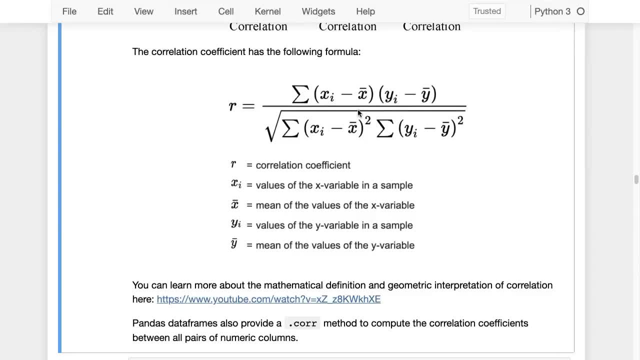 I'll let you figure out what this formula means, because it's not very important. It's simply a question of carefully looking at each of the terms and listing out what it means, but this is the more Important interpretation that you should have. 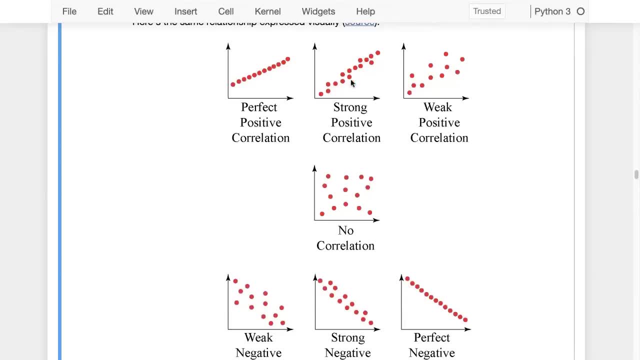 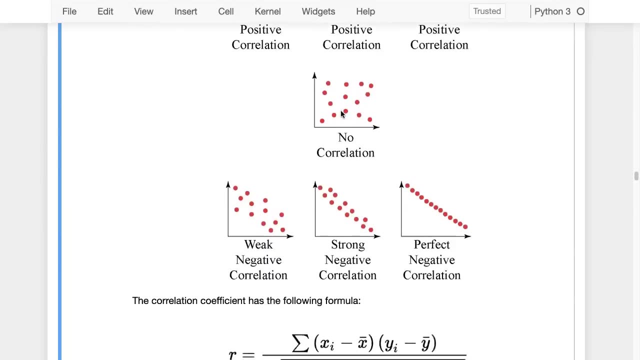 When you see correlations, you see plus one. This is what you see. You see something, let's say, greater than 0.5, greater than 0.7.. This is what you should imagine. less than 0.5. This is what you should imagine. close to zero is this and less than zero? 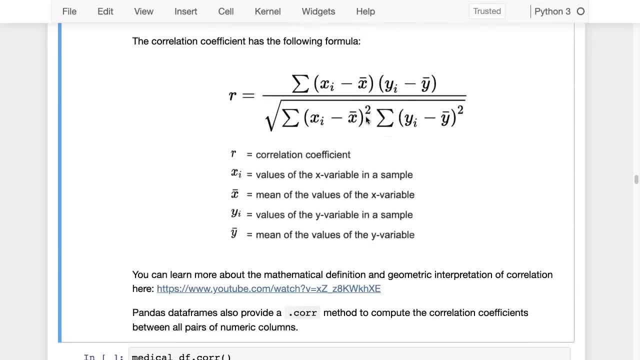 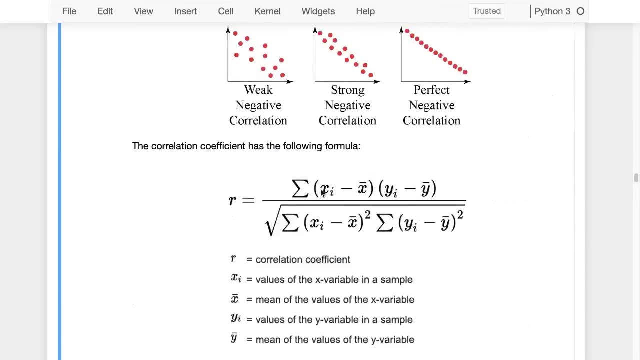 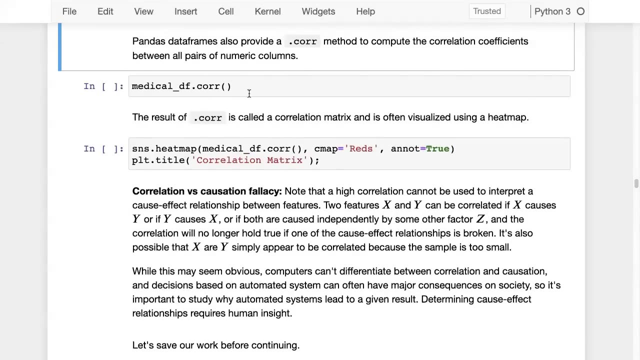 These are the pictures you should have in mind. Okay, If you really want to learn the mathematical definition and the geometric interpretation, I have linked to a video here, but this picture pretty much summarizes everything we need to know. Okay, Now the pandas data frames also provide a CRR method to compute the correlation coefficients between all pairs of numeric columns. 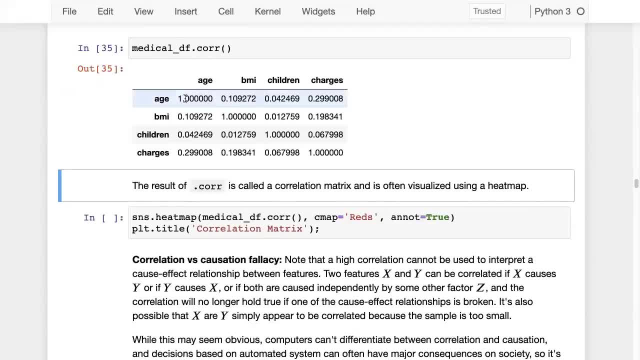 So if I just call medical DF dot C O R R, that's going to compute the correlation between each BMI, children charges, which are the numeric columns, with the other numeric columns And you can see age and age. So age has a perfect correlation with itself. 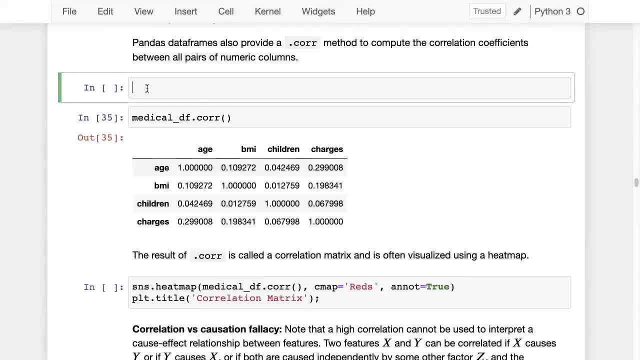 If you plot age with age- and you can do that- you can do something like this: P X dot scatter, You have medical DF, X equals age and Y equals age. You see that there's obviously a perfect correlation. It's a straight line. 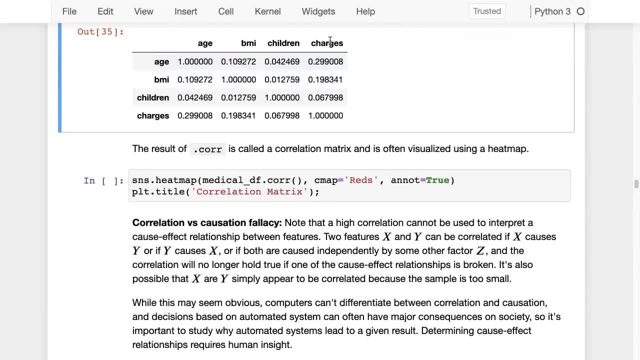 So age has a perfect correlation, but what we're interested in is the correlation of charges with the other columns. You can see that age has a correlation of 0.2, nine nine, which charges BMI, has a weaker correlation of 0.1, nine eight and children has an even weaker correlation. 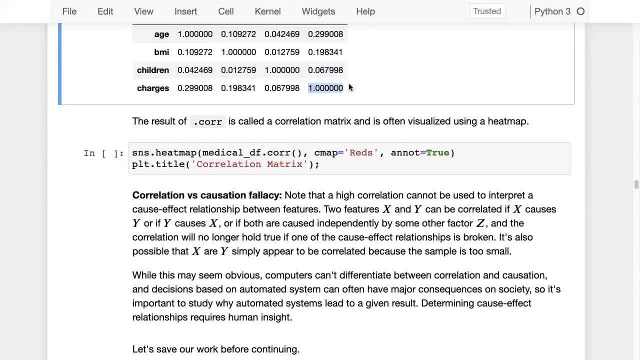 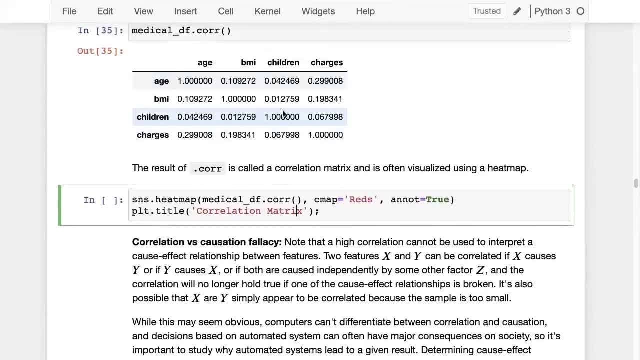 Of 0.067.. Okay, And finally, charges, with charges obviously has a correlation of one. Now, this is normally displayed using a heat map, because it's difficult to look at all these numbers and figure things out, So you can just show a heat map like this: 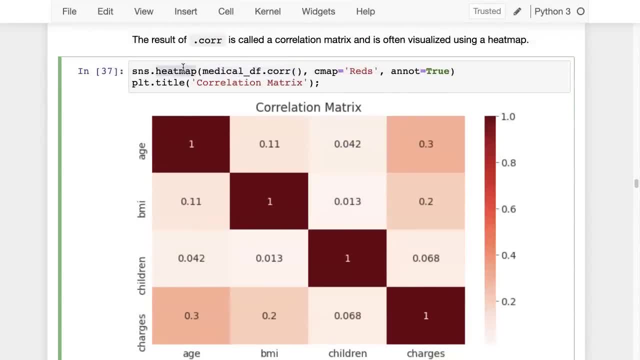 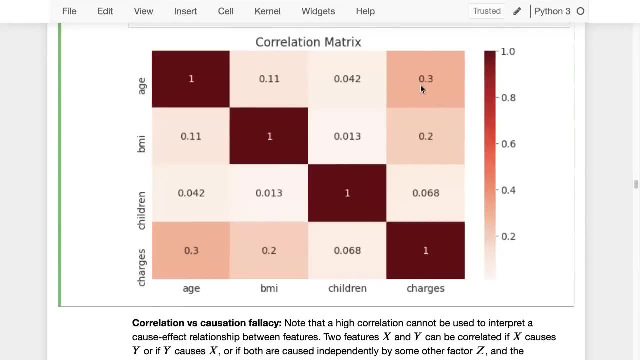 This is called a correlation matrix. I've simply passed it into SNS dot heat map from Seaborn And this also adds some color and helps you visualize that seems like agent charges have a high correlation. Okay, So that's the core. 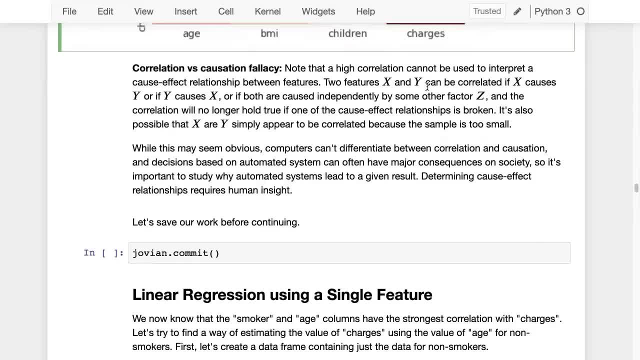 Relation matrix. And one last thing I want to mention is the correlation versus causation policy. Note that a high correlation cannot be used to interpret a cause effect relationship between features. Two features, X and Y, can be correlated If X causes Y or if Y causes X. you can see that in the formula. if you replace X with Y and Y with X, nothing changes. 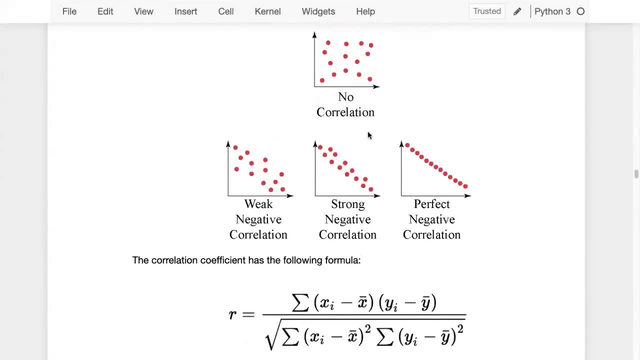 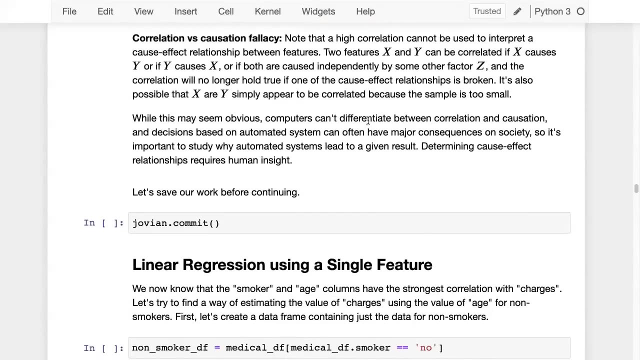 It's the same formula. If you flip the axis here, nothing changes. The relationship remains the same. So it does not Give you a direction to interpret causation in. Okay, That's very important. X could cause Y, or Y could cause X, or it's possible that both are caused independently by some other factor Z, and the correlation will no longer hold true. If one of those cause effect relationships is broken, like if Z causes X and Z causes Y, but if you fix or change whatever effect Z has on Y, then X and Y will no longer be correlated. So that's why I do not interpret cause effect relationships from correlations. 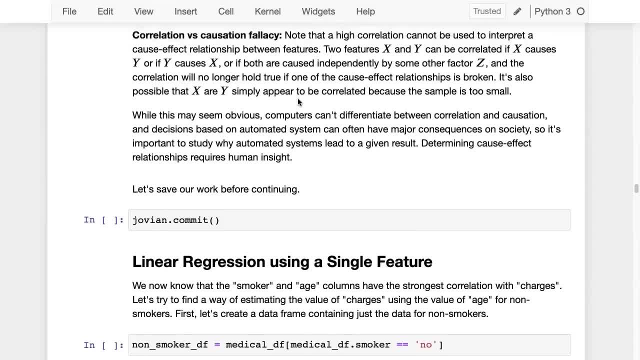 It's easy And a lot of people do it, even though it seems obvious. a lot of people do it, but it's wrong. Just to give you an example, for example, if you, let's say, created a scatterplot between race and income, you would find that maybe a certain race has lower income and a certain race has higher income. 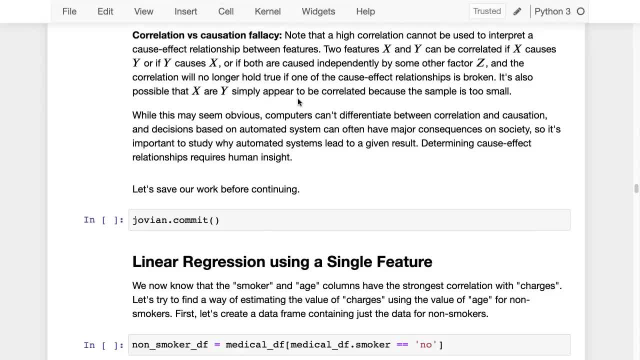 And if you want to create a cause effect relationship there, you could say that income is a function of race, that if you belong to a certain race you will learn less, and then you may read more. So you could say that income is a function of race, that if you belong to a certain race you will learn less, and then you may read more. 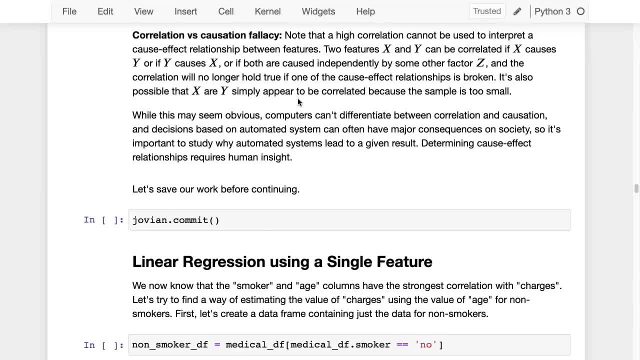 So you could say that income is a function of race, that if you belong to a certain race you will learn less, and then you may read more, And so that's why I do not interpret cause effect relationships as a cause effect relationship. But it's possible that this is because of something else entirely. 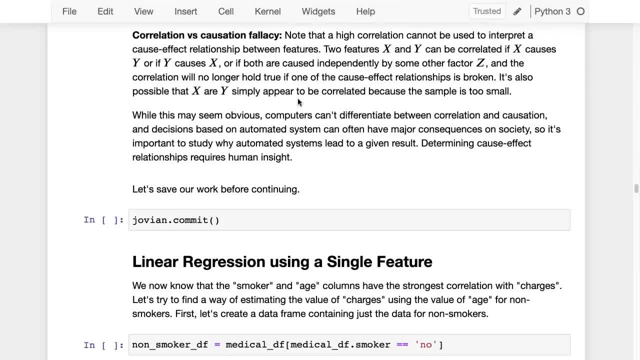 For example, Racism, systemic racism- that may have caused incomes to be lower for a particular race- Right- And once you fix that, and maybe if you control for that, if you see people who have not been subjected for several generations to racism, you might find that you no longer have the same correlation. 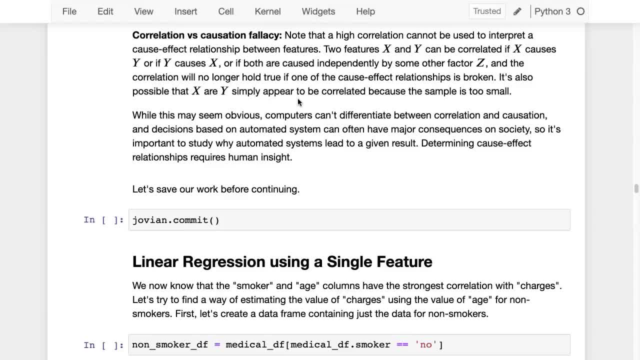 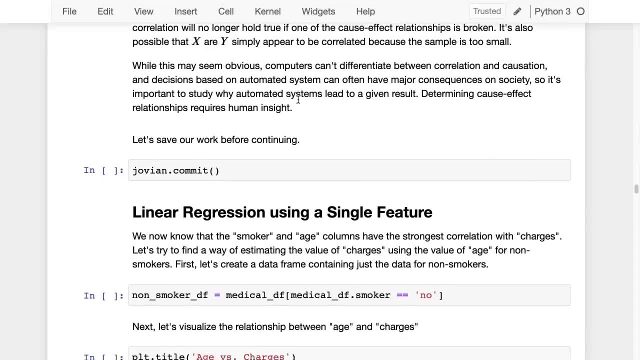 Right. So try not to read too much into these graphs. Right, Right, Right, Right, Right, Right, Right, into these graphs. always be careful, because it's a very natural human tendency to create these interpretations. And when it becomes even more magnified is when these into these correlations. 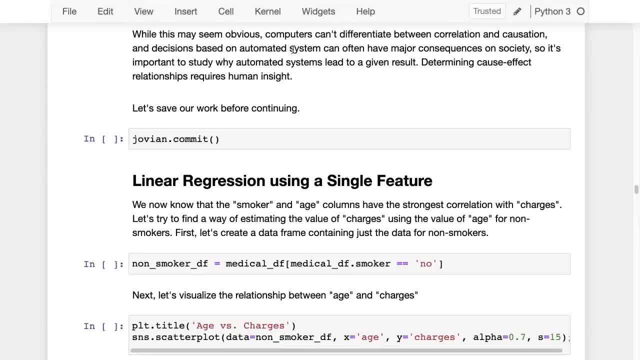 are captured in automated systems. computers cannot differentiate between correlation and causation, And decisions based on an automated system can often have major consequences on society. So it's important to study why automated systems lead to a given result, And again, another example of this. you may have heard about this: facial recognition technology. 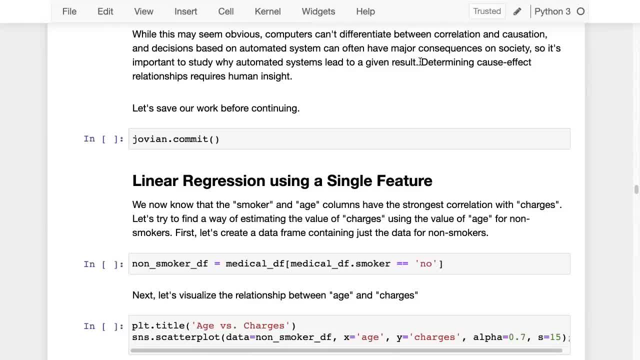 developed by Amazon is being used in law enforcement, And it just so happens that, because of the current distribution of people who are incarcerated, a certain race has a higher representation in the incarcerated population, And so the model is more likely to predict a person with a certain race is a criminal. 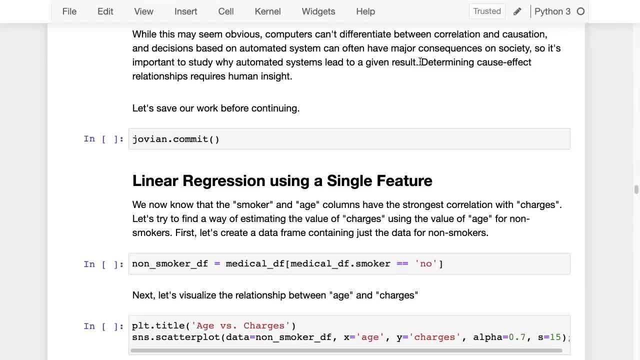 Or detect them as a criminal, And so more people are likely to be incarcerated from the same race, right? So it can actually aggravate the problems, the problems we have in our human systems, And that is why it's very important to be mindful of why we're getting a certain result out of a 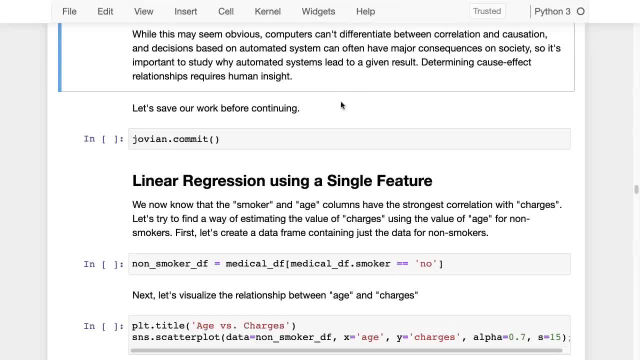 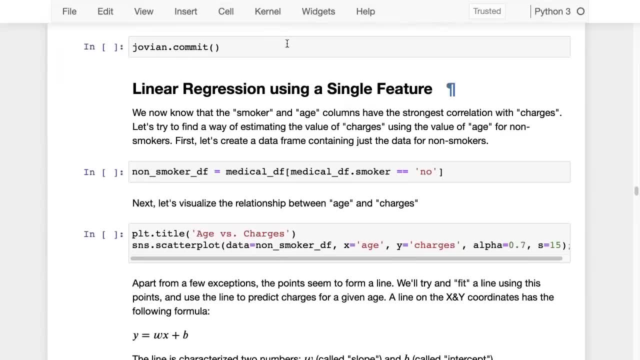 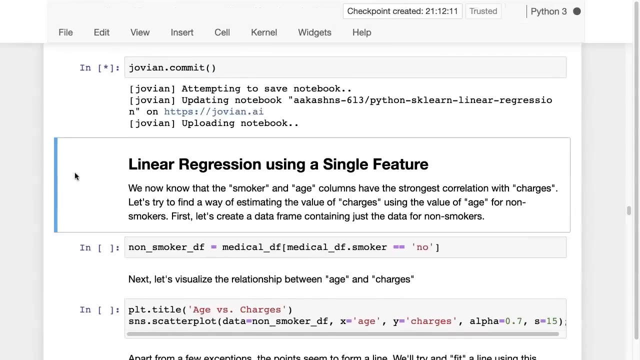 system that we create and realize that determining cause effect relationships requires human insight. we shouldn't blindly trust computer systems. Okay, So that's just one small note about correlation and causation that you should keep in mind. Okay, So that's our exploratory data analysis. We've done a lot of analysis. We've spent half the lecture just doing analysis. 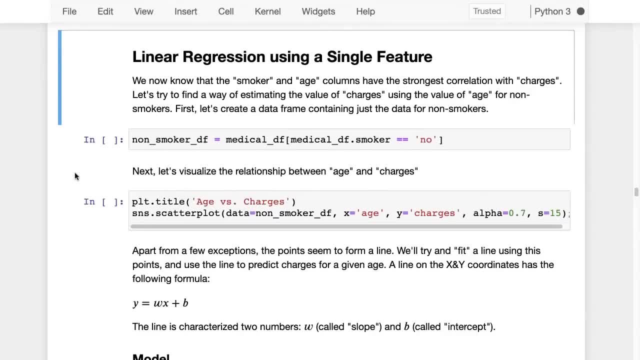 but it's important. Once you, this is a more important piece of machine learning really, which is before you get to the actual machine learning, and then the machine learning part becomes fairly straightforward after that. Okay, So let's move on to linear regression with a single feature. 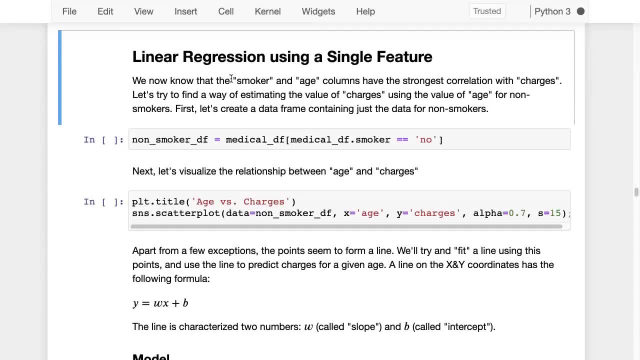 And we'll define what linear regression is. We know that smoker and age the columns have the strongest correlation with charges. We've seen that already. So let's try a way of finding, or let's try a way of estimating the value of charges using the value of the age column. 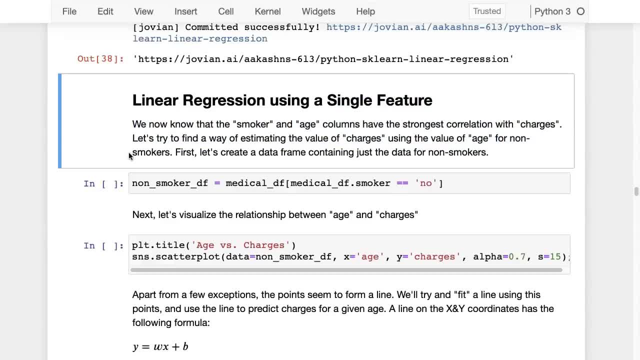 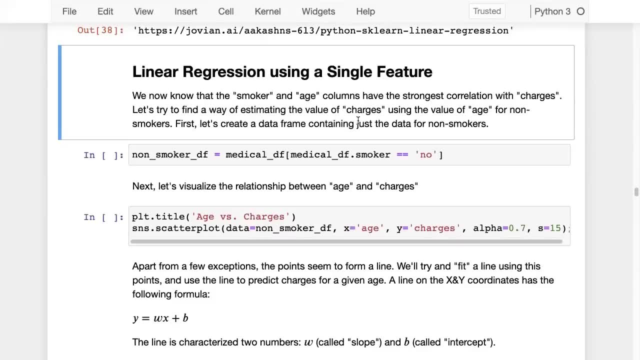 We can't really use smoker because it's just a yes, no value. So how exactly are you going to use that to predict charges? but the age has a continuous value. So let's do one thing: Let's estimate the value of charges using the value of age, just for non-smokers. 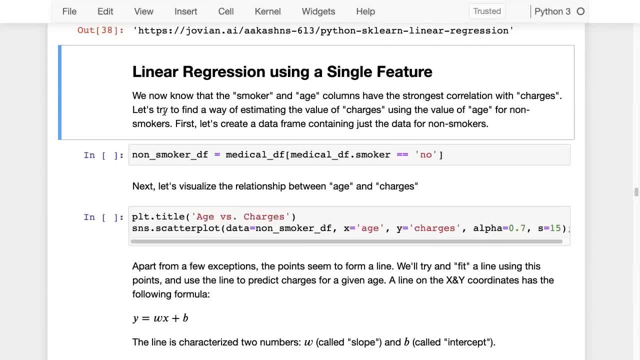 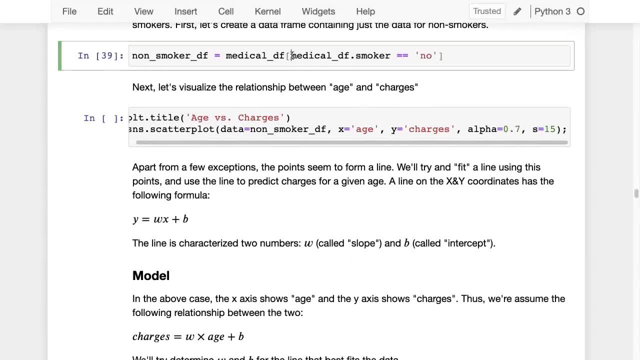 And then we'll deal with smokers later. So first let's create a data frame containing just the data for non-smokers. Okay, And that's done. We simply pick medical DF dot- smoker equals no- and pick those rows of those columns of data from medical DF. 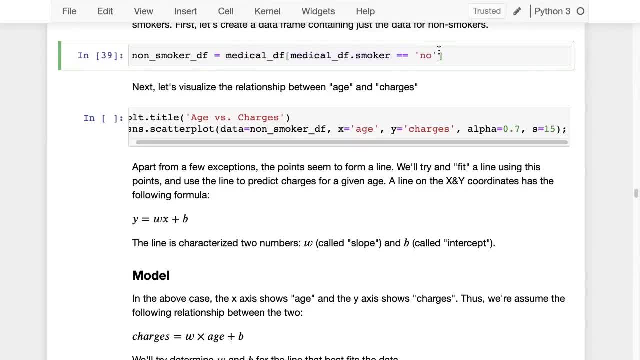 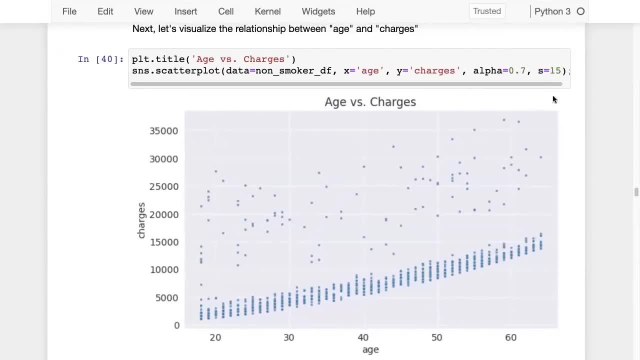 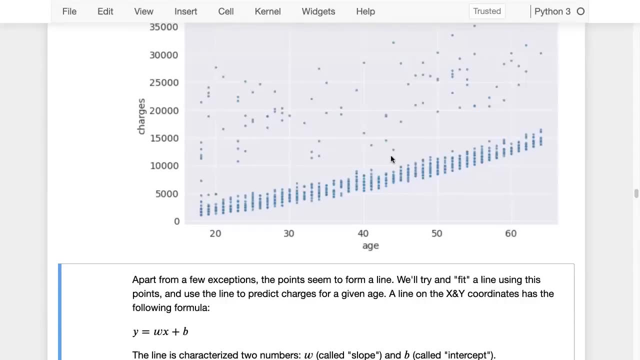 Sorry, those rows of data which belong to non-smokers from medical DF. And let's plot Once again. I'm just using a CBON scatterplot this time Don't need any interactivity, And you can see the strain that there seems to be a generally linear train that I could maybe fit a line here. 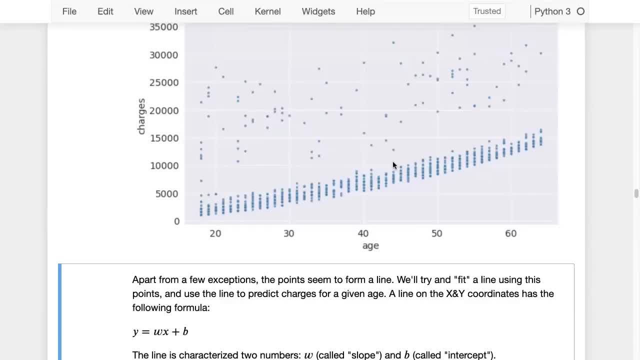 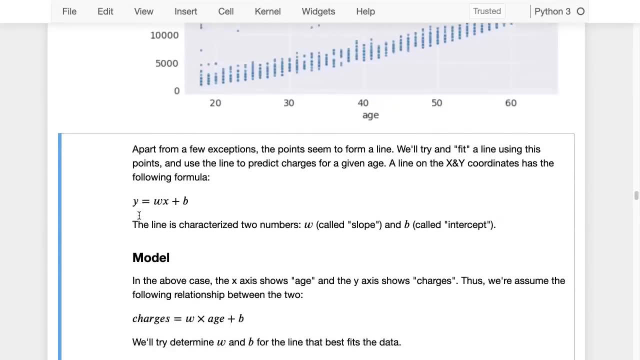 Although there are a bunch of outliers. So maybe I move my line up a little bit just to account for the average. Yeah, So, maybe a line like this would be ideal. Okay, So, apart from a few exceptions, the points seem to form a line and we'll try and fit a line. 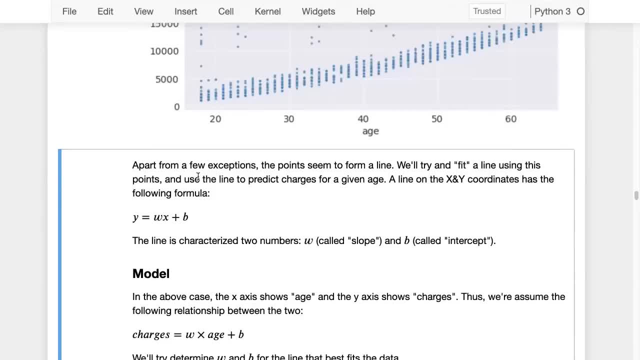 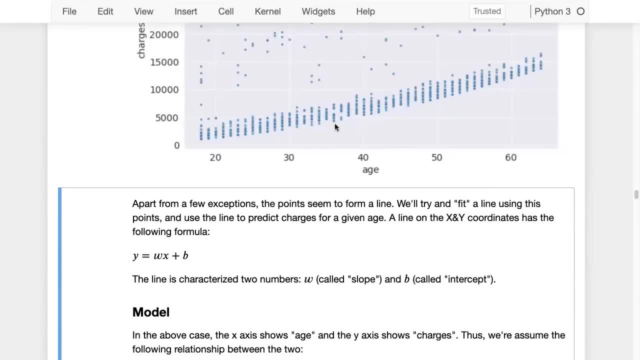 Using these points, And then we will use that line to predict charges for a given age. So let's just fit a line somewhere like this, And once the line is fit, let's say somebody, a new customer, comes in and they provide their information. 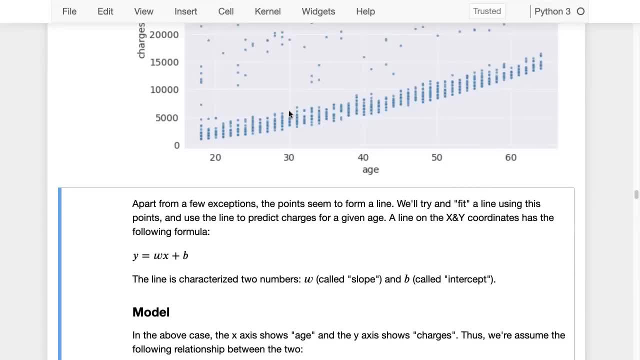 Let's say they're 30 years old. Then we'll just look at the line and we'll see where the line intersects the Y axis or the Y value for the line at 30. And that would be maybe somewhere around here And we would predict that their medical charges are maybe 5,200.. 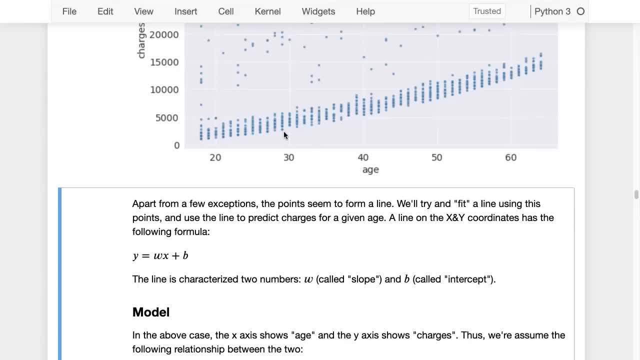 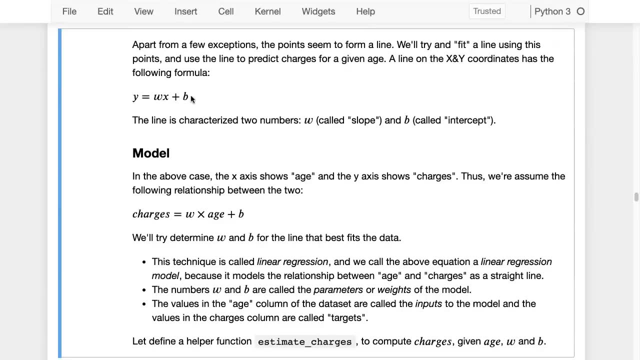 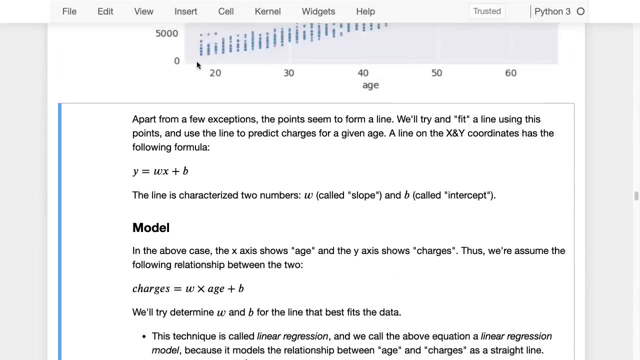 Okay, That's how prediction works. Once you get the line, you use the line To make predictions, and a line on the X and Y coordinates has a formula like this: A line has a formula: Y equals W, X plus B. So as you make changes to the value of X, the value of Y changes, and it is determined by two factors. 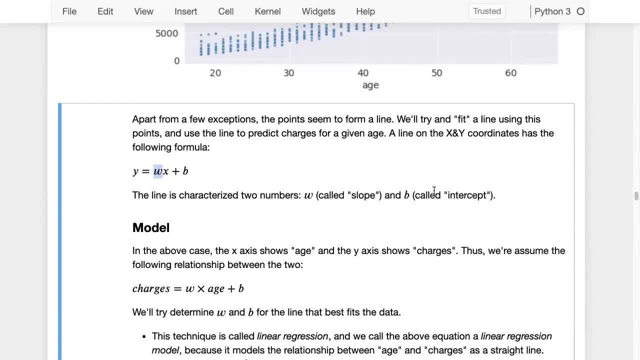 So why the number W is called the slope and the number B is called the intercept? Okay, So what you do is you pick a value for W- Let's say you pick that W has the value a hundred. Okay, And you pick a value for B and you say B has the value of 50.. 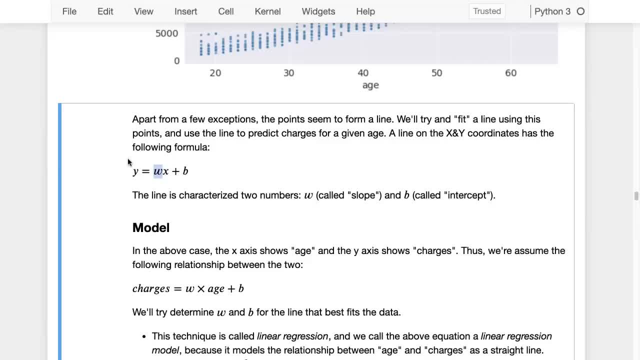 And as you change the value of X, the value of Y changes and that is what draws a line on the 2d plane- basic geometry, something you would have seen in high school- And W is called a slope because it determines how much change you will see in Y when you make some change in X. 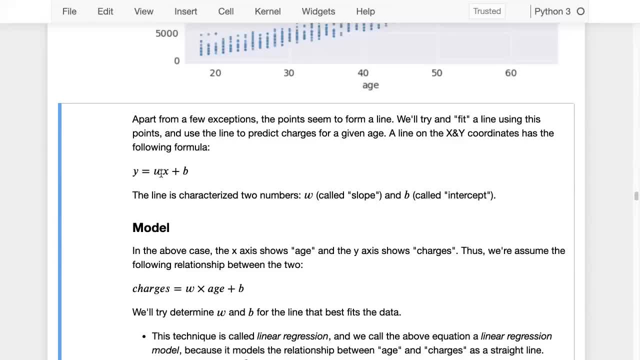 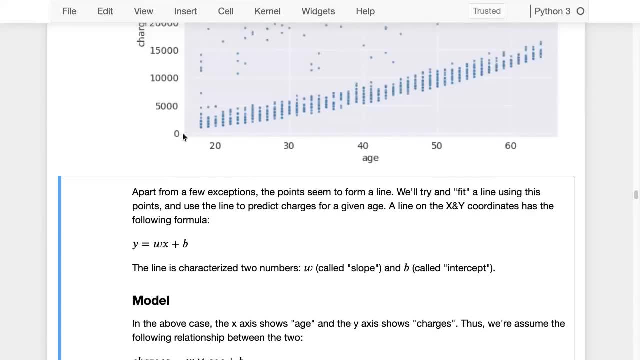 So the, the rate of change of Y with respect to the change in X, is W And B is called Intercept, because B is the value of Y. when you said X equals zero, So X, X equals zero means this. So that means a. B is the point at which the line intersects with the Y axis and that is called the intercept. 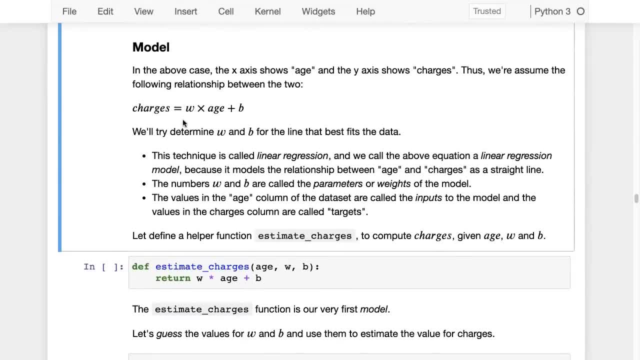 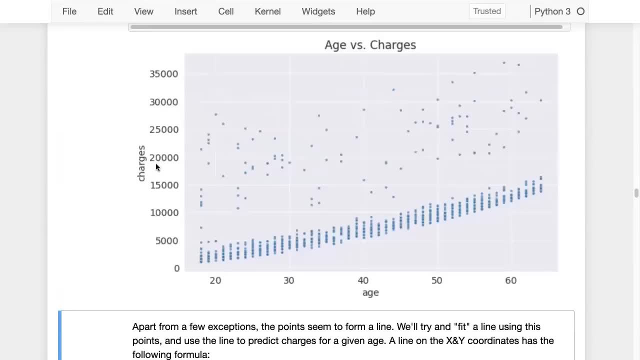 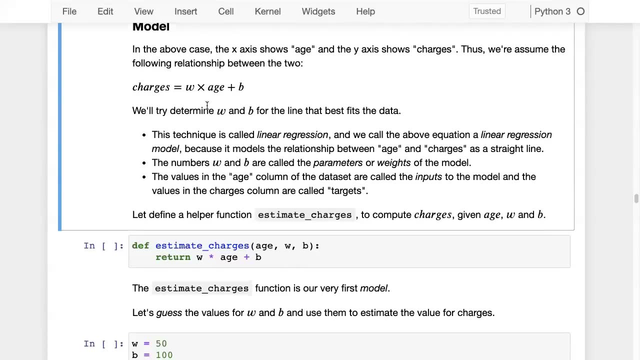 Okay, So in the above case, in this graph, the X axis represents age and the Y axis represents charges. So what we're trying to say essentially is that we are Assuming that charges and age have the following relationship: We are saying that the charges is some number W multiplied by age plus some number B, and we will then try and figure out a, W and B to get the line that best fits the data. 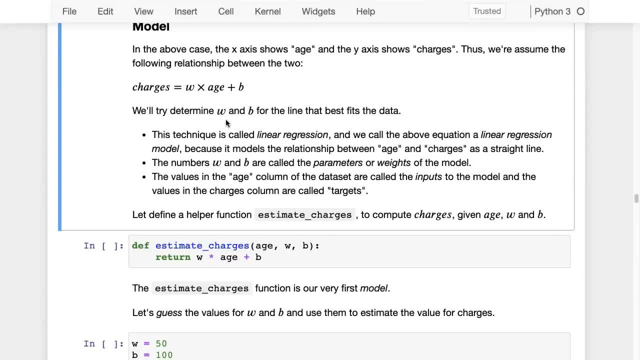 Now, obviously this is not a perfect relationship. Medical charges depend on a lot more than age, as we've already seen, And maybe you can't even predict medical charges exactly, because there's a lot of uncertainty, but there's a certain trend we are trying to capture. 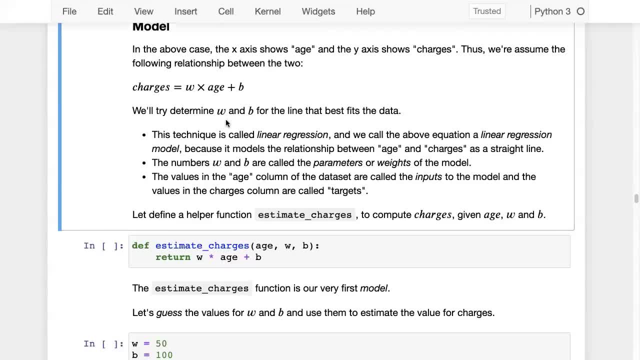 Because some information will be more useful than no information. at least, knowing that a person at a higher age we should probably be charged a higher premium, is useful information that we'd like to draw. Okay, So here we have. charges equals some weight, W, or some number, W plus B. 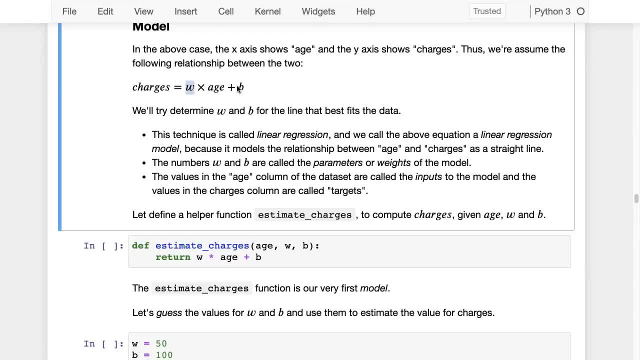 Now this number W is also called a weight sometimes, And then this number B is called a bias. So they're called slope and intercept in geometry, but they're often called weight and bias In statistics and machine learning. in any case, this is a relationship that we are assuming. 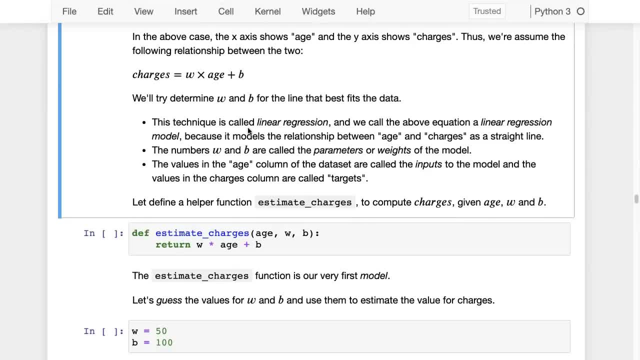 Okay, So this technique is called linear regression and we call this equation a linear regression model because it is modeling the relationship between age and charges. You are setting forward a hypothesis that the charges is some weight W multiplied with age, plus some number B. 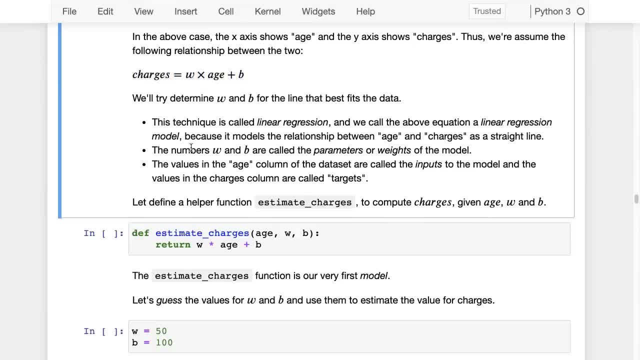 So this is our model. This, literally this equation, is our model. And then the numbers W and B are called the parameters or the weights of the model. So the model has a structure or an equation and the model has some parameters. 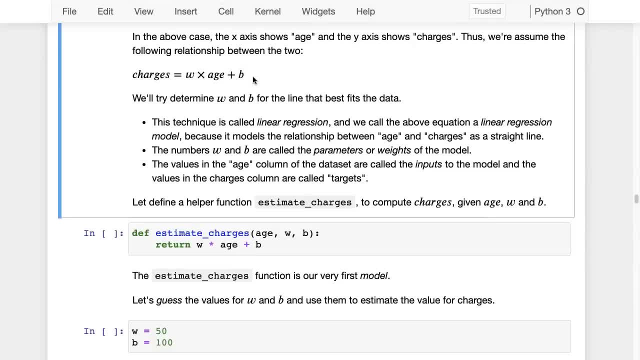 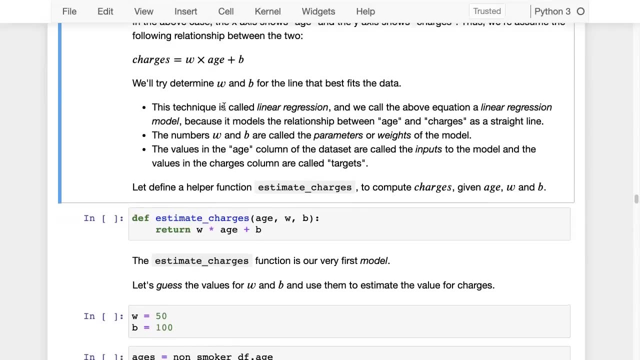 As you change these parameters. you will still have a line. The structure will be maintained but the line will move around. So the model will give different predictions When you input a certain age. it will give a different output for charges As you change the values of W and B. finally, the values in the 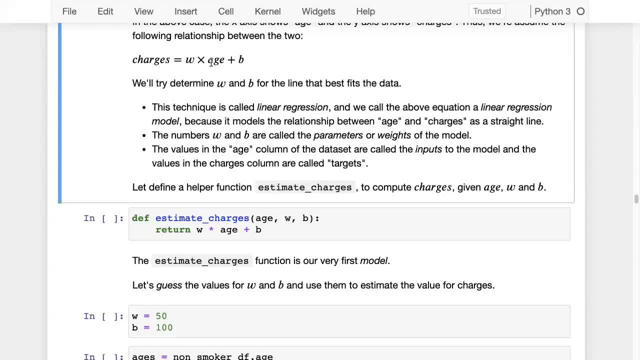 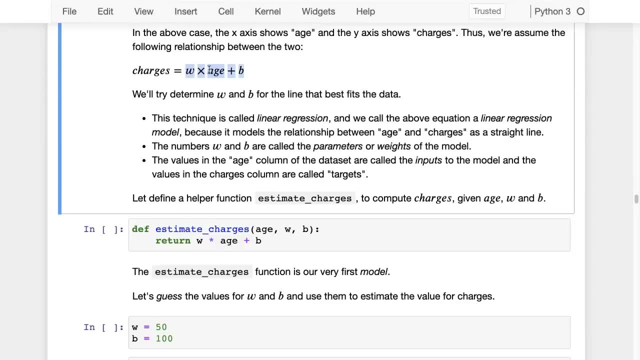 Age column of the data set are called the inputs to the model and the values in the charges column are called the targets. So we assume that when we multiply the inputs with this number, W and add B, we are going to get something close to charges, and we want to get as close as possible. 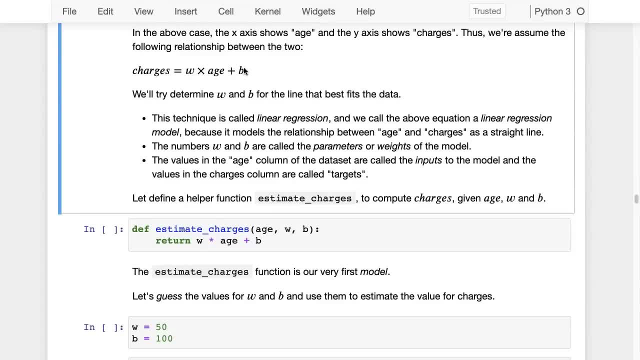 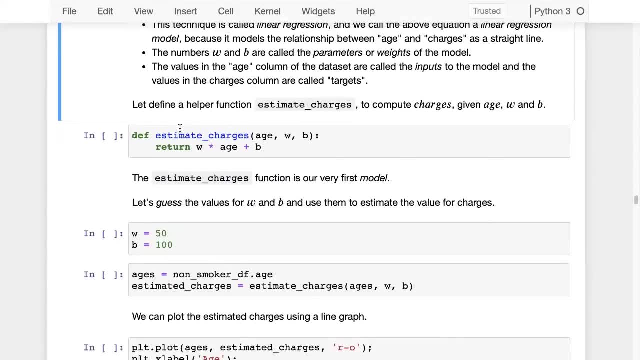 Okay, So that's our linear regression model. It's called linear regression because it's a line and we're trying to fit the line. So we're trying to make sure that the line fits as closely as possible with the points No this: 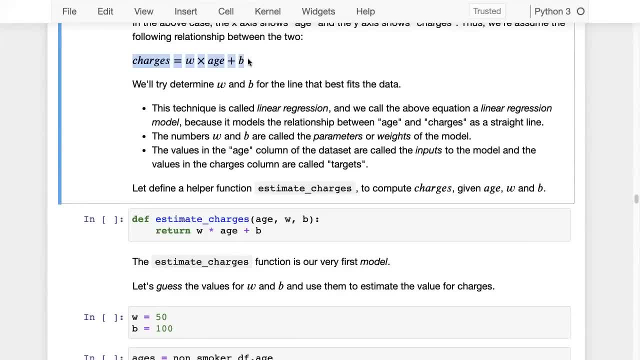 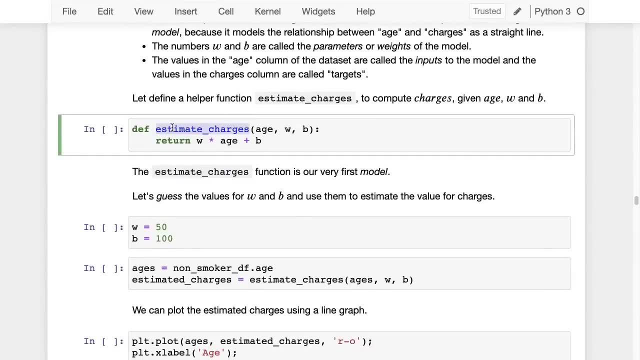 Okay, Question is well and good, but we would like to express it in a way that we can compute, which is using code, So we can turn this equation into a function. So let's define a helper function- estimate charges- which takes an age. 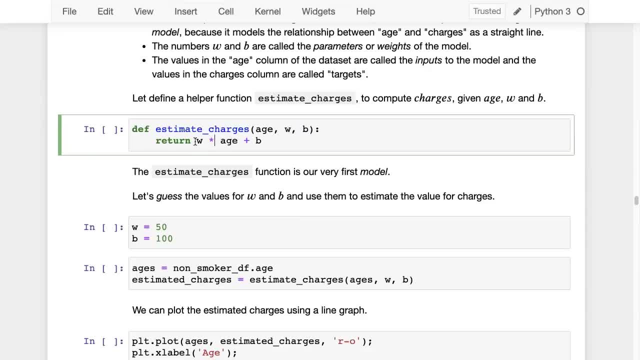 It takes a value of w, It takes value of B and it multiplies the weight with age and gives us and adds the B bias and gives us a result which is an estimate for the charges. So this function- estimate charges- is our very first. 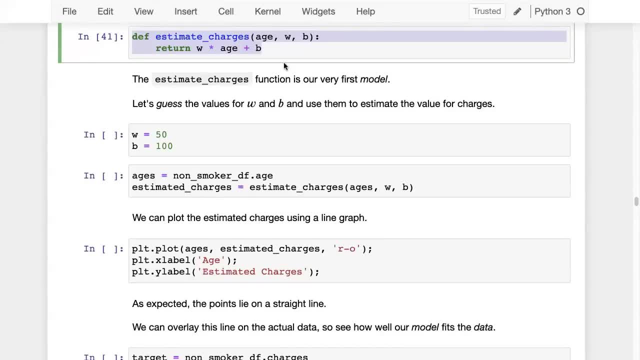 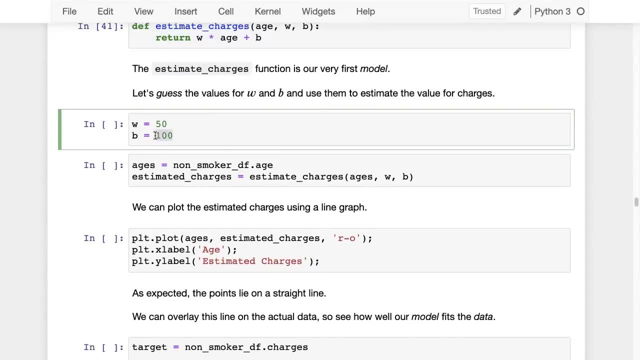 Model, our first machine learning model, and we'll define machine learning in just a second. Now we don't know what values we should pick for w and B. I'm just going to assume the weight of 50, and I'm just going to assume the bias of a hundred. 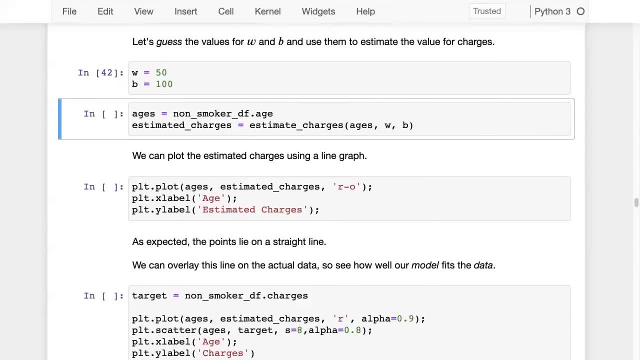 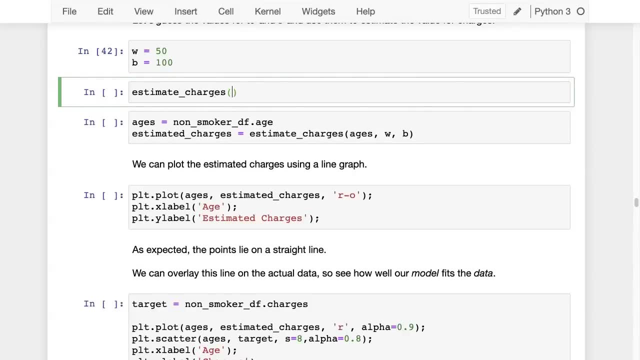 Let's see how it works out. I don't expect it to be perfect. We can call estimate charges on a single age. So let's say, now we have estimate charges, We call it on the age 30 and we pass in w and B, you would get that, the estimated charges. 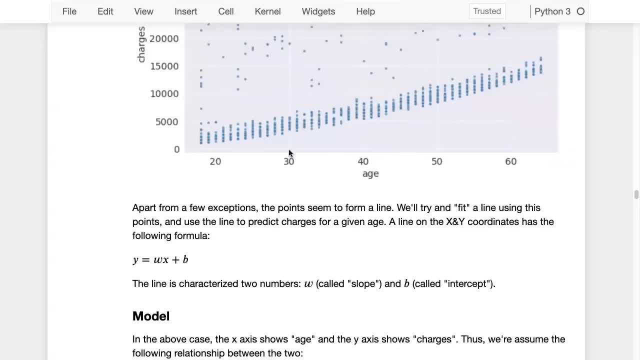 Okay, Are 1600.. Is that correct? Let's see for 30.. We are estimating that the charges are 1600, 1600 would be somewhere here. So it seems too low. So I think my guess is bad. 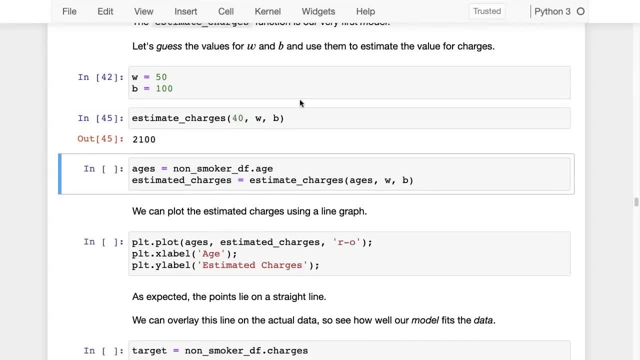 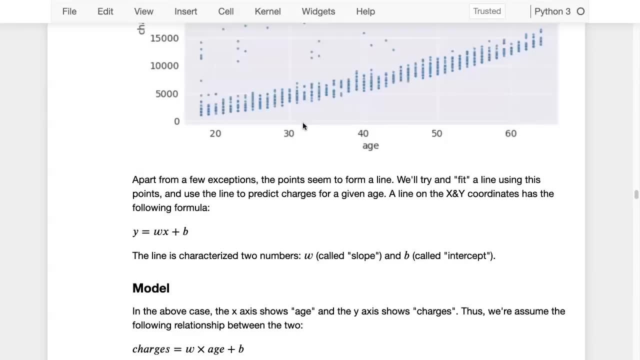 I can even maybe check 40.. So then for 40, I'm saying my estimate is 2100.. Okay, Still seems pretty bad, because 2100 would be somewhere around here. So I guess my line is going something like this: 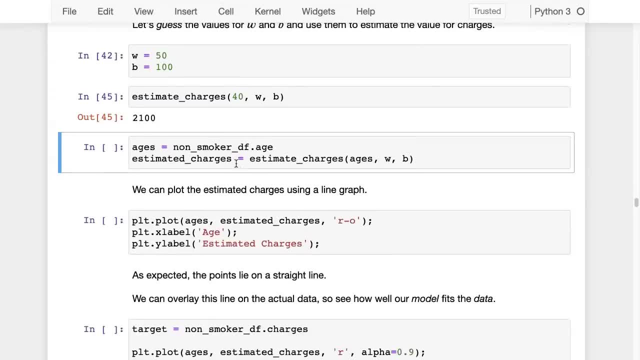 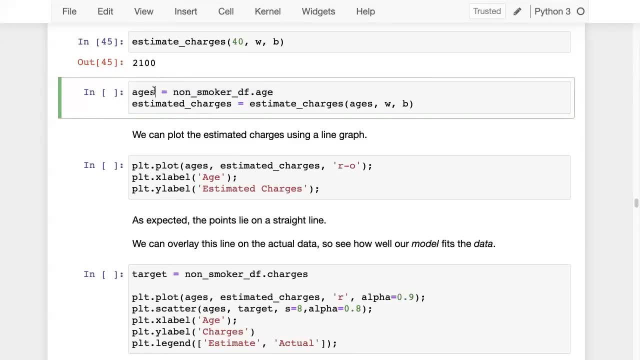 It is going below these points, So maybe I should try and verify that in some way. Here's what we can do. Let me take all the values in the age column: non-smoker, DF, dot age. So this is a list of all the ages, right? 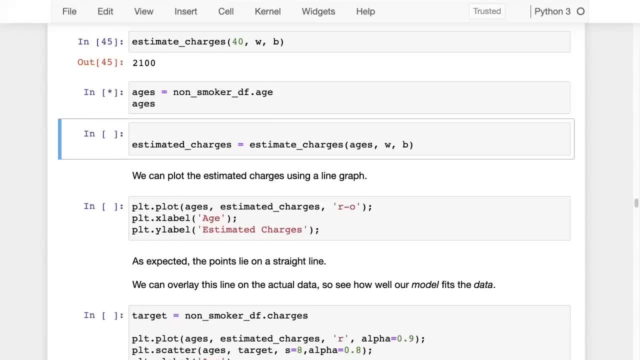 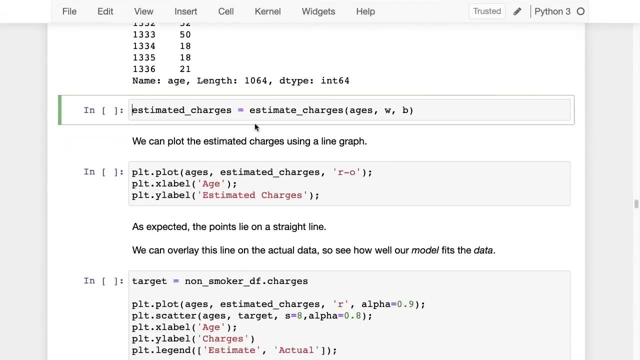 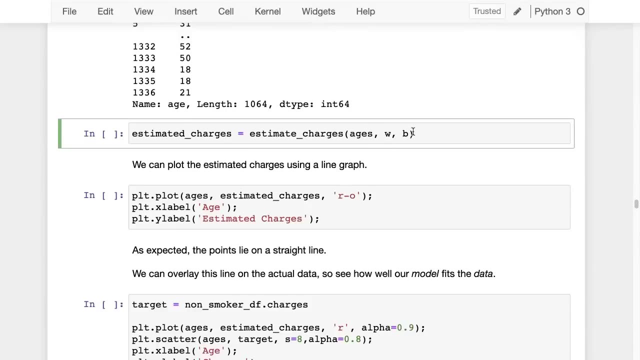 Let's just get a list of all the ages. Okay, These are all the ages that we have in the dataset and let us get the estimated charges from our model using these ages. Okay, So we put in into estimate charges, We put in ages, we put in w and B. 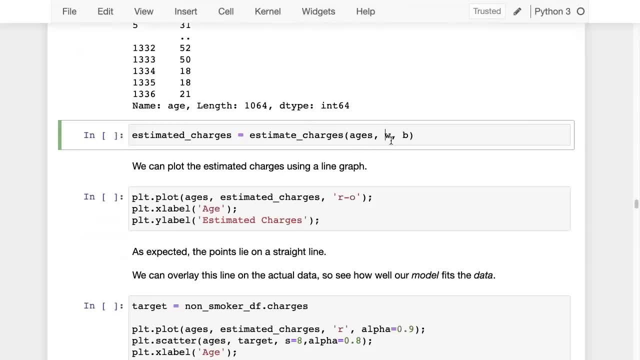 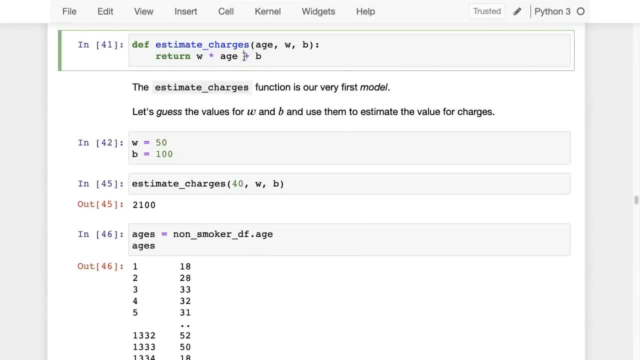 So w has a value 50, B has a value a hundred and we are going to do w Multiplied by ages plus B. now, because this is an umpire array, these same operators, multiplication and addition, work just fine for an entire area of. 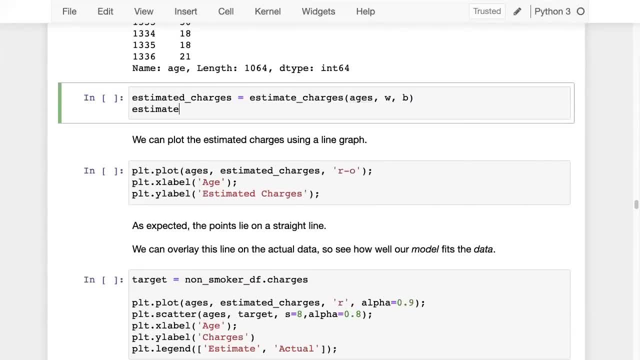 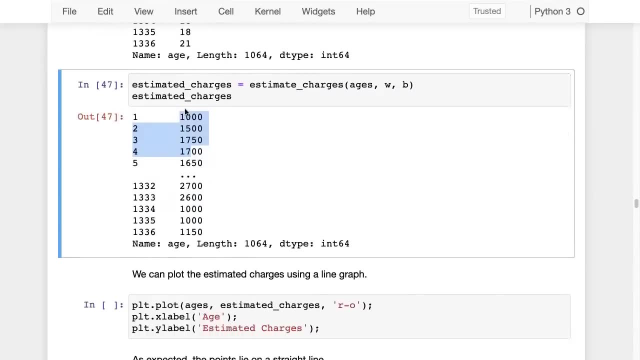 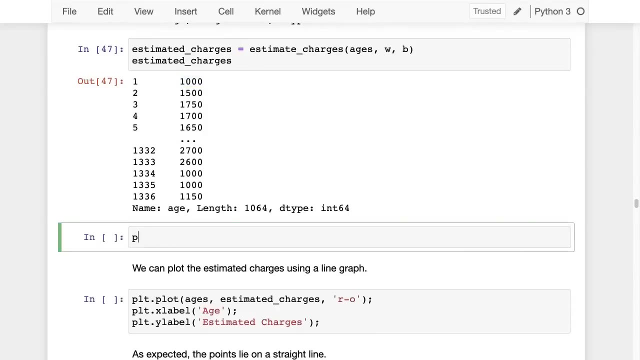 data and not just a single value. So let's look at estimated charges. So here are the estimated charges. It seems like for the age 18, the estimated cost is thousand, And then for age 28, it is 1500, and so on, and you can compare them with the actual. 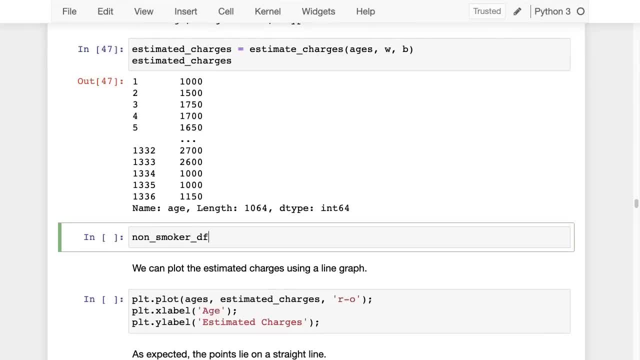 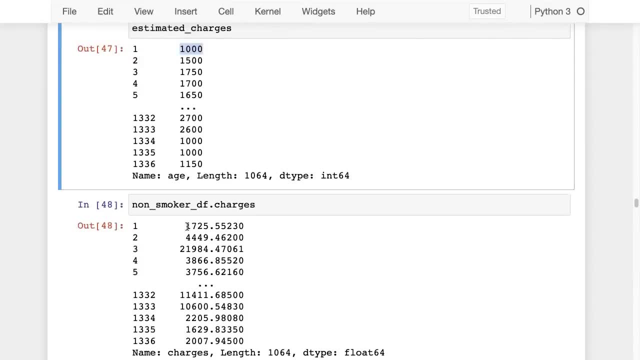 charges, which is Non-smoker DF dot charges, And you can already see that these are pretty bad. You have thousand here and you have a 1700 here. You have 1500 here and you have a 4,500 here. 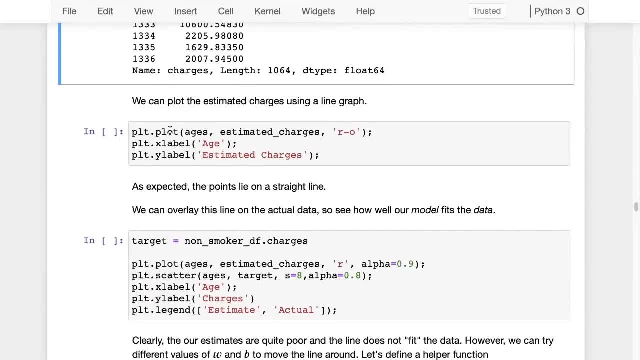 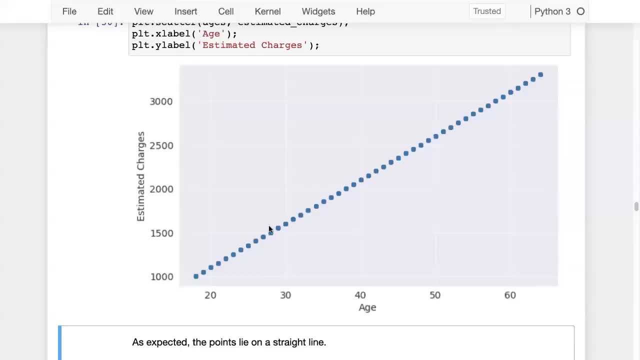 So we are way off. Let's plot what this looks like. So maybe first I'm going to do a scatter plot. Yeah, So if I do a scatter plot, this is what it looks like. You can see that the age and the estimated charges have a linear 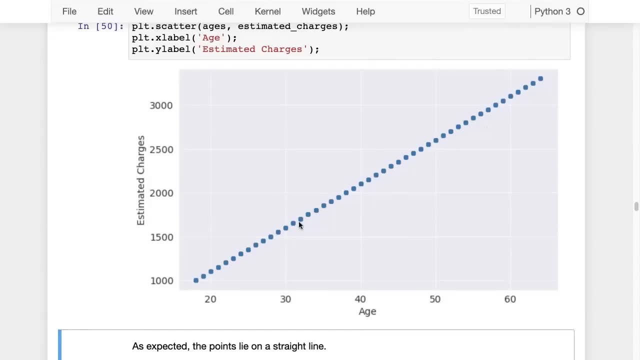 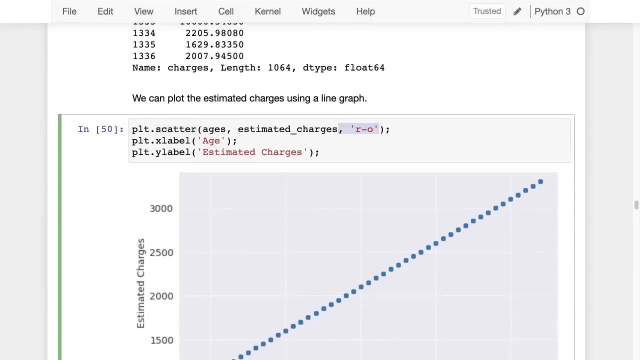 relationship and that's what we assume. We have assumed a linear relationship between them And this is what the graph looks like. So it might be even easier to just plot it as a line instead of a scatter plot. So I'm just going to put PLT dot plot, which creates a line, and just make it a red line. 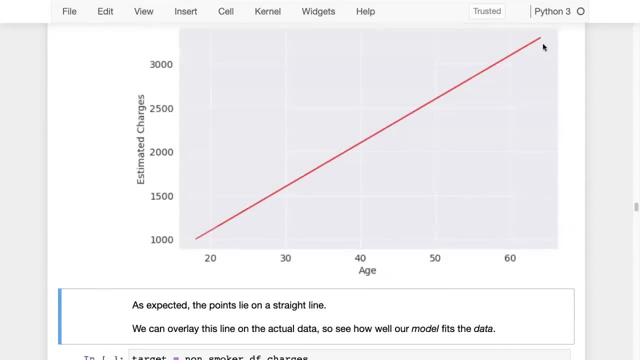 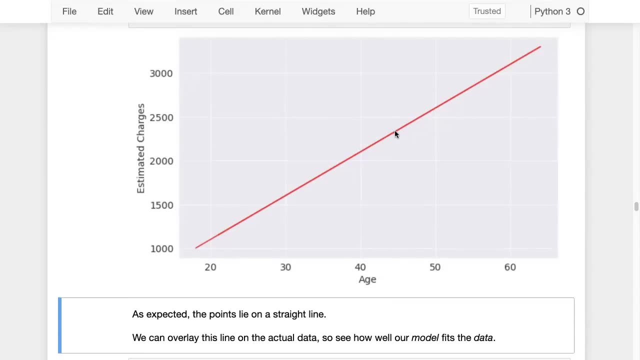 So we don't need actual points to tell us that it forms a line. We can just draw a line. And now, if you want to predict, let's say at 45,, what is the charges? So the charges would be around 2,400 or so. 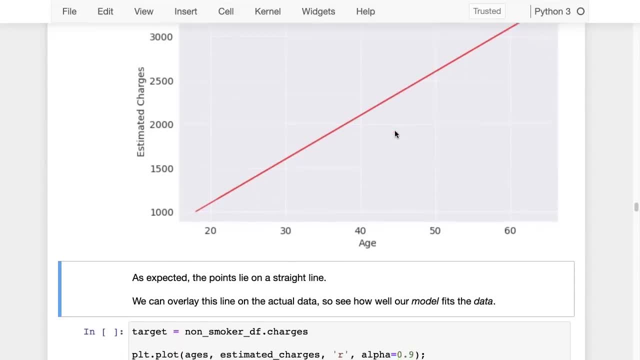 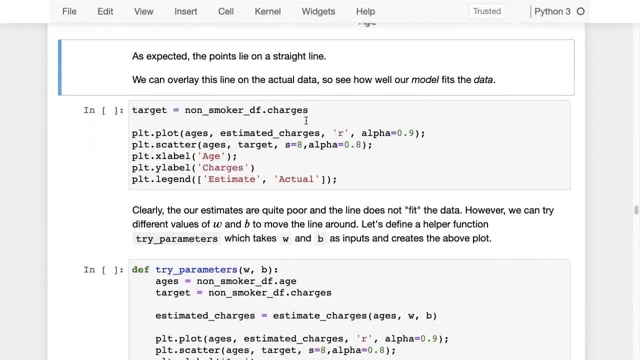 So now we have a model, We give the model Some data, some age, and it gives us an output. but we want to know how good our model is, And for doing that we can just plot this line on top of the: 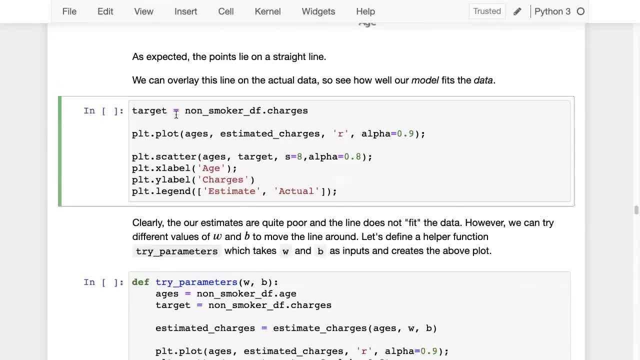 scatter plot for the actual data. So here's what we'll do: We get the actual data, which is non-smoker DF dot charges. This is the actual data that we want to predict. We get our estimates. We first bought our estimates. 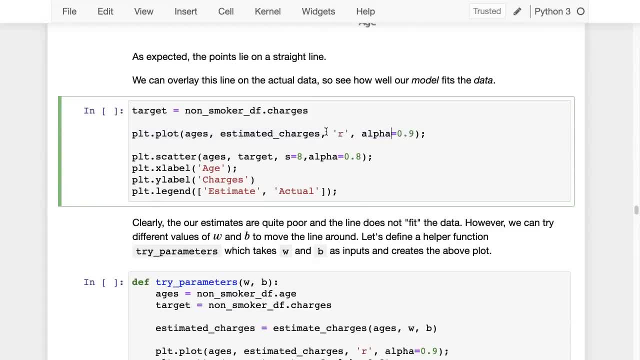 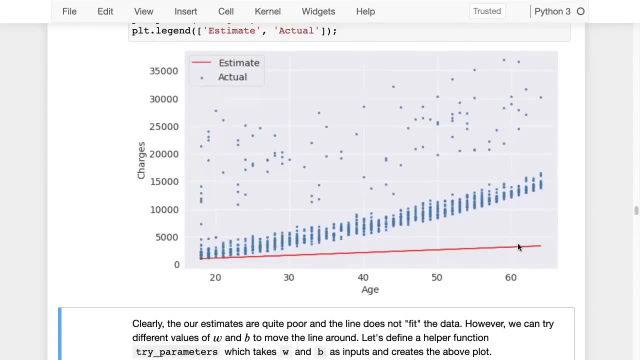 We said PLT, dot, plot ages and estimated charges as a red line, And then we plot a scatterplot of the actual data ages and the actual charges that people have incurred in our data set. Okay, So here's what it looks like. This is our estimate, based on the current value of W and B, which we have chosen, which is 50 and a hundred. 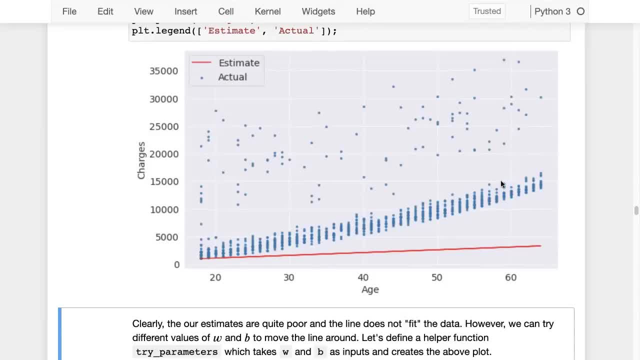 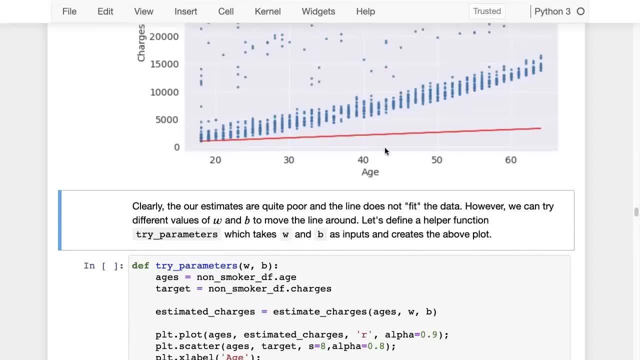 And these are the actual values of the points of the different customers that we have. So obviously this is pretty bad, This looks quite bad, but let's try and improve this. We now have a starting point and we maybe know that- Hey, maybe my weight. 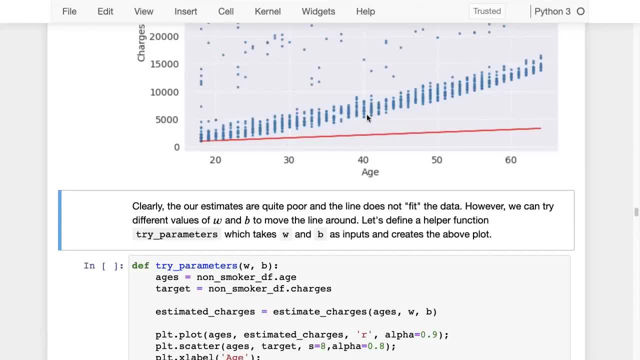 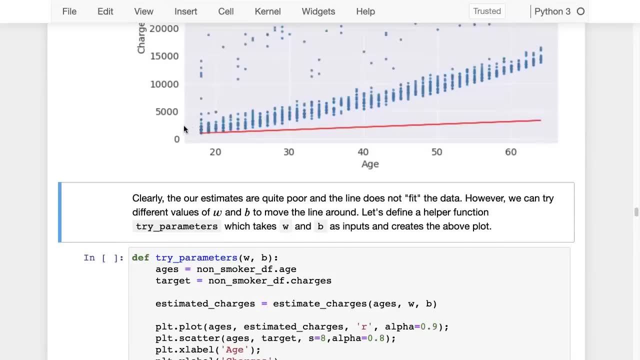 Needs to be higher, because as I go from 30 to 40, the increase needs to be higher. So maybe I need a higher weight and maybe the bias is okay. I don't see any problem. If I had a line like this, it would probably intercept somewhere here. 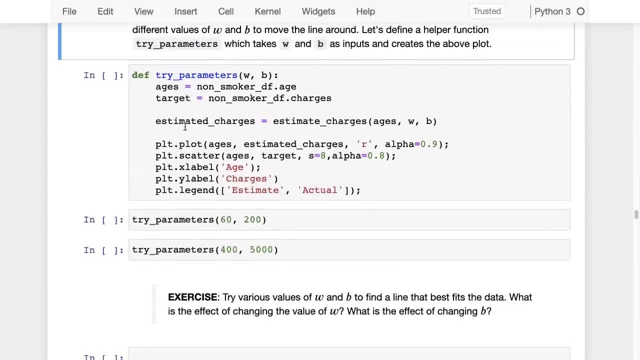 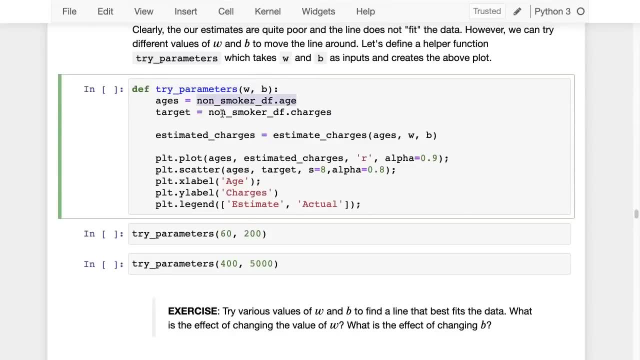 So maybe B should be around 2000.. I don't know. So I've just defined this function, try parameters, which takes W and B, and it's going to get the ages, It's going to get the targets. It's going to first get the estimated charges using the estimate charges function. 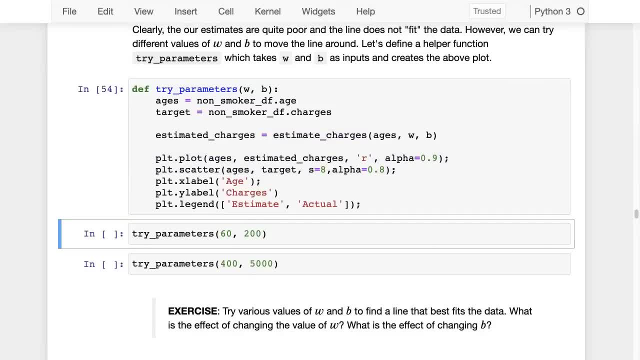 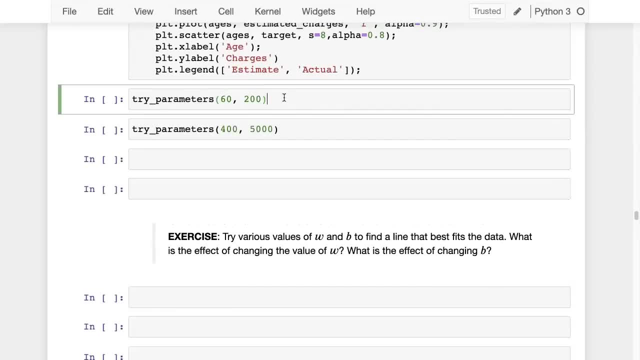 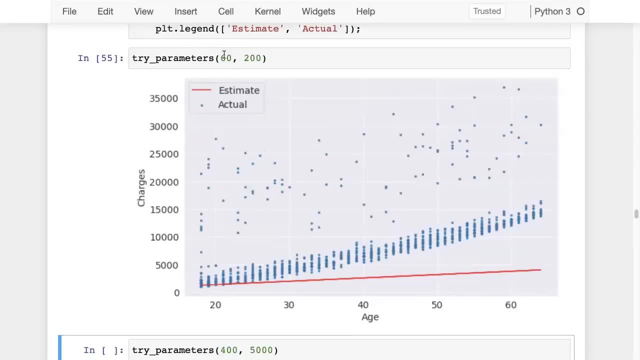 And It's going to plot the line, It's going to plot the scatterplot and we can call try parameters with different values of W and B to see what value best fits the data. So here we are calling try parameters with 60 and 200, slightly better than 50, and a hundred. 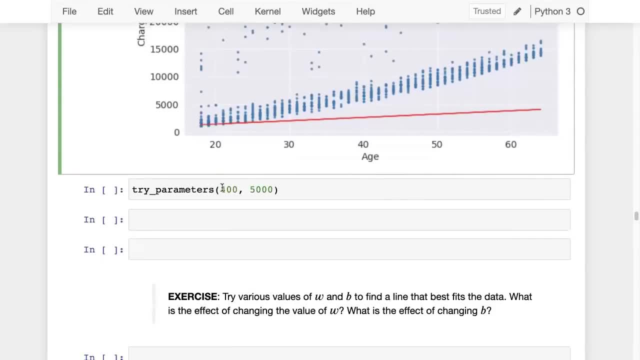 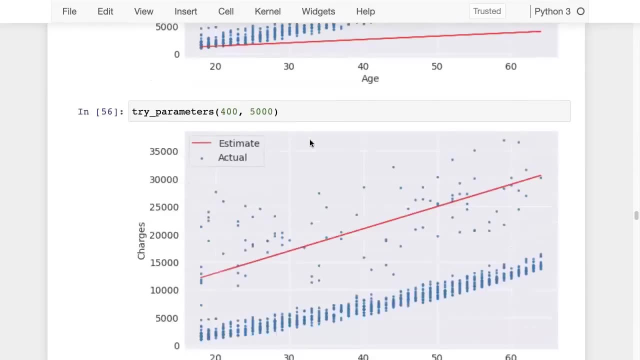 No good, still let's maybe go high. Let's go. let's increase weight to 500,, 400, and let's increase the bias P to 5,000.. Okay, That seems to have moved up the line by quite a bit. 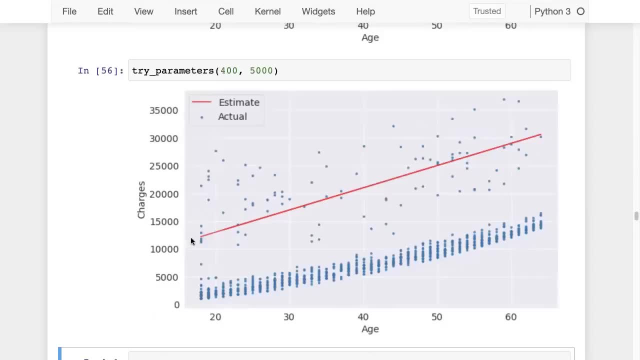 Maybe if I just shift down the bias a little bit, if I maybe, instead of doing 5,000 here, if I put in 3000, let's say, maybe that might be better. Okay, Maybe 2000.. So, as I'm changing the value of B, the line is moving down. maybe thousand. you can see that the line is moving down. maybe 500.. 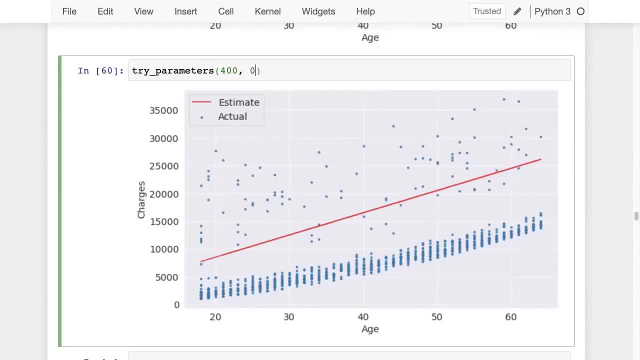 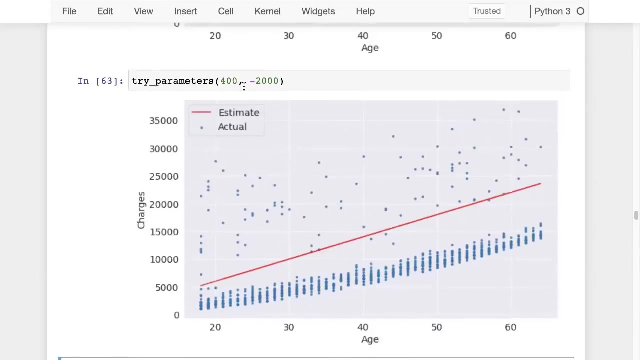 Maybe I need to go negative, even Okay, Maybe I need to go negative, So maybe go 600.. Yup, Maybe go negative 2000.. Yup, Yup. So there you go. You can now start to see what's happening as you move the line, as you change the bias. 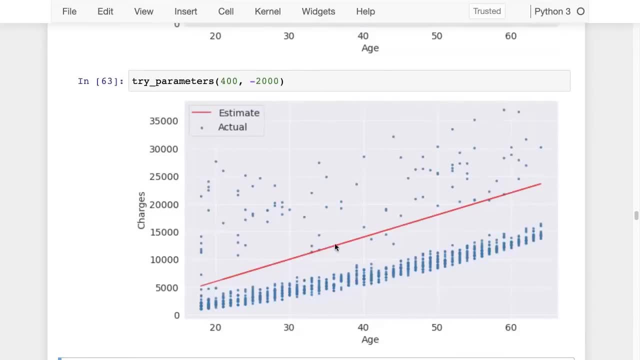 And as you change the weight, the line shifts and moves up and down. So with when you change B, that It's going to move the line up and down And when you change W, that is going to increase or decrease the slope of the line. 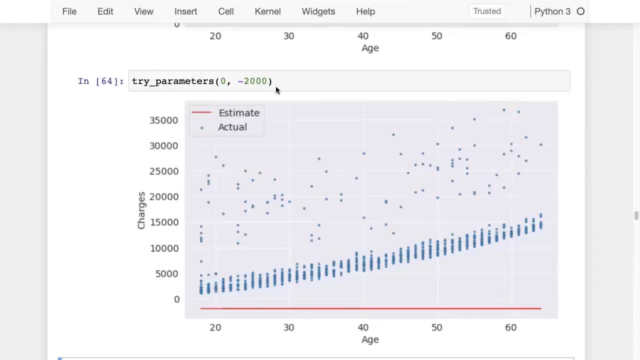 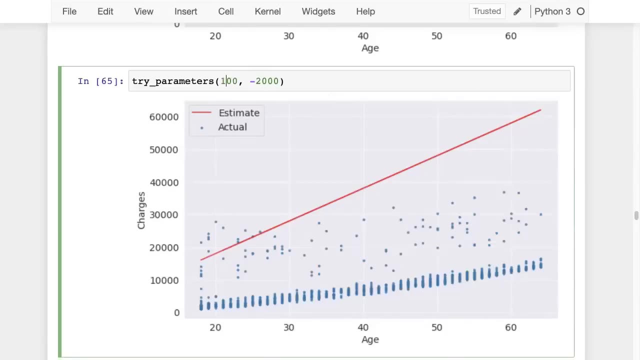 Let's say we said the way to zero, that makes the line flat. Let's say we said the way to a thousand, that makes the line really steep. Then maybe you want to go somewhere between like around 500, and that's what we want to go with. 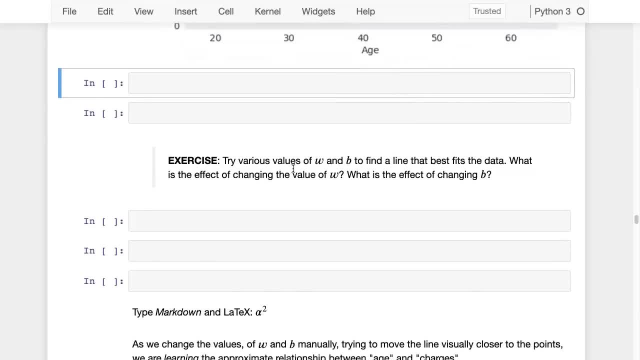 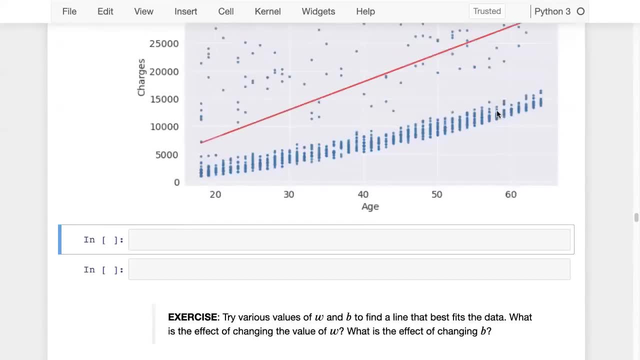 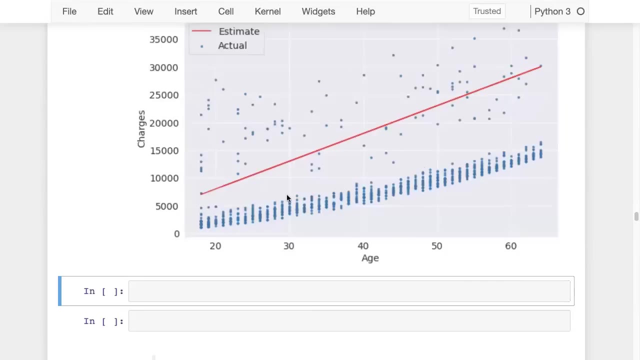 So that's how you try and fit a line. So here's an exercise for you: try various values of W and B to find a Line that best fits the data. Just try it out. spend maybe five or 10 minutes trying out various values and you will be able to get to a pretty good point by just guessing. 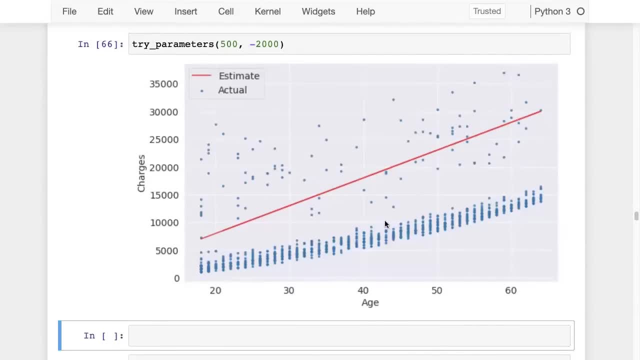 And as you saw that what you do is you look at the line and then you compare it with the points and you see if you need to move the line down. If you need to move the line down, decrease the value of B. Then if you need to increase the slope, increase W. if you need to decrease the slope, decrease W. 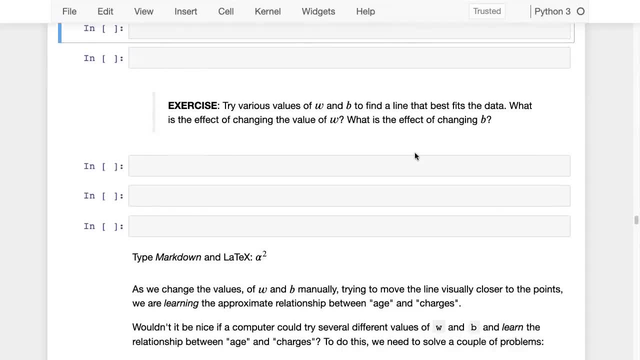 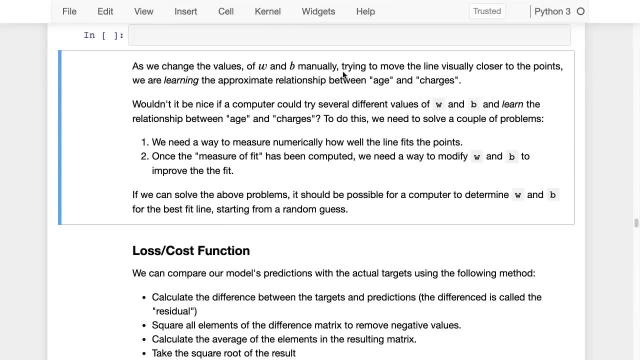 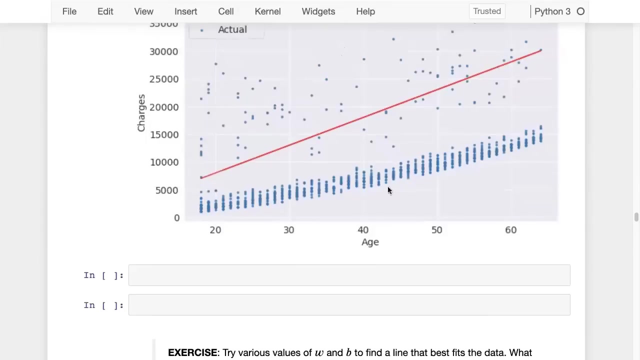 So you already have a strategy in place that you can apply each time. Now, as we change the values of W and B manually, trying to move the line visually closer to the points, we are learning the approximate relationship between age and charges. So wouldn't it be nicer if a computer could try several different values of W and B and learn the relationship between agent charges? because ultimately now, once we've established that there's going to be a linear relationship, we just need to move the line around. 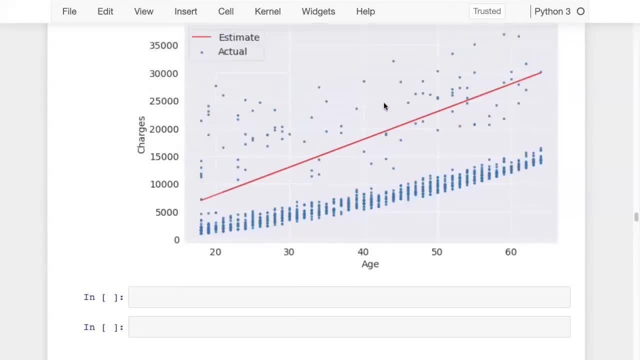 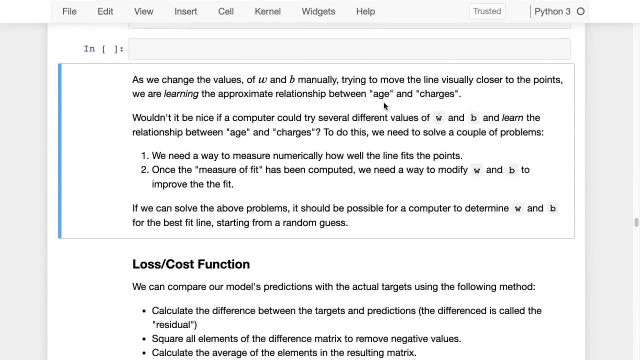 Okay, Okay, Okay, Okay, Okay Okay. Up and down, left and right, change its slope And we should be able to get to the right point. Well, to do this, we need to solve a couple of problems. 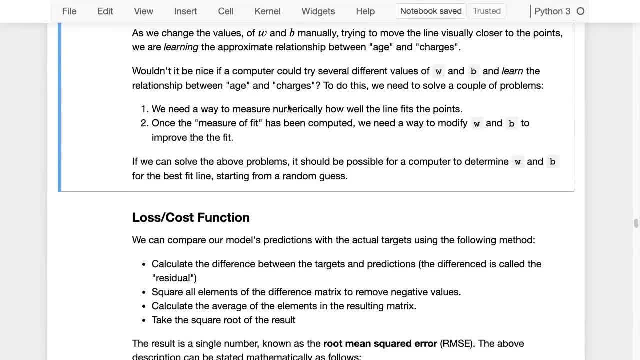 One. we have eyes and we can see that the line is far away from the points. but the computer does not have eyes, so to speak. So we need a way to measure numerically how well the line fits the points. That's the first thing. 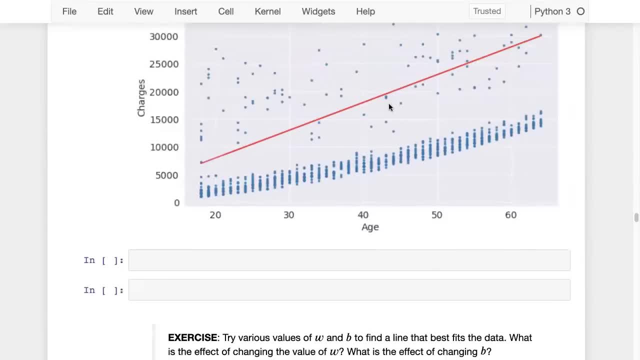 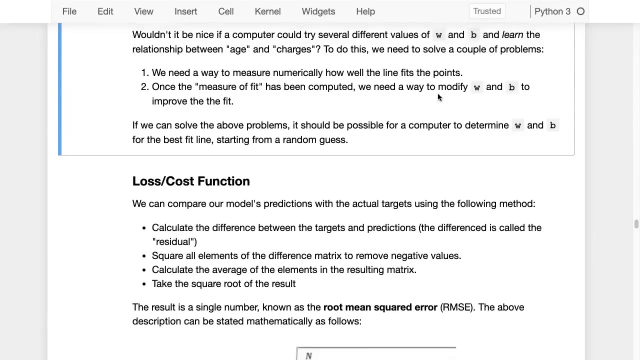 Okay. Second, we are able to guess Which way we should move W and B by looking at how far the line is from the points. But again, we are applying a lot of insight here. So once we measure the fit of the line, we need a way to modify W and B to improve the fit of the line. 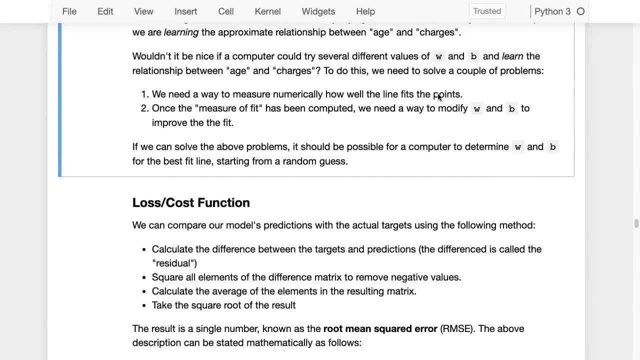 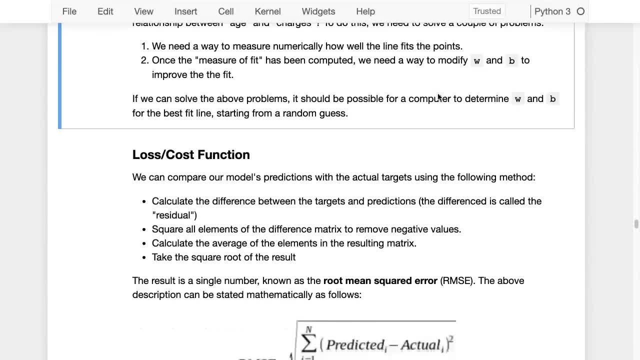 Okay. So we need a way to measure how well the line fits the points and we need a way to improve W and B once we have made a measure And we realized that this measure is bad. So if we can solve the above problems, this will be a breakthrough. 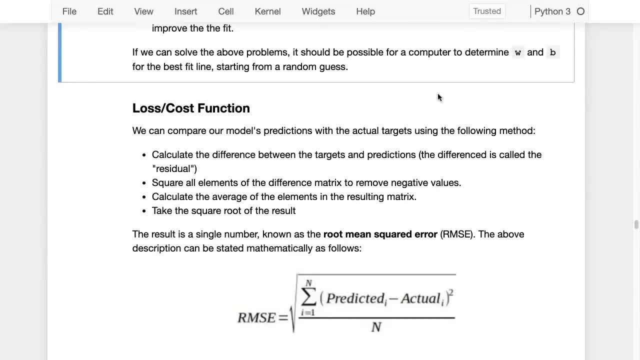 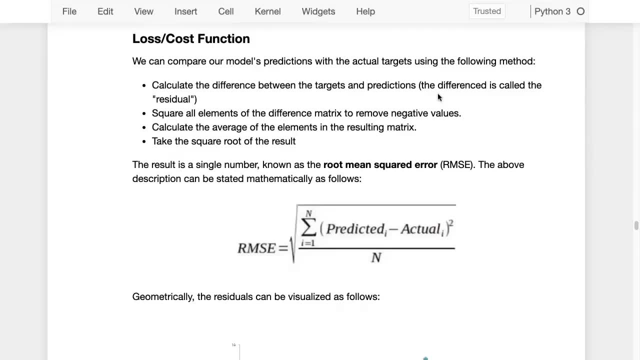 Okay, Because it should then be possible for a computer to determine W and B for the best fit line, starting from a random guess. So let's solve the first problem Now. we want to compare our models predictions with the actual targets, and this is the method that we can follow. 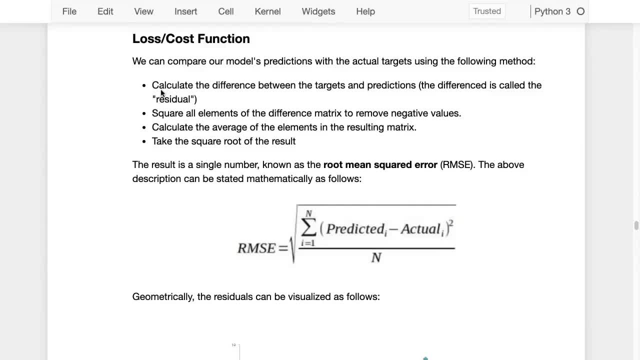 We calculate the difference between the targets, which is the actual charges from the dataset and the predictions from our model, And this difference is called the residual. So for each target you have a bunch of targets. here The targets are simply the actual charges. 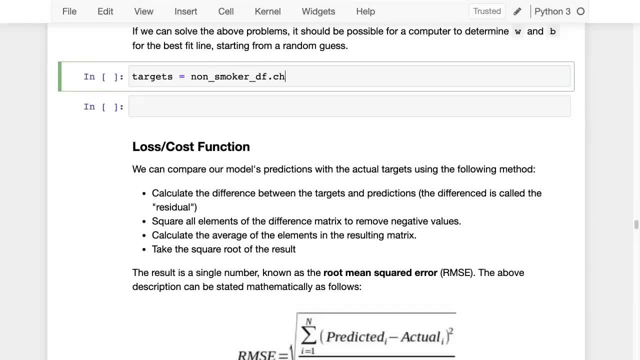 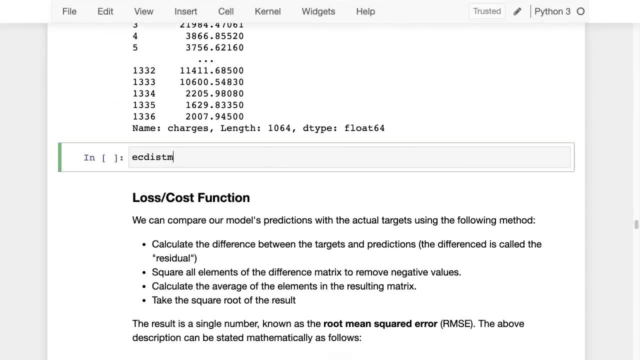 So we have non-smoker DF, not charges. These are the targets, And then you have the predictions, which is the estimated targets. This is what our model has predicted for the input data. So predictions is estimated charges. Okay, Okay. 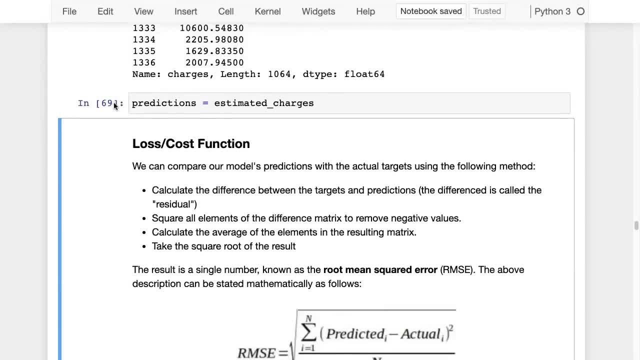 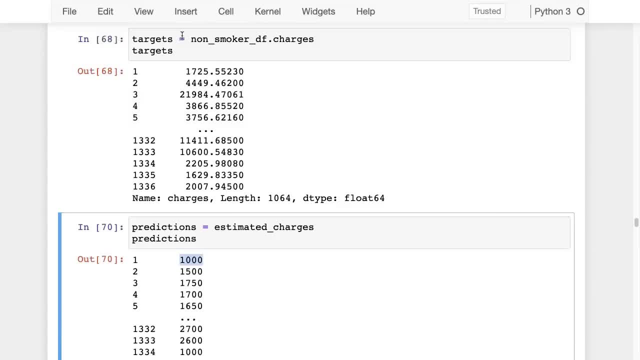 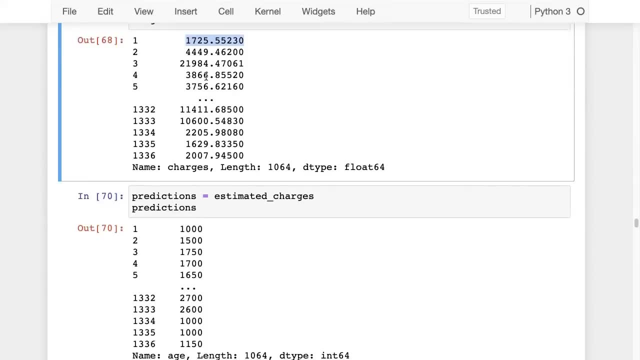 So what we do is we subtract each prediction from the corresponding target. So this is going to tell us how far away our prediction is from a target. But the problem is, some predictions may be lower than the target. Some predictions may be higher than the target. 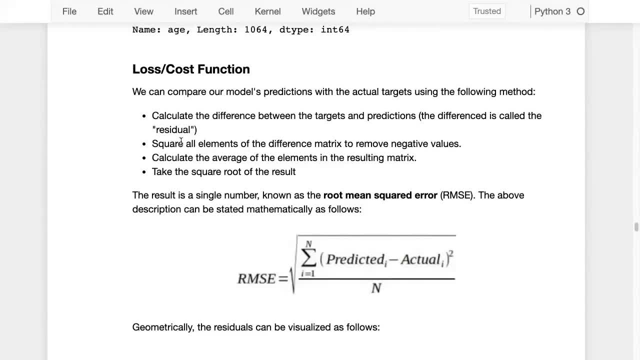 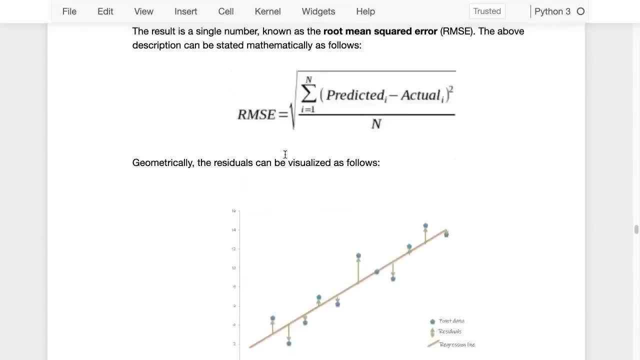 So to remove negative values, we square all the elements in the difference vector. Let me remove this matrix term here. Yeah, Okay. So we square all the elements to remove negative values. So you subtract 1000 minus one, seven, two, five, that's seven, 25.. 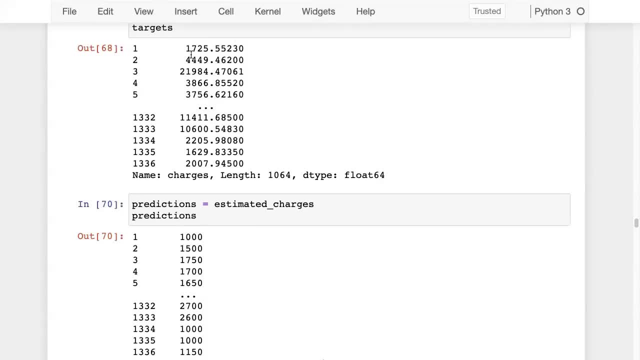 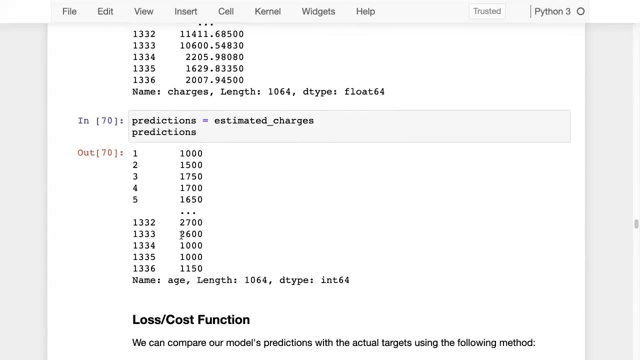 And then you square it. So 25 squared, then you do 1500 minus four. four four nine, That's again some negative value. a square it. at some points You may have positive values. Maybe you have 2,600 here and 1600 here. 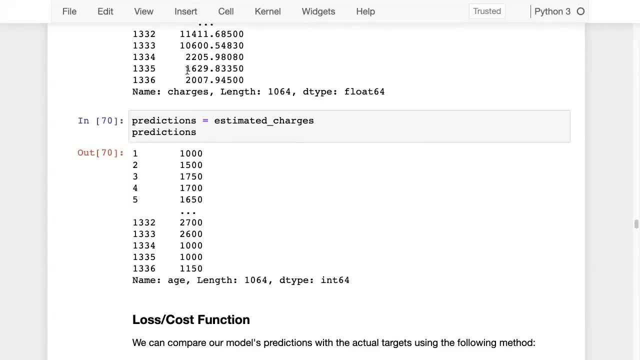 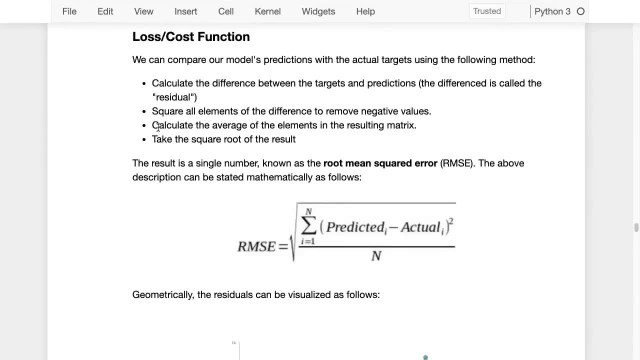 So you'll get a positive value. square it. So we take the residuals- Each difference is called a residual. Then we square all the residuals, Then we calculate the average of all those elements in the result, right? So we have all of these residuals. 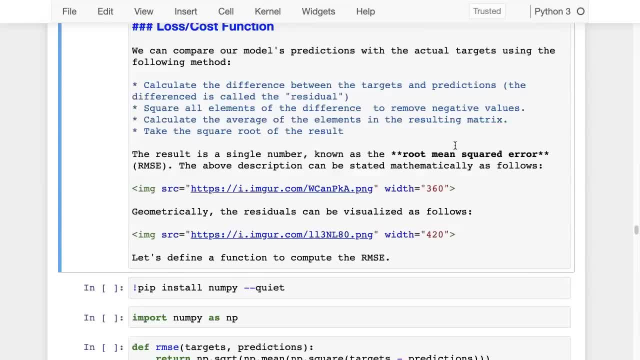 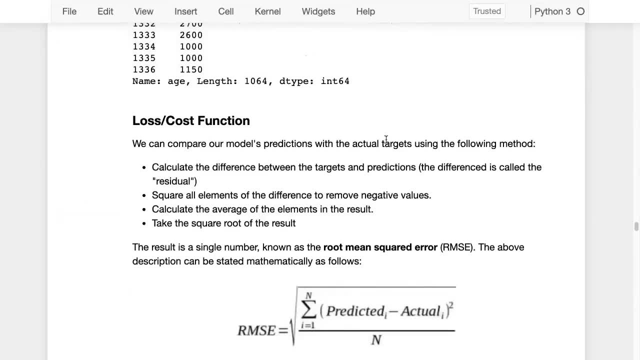 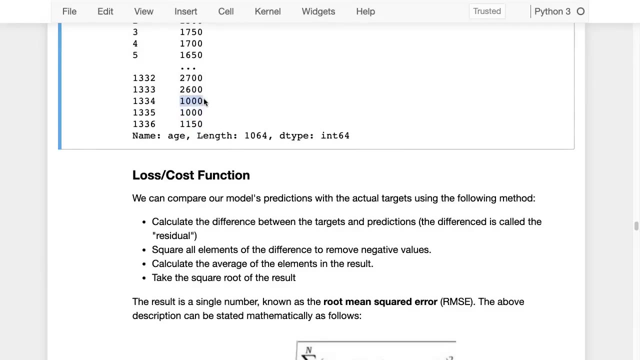 We simply add up all the squares of residuals and calculate the average. So now we have this minus the actual target squared, plus this, minus the actual target squared, plus this minus the actual target squared divided by the total number of entries We have. 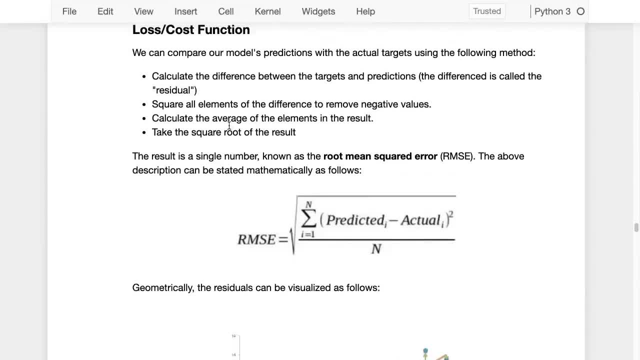 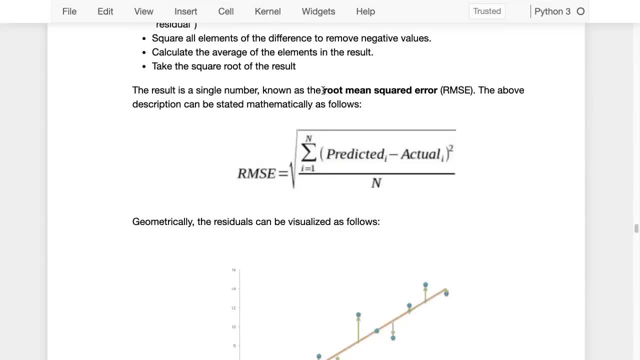 And finally, we take the square root of the result. Okay, Seems like a complicated process, but it's actually fairly straightforward. What it's giving us is called the root mean, squared error. So let's break that down. Error is simply the difference between the targets and the predictions. 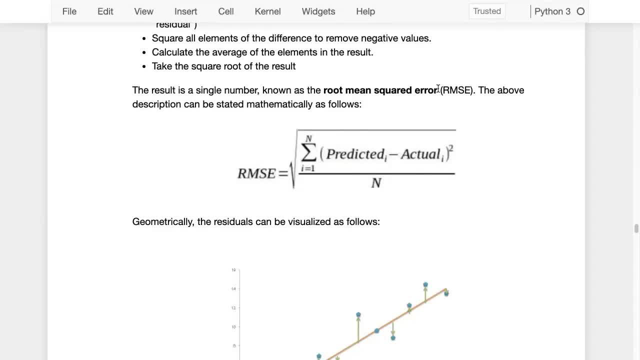 So that is the error. But of course, if you just add up errors, positives and negatives may cancel out, So that's why we squared it. So now, when we square it, all the errors become positive and then we take their average. 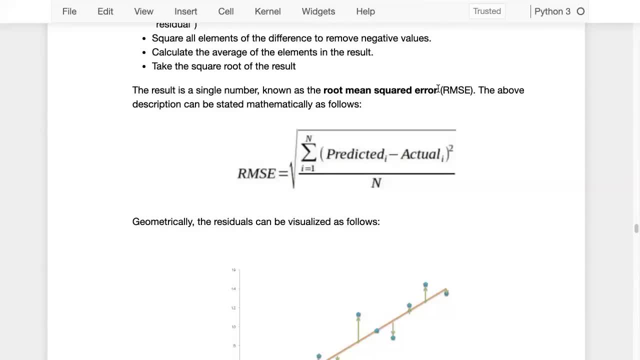 So that gives us the average squared error or mean squared error. But then we want to take the square root again, because we want to interpret the number that we get as a dollar value essentially. So now, when we took squares, we converted the difference in dollars into dollar square. 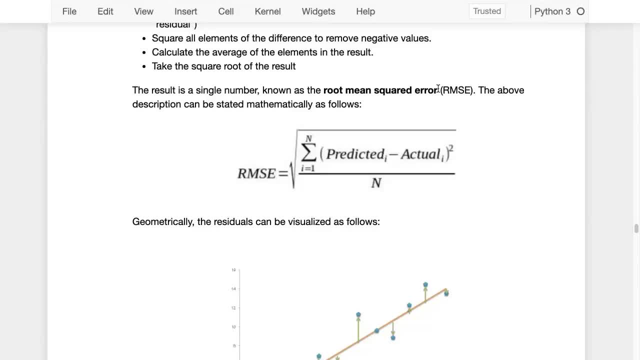 So we just took take a route again, and that just gives us a dollar value. So that's why this is called a root mean squared error, And it tells us on average how far away we are, how far away each point is from the line. 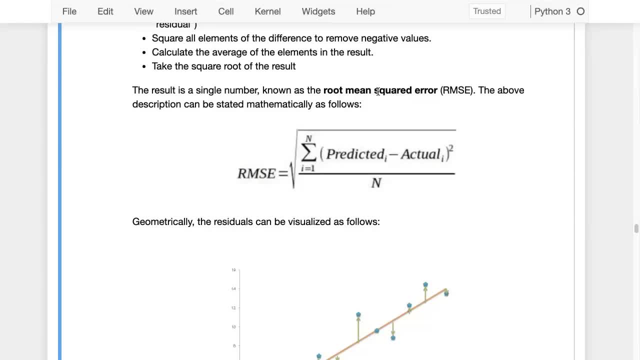 Now, this is not the only way to do it. There is also something called the root mean absolute error, where you do not take squares, You actually take the absolute value, which means you simply ignore the sign. And the difference between root means squared error and root mean absolute error is simply that outliers have a big 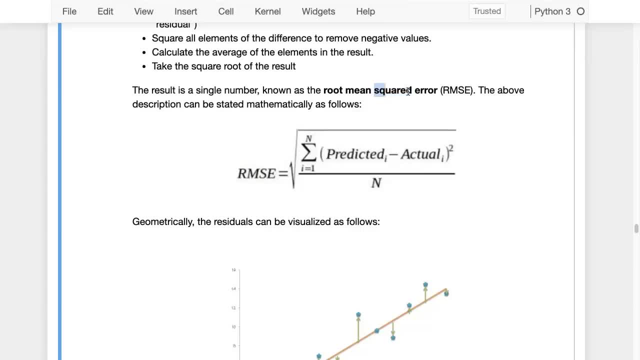 factor or outliers, contribute highly in a squared error, because the greater the error, the greater it square is going to be, So it's going to be a bigger factor in the overall error. Okay, So that's it. That's just one thing to keep in mind. but root mean squared error. make sure you understand this. 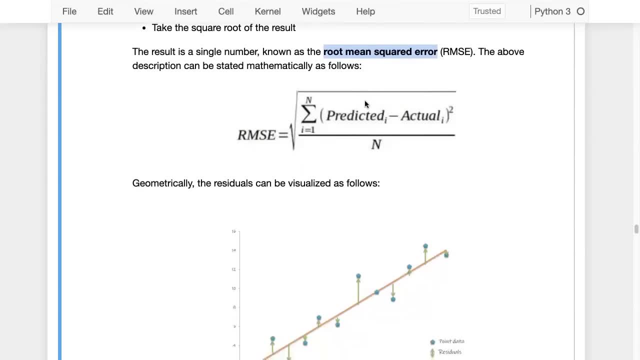 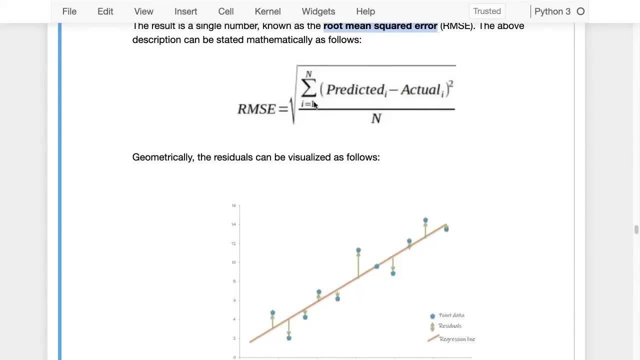 This is the average on average, how far away we are from the line right. And this is the formula, which is exactly the same thing: Prediction minus actual squared sum over all the predictions divided by N square root of that. And this is how you can visualize: root mean squared error. 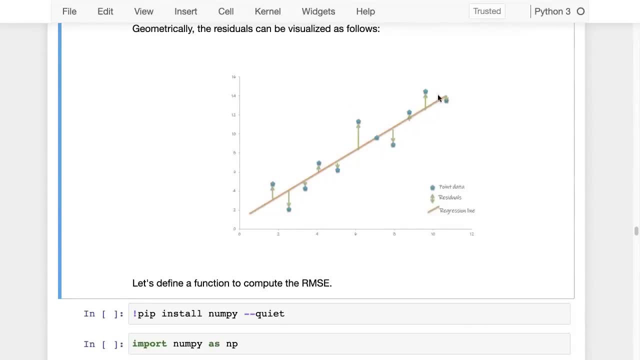 So these are the rest. So suppose this is the line, and then these are the actual target points. for each point You calculate how far away it is from the prediction, and the prediction is simply the point On the line at the same X value. 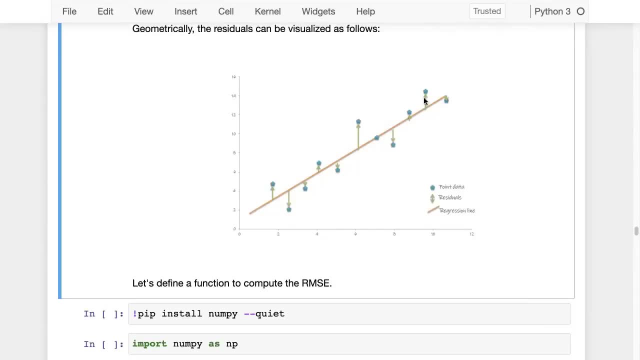 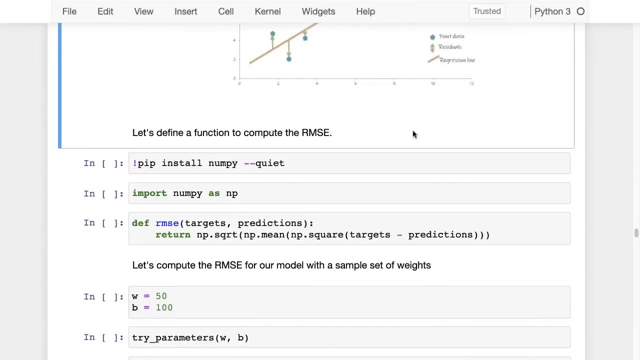 So this is a prediction. This is the actual point. you calculate the residual for that point And then you add up the squares of all the residuals, take their average and take the square root. So these are all different ways to look at the root mean squared error, but let's look at it in a way that we understand best, which is using code. 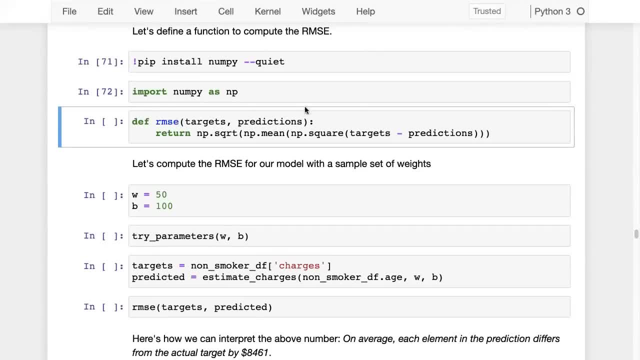 So I'm going to install the NumPy library here and import NumPy as NP, And then I'm going to define this function, RMSE, Which takes a set of targets. It takes a set of predictions. First we get target minus predictions. 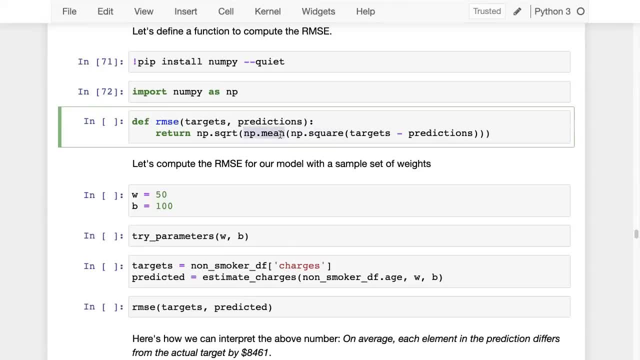 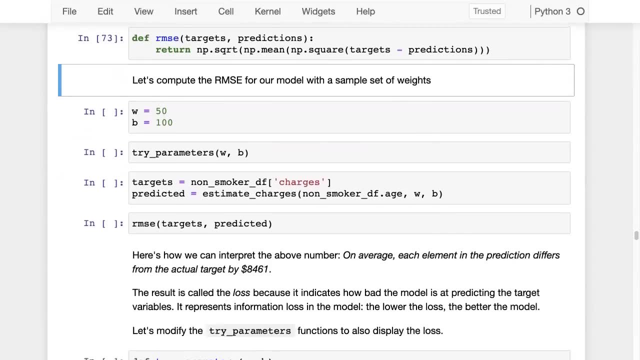 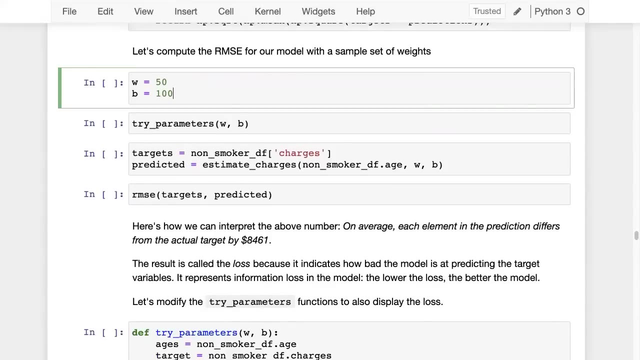 That's the error. We square it, We take the mean, and then we take the square root mean squared error. All right, So now we have a way to tell how bad our model is. So let's compute the root mean squared error for a model with a sample set of weights. 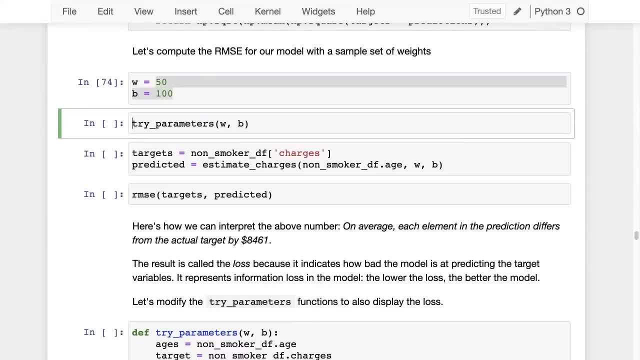 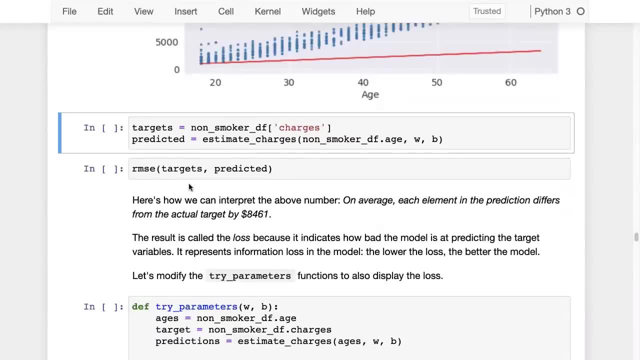 Here is the weights: 50 and a hundred. This is what we started out with, And here are the here's what that line looks like, The line made by these weights. Now let's get some predictions, So let's get. these are the targets. 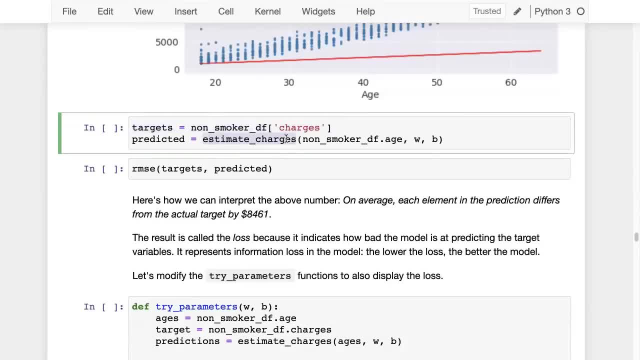 The targets are simply non-smoker DF dot charges and the predictions are simply by calling the model or putting the weights and the inputs into the model. So the age- I'm taking the list of ages, putting that into the estimate charges function, along with the weight and bias. that will give us some prediction. 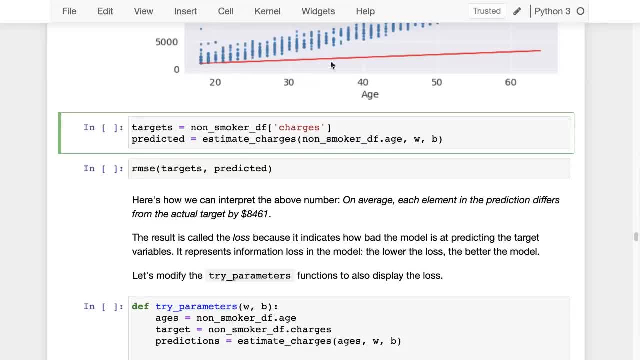 So that will give us, for each of these ages in the actual dataset, The point on the line where the point on the line is what we'll see in prediction, specifically the Y portion of the point on the line or the Y coordinate of the point on the line for that age. 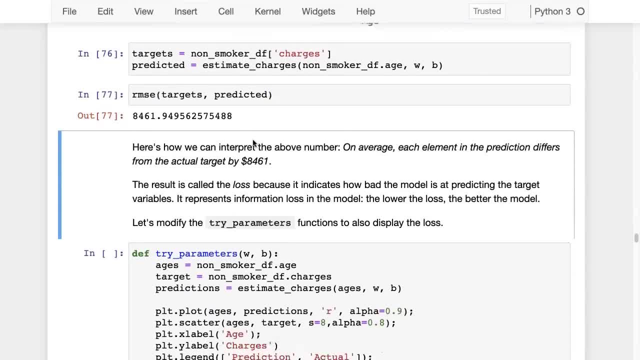 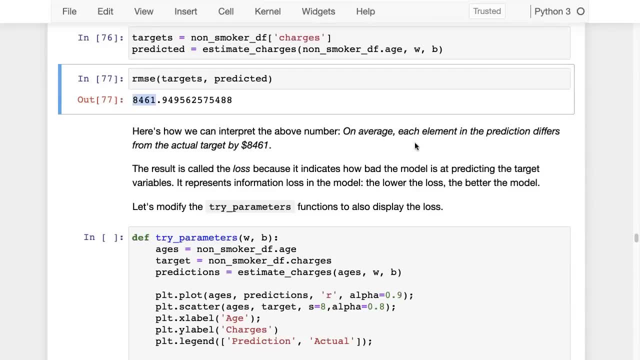 Now we can compute the root mean squared error between the targets and the predictions, And it seems like the root mean squared error is eight, four, six, one. So how do we interpret this number? Well, on average, each element in the prediction differs from the actual target by 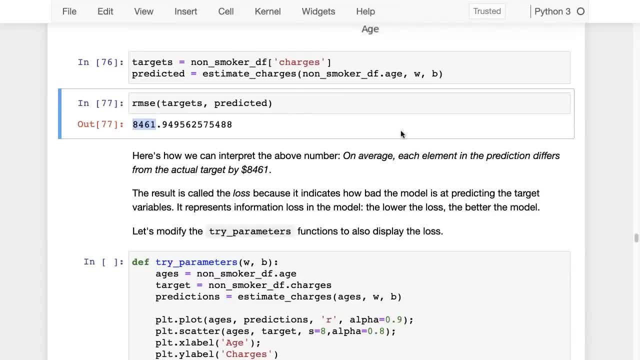 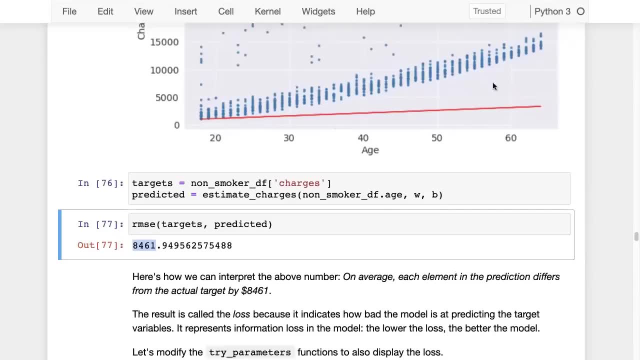 Eight, four, six, one. That's not the exact interpretation, but it's pretty close and this is how we can look at it. So is that good or is that bad? Well, visually we can tell it's bad, but even on average you can see that the values of charges go anywhere in the range of maybe 2000 to 15,000 here, right. Normally for somebody who does not have high, high medical expenses. So if you're trying to predict the value between 2000 to 15,000.. Yeah, Yeah, Yeah, Yeah, Yeah, Yeah, And you're off by 8,000.. 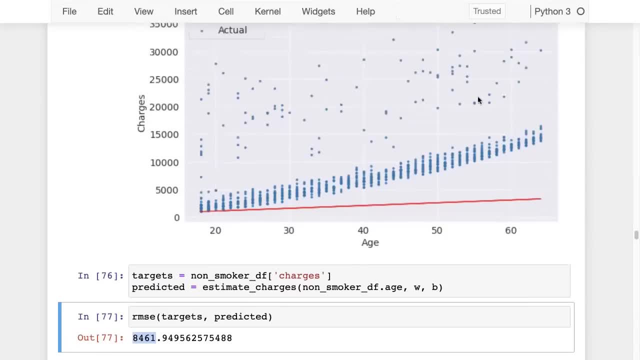 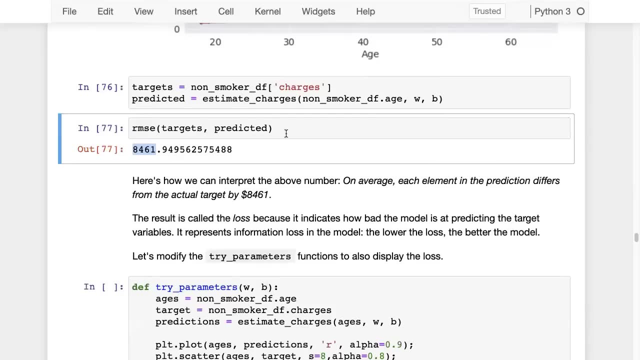 I think that would be pretty bad, even considering that you have some outliers. because these outliers are smaller number, I think 8,000 would be pretty bad. Maybe I would be willing to live with an error of maybe four or 5,000 at most, but 8,000 is just all over the place. 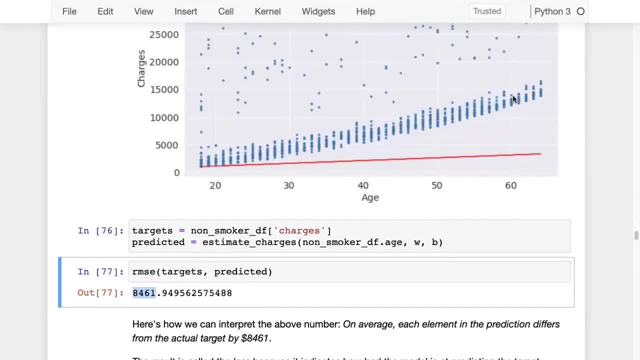 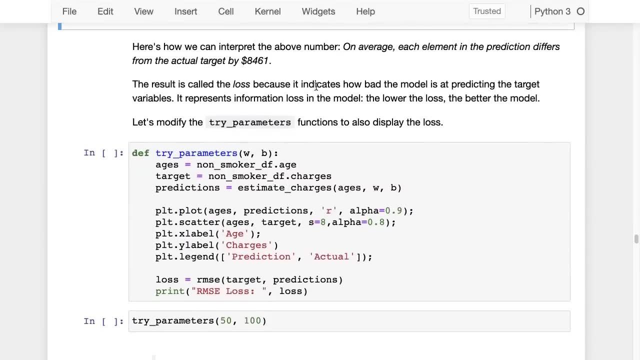 And you can tell the same thing by this line as well. This is too far away from the actual data, So that's how you Interpret the root mean squared error, And this error is also called a loss because it indicates how bad the model is at predicting the target. 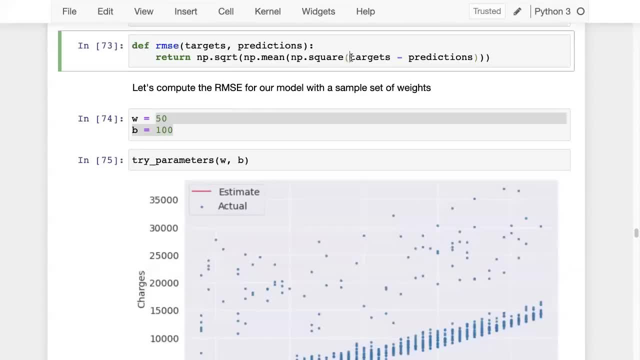 Remember the difference between the two things, which is targets and predictions, will be higher, And then the squares will be even higher and the average will be higher, And so the square root will be higher If the targets are very far away from the predictions. that means if your model is really bad, then the root mean squared error is going to be very high. 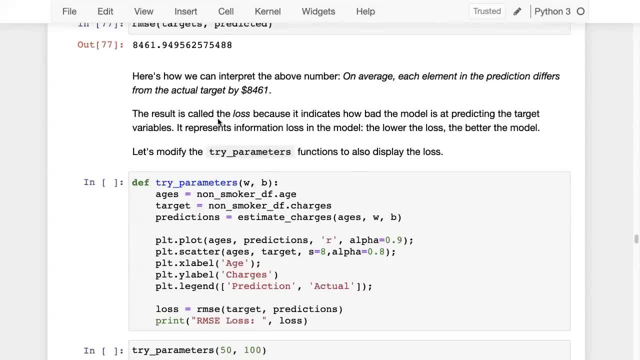 That's why it's called a loss, because it Represents the information loss in the model. Remember, we are not capturing the actual relationship, We are simply modeling the relationship. and all models are wrong. It's just that some are useful. How do we figure out which models are useful? by looking at the loss. the lower the loss, the better the model right. 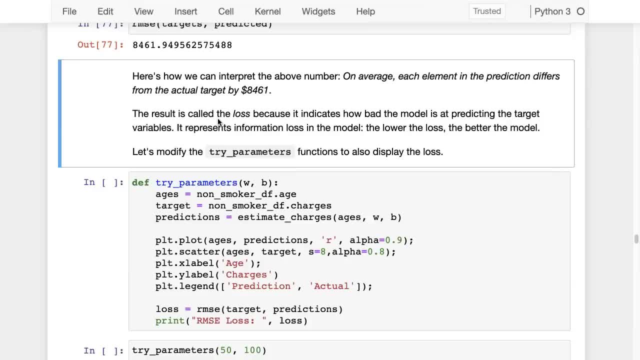 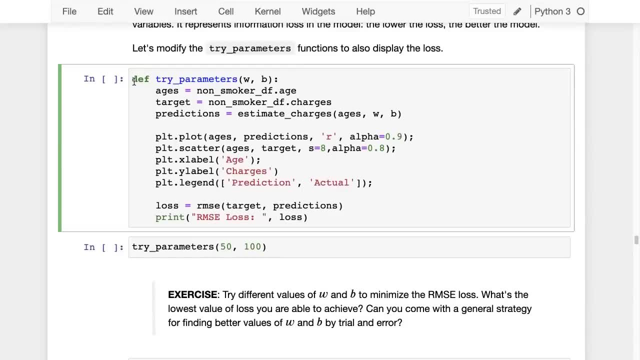 The higher the loss, the more noisy, the more useless the model becomes. So let's do one thing: before we train a computer to figure out the lowest loss, let's try and do it manually. So I have the stripe parameters function here, which takes a set of weights and biases and then make some predictions using our estimate charges. 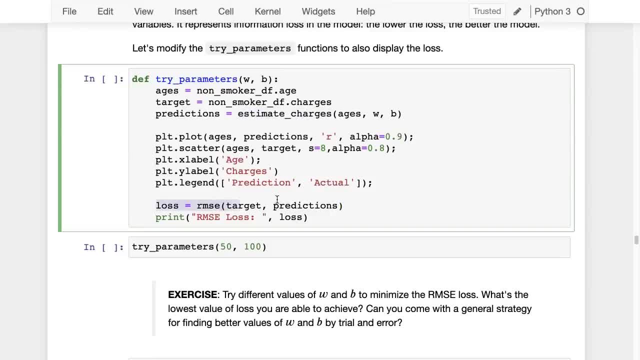 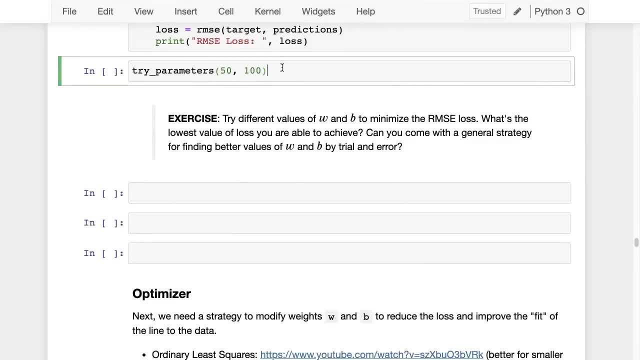 function and plots a graph at the end. I have also computed the loss for the predictions made for these weights and biases and I've printed the loss. So here's what that looks like. This is the graph. This is the same line we have and the RMSE loss of eight, four six one. 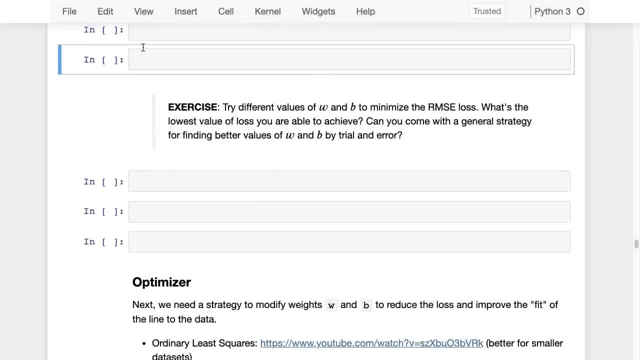 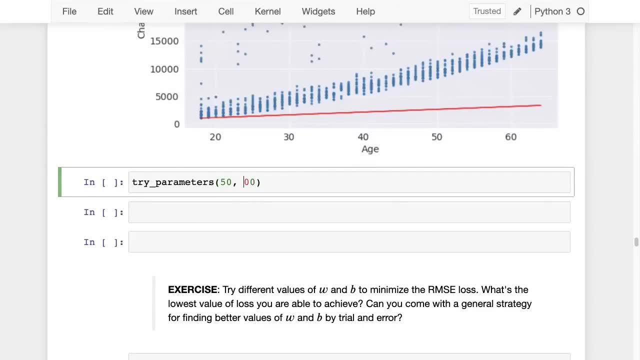 Now let's take up the challenge to try and Fix The RMSE loss. Let's try and make it as low as possible. So one thing that's clear is that I should be increasing the slope of the line. Let me make this 300.. 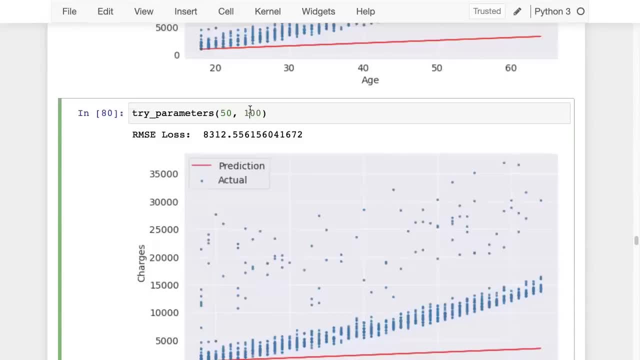 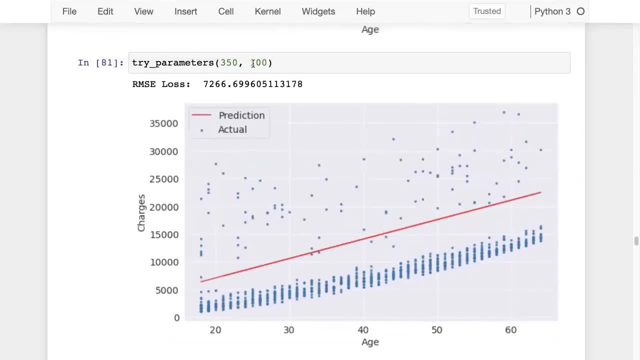 Okay, That did not do much, maybe. Okay, This is not the slope, This is the slope. Let me make this three 50.. All right, That pushed it up by quite a bit. Maybe let me push it down a bit. 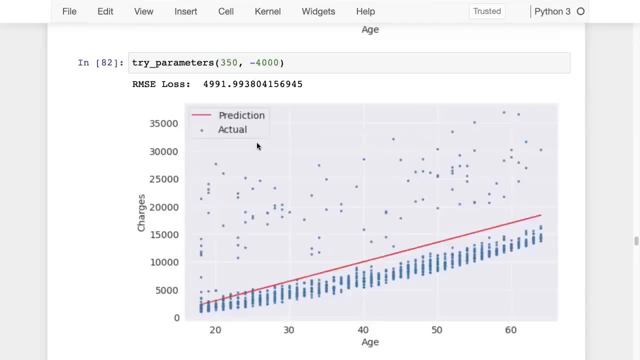 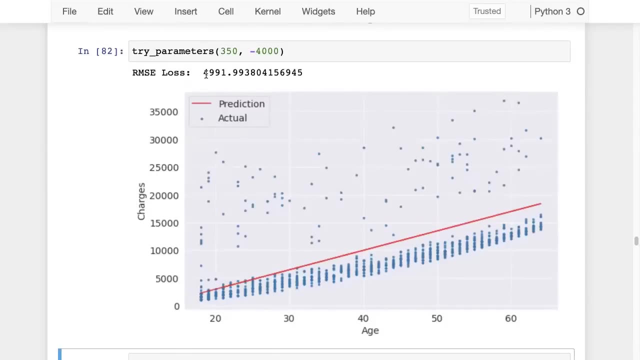 Let me push it down by 4,000.. Yup, That's getting pretty close And I've already arrived at RMSE loss of four, nine, nine one. So that's what you want to do And you can experiment here. 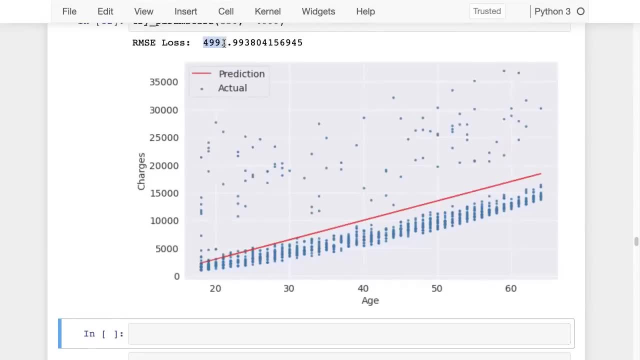 You can try and get it to as low a value as possible And now you have a very clear target. You don't have to figure it out visually, but you can see. as the RMSE loss gets closer and gets lower, You will see that the line gets closer and closer to the points. 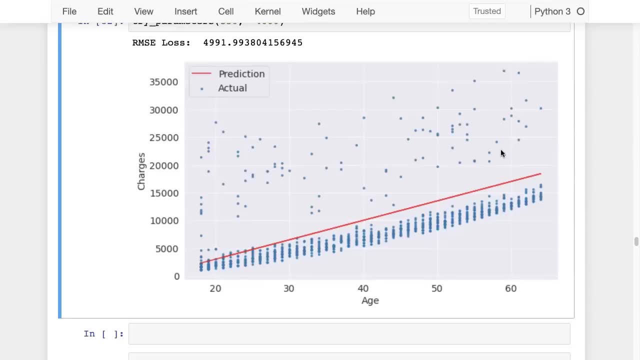 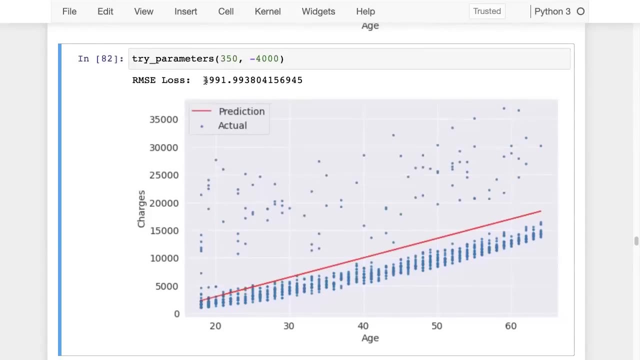 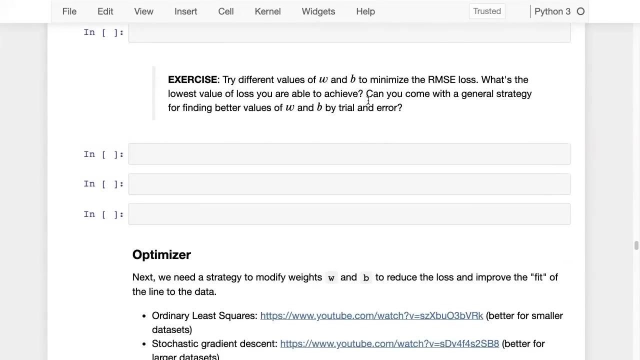 It will not lie exactly in between the points because we have all these outliers that we need to account for, Okay, But it should lie somewhere along this region. So three, 50 and minus 4,000 is my best guess. Let's see if you can beat that and try and come up with a general strategy for better, for finding better values of W and B just by looking at the loss, not necessarily by looking at the graph, but just by looking at the loss. 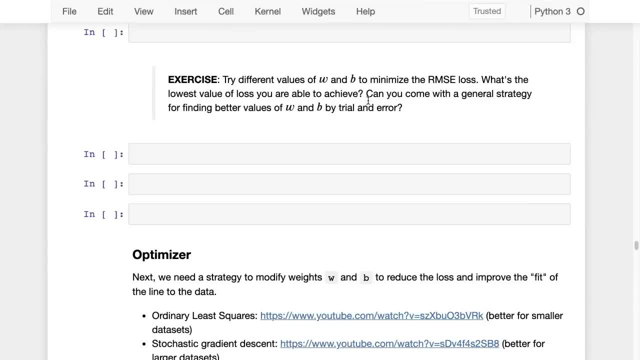 Here's one strategy that I will suggest: if you have a weight, if you have a certain W and a certain B, try slightly increasing W. If that reduces the loss, then you can increase W by a large amount. If that does not reduce the loss, right. 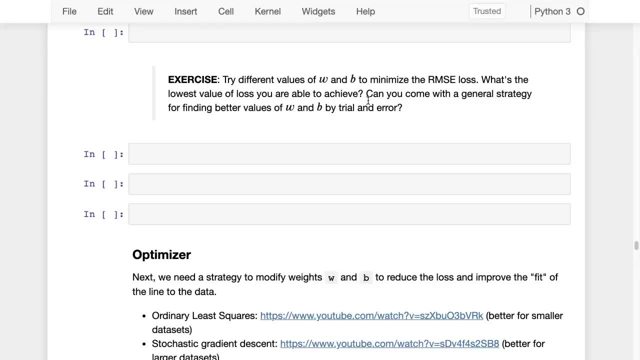 Slightly decreasing W. if that reduces the loss, then maybe you can reduce W by a significant amount. If that does not help, try the same with B, or maybe try the same with W and B in parallel. Okay, And this strategy of just trying a small change and seeing whether it leads to an increase or decrease and then taking a larger step in that direction, which is 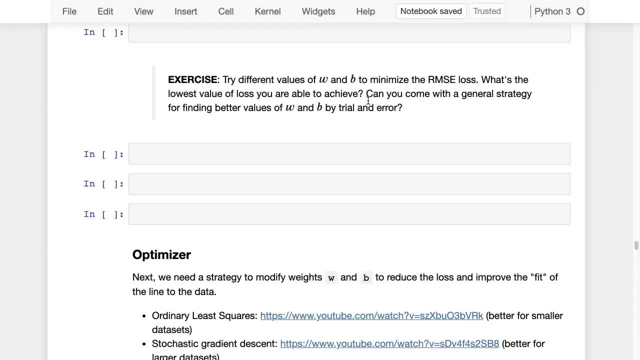 Sort of you know. assume that you're in a dark room and you have to figure out which way goes down, right If it's an uneven surface that you're on. So you put one foot and you realize, okay, this is higher ground. and you put one another foot and you realize, okay, that is lower ground. 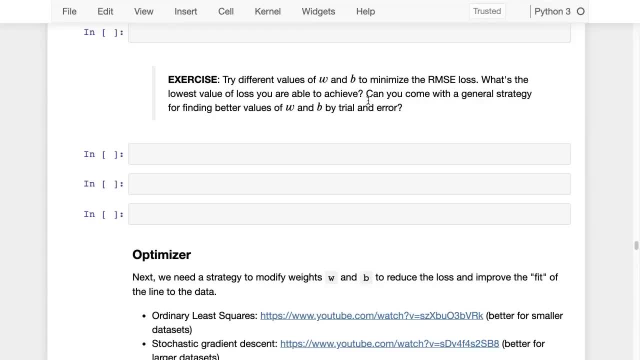 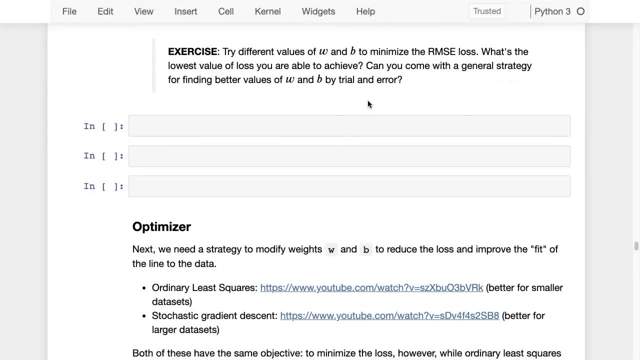 If you want to go downhill, then you take a couple of steps, maybe along the lower ground, and then you repeat the process. So the strategy is called the gradient descent strategy and it can be implemented mathematically using derivatives. but that's what we want to come up with. 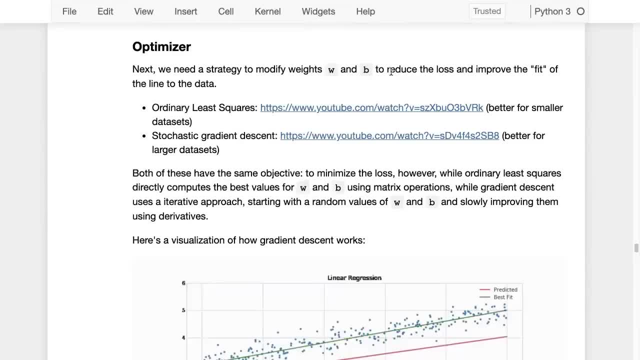 Right. So we need a strategy to modify the weights and the BI and the biases, which is the parameters of our model, to reduce the model, to reduce the loss and improve the fit of the line to the data. And there are a couple of strategies that are used to do this. one is called the ordinary least squares method. 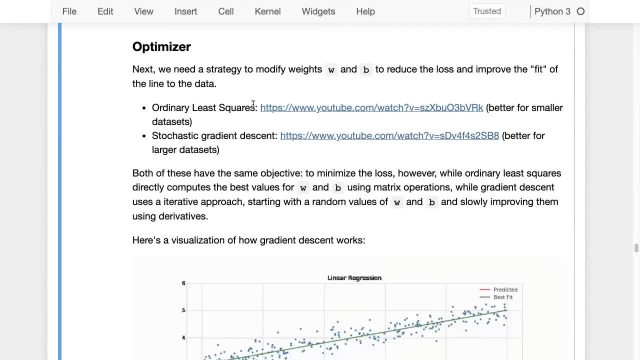 And the way it works is using some matrix operations and some matrix inversions, It directly arrives at the best value of W and B. So it uses a combination of calculus, Okay Linear algebra, to directly give you the values of W and B. it works well for small data sets, like data sets with a few thousand rows of data, but for larger data sets it is very inefficient. 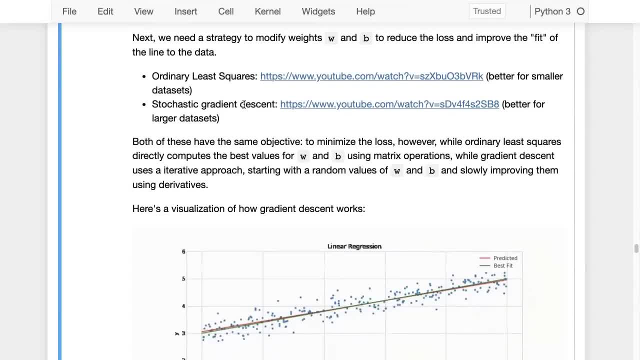 And sometimes it takes up a lot of memory. So for that you have this another technique called the stochastic gradient descent techniques, which is what I just talked about, which is, imagine like you're on a hill and it's dark and you want to figure out how to go down. 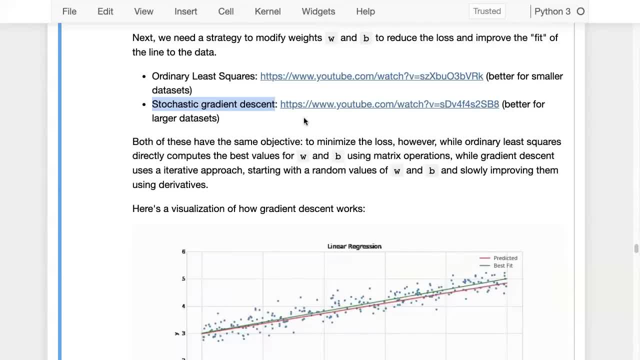 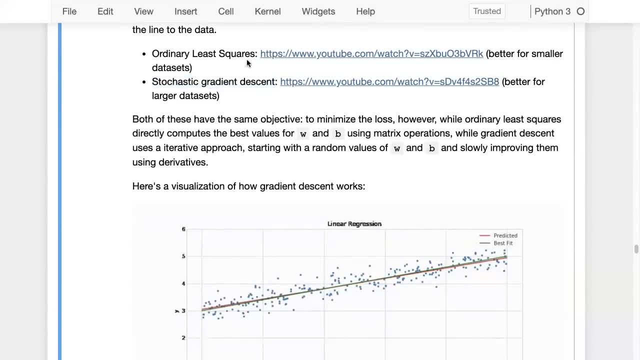 You just take steps in each direction, figure out which direction Go- It goes down- and then take a few steps in that direction and then repeat. right, So that's called stochastic gradient descent. You can check out these videos for some explanation of how these work. 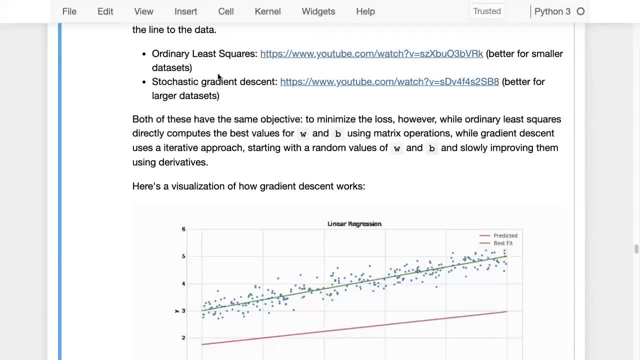 Some mathematical explanation in general. we are not going to look at it in a lot of detail because you will never have to implement these. You will have to. just it helps to understand them. but in general you won't and you can't really implement these. but you will mostly have to depend on the libraries to do this and the more important skill for you is to know. 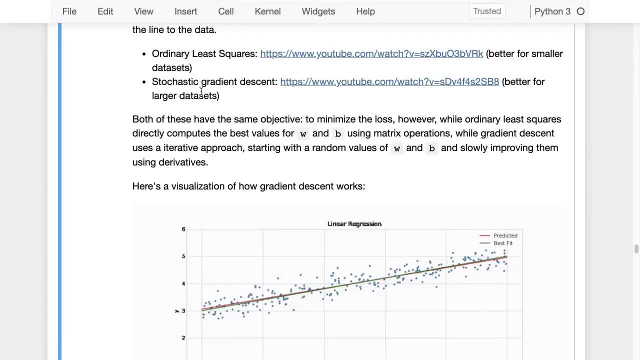 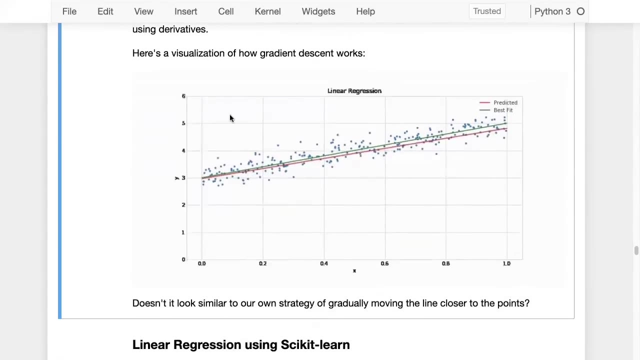 How to use these rather than to understand the mathematical representation. Okay, But yeah, ordinarily three squares works well for small data sets, uses some direct matrix computations. gradient descent works well for larger data sets and uses an iterative approach. So here's a visualization of how gradient descent works. 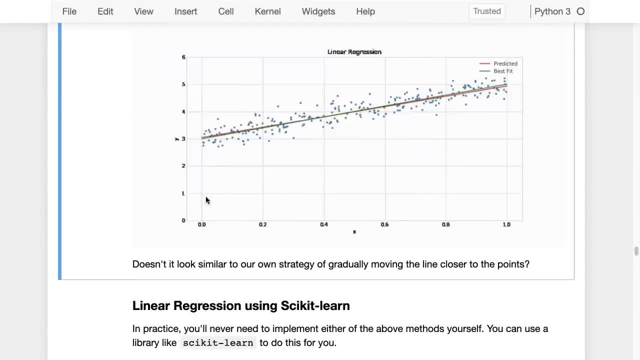 It starts out with a flat line. It's going to show up just now in a second. Okay, Let's give that a second. Yeah, it starts out with a flat line and then slowly improves both the weight. So you can see now it is improving the bias so far, but once it gets close enough it's going to start turning the line. 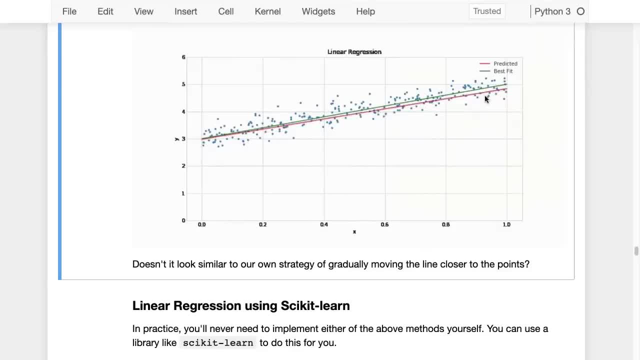 So it's going to start changing the line. So it computes the loss, It figures out whether it should increase or decrease the weight, It figures out whether it should increase or decrease the bias or the intercept. And that's how it keeps changing the line, step by step. 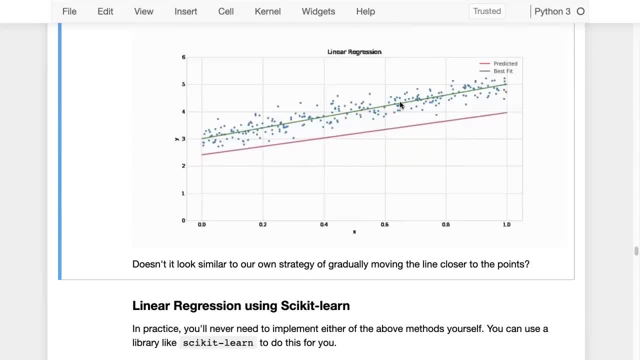 And then it gets to the very close to the best fit line and it works Really well for large data sets where you have millions or tens of millions of data points. So you will be applying linear regression to some really large data sets and that's where you'll get to see gradient descent in action. 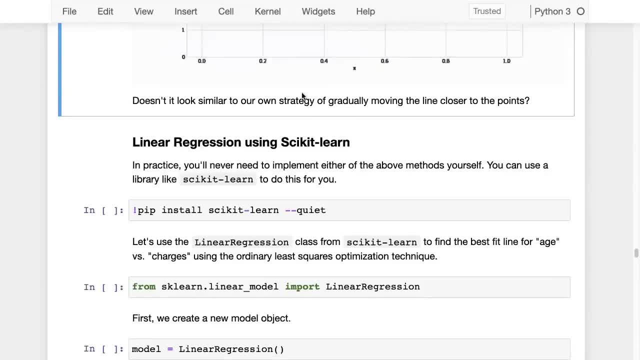 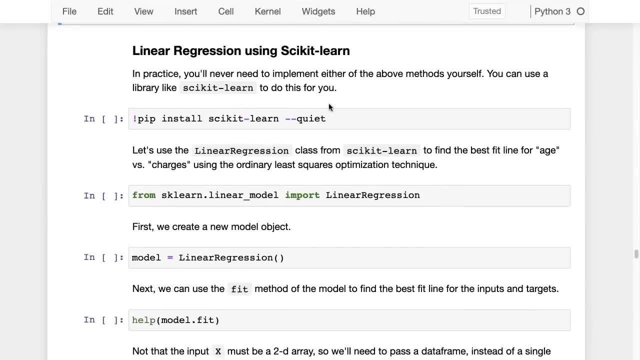 Okay, And it is actually quite similar to our own strategy of just gradually moving the line closer to the points. So that's what we are going to do now. in practice, you will never have to implement either of these methods yourself. You can use a library like psychic loan. 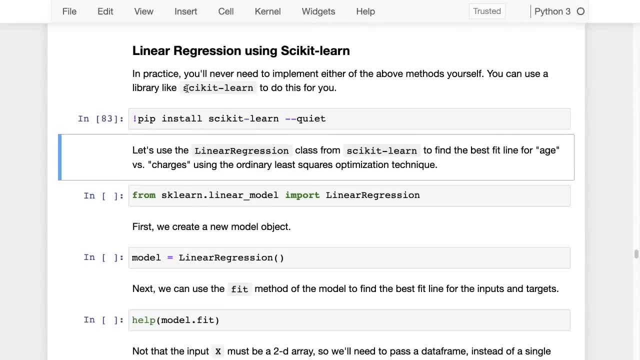 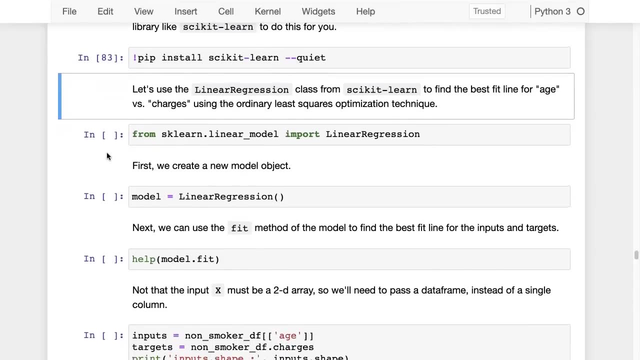 To do this for you. So I'm going to install this library, psychic loan. psychic loan contains functions, modules for doing machine learning with Python. It's one of the most most used libraries in the world for machine learning, And we are going to start out by using the simplest function that it offers, which is the linear regression class. 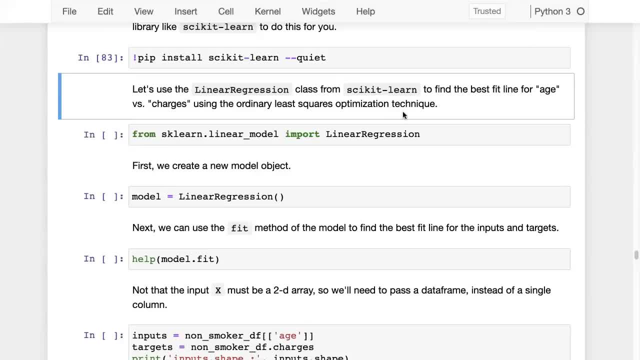 So let's use the linear regression class from psychic loan to find the best fit line for age versus charges. Okay, So let's find the best fit line for age versus charges using psychic loan. So I'm going to install pip, install psychic loan. 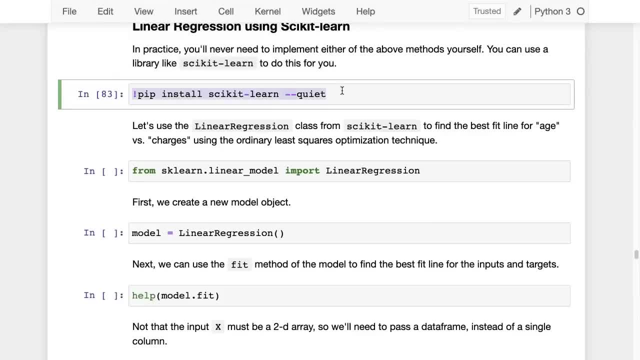 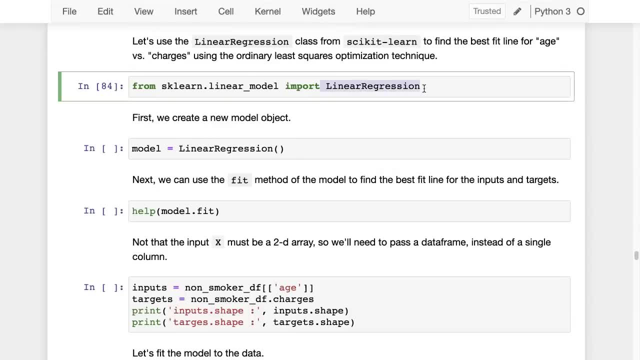 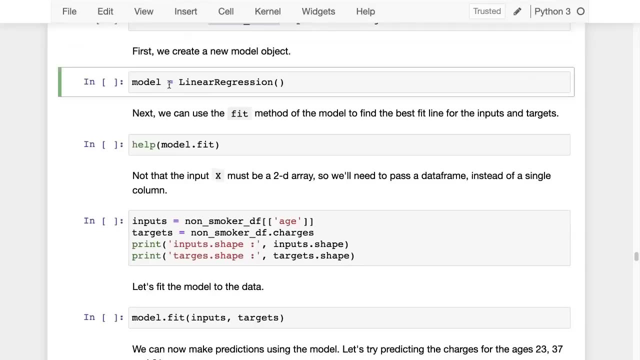 All right, And then I'm going to import from psychic loan the linear regression model, the linear regression class. Haven't done anything so far. It's in the linear model section. Then we need to create a new model object. So we create a new model equals linear regression. 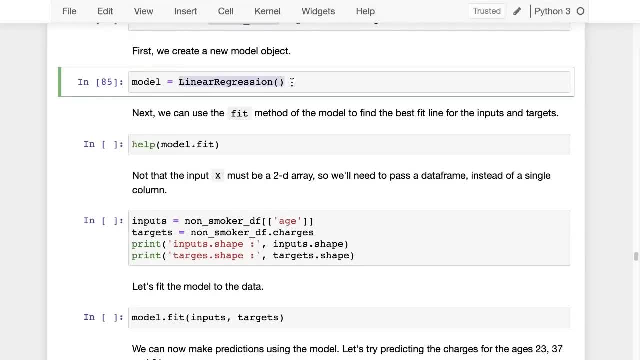 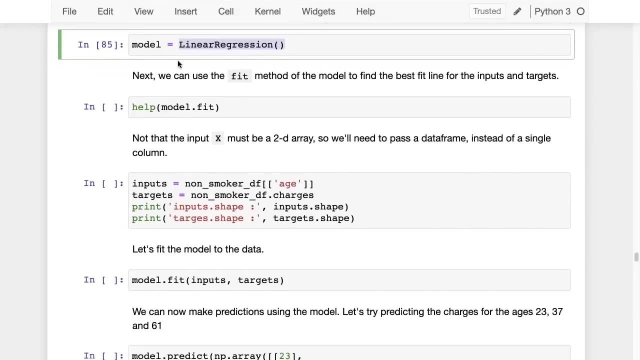 And then we need to create a new model object. So we create a new model equals linear regression. Next, here's what happens. You call that every model in psychic loan has a fit method. And let's look at the help for the fit method. 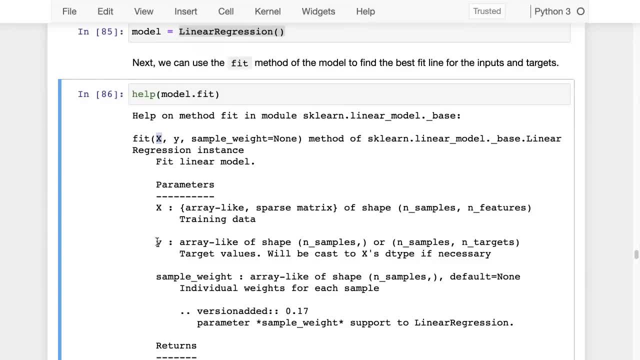 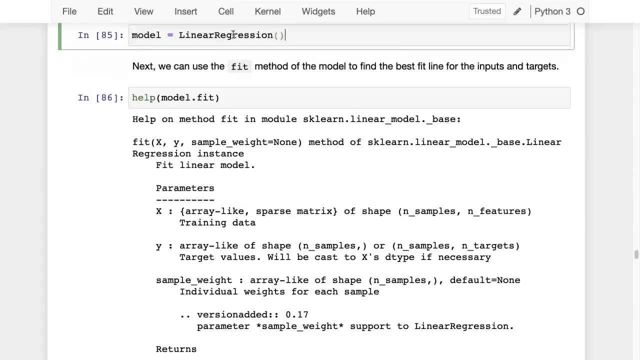 So fit method. take some parameters and take some targets and it fits a line. In the case of linear regression, it fits the line between those parameters and targets. Okay, So that's what we're going to do. next, We are going to fit the model to the data. 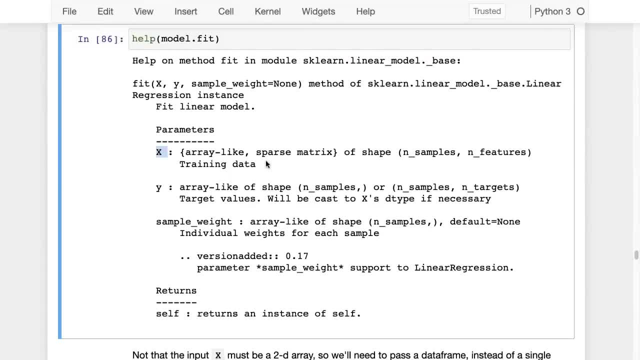 Model dot fit takes an X, which is the inputs, And this should be of the shape. number of samples, which means number of data points. We have comma number of features And in this case we just have one feature, but important thing is that this should be a two-dimensional matrix or numpy array. 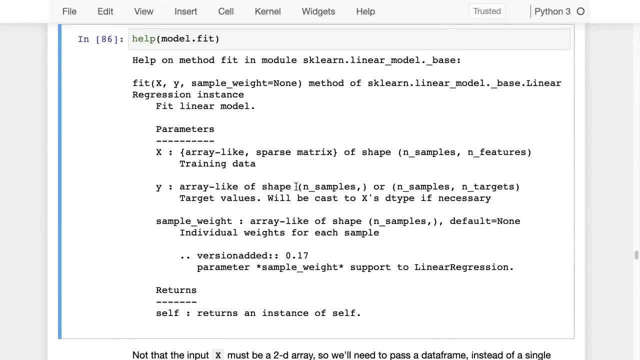 Then you have this Y, which should be array like. so it should either be a one-dimensional array which is simply, for each sample, What is the target value, Or, if you can even predict multiple targets, let's say you want to predict medical. 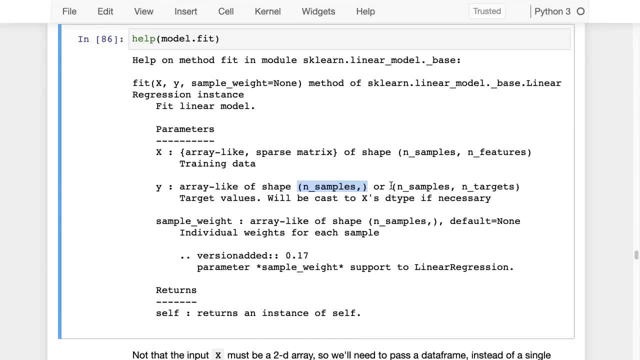 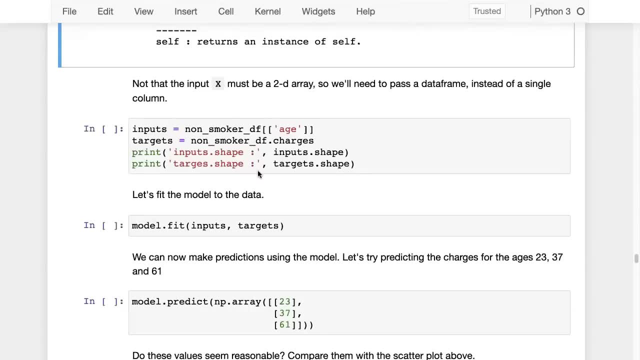 Charges. You want to predict travel charges, You want to predict some other charges, So you can have multiple targets as well. In our case, we have only one. Okay, So let's now create some inputs and let's create some targets and let's put them into model dot fit. 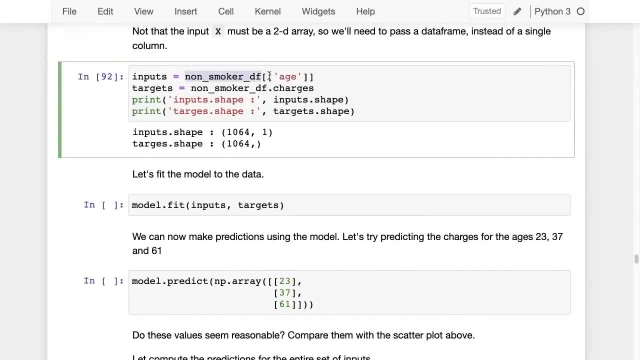 So here's what I'm going to do: from non-smoker DF, I'm going to pick age, but I don't want to just pick age. I don't just want to do this, because this is going to give me a series, and this is. this just has one dimension. 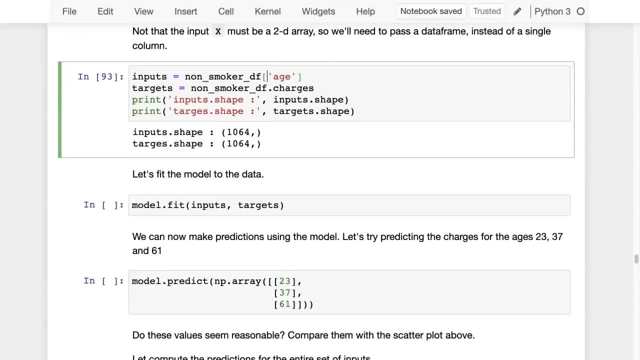 Remember, model dot fit requires two dimensions. So I'm just- I'm going to give it a list of columns that I want to pick, And in the list I just want to put the single column age. Okay, So it's a subtle difference here that we want. 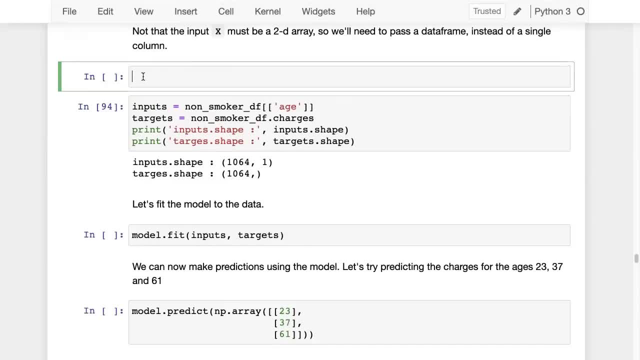 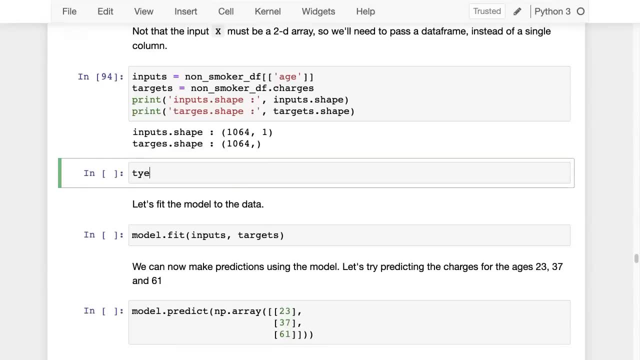 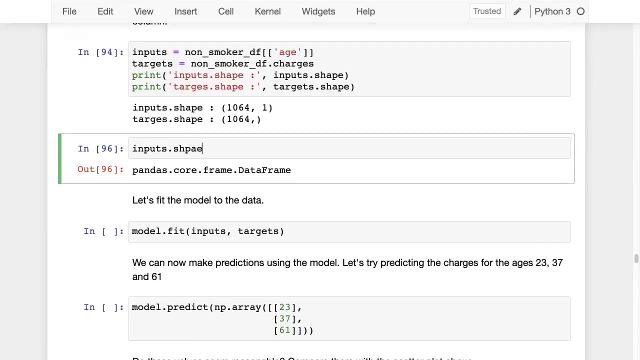 We don't want a series, We want a data frame. And if you check inputs here, inputs is a data frame, not a series, and you can check type of inputs. Type of inputs is data frame and inputs has the shape Yeah. 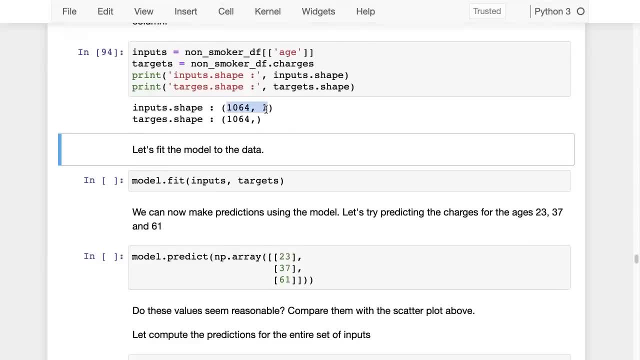 Inputs has a shape, one, zero, six, four comma one, Okay. So it needs to be a two dimensional answer, Very important. And the targets can just be an area. So the targets are simply the charges, So non-smoker, DF dot charges, and then we check the shape of inputs and we check the shape of targets. 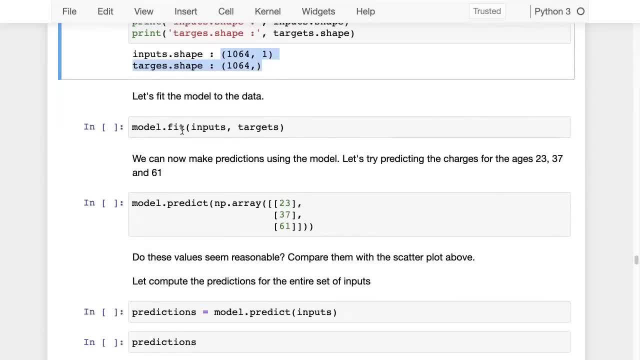 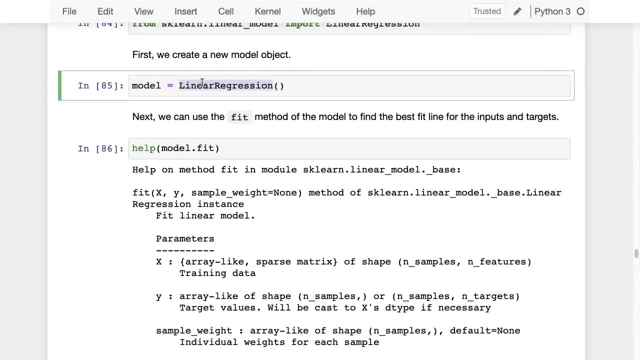 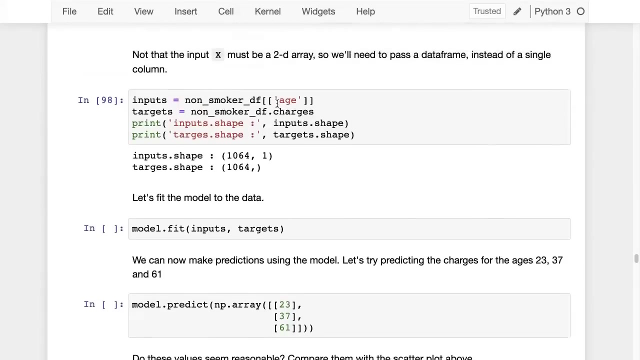 You have the expected shapes. So now this is everything That we've been building towards. This is the one line that does everything that we need to do. When we said model equals linear regression, we already mentioned to scikit-learn that we want to assume a linear relationship between our inputs and our targets, which means we want to. we want our targets, which is charges, to be some weight w, to be some weight w multiplied with the age, which is the input. 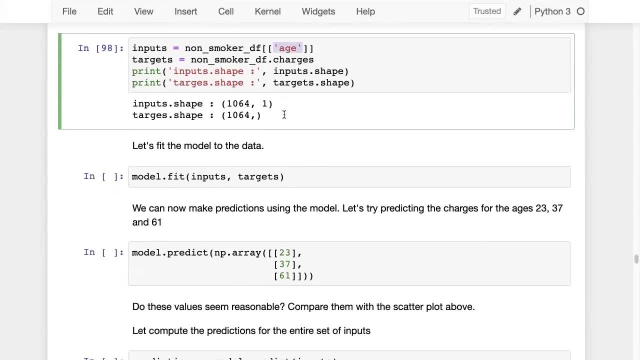 Plus Some number B. So now we're telling scikit-learn that, Hey, these are some inputs for you And these are the targets for those inputs means these are some ages and these are the charges for these ages. Can you please calculate the loss? 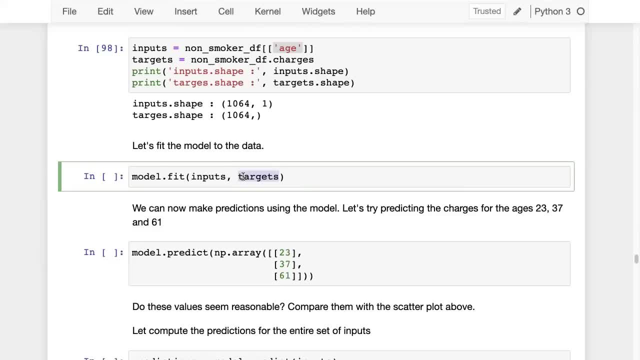 So maybe first guess some random w and B and get the predictions, compare the predictions with the targets, see how bad your predictions are, and then use a gradient descent algorithm Or Use some other optimization strategy to improve your the values of w and B and keep improving, keep improving, keep improving until you cannot improve anymore. 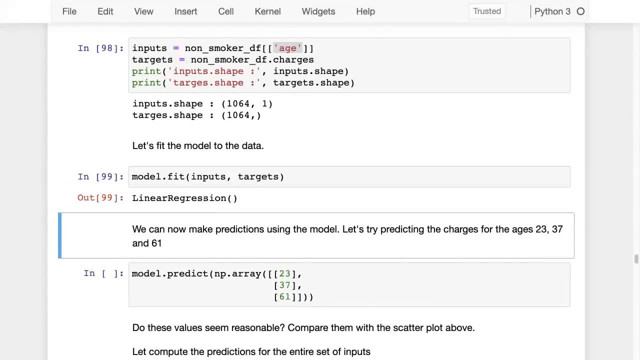 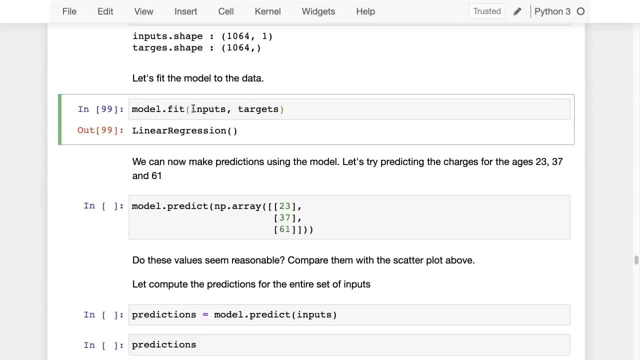 And then give me the final result. So that's what happens when you call model dot fit. So when you say model dot fit, now inside model a line has been fitted which means a w and a B have been found, which make the loss- the mean squared or root mean squared loss- the lowest possible. 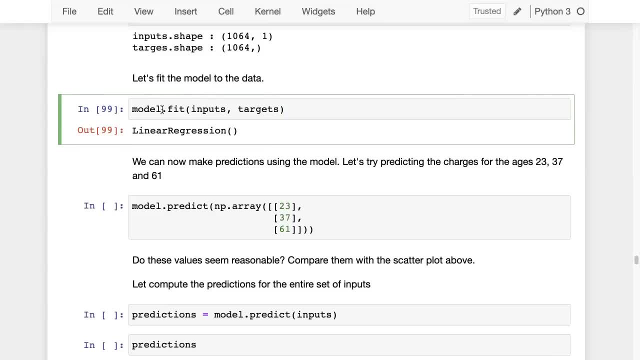 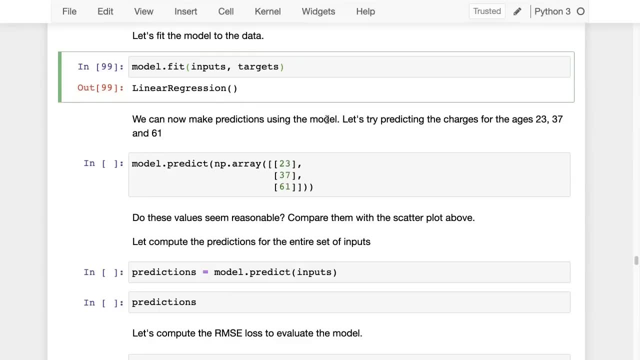 So again, the losses. the loss is also coded inside the model. We don't need to worry about that either. but here's now what we can use it for. We can now make predictions using the model. So now we have a model. 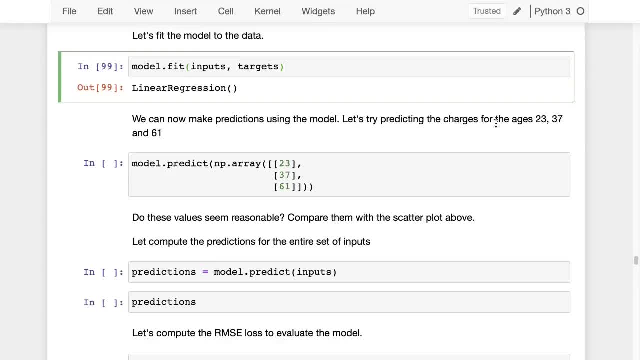 We have fitted our model. Let us try predicting the charges for the ages 23,, 37 and 61. So we say model dot predict. and then we give it this two dimensional area. So in this two dimensional area we have a bunch of rows and in each row we have just one column. 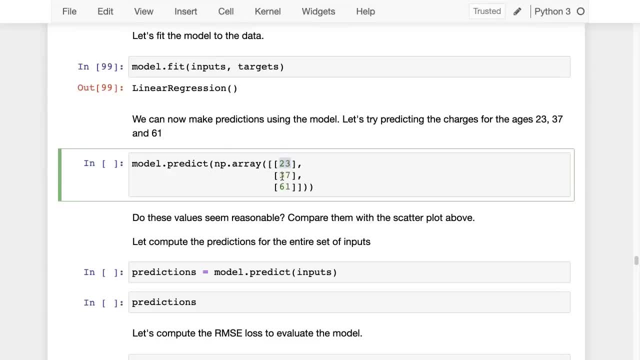 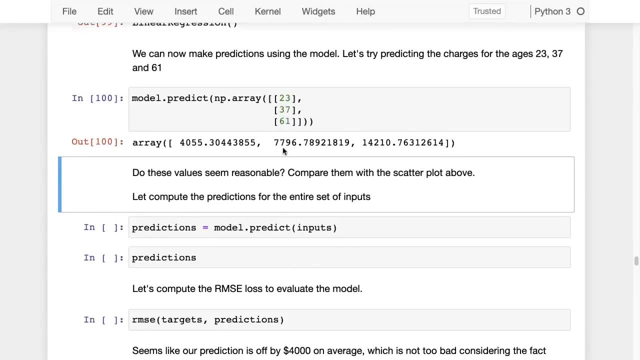 So we have The value 23,. this will be the value of age. another value: 37.. Again, another value of age. another value, 61, another value of age. So we expect to get three values for the charges. So for this row, or for this age 23,, the model predicts four, 0, 5, 5. for this age 37,, the model predicts seven, seven, nine, six. for this age 61, the model predicts one, four, two, one, zero. Okay, So it's starting to look good. Remember When, for for smaller ages, the cost is around $4,000.. And then for the larger ages, like around 60 or 64, it gets to be, it gets closer to 15,000.. 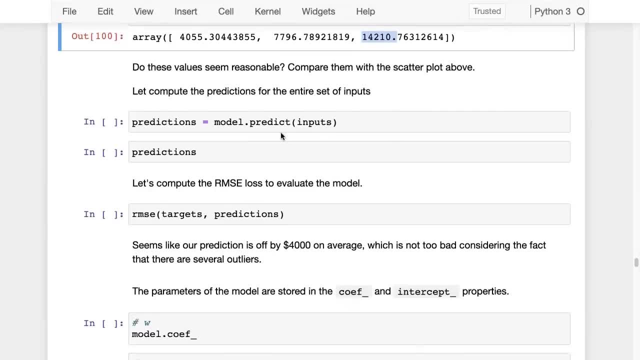 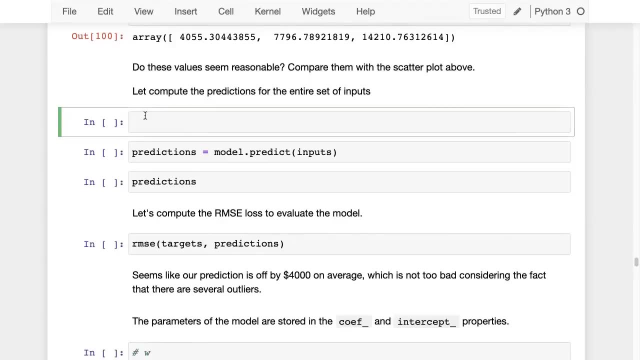 So it seems like our model has done a pretty good job. Let us maybe compute the predictions for the entire set of inputs that we've given the model. So what does our inputs are? inputs are simply the ages, right? So we, you can see here, our inputs are simply the ages. 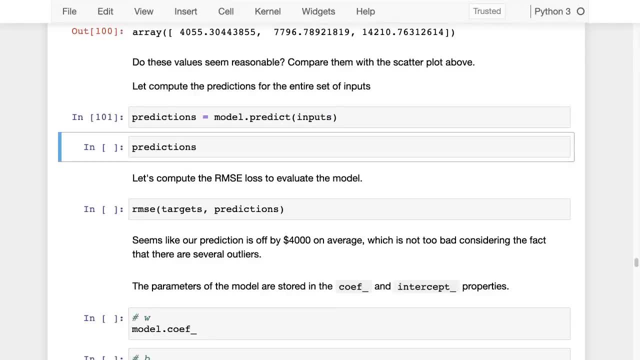 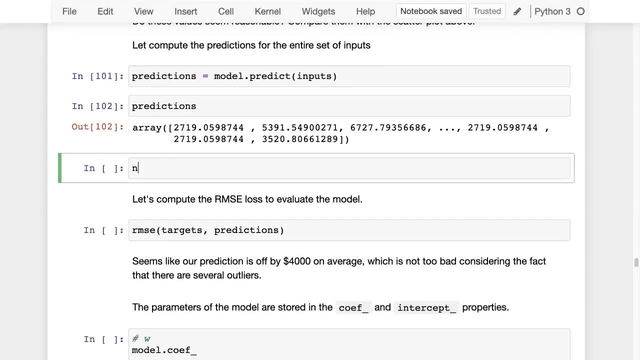 So let's give a full list of all the ages and let's see what the model predicts for all the ages. So this is what the predictions look like and you can check what the inputs are and see if these seem reasonable: 18,, 28,, 33,, 31.. 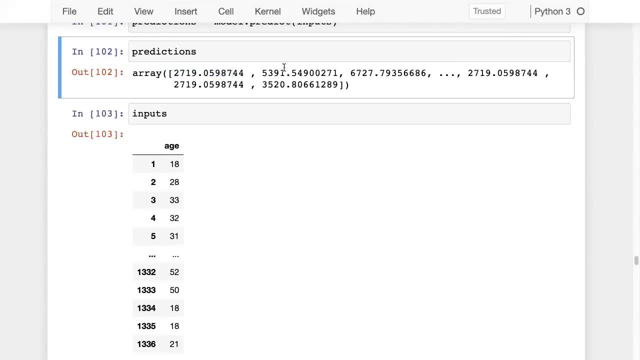 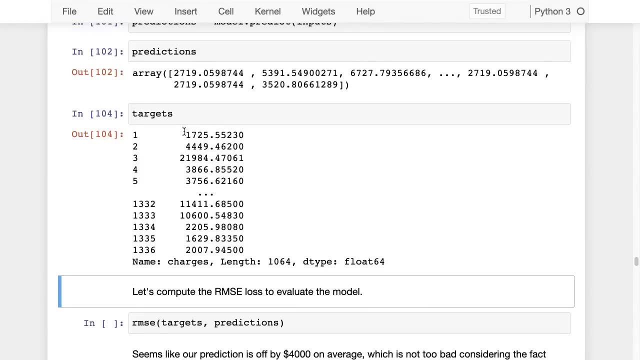 So for 18, we predict two, seven, one, nine. for 28, we predict five, three, nine, one and so on. Maybe let's compare them with the targets. The targets is the actual costs that these people incurred. 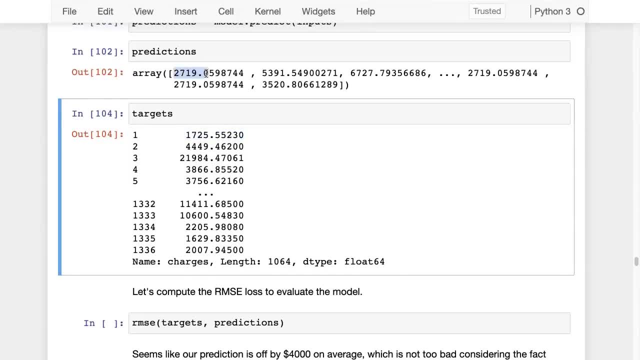 So this person incurred a cost of one, seven, two, five and we predicted two, seven, one, nine. this person incurred a cost A four, four, four, nine and we predicted five, three, nine, one. this predict. this person incurred 21,000 and we predicted six, seven, two, seven. 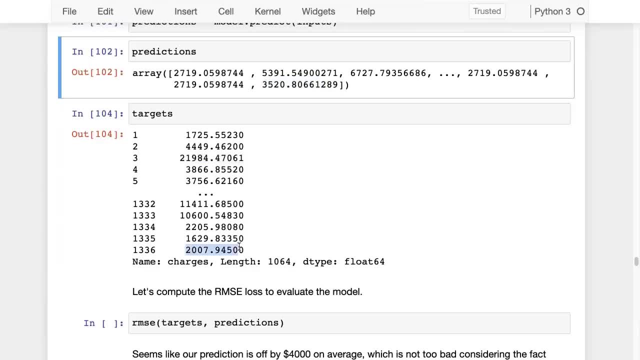 This person incurred three five. this person incurred 2007 and we predicted three five, two zero, So it's in the good range. It's not that bad. It's maybe off by a thousand or so, but when you're dealing with values in the range of about 15,000 or so, the error of thousand is probably acceptable, right. 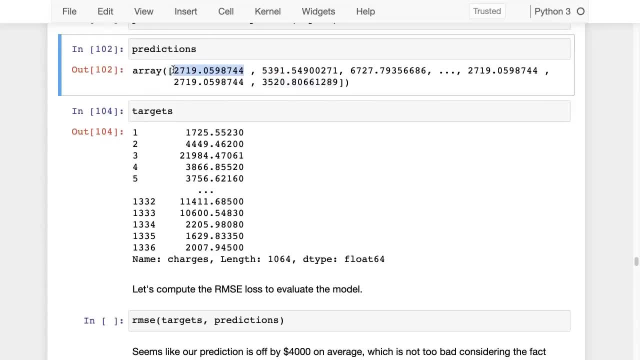 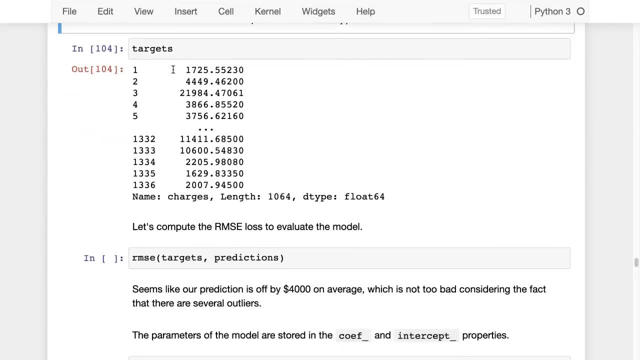 And it's mostly on the higher side for lower values, which is fine too, because we know that there are a lot of outliers which are quite high in value. Okay, We can also look at the loss. We have this RMSE function, which is the root means squared error. 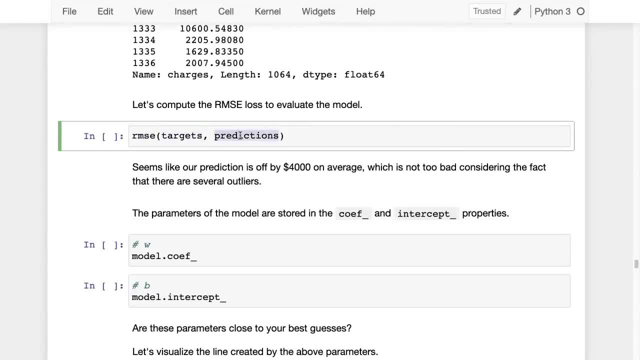 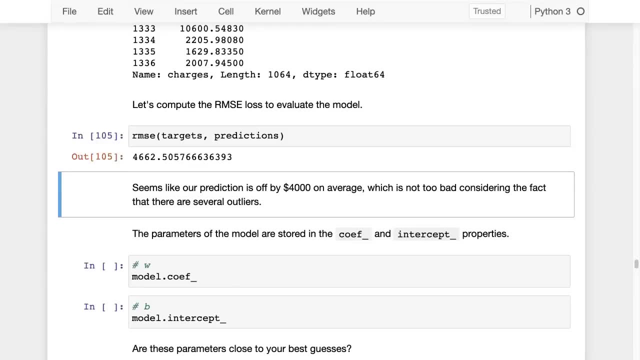 So with that we will take the targets minus predictions, square all of the numbers, add up all the squares, take the average and take the square root of that. Let's look at the RMSE. So the RMSE for this model- the root means squared error- for this model is four, six, six, two, which means on average we are off by about $4,600.. 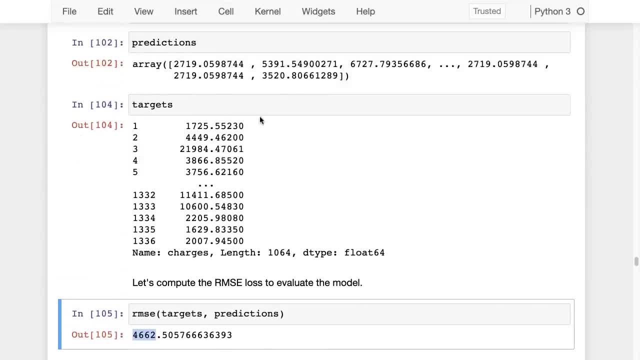 And that's the average. but actually when you look at the values, you'll see that you're not. you're off by much less. It's just that some of these are such big outliers that we cannot capture that relationship with just a simple line, right. 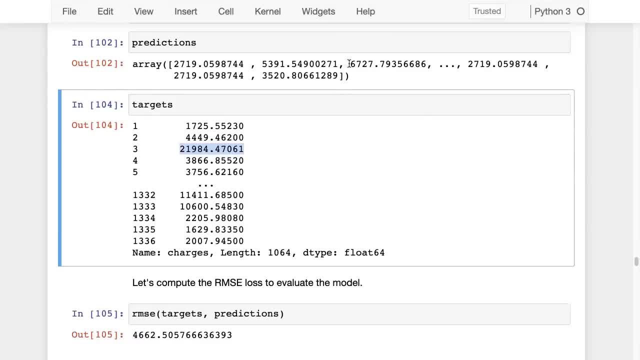 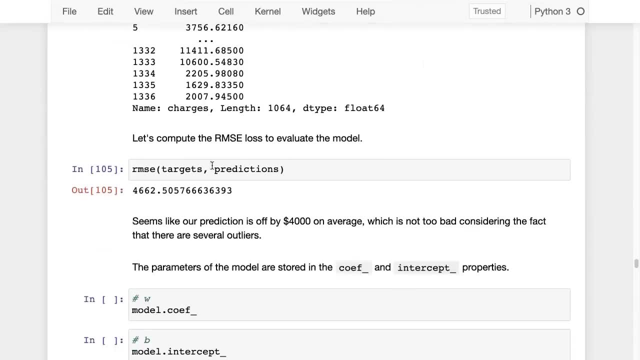 You can see that this one we should be predicting 21,000, but we get six, seven, two, zero, and it's simply not possible to get that far out of an outlier Using a line. So on average, we're actually doing much better than four, six, six, two. 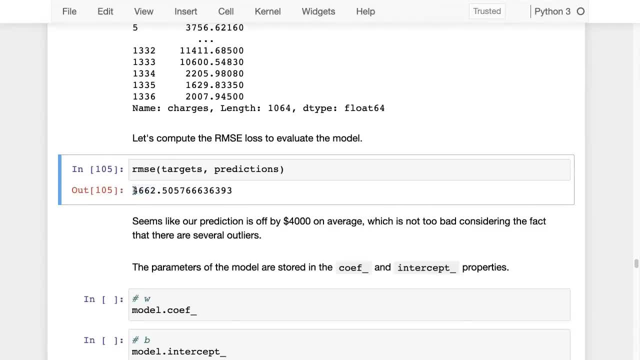 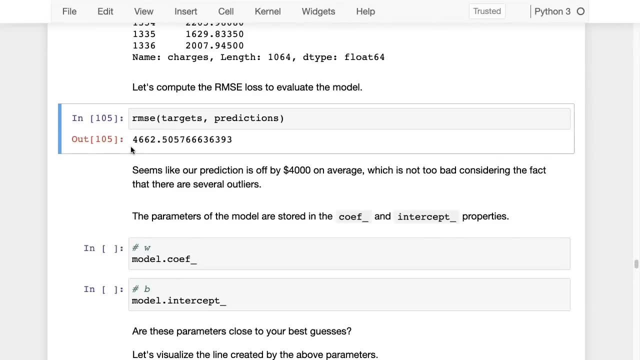 We are probably in the thousand 2000 range. but yeah, this captures the fact that there are a bunch of outliers and in the model as well. So this is the whole process of machine learning, that you assume a certain relationship between inputs and targets, which is the linear relationship. 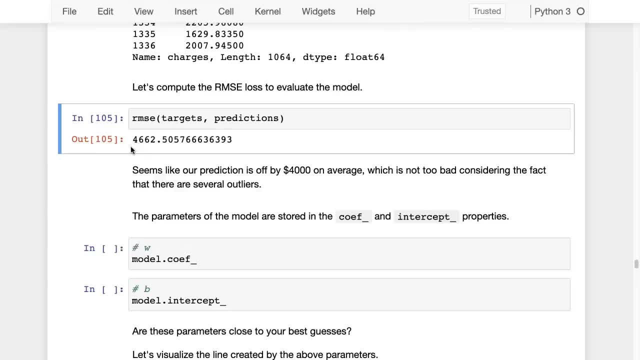 You then find a loss. you find a way to measure how bad your model is, based on certain random parameters that you've picked Initially, And then you use some kind of an optimization algorithm to improve the parameters of the model, in this case w and B, till you can minimize the loss. 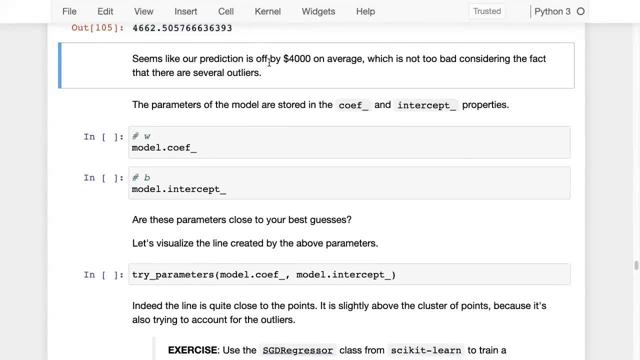 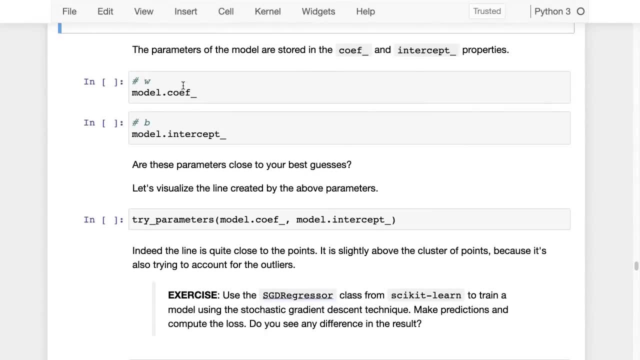 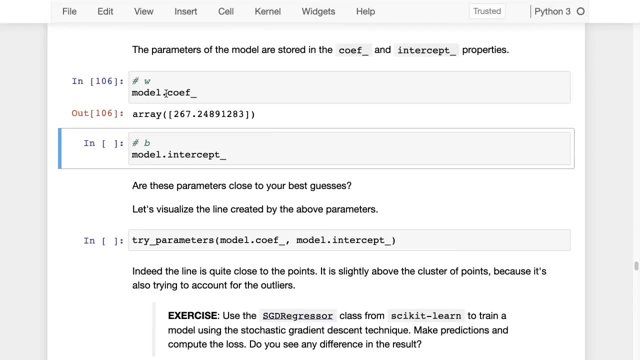 Okay, So we've gotten to a good point on. model is off by 4,000 on average, which is not too bad considering that there are several outliers. Now you may be wondering where's the w and B? well, in psychic lawn, the w is stored in modelco F. it's stands for coefficients. 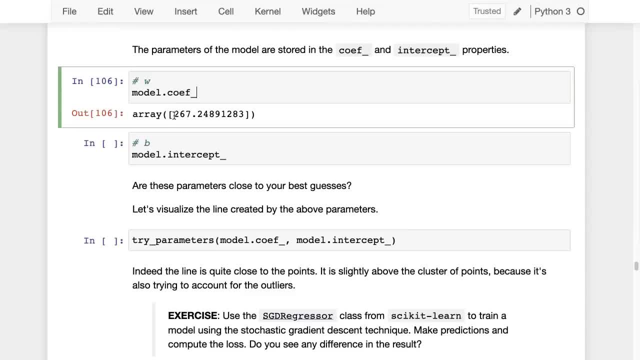 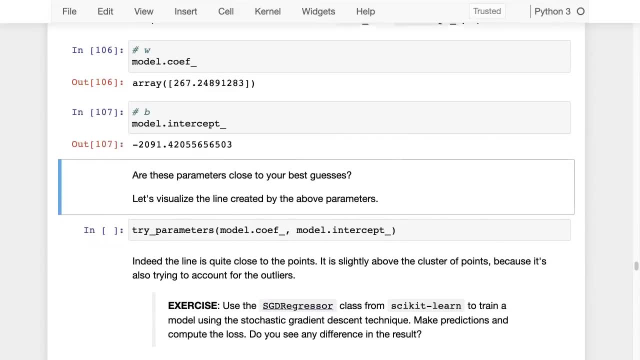 Which are the coefficients or the weights applied to each individual feature. In this case we're just working with age. So we have two, 67 is the coefficient w, and then we have B here. Okay, So model dot intercept contains B, and that is minus 2, 0, 9, 1.. 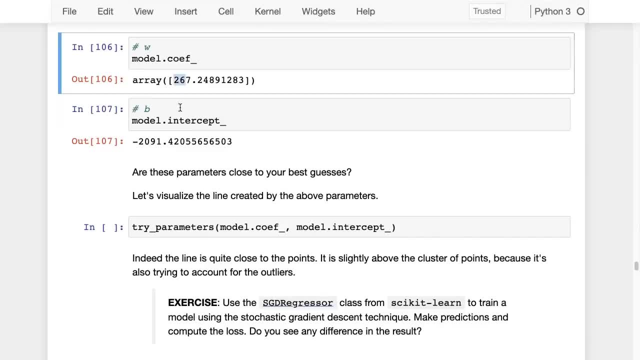 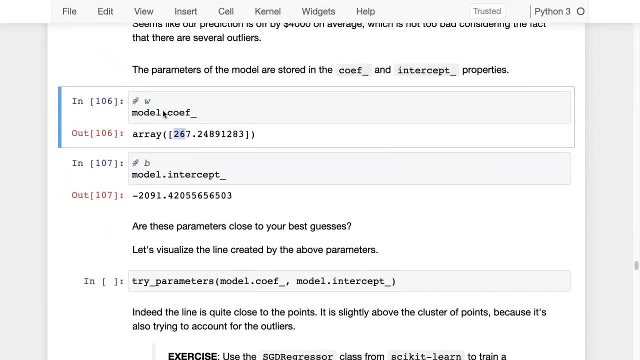 So it seems like if you had picked a w of 2- 67 and a B of 2 0- 9- 1,, we would have gotten a pretty good line, And that would have been our best. That would be would have been the best possible model. 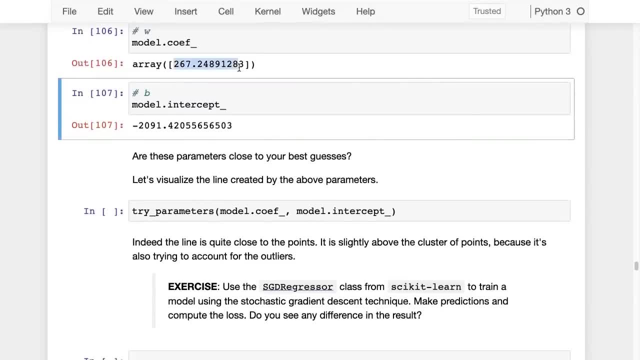 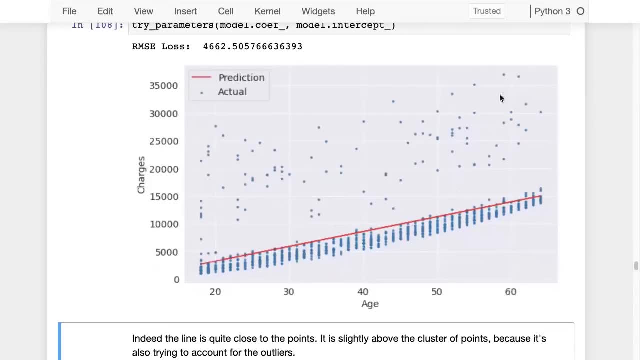 So when you try this out later, see How close you can get without actually looking at the values of w and B. Okay, So let's maybe just plot them once again. So here we have all the points in blue and here we have our model, our line showing the predictions. 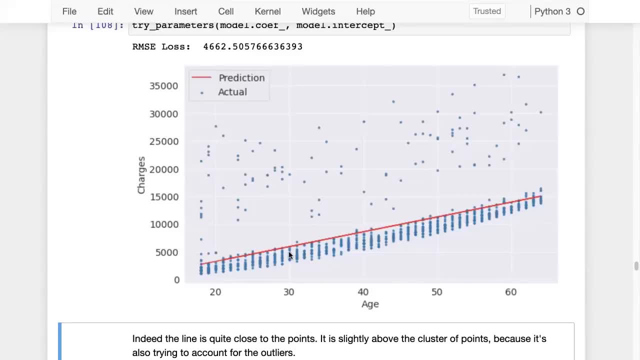 So you see that our line is fitting quite nicely. I wouldn't say it's bad and it's slightly above this cluster, because we also want to somehow capture the fact that there are certain outliers at the top. So if we, if the line was somewhere here, 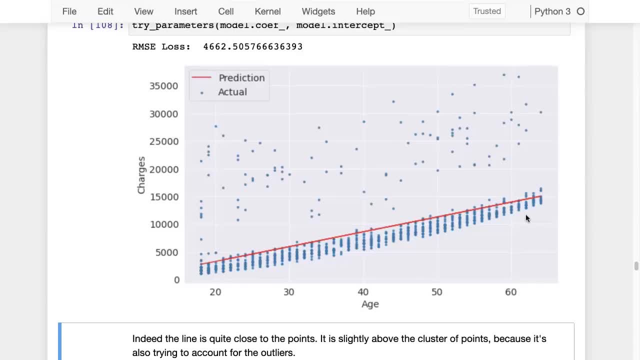 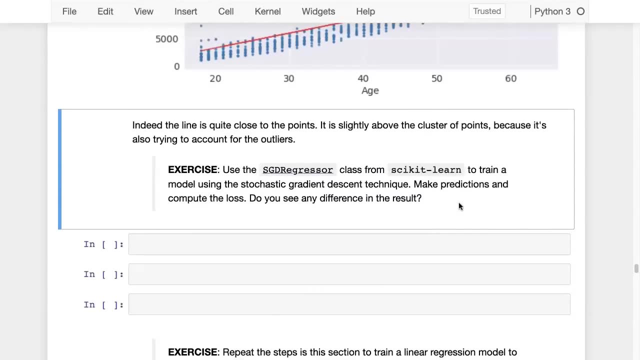 It would technically not be giving the right information because it would not be suggesting the fact that there are outliers. So to account for all these outlets, it's slightly above the data, but that's pretty good. It's yeah, And that's how you do it. 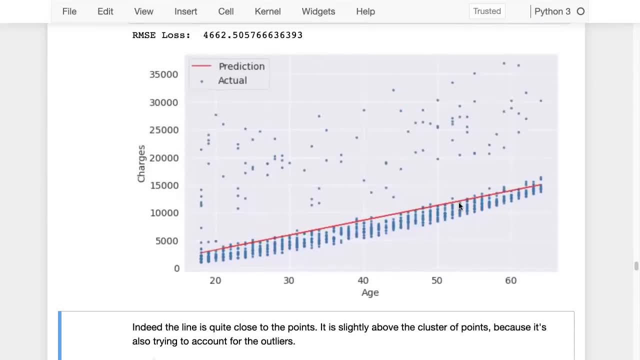 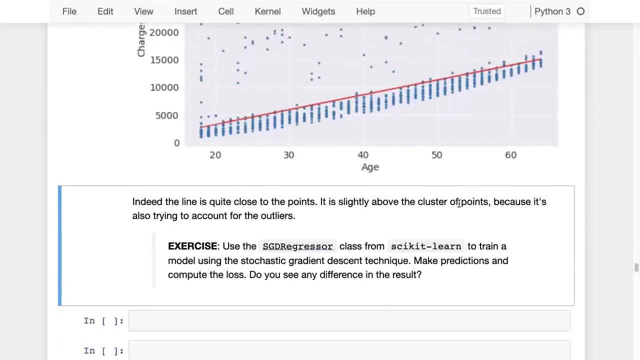 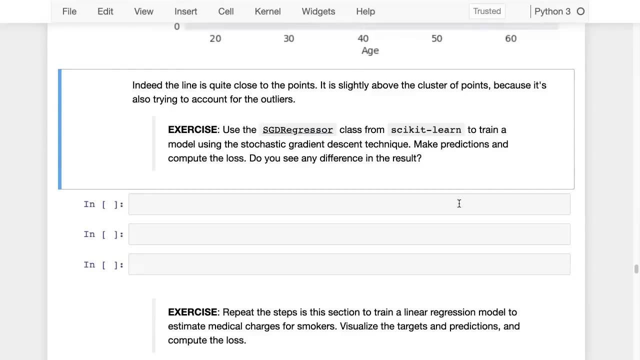 That's how you do linear regression using scikit-learn. You use a linear regression class, then you fit the model and then you generate predictions on new data or on existing data. Now the linear regression class uses this optimization technique called ordinary. There is another technique called gradient descent that I had mentioned for that. 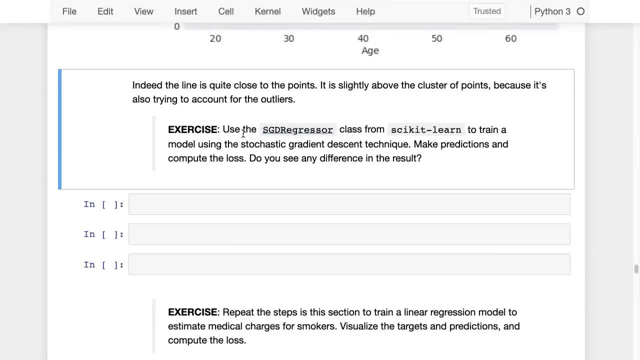 You need to use the SGD regressor, So I encourage you to try out SGD regressor. It works in exactly the same way. This is the one of the nice things about scikit-learn: If you know how to use one model, you know how to use all the models. 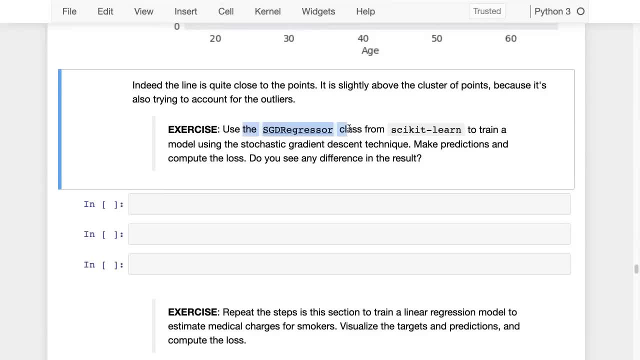 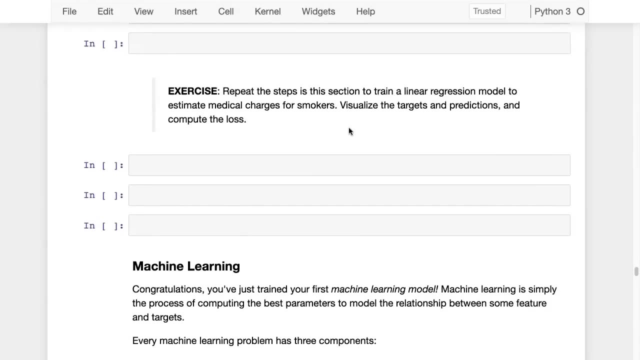 It's just that internally what's happening is different. So try out the SGD regressor and train a model. make some predictions, compute the laws and see If you see any difference in the result. Okay, One other exercise for you is to repeat the steps in the section to train a linear regression model to estimate the medical charges for smokers. 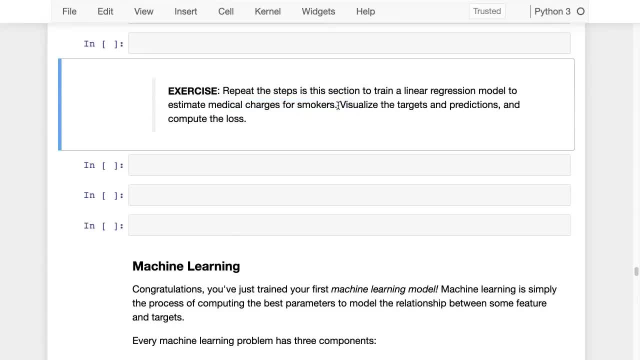 So till now we've been dealing with non-smokers. So now you work with smokers and then visualize the target and predictions and compute the loss Once again. are you able to get a better model for non-smokers? What does that look like? 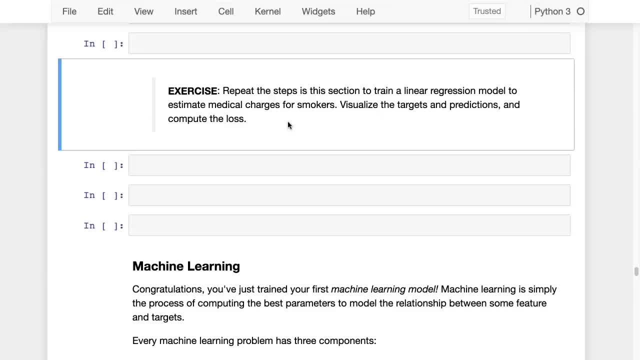 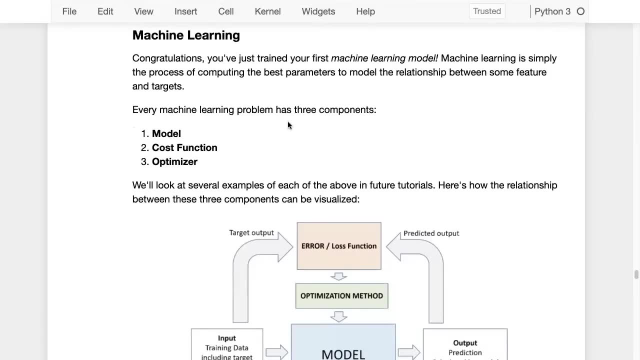 Because for non-smokers, we seem to have these two clear clusters of data, so that would be worth figuring out. Okay, And that's it. Congratulations. You have just trained your first machine learning model, and machine learning is simply the process of computing the best parameters to model the relationship between some feature and targets. 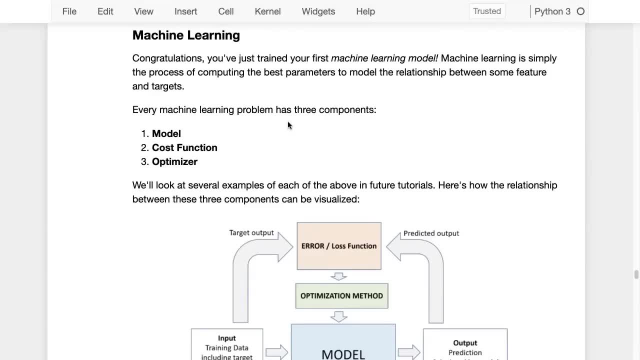 So every machine learning problem that we'll solve in this entire course or in general, that you'll solve any time, will generally have three components. The first thing you will have to decide is: How do you want to model the relationship? Do you want to model the relationship as a linear equation? 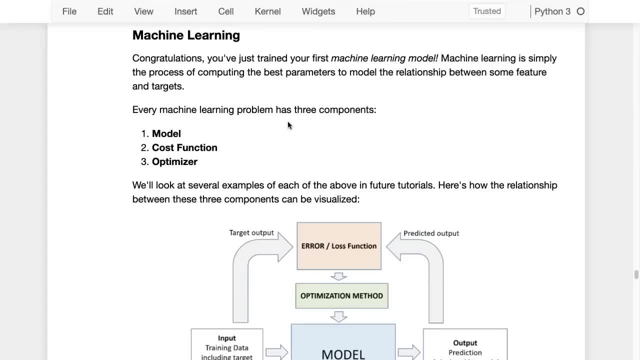 Maybe you want to model the relationship as a polynomial equation. Maybe you want to model the relationship as some kind of a decision tree. Maybe you want to model the relationship in some other way. There are many, many, many ways to model relationships. 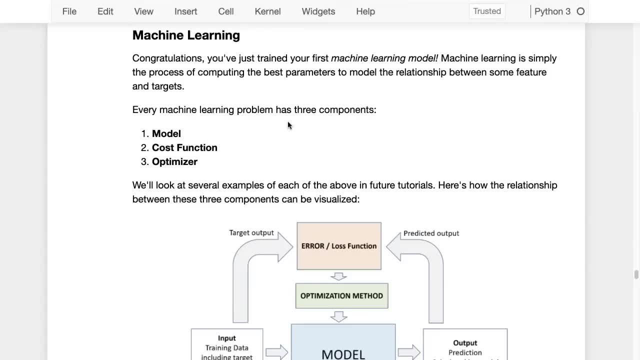 The simplest one is to just say that the the thing that we're trying to predict the target is some kind of a weighted sum of the thing that we're trying to predict. the target is a weighted sum of, Okay, The input features that we're interested in. 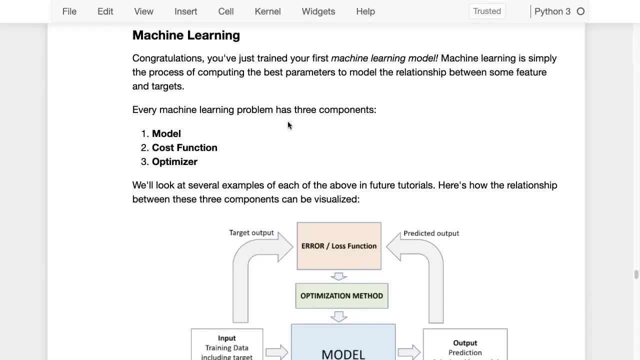 For example, we could say that the charges is simply some weight w one multiplied by age, some way w two multiplied by number of children, Some way w three multiplied by BMI, plus some number B. some intercept right. So that's the model, and every model has parameters. 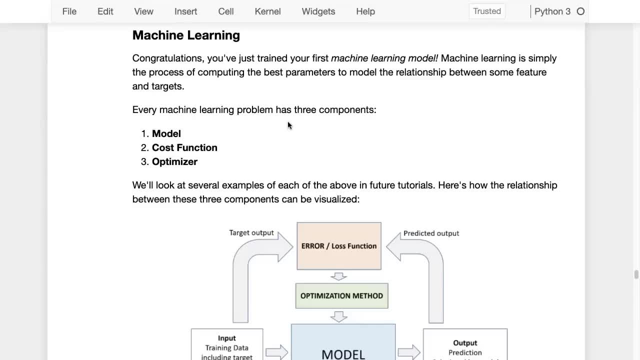 That's what the machine has to learn, So to understand how good the parameters are of the model. we have a cost function and there are several choices for Cost function. but the idea for the cost function is that it should give you a cost, which it should give you how badly the model is performing, and the lower the cost, the better the model. 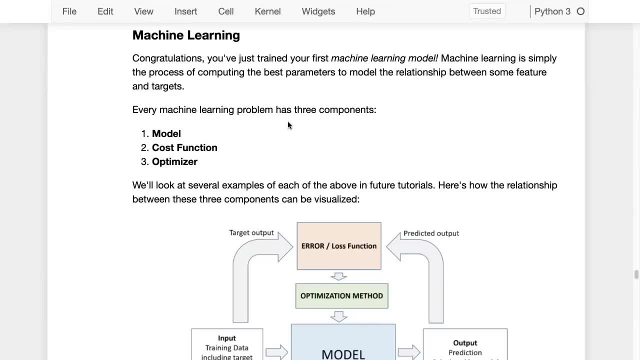 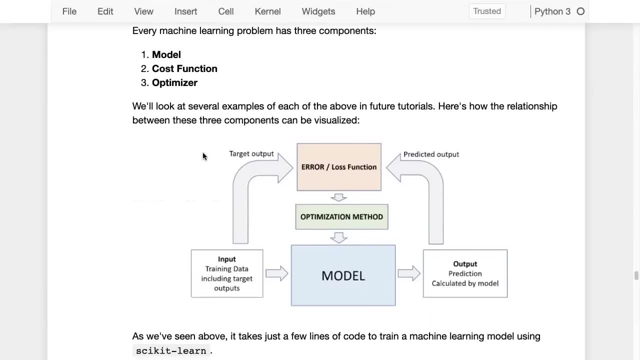 Okay, Once you have a cost function that can be computed, given some targets and predictions, then you need to use some kind of an optimization technique to optimize the cost, which means to change the parameters of the model so that it better fits the data. 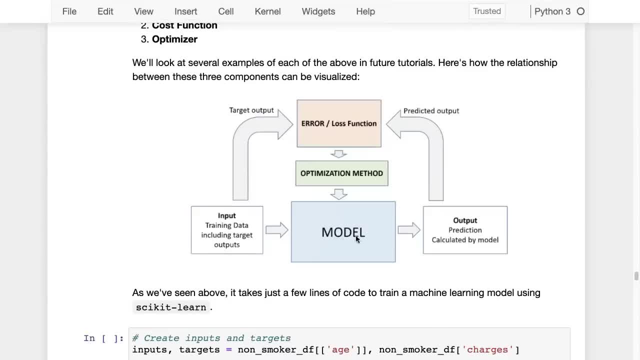 And this is what this entire process looks like. You put some input data into the model and you get some outputs. You put- you take- both the target and the output into the error or the loss function. You then apply an optimization method and that optimization method changes the weights and biases or changes the parameters of the model. 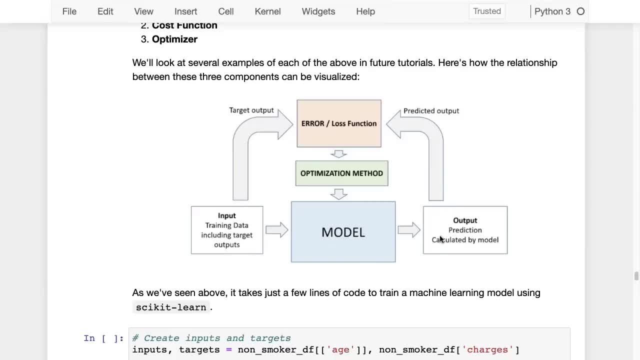 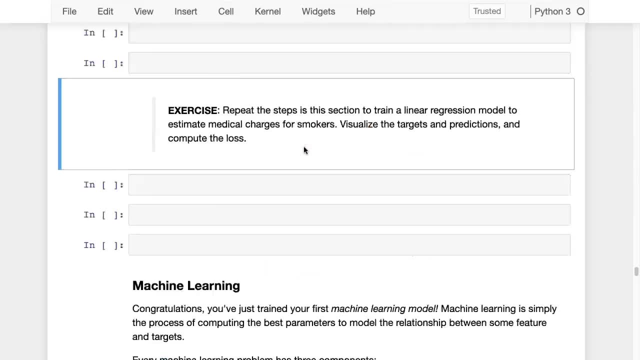 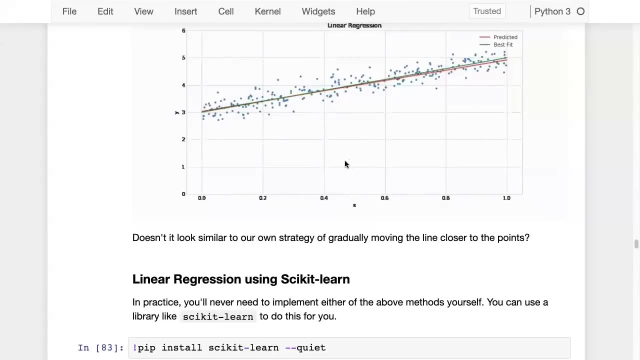 So the model gets slightly better. Then you put some more input data, you get some more output. You take that, put that into the loss function, perform optimization and improve the model. This, what we're seeing here is Is essentially this animation that we saw here, which is taking the line and slowly moving it so that it perfectly fits the data right. 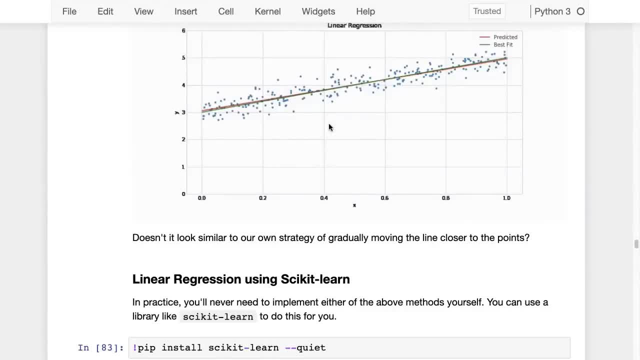 So most of machine learning, and even a lot of deep learning, is basically glorified line fitting. That's all we are doing. We are fitting lines And the fact is that the only difference is we are saying that the relationship, instead of being a line, is something else, and we're asking the computer to compute the parameters in that. 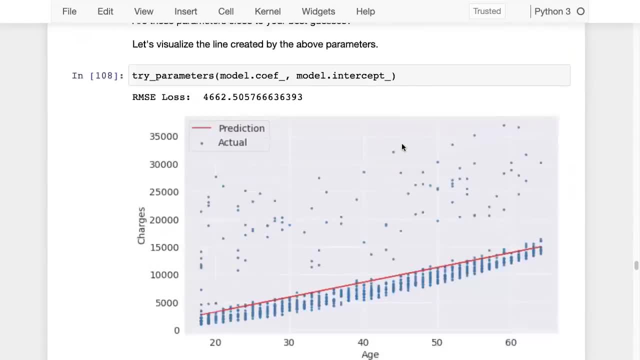 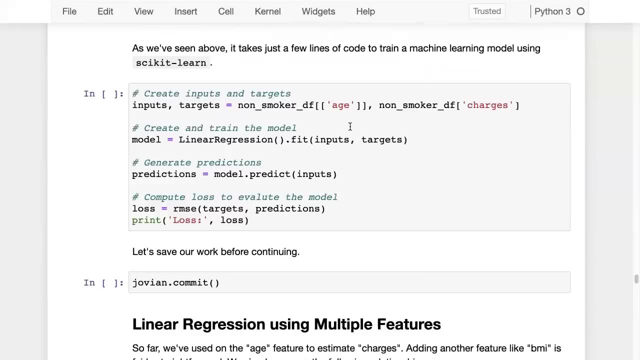 Relationship or the parameters of that model. Okay, So that's, that's machine learning And as we've seen it, just it takes just a few lines of code to train a machine learning model using scikit-learn. You start out by creating some inputs and some targets. you, for example, in the inputs in this case are non-smoker DF, and we are just picking a set of columns. 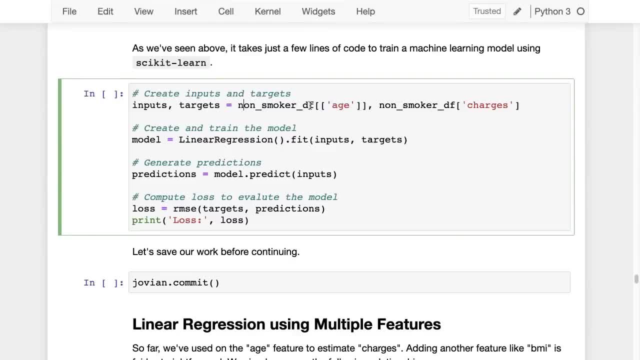 And currently we're just picking one column: age. So the inputs need to be a two dimensional area. Then you have targets, Which can be one dimensional or two dimensions. So you have a list of inputs and a list of targets and then you create a model. 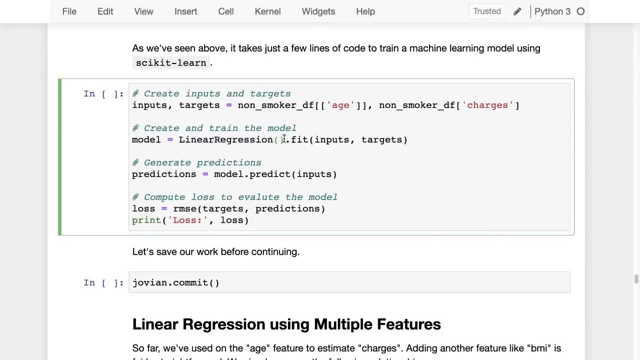 So here we are creating this model, linear regression, and most of the time, immediately. you just want to fit the model, not always, but most of the time. So if you just want to fit the model, you can create the object and immediately call dot fit on it. 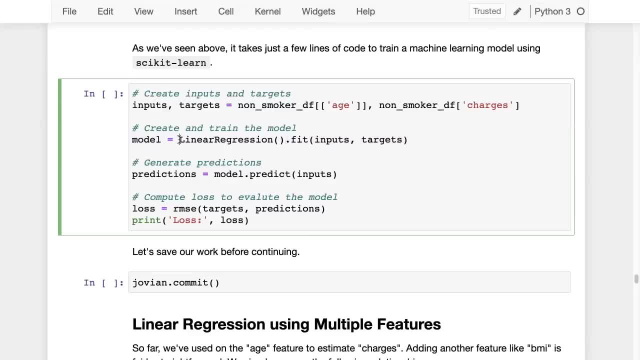 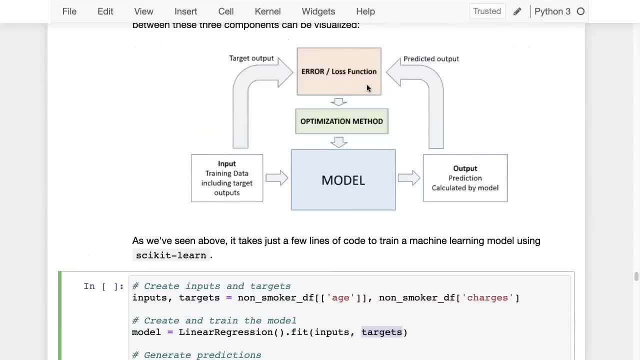 And that will also return the model. So you can just do this linear regression dot fit and into it you provide the inputs and the targets and it's going to go and do its thing. It's going to do all of this for you. 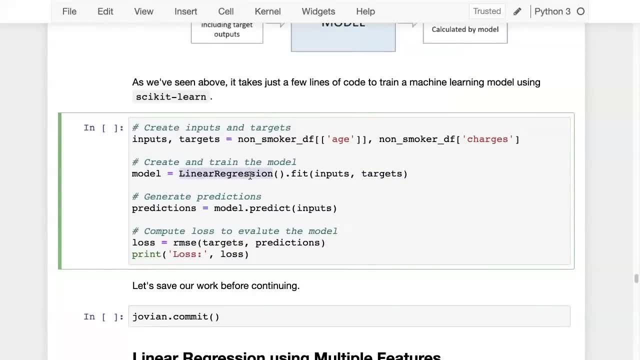 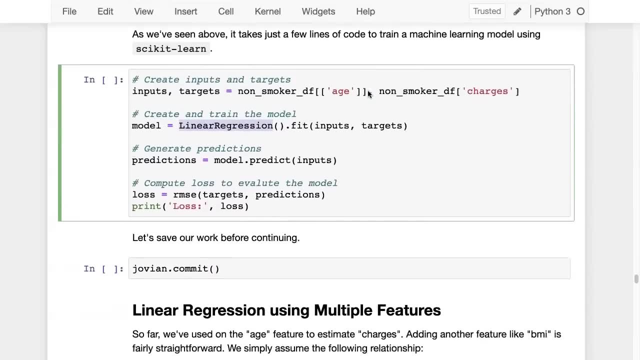 This class determines what kind of relationship you want to assume. Like here: you want to assume the linear relationship, right, So you fit the data and that gives you a model. Then you can use that model to make predictions. So now you can just take this model. 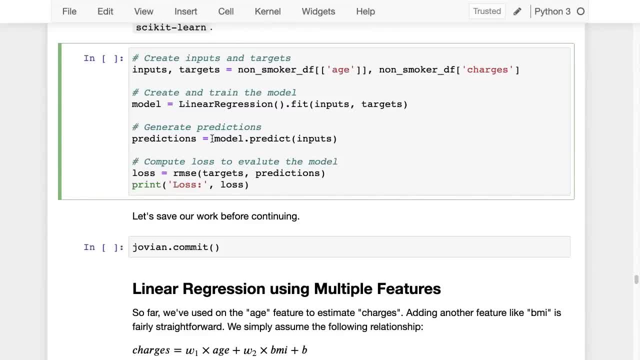 And every time a new customer comes in you ask them: Hey, what's your age? And they say 32, and you put in the number 32 and you get a certain estimate for the medical charges. that estimate can then be used to compute that. 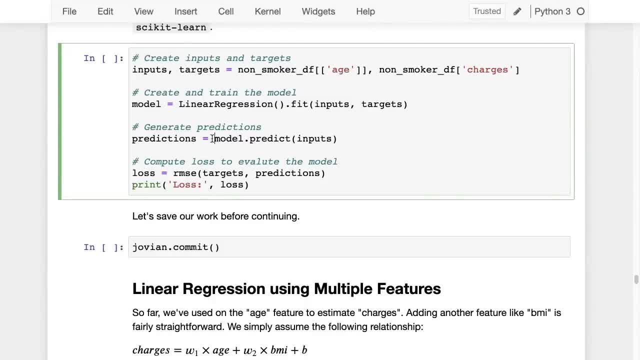 Sure, Sure. So if that's the case, you're going to start doing that. So these are the two things that you can use to calculate the insurance premium And off the go. right, So it automates that piece of analysis which you had to do with, maybe using several experts with years of expertise, and there's a certain error. 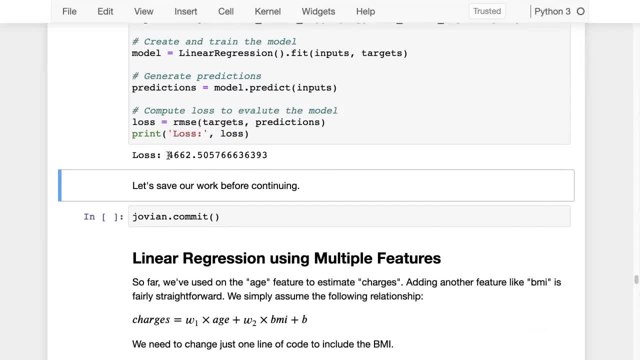 So whenever you use a model, you should be aware of what the error in your model is or what the loss- the information loss- in your model is. So in this case, what we say is that, Hey, my predictions are off by maybe about three or 4,000.. 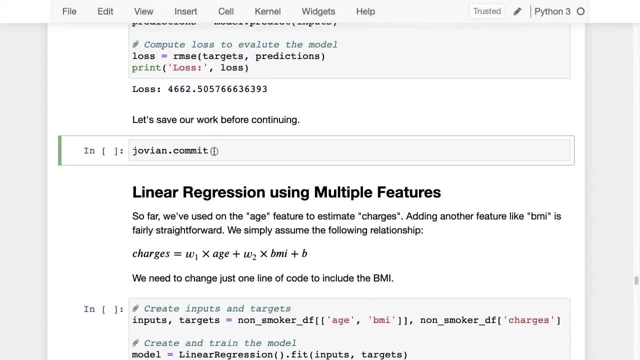 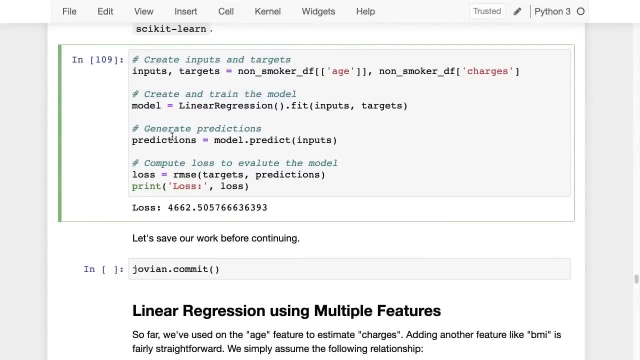 So you may just want to this person, All right, And that's your three or four step process: create inputs and targets, create a training model, create and train a model and generate some predictions with the model. And, whenever possible, you also should have 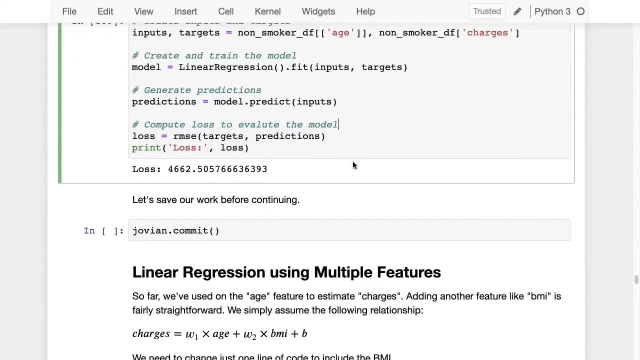 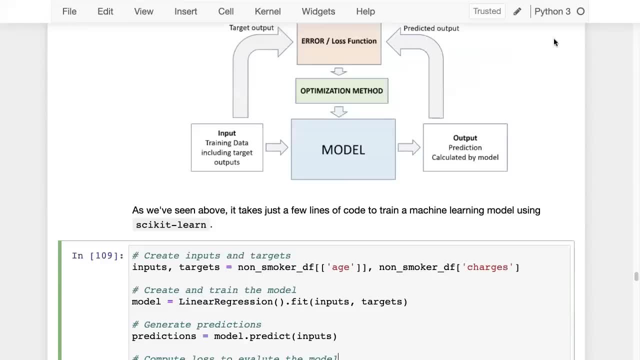 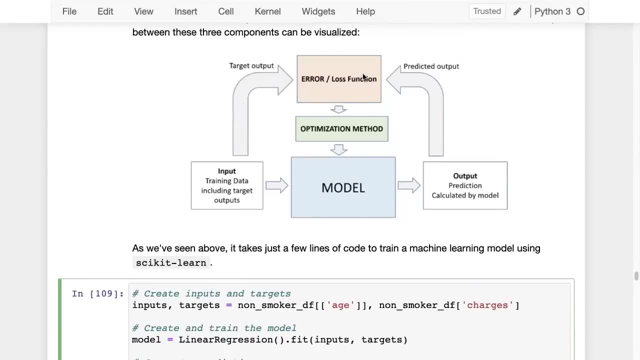 a measure of what is the information loss or what is the error in your model. So you create the input data and then you put that into some kind of a model and the model gives you some predictions. Now you compare the predictions with the actual outputs and that gives you some kind of a measurement how bad your model. 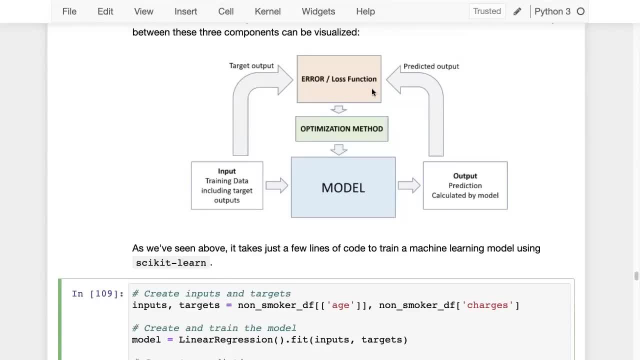 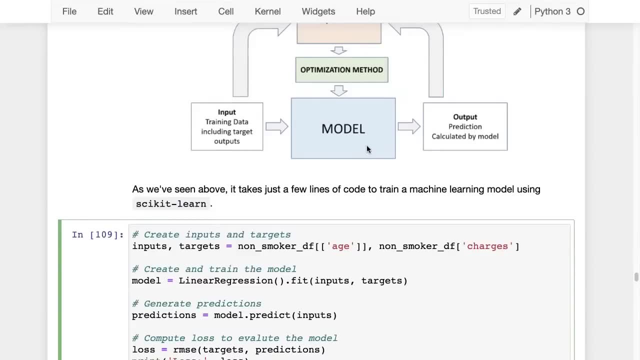 is your model is really bad initially. Then you run some kind of an optimization method and that improves your model. So as you give some data into the model, it learns from the data, It makes better predictions. Then you give it some more feedback using the loss function. 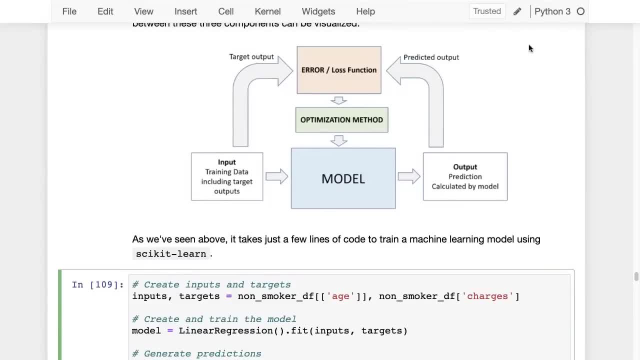 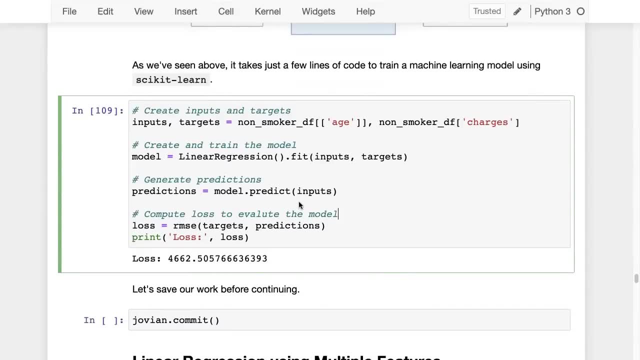 It makes a better prediction and it gets better over time. If you can just grasp that basic idea and see how it is translated Code here, that is enough to get started, And it is a fundamentally different way of thinking about problems. If you are struggling with it a little bit, that's okay. 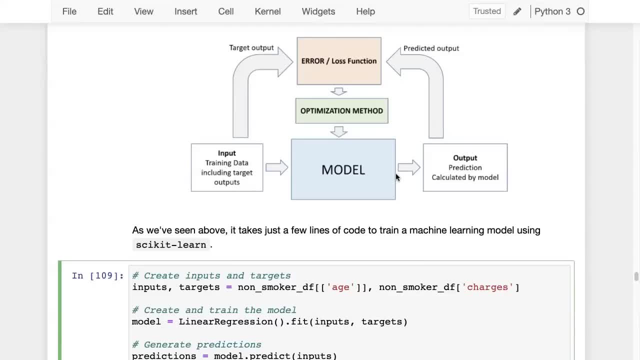 Once you struggle through it and once you get the idea, once it clicks what's happening here, you will suddenly realize the potential of what it makes possible. Because now, instead of, let's say, having several years of expertise in analyzing or evaluating insurance applications, you just have this one system. you just feed. 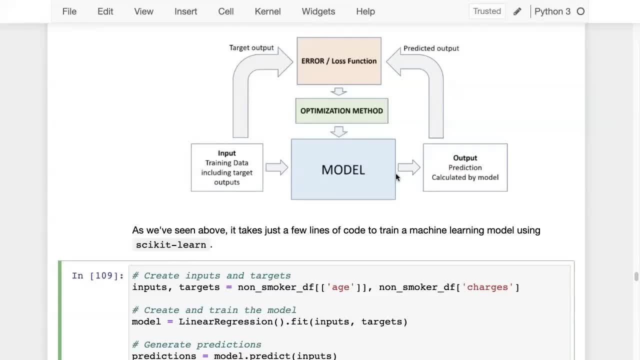 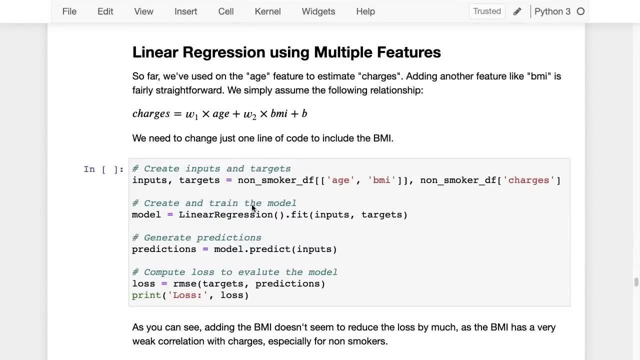 in some input and it's going to give you an output and you know how much it is going to be off by and you can use it. What about some of the other features? so far we've used as the age feature to estimate charges. adding another feature like BMI is very straightforward. 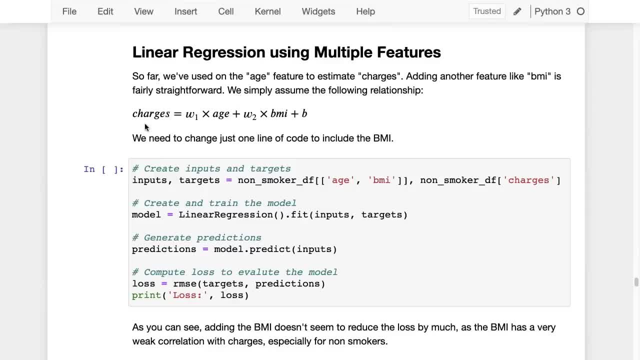 So we simply assume this relationship. Now, instead of saying charges is some weight w plus B, Now we say that Hey, for calculating the medical charges, we give some weight to the age And some way to the BMI. And then we have this other intercept term which is simply to just move the line up or down. 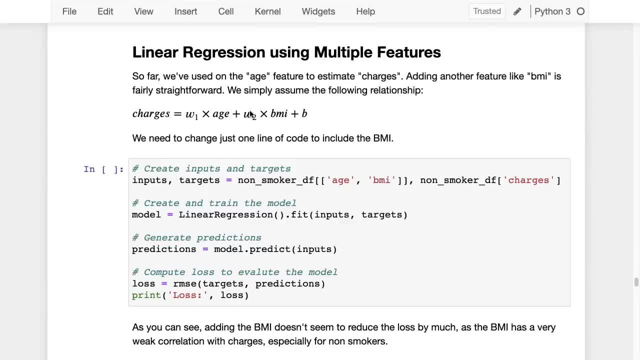 Of course, now this is no longer a line. It's linear in the sense that there is still a linear relationship, You're not doing squares or cubes or anything. but this becomes now a plane in three dimensions. essentially, If you see the, if you put age, BMI and charges on each dimension, this 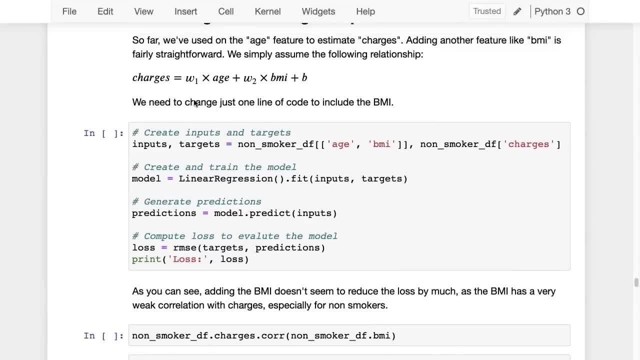 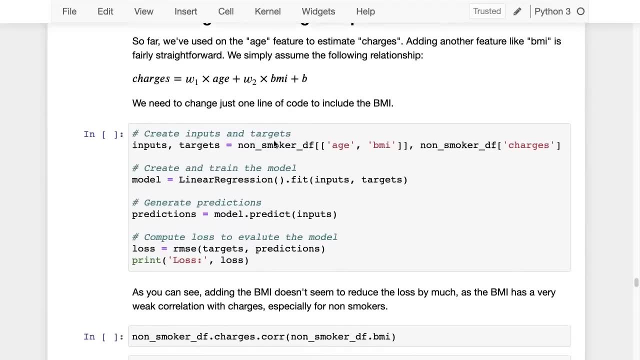 becomes a plane in three dimensions. So now we are working with a plane, but still called a linear regression, simply a linear combination or a weighted average Of the agent BMI, the charges. So how do we apply this in code? The exact same four steps: create inputs and targets. 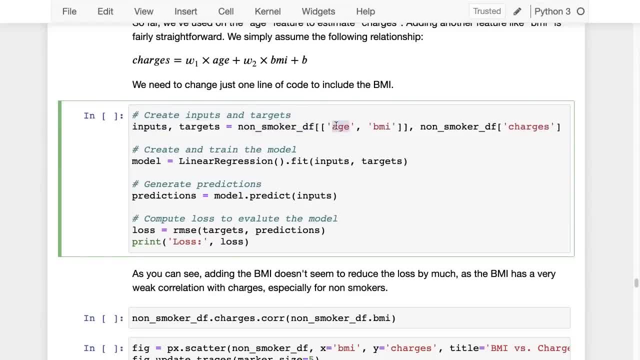 So the inputs are from non-smoker DF. We take age and we take the body mass index and then the targets are simply the charges. The only change we made here is this: the way to train the model and create the model is the same. 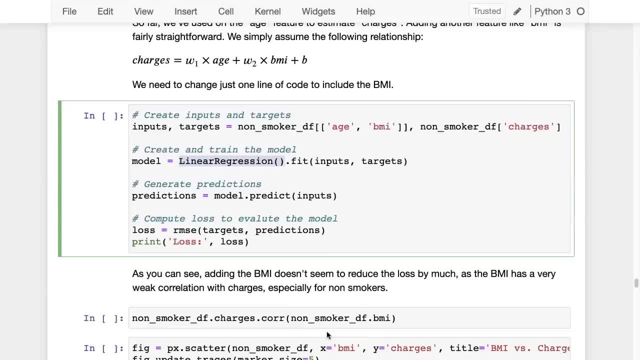 So you create linear regression, You call dot fit And then you put in the inputs and the targets. no change here. It's automatically going to detect that Now you have two columns of data, Then you generate predictions. generate predictions by passing. 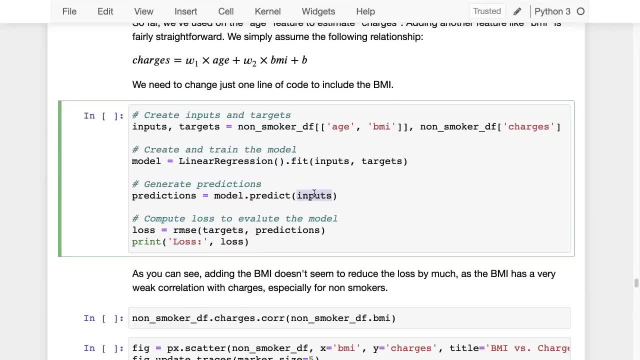 the inputs into model, dot, predict And then finally, you compute the loss. So this is not something that you have to do, Strictly speaking, you, just once the model is trained at fit, you can make predictions on any new input data. 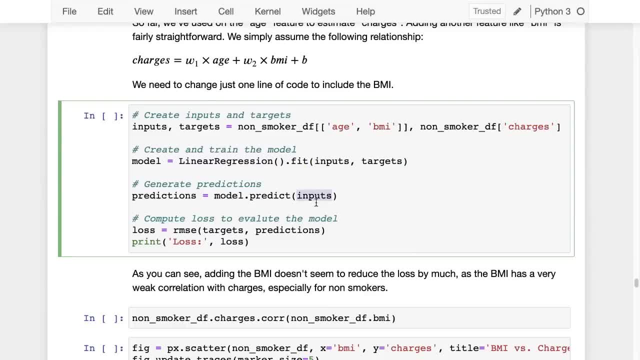 At this point, of course, we don't have any other input data, We just have the original input. So we just passed back the original inputs. but you call it model dot- predict inputs- and that's going to give you a set of predictions. 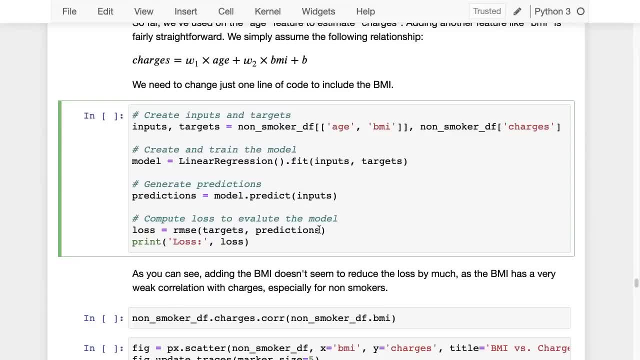 And then you have RMSE, you compute the loss. So whenever you calculate some predictions, it's always a good idea to like: if you have the actual targets, which we do for the inputs, just compare the predictions of the model with the actual targets for those inputs and get the loss. 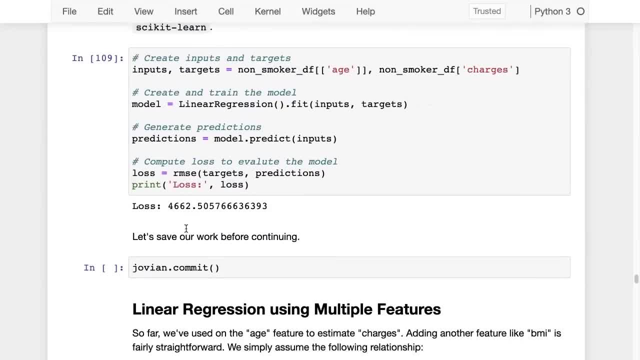 And you can see here we now go from the loss of What's that? 4, 6, 6, 2.5, 0, 5 to 4, 6, 6, 2.3, 1, 2.. 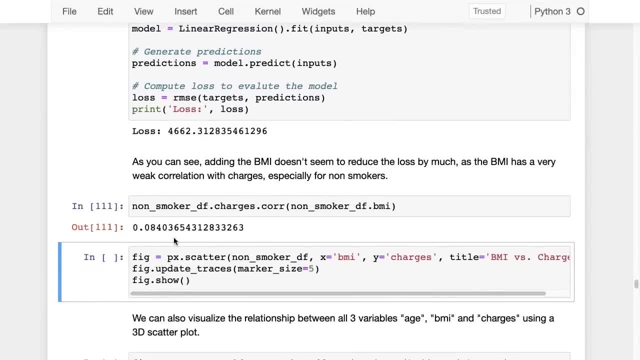 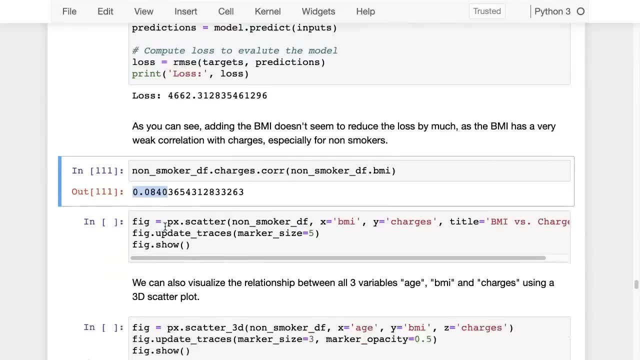 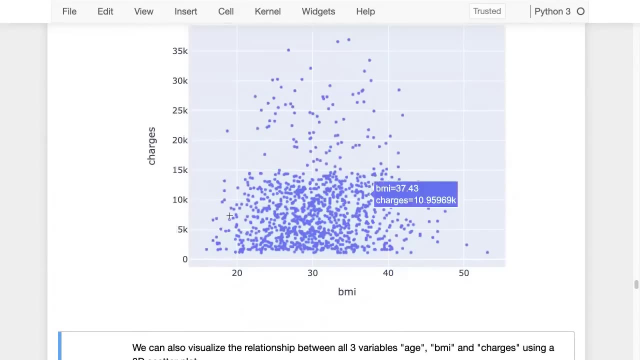 So clearly BMI did not create a major impact, and you can see why: because BMI has a very weak correlation, especially for non-smokers, And you can even see this in this 3d scatterplot, also in the scatterplot between BMI and charges. 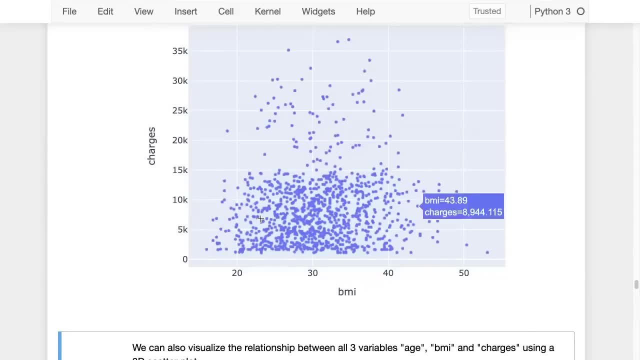 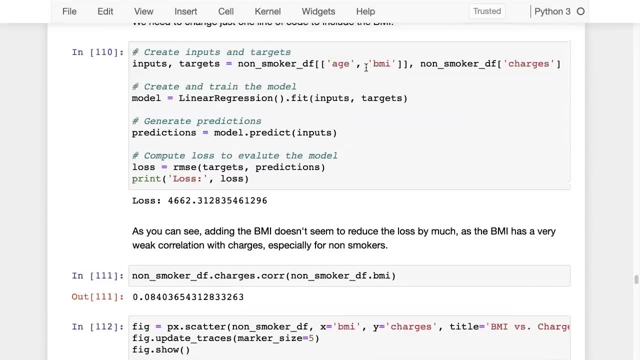 So you can see here that you have BMI and you have charges and there's no real relationship that you can see here, Like there's no line that you can see. And that's where the correlation is low. And that is why, even though we included BMI now, even though we included BMI now, you are unable to see any improvement in the loss. 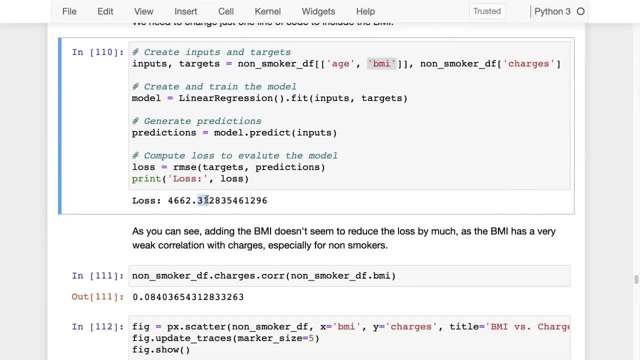 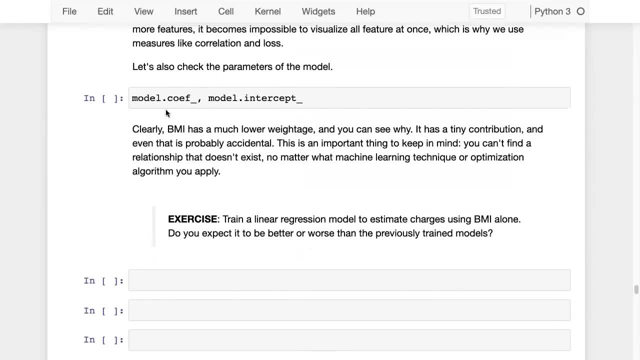 The loss still remains 4, 6, 6, 2.. There's a very minor improvement of a less than a dollar on average. Let's also check the parameters of the model. You will find that the parameters have also not changed much. 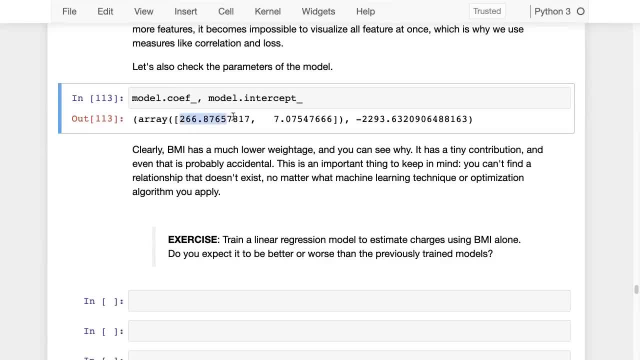 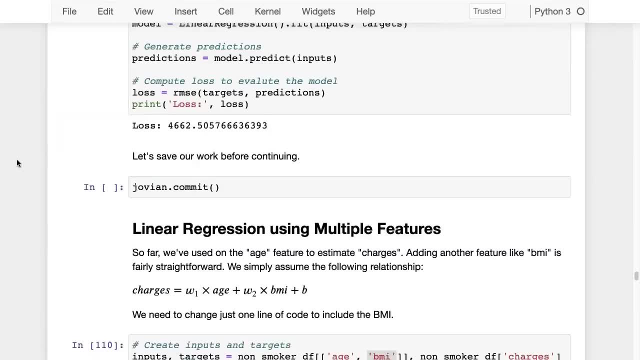 So this is the parameter for age. So for age, we're still using the weight of 2- 66.. This is the model. This is minus 2, 2, 9, 3.. So you can see that these are still quite close to the original parameters. 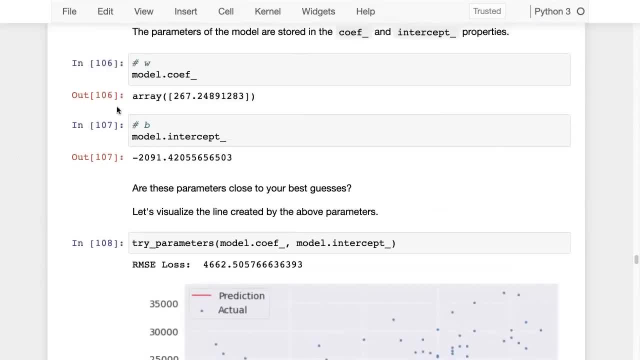 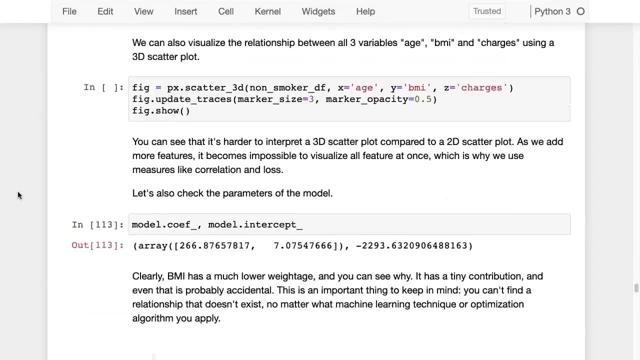 The parameters that we had here were 2, 67 and 2 0, 9, 1.. So the parameters have still remained the same for age and for the intercept: Yeah, 2, 66 for age, That is the weight applied to age. 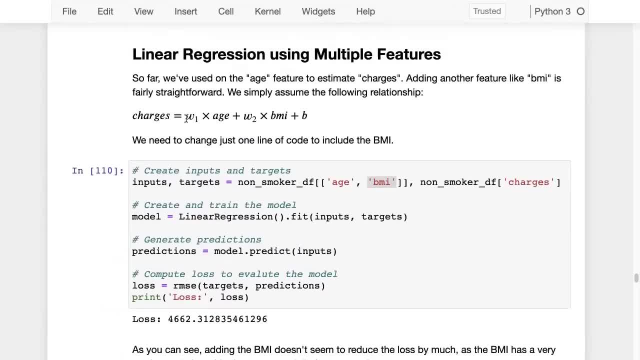 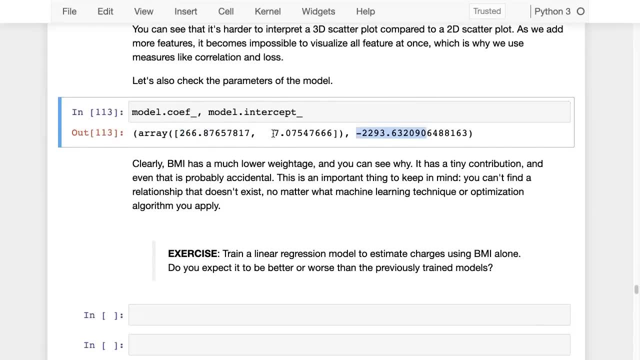 That is w one here. You can see w one. This Is 2: 66.. And this is the intercept: minus 2, 2,, 9,, 3.. And you can see that the parameter or the weight applied to the BMI is very small, which means BMI has very low weight age. 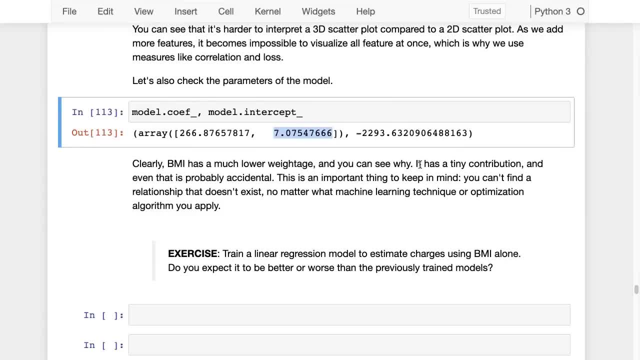 And you can see why it has a tiny contribution to the charges for non-smokers, And even that is probably accidental And this is something that you may want to report to your company- that he there seems to be no relation between BMI and medical charges. 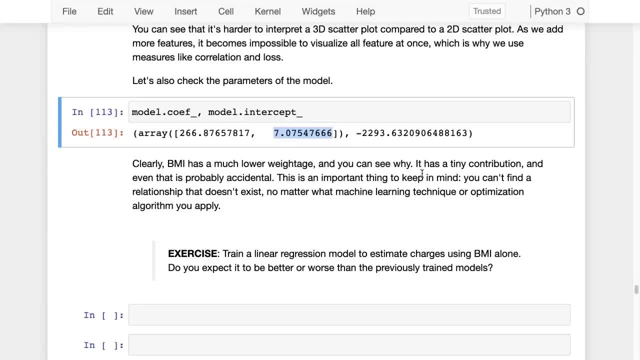 Should we even be looking at BMI? And another Important thing to keep in mind here is that you cannot find a relationship that does not exist. If your boss came to you and said: I want to create, I want you to create a model that uses the BMI and minimize medical charges. 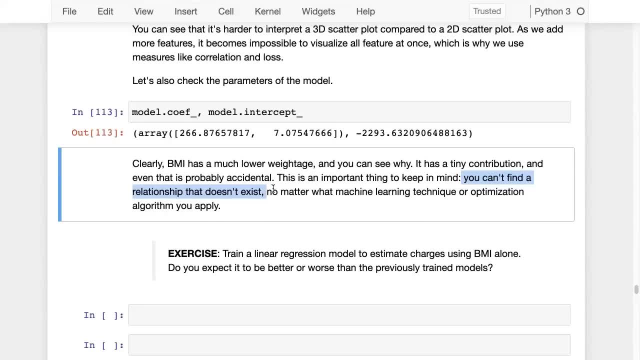 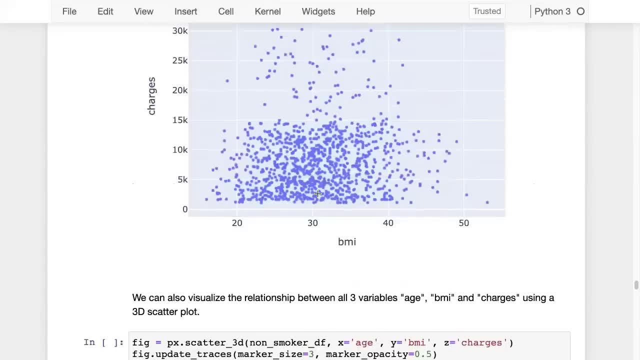 You should just go back and tell them there's no relationship here. no matter what machine learning technique you use, no matter how much data you give me, there is simply no relationship here. All I'm seeing is this. so you can't expect to fit a line to this. 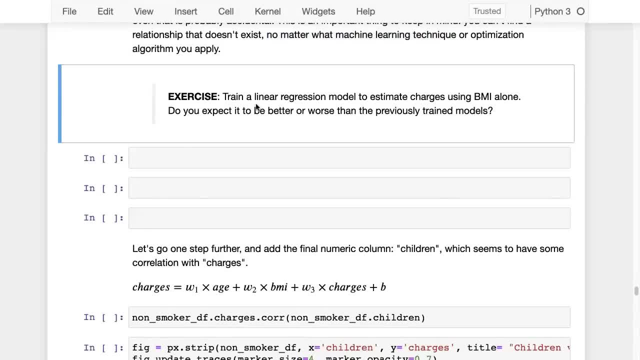 Okay, And you can verify that. train a linear regression model to estimate charges using just the BMI. See, if you expect it to be better or worse than the previously trained model. It should be worse, but it's something that you should verify, maybe even visualize it by plotting the graph. 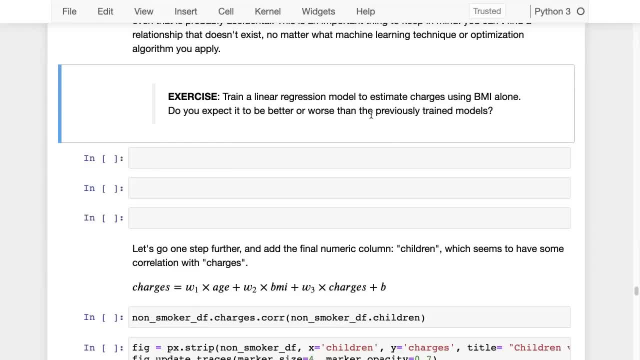 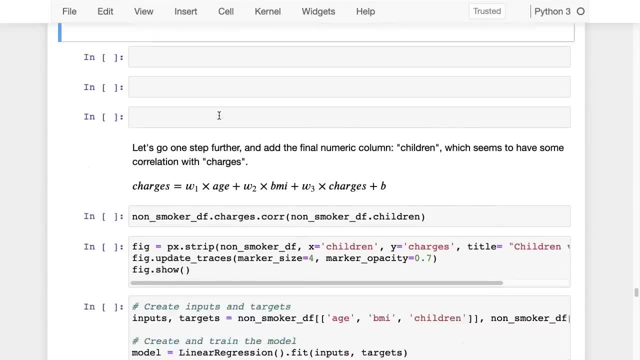 Once again, when you have a single, when you have a single feature, you should be able to plot it easily. Once you go beyond one feature, beyond one input, There's no easy way to visualize. and let's go one step further. Let's add a third numeric column. 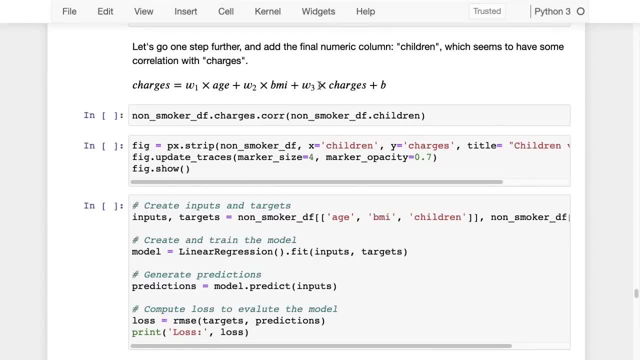 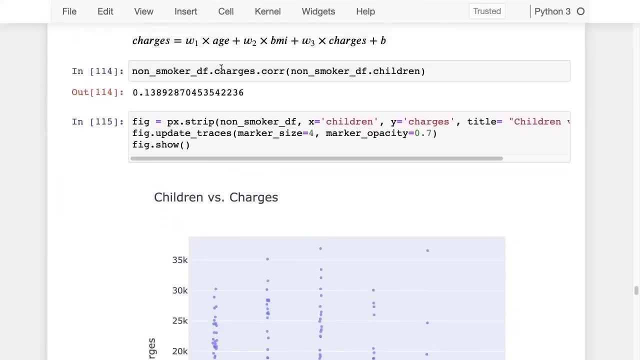 So here we have w one times age, w two times BMI, w three times charges plus B, And this is what you can see here, the correlation between charges and children. So the correlation here is 0.138.. It is lower than age, but it is higher than BMI. 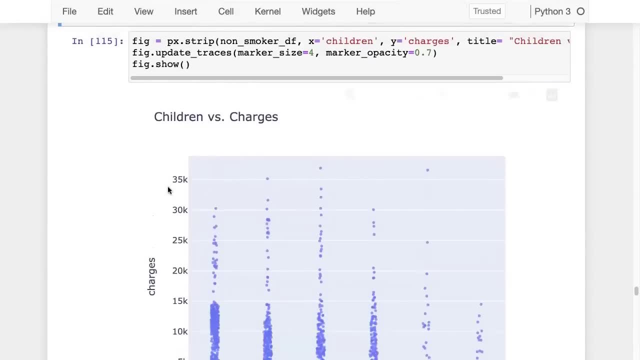 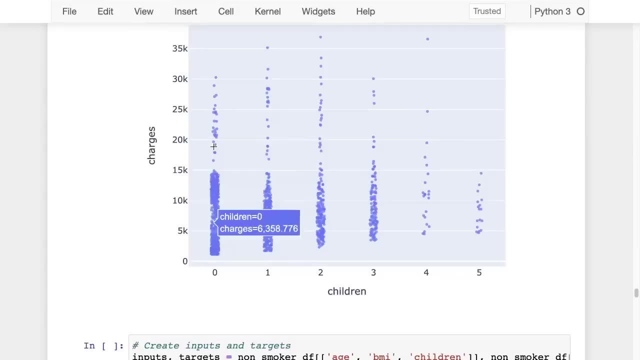 And we can see this using this. this is called a strip plot, similar to a violin plot, but we show actual points. So you can see that there are a lot of these points around, uh, at the lower values here, And then there are more points at the higher values here. 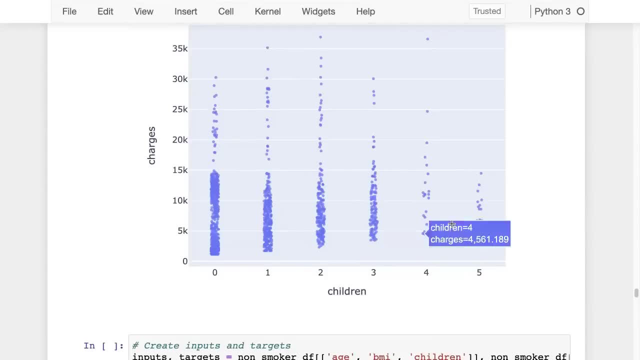 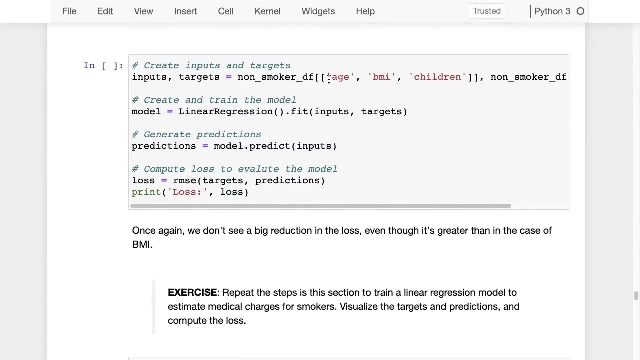 So you can see a somewhat increasing trend. There's definitely a somewhat increasing trend here And that's why you have a slightly positive correlation, although very small. And now to use children, once again we create the inputs and targets, which is, we use age. 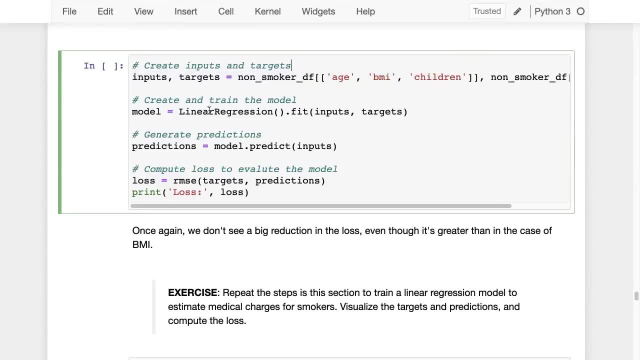 We use BMI and we use children Great. Then we train a model. So we say linear regression Dot fit inputs and targets. Then we generate some predictions. So we say model dot predict inputs. So we pass in the inputs. This time we have three, three columns of data and then we compute the loss for those predictions. 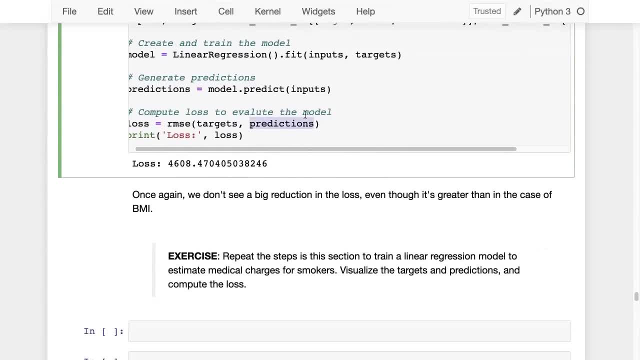 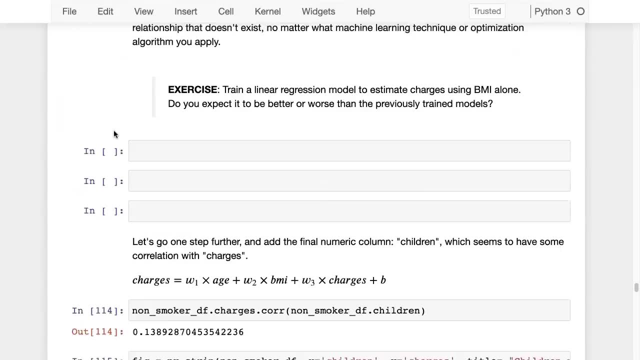 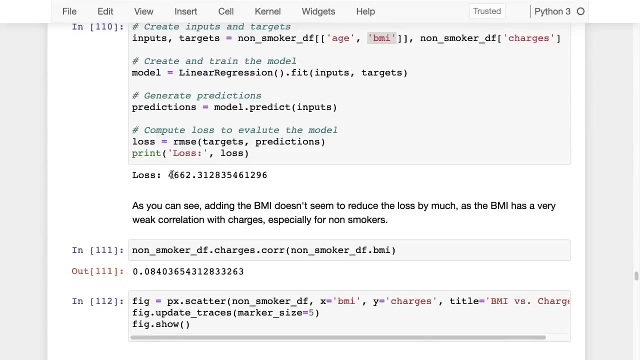 But these are the targets and these are the predictions from a model for the input data and the losses: 4,600.. So there's a slight reduction in the loss. We went from what's that? We went from 4, 6, 6, 2 to 4, 6 0 8.. 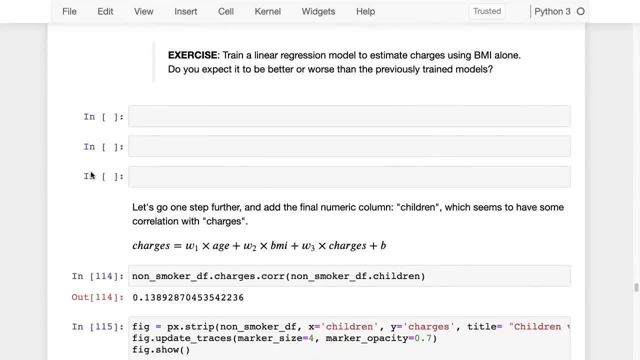 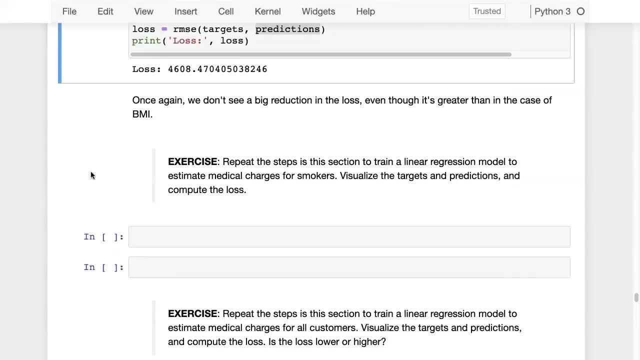 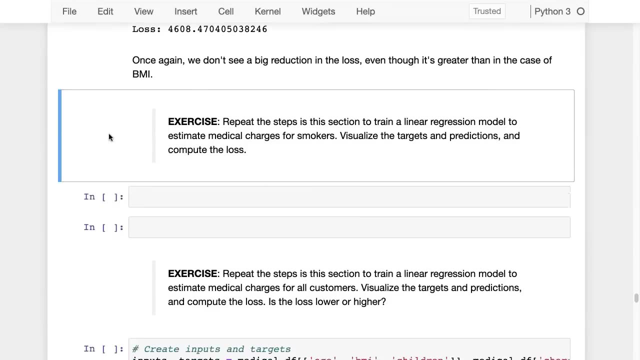 So we, on average, like the loss reduced by $50.. That's better than nothing And this increases definite. This change is definitely greater than in the case of BMI. Okay, So now an exercise for you is to repeat the steps in this section to train a linear regression model to estimate medical charges for smokers. 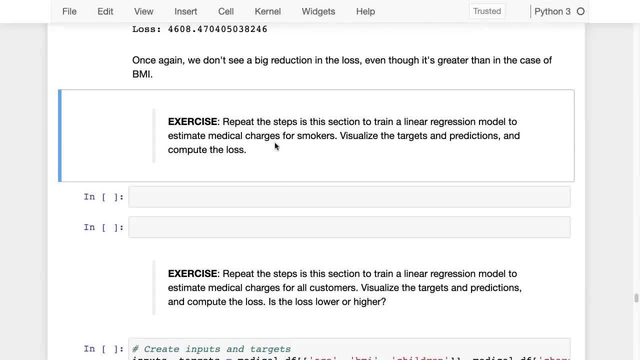 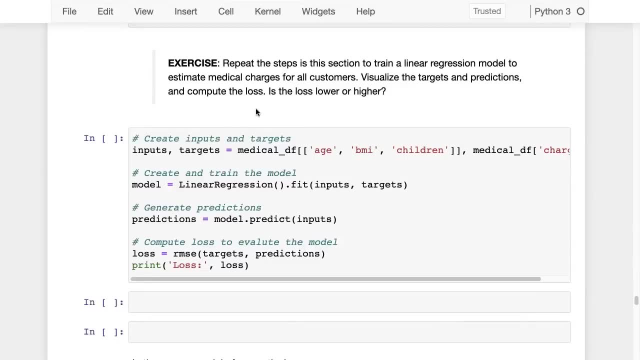 So use all the numeric Columns and visualize the targets and predictions to compute the laws. And here's another thing we can do. this time Let's consider the entire dataset. Let's maybe ignore the distinction between smokers and non-smokers and see if we can still fit a line. 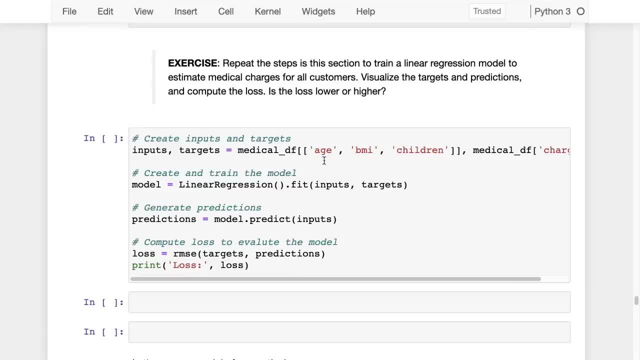 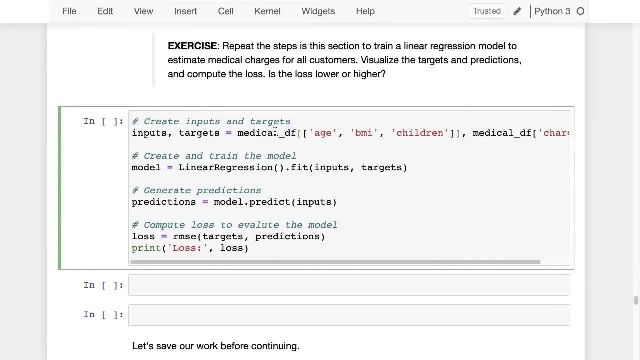 So we now repeat the steps in the section to train a linear regression model on the entire dataset. So all I'm changing here is now, instead of using non-smoker DF, I'm going to use medical DF, which is the entire dataset consisting of smokers. 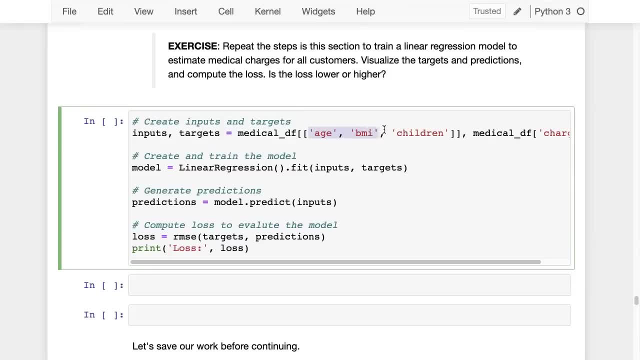 and non-smokers. I'm going to consider age, BMI and children as the inputs And I'm going to consider charges as the target. I'm going to pass the inputs, which is a now a 2d tensor, and it has, which has three columns of data, and the targets. 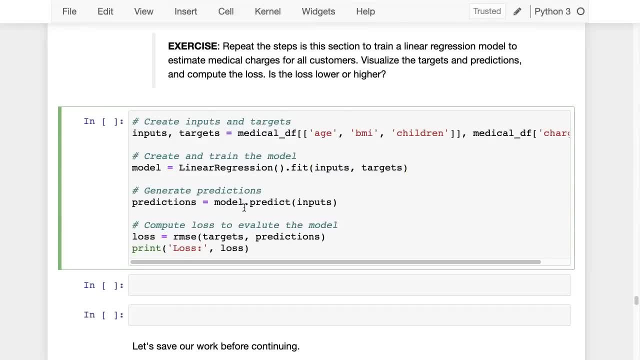 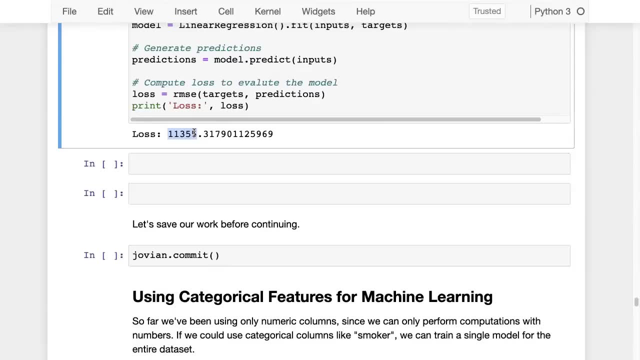 which is simply a series or a array of numbers. I'm going to make some predictions and I'm going to compute the loss. And the loss is much higher. It is 11,355 on average and you can probably tell why we know already or when we do PX dot. 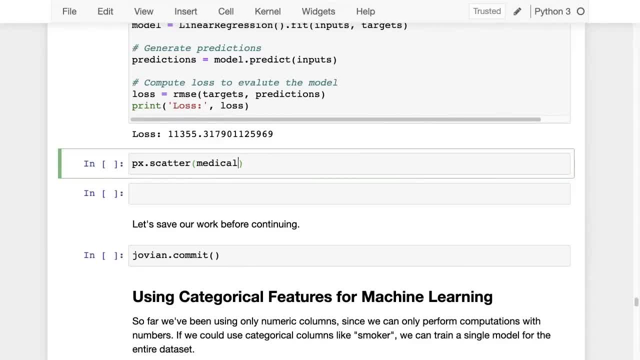 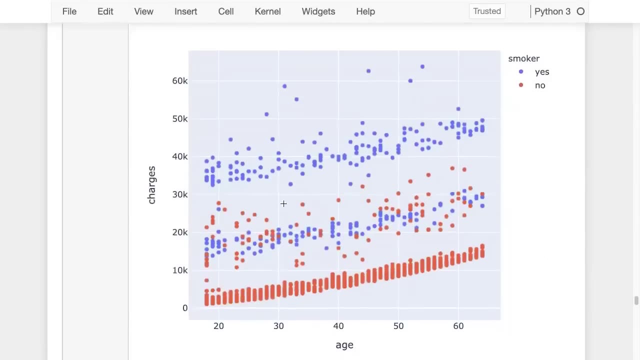 scatter between medical DF. and you said X as age, let's say, and Y as charges, and you said color: a smoker. you know that all this data was not there earlier, when we were just dealing with non-smokers, when we were dealing with. 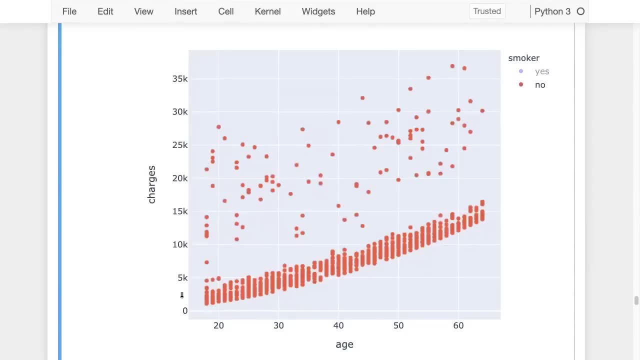 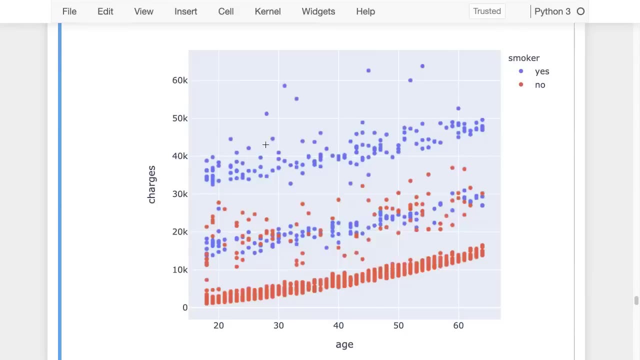 non-smokers. we were just looking at this, Which is obviously much easier to fit than this, like here. where do you put the line? You put the line somewhere here. That's going to increase the error with these. That's going to also have a higher with these And these are like really far away. 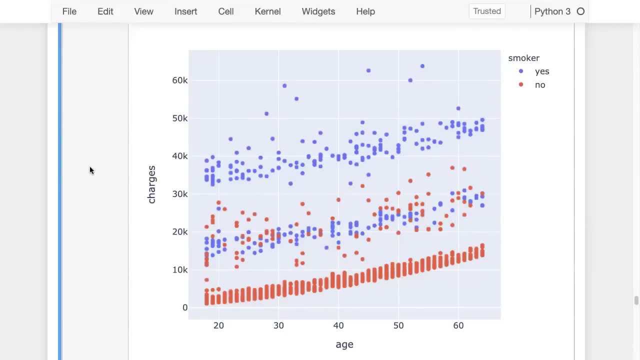 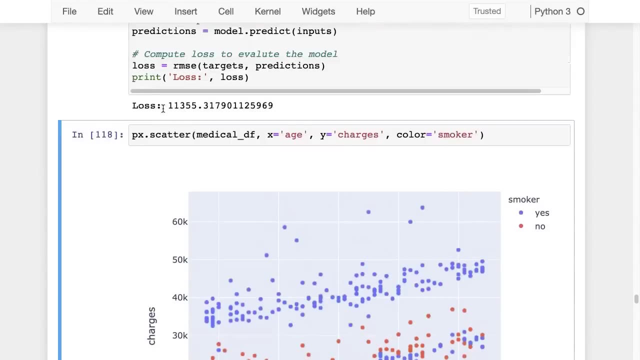 These are quite far away from this line here. So obviously your loss is going to become quite high, Probably completely. your model is completely useless at this point because most of the values you're trying to predict are in this range of five- 6,000.. And if you're off by 11,000, then that doesn't. 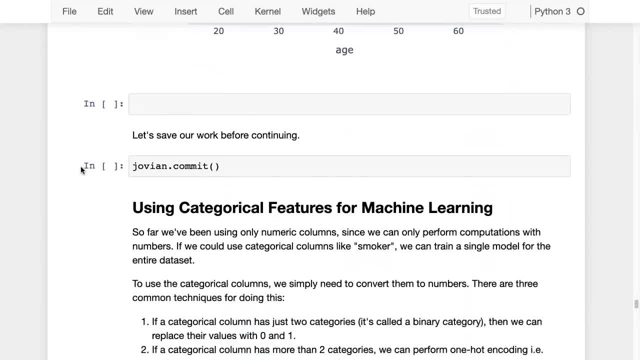 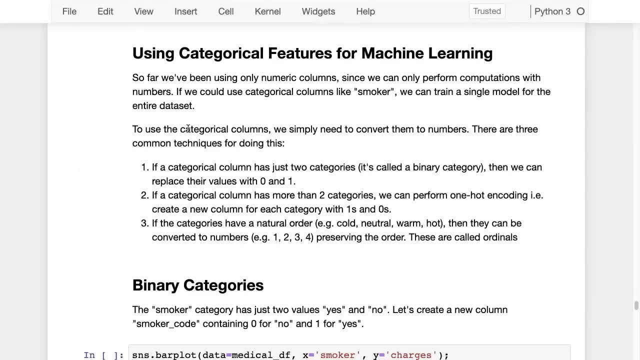 really make sense at all. So the next thing that you might want to do is to start using the categorical features for machine learning as well. Now, so far, we've only been using numeric columns, because we can only perform the computations with numbers. 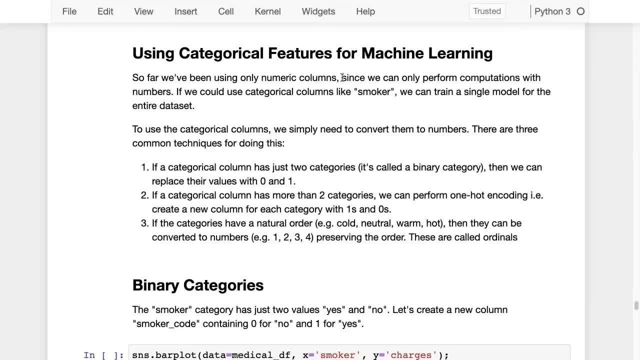 Remember the computation of the loss, the optimization, that is again using calculus and linear algebra. So all of that can only be done with numbers. Now, if we could use categorical columns like smoker, then it would be possible to maybe train a single model for the entire data. 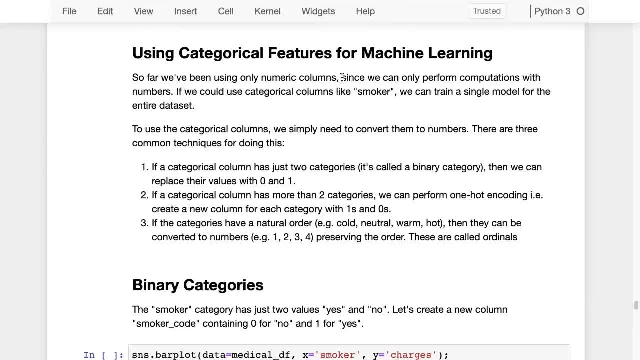 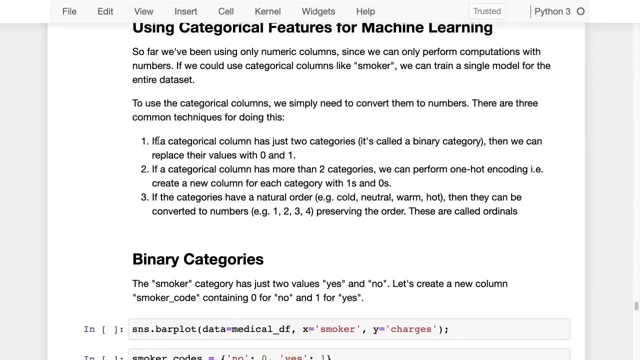 Set which can also account for smokers in some fashion. or to use the categorical columns, One trick is to simply convert them into numbers, And there are three common techniques for converting categorical columns into numbers. The first one is if a categorical column has just two categories, let's say smoker, non-smoker, yes, no. 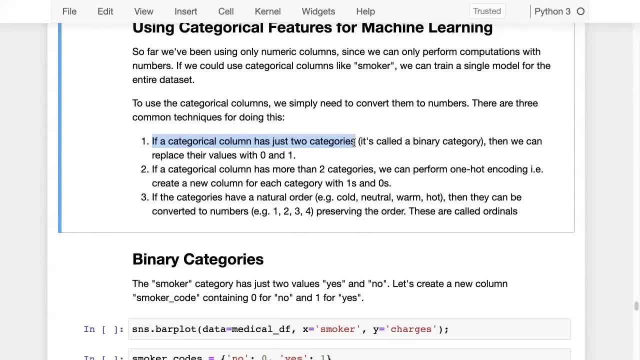 Then it's called a binary category. It simply indicates the presence or absence of something. In Such a case we can replace the values with zero and one, We can replace no with zero and we can replace yes with one. So now a weight would apply when we have a smoker. 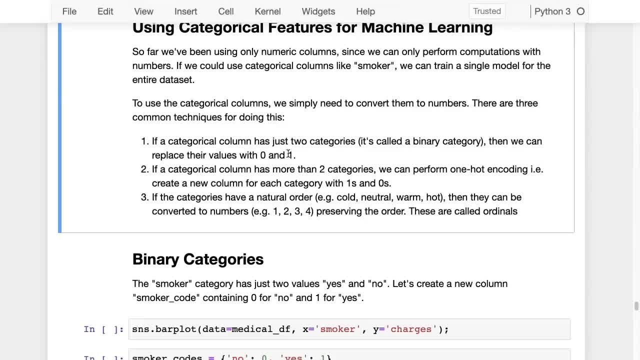 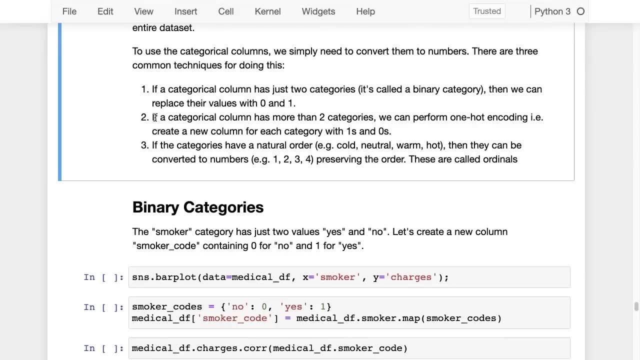 And when the when the person is not a smoker, then that weight would simply not apply, right? So there's a certain term that gets added. It's like a penalty that we're adding for a person is a smoker or not. Then another way to go about it is if a categorical column has more than two categories, for example the. 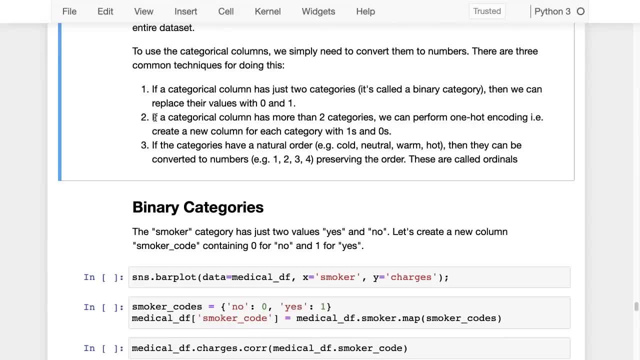 region, Then we can perform a one hot encoding, which means that we perform a new. we create a new column for each Category in that region. So let's say, for the Northeast column- Northeast region- we create a category which contains ones and zeros. 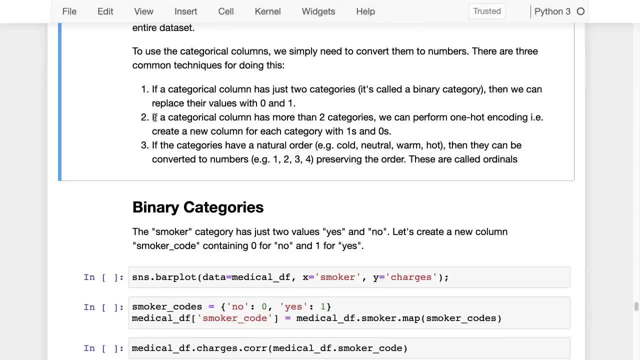 once at the places where the row belongs to the Northeast category. we can create a Northwest and Southeast and Southwest. So we create these four categories. Each of them contain numbers, and then we can ignore the original region column. So each of these columns not Northwest, Northeast. 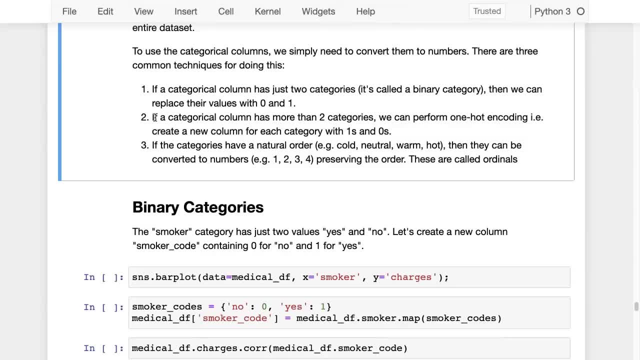 Southwest, Southeast, will contain zeros and ones, and every row will contain exactly a single one. So it'll contain three zeros and a single one, And that's where it is called one hot encoding. So that's why it's called one hot encoding. 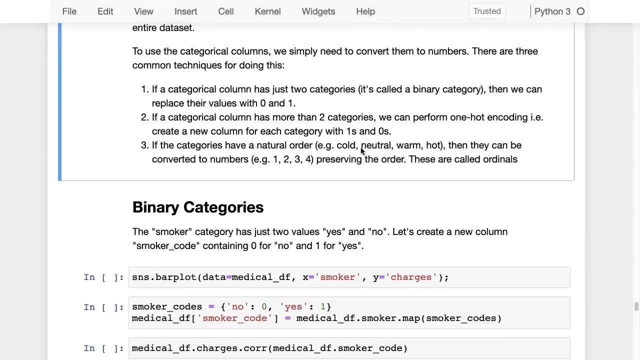 Okay. Next, if the categories have a natural order- So sometimes You may have a natural order like this: cold, neutral, warm, hot- Then they can be converted into numbers like one, two, three, four, while still preserving the order. 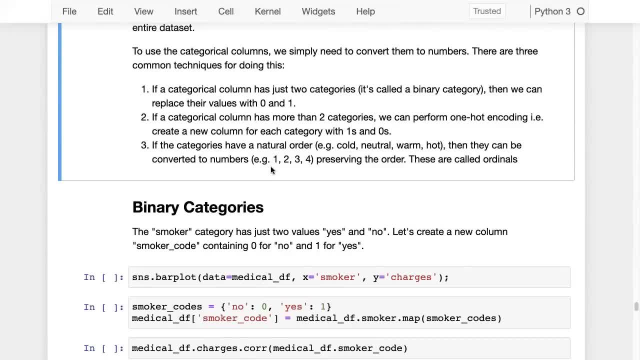 So it's possible- not in this problem but in some other problem- that cold, neutral, warm, hot are indications of temperature And there is actually a linear relationship between what you're trying to predict and the temperature. So in such a case it may make sense to convert them into numbers to preserve that order. 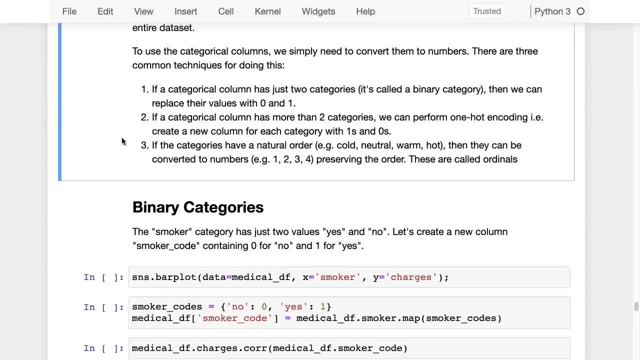 And in these cases they are called ordinance. So you will often have to Decide whether you want to convert certain categories into numbers or do you want to convert them into one hot? When should you convert them into numbers? When you see that there is a high correlation between these categories in their original order and the natural order and the target, then you should convert them into numbers. 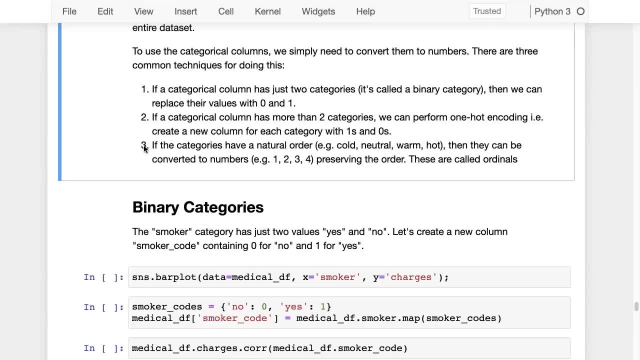 If you do not see a correlation, if you see things go up and down like region for example, there's no clear region. There's no clear reason why region should have some kind of an order in determining How much, what kind of charges, you have. 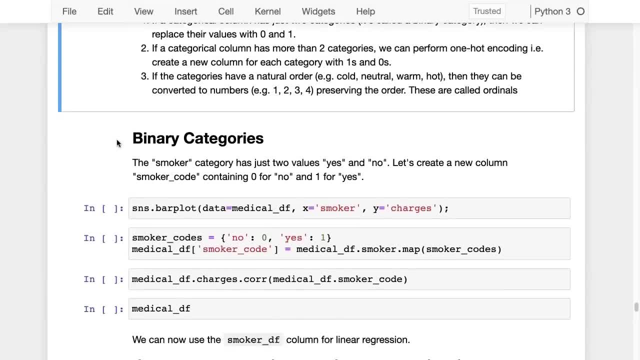 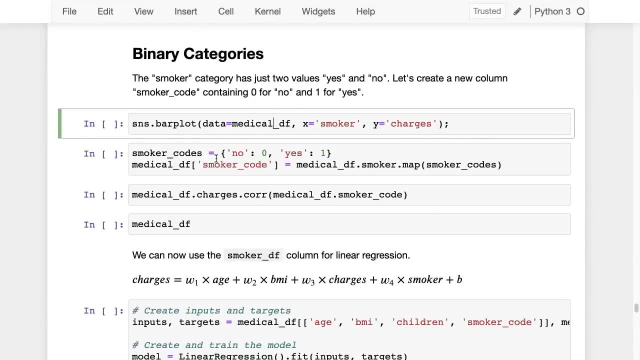 So you can just convert them into one hot or encoded columns. Okay, So let's start with the smoker column. We are going to convert the smoker column into. we're going to add a new column called smoker code. So here, this is what the smoker column looks like. Smoker versus charges. So on average, for the charges for smokers are close to 35,000 or 32,000, the medical charges that's the mean. But that's because you have a lot of outliers, right, So do not. this does not really convey the full picture, but at least it. 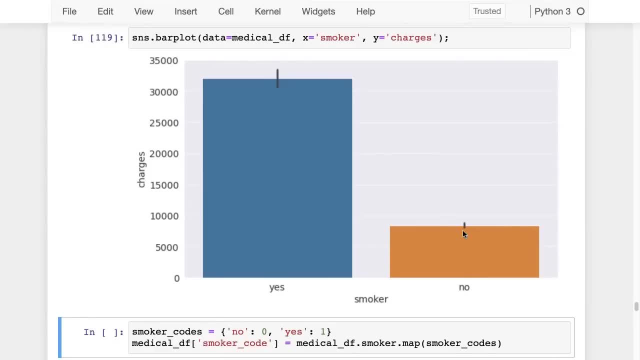 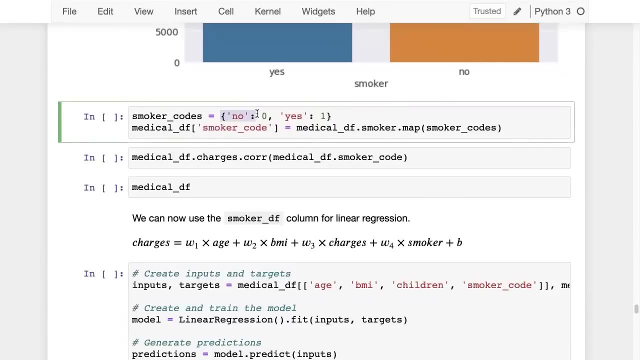 tells us that the average is 32,000.. And here, for non-smokers, the average is more around six, 7,000.. So now we are going to create two codes, no and yes, And we store these, and we store these in a map and we call medical. 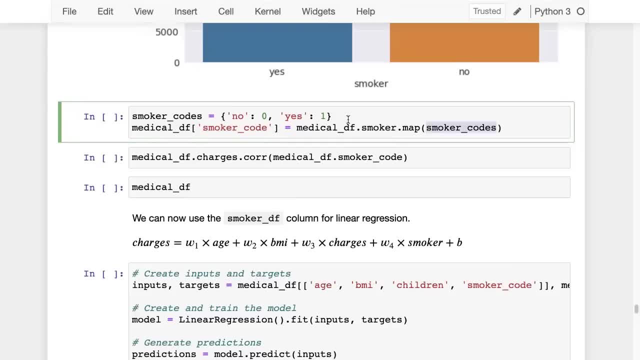 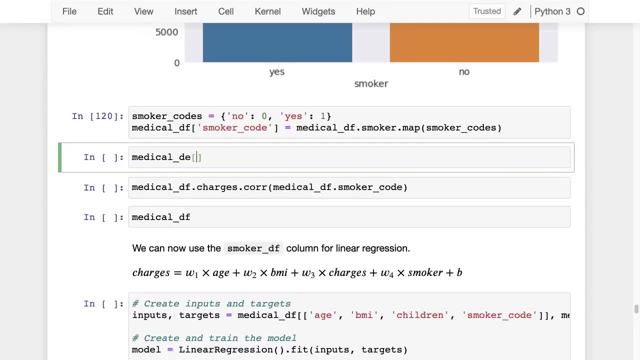 dfsmokermap and then we pass in this dictionary here. So what this is going to do is this going to replace all the no values with zero and yes values with one. So now we have smoker codes. You can check medical DF and maybe the allergies checks medical DF and you see. 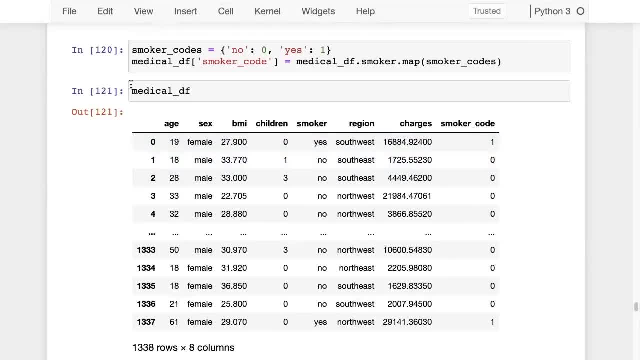 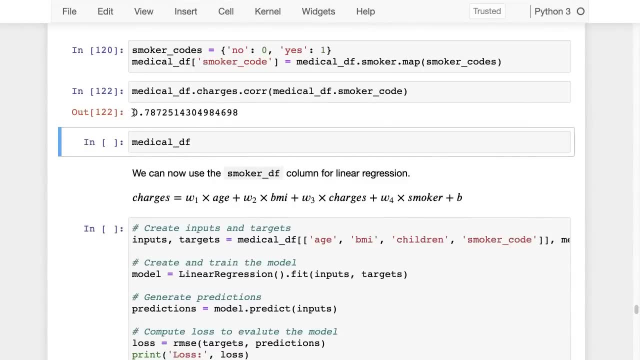 smoker. you have smoker yes, Smoker code one, smoker no, smoker code zero. And we can check the correlation now between charges and smoker code And it seems like the correlation is quite high, 0.787.. And so now we can just use the smoker. 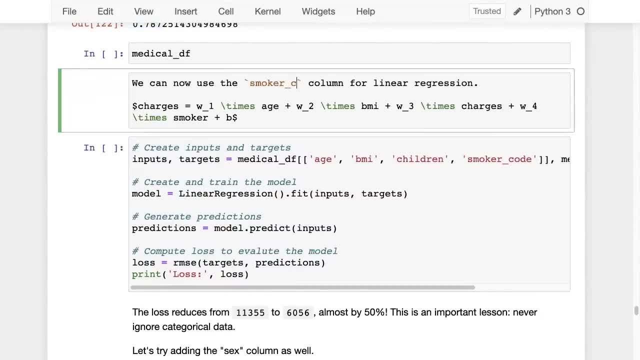 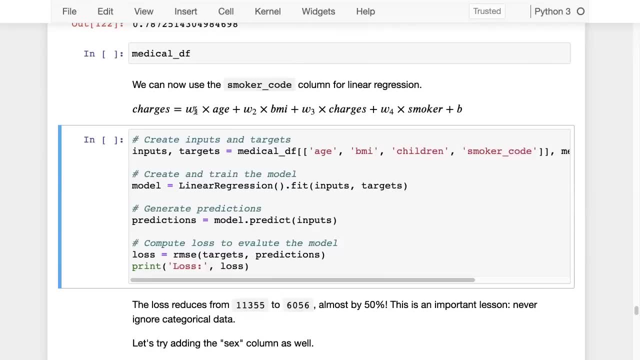 Code column, they should say smoker code. So we can now just use the smoker code column for linear regression. We say: charges equals the weight W one times age, w two times BMI, w three times charges, w four times smoker, w plus B. So HBMI, children's smoker code, the number and the rest of 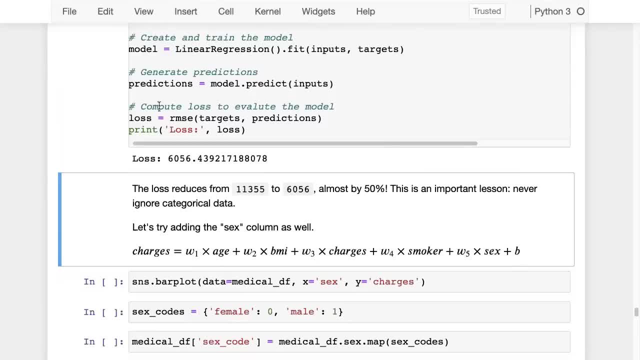 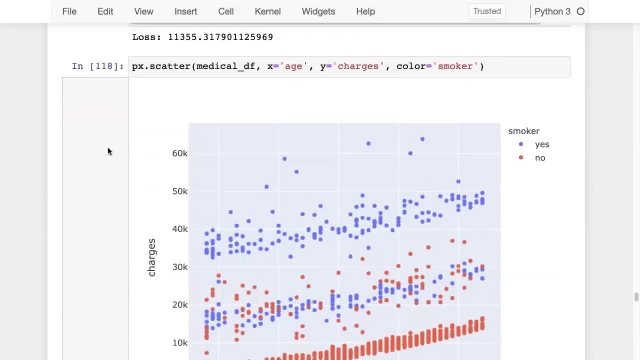 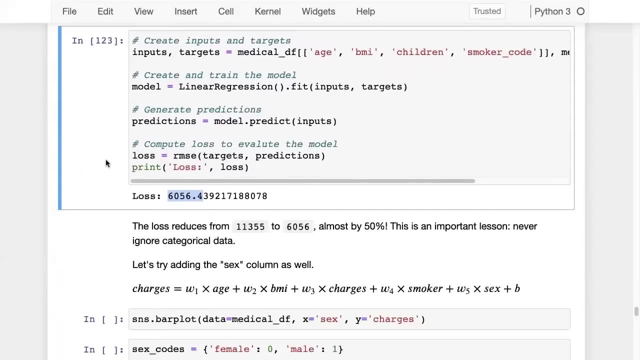 the code is exactly the same grade, So we end up with a loss of 6056.. That's all Most of 50% reduction in laws. We've gone from what's that? 11,000.. The on average being off by 11,000 to on average is being off by 6,000.. 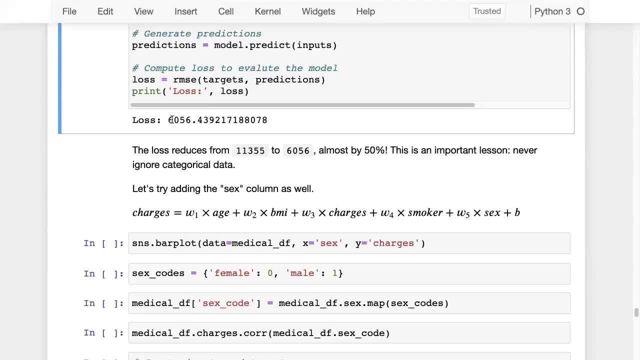 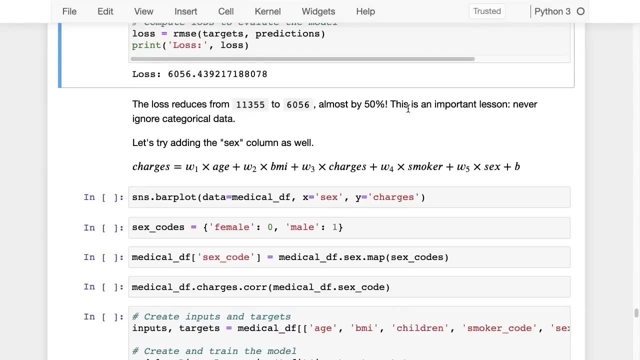 That's not as good as we had just for non-smokers, but still it's better. It's better by 50% from the previous value. So that's an important lesson: Never ignore categorical data. It may be a deciding factor in what makes your model good. 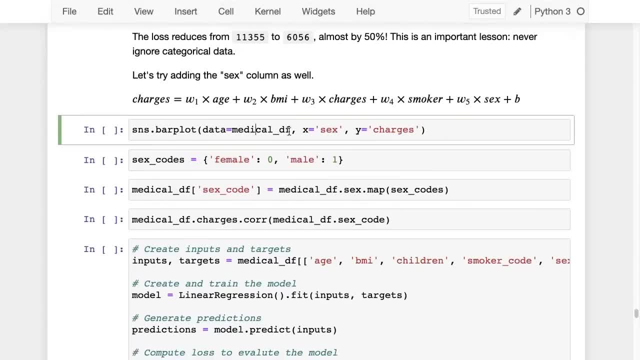 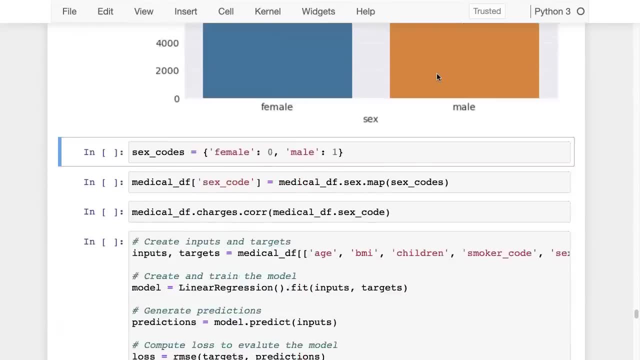 Let's try adding the sex column In as well. So we're going to do the same thing. If you see, here it turns out that for females the average is slightly lower than males. So I'm just going to put zero for female and one for male as a sex code. 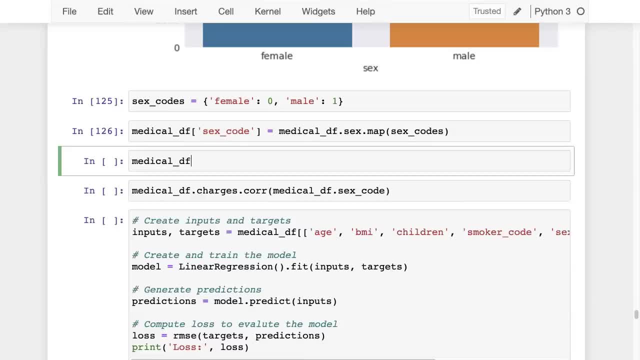 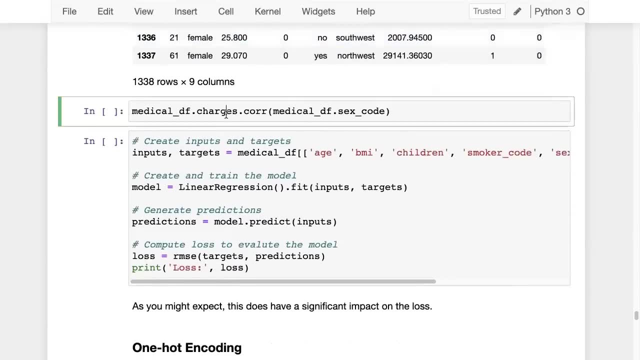 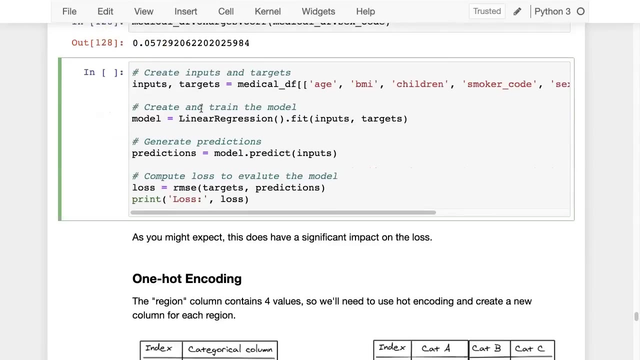 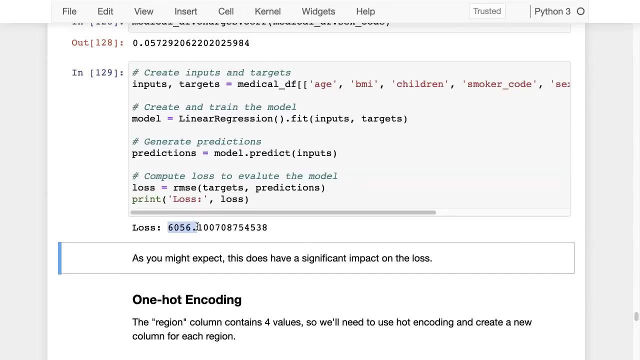 And we have medical DF here You can see where we have female we get zero, where we have male we get one. And let's check the correlation. So the correlation is very Hardly anything. So we can run the process again: age, PMI, children's smoker code, sex code, and you can see there's no real change. 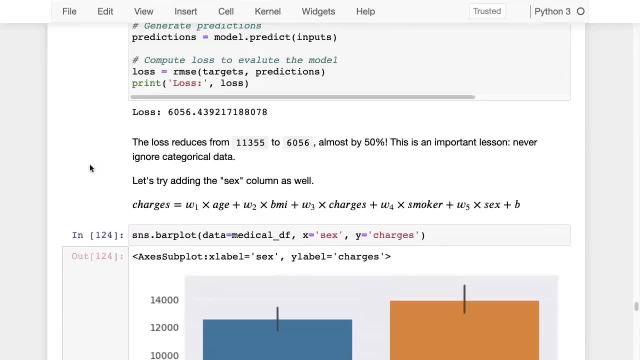 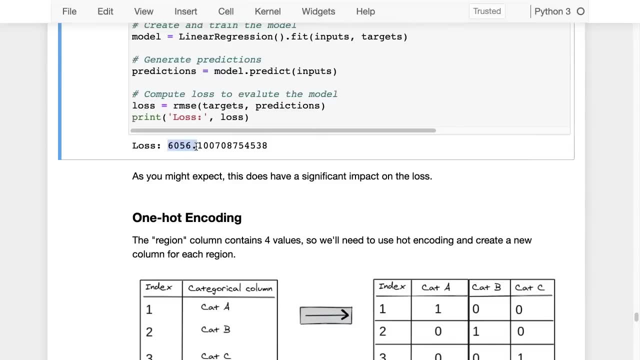 It goes to 6 0 5 6 from what was the previous value: 6 0 5 6, 0.4. 3 2, 6 0, 0.6, 0.1 0 0.. So hardly any change. even what? whatever changes, there is less than a dollar on average. 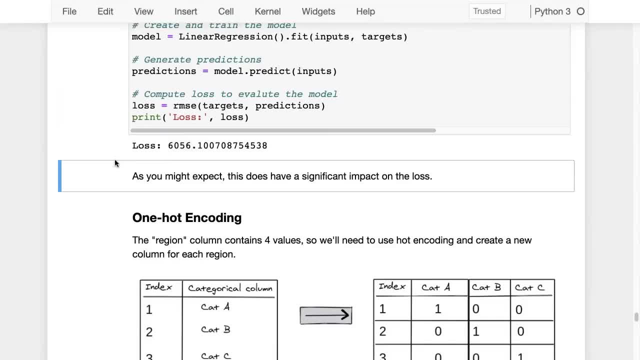 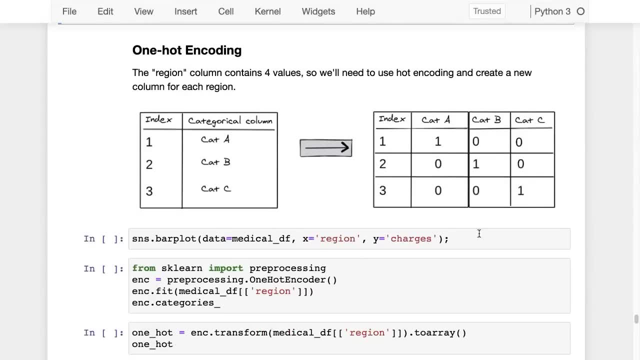 So it's not really important. We can maybe even ignore the sex column All together. Next up, we have the region column. The region column contains four values, and that's why we'll need to use one hot encoding to create a new column for each region. 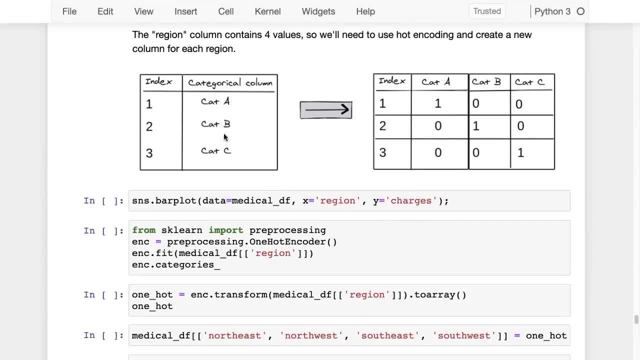 Here's what we want to do: instead of like Northeast, Northwest, Southeast in the same column, we want to create a column for Northeast and put ones and zeros there. create a column for Northwest, put ones and zeros. Create a column for North uh for Southwest, and put ones and zeros. 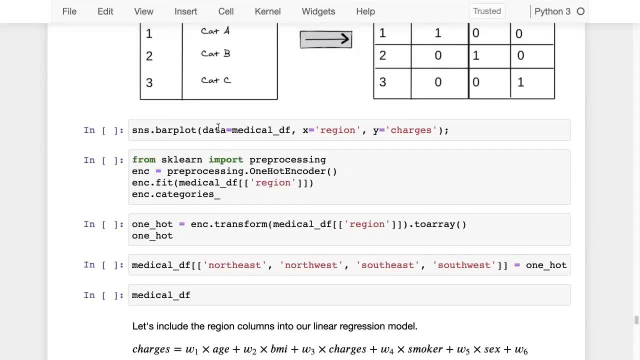 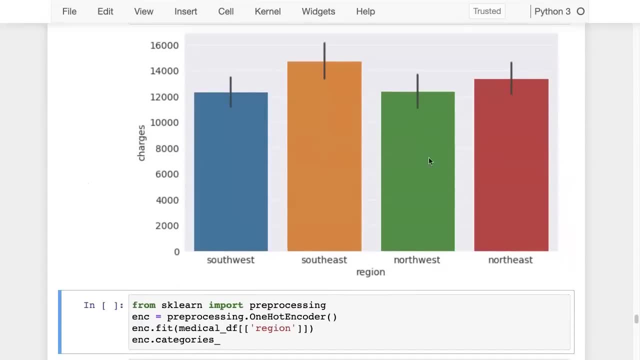 There is a way to do this in scikit-learn And I typically just look it up and this, this process is called one hot encoding, So I typically just look up an example. So here again, if you see that there is a difference by region, so maybe region is a factor. maybe different regions, based on different average incomes, have different medical costs at different hospitals. 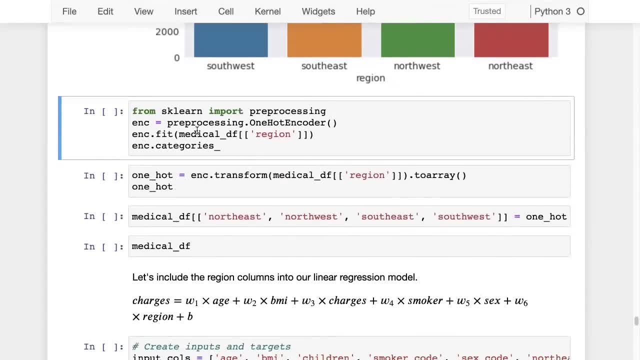 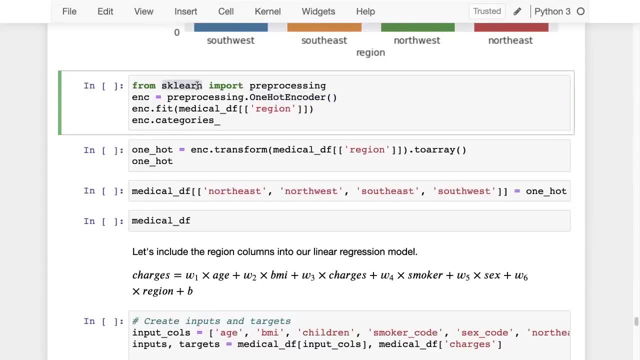 So maybe region is a factor, so we should include it. So the way you add one hot encoder Encode this data is you use this one hot encoder class from scikit-learn dot pre-processing. So from a skill on we import pre-processing and then we use pre-processing or one hot encoder. 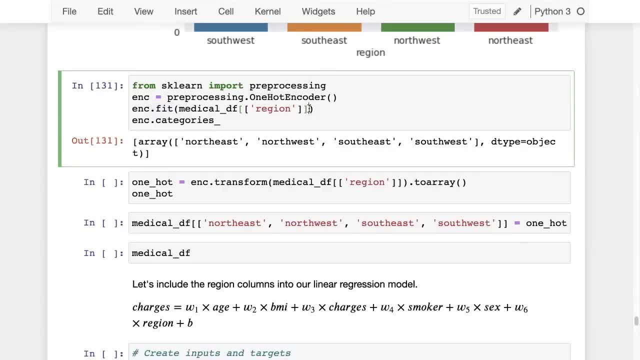 And we just call on the encoder, We call, we give it the list of regions and it's simply going to identify the list of regions It's called fit here. but it's really all it's going to do is it's going to find that there are four different values: Northeast, Northwest, Southeast, Southwest. 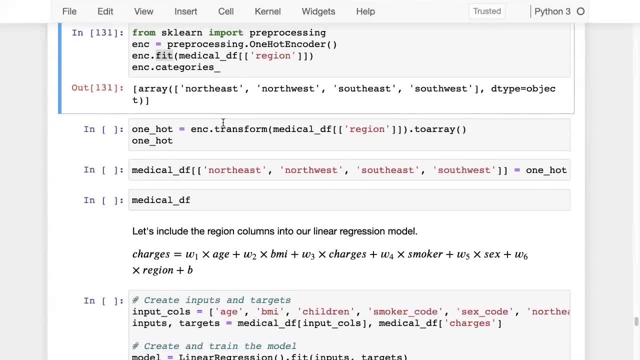 Okay, So it has identified these values. Now we can give it some input and this could be our original imports or this could be something that we want to test out later, So we can give it some input. Let's say we want to, we have not. we have the Northeast region. 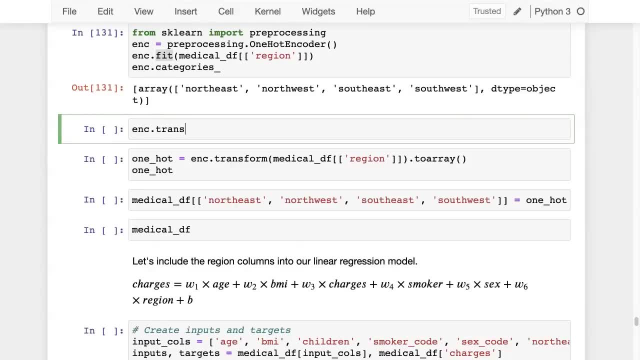 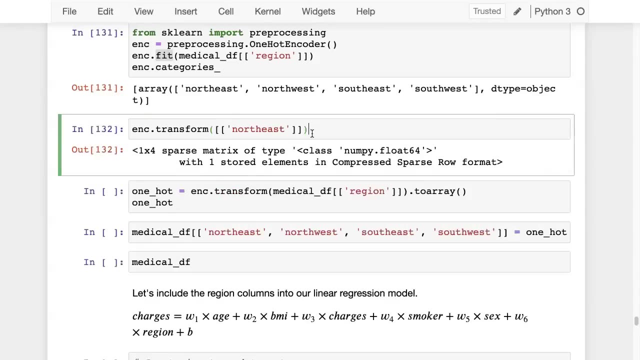 So let's say we, we give it ENC, dot transform and we need to give it the Northeast region. So let me just give in Northeast as the input And it's going to convert Northeast into. I need to call two array here to actually see the values. 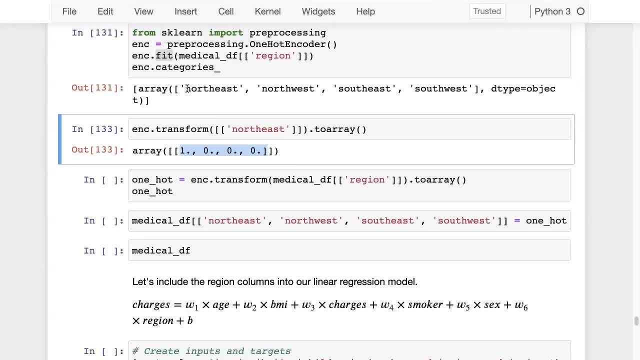 So it's going to convert Northeast into one zero, zero, zero. So for Northeast, which is the first category, it's going to create a one. for the rest of the categories, That's going to have a zero. Let's maybe give it to call two rows of data. 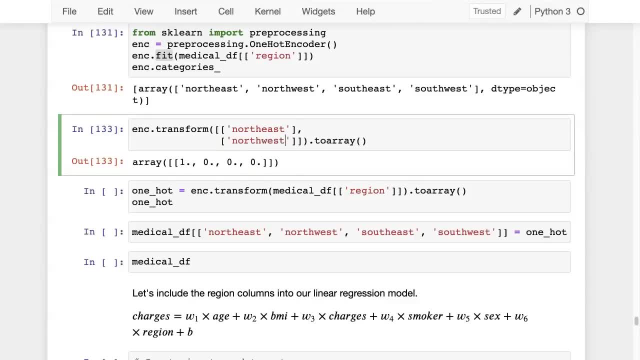 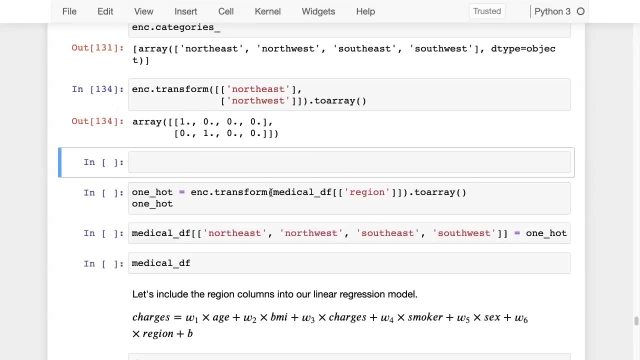 So this time we give it Northeast and Northwest. So one zero, zero, zero, zero, zero, one zero. Right now, what we can do is we can take this, The original regions from our data frame, which are Southwest, Southeast, Southeast, et cetera. 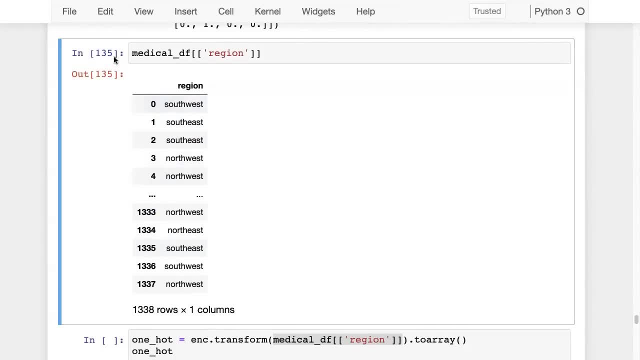 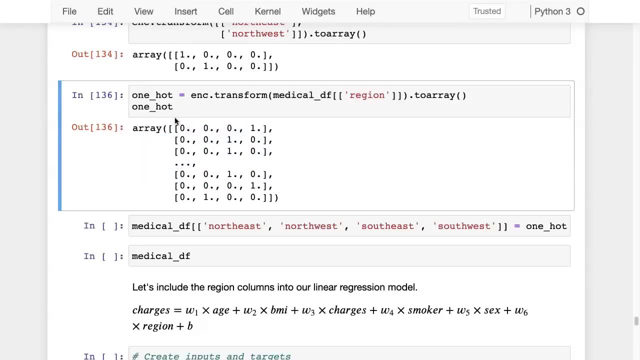 Those are, this is the region per customer, and we can put that into encoded or transform and that's going to give us this kind of data. So now we have this column for Northeast, this column for Northwest, this column for Southeast and this column for Southwest right. 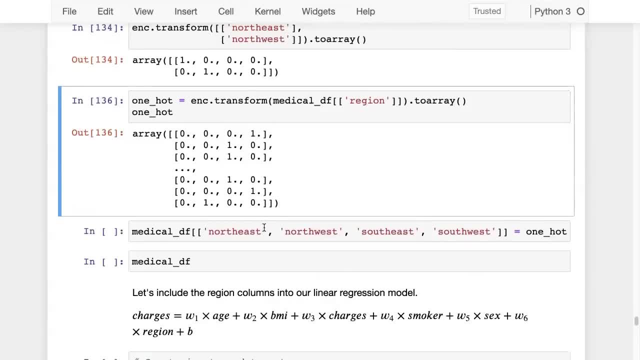 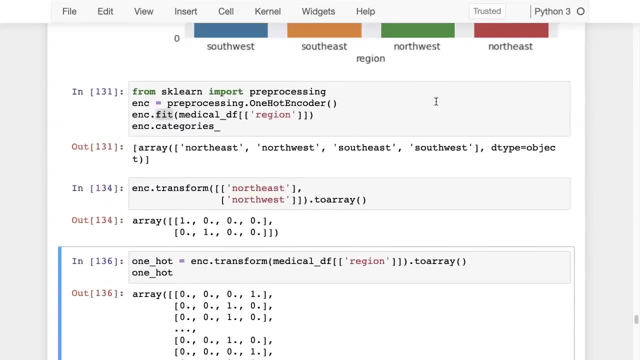 All this is doing is this process: taking a categorical column and giving us one hot vectors, And then we're going to do the same thing for the rest of the categories. So we're going to give it this column for Northeast, this column for Northwest, this column for Southeast and this column for Southwest right. 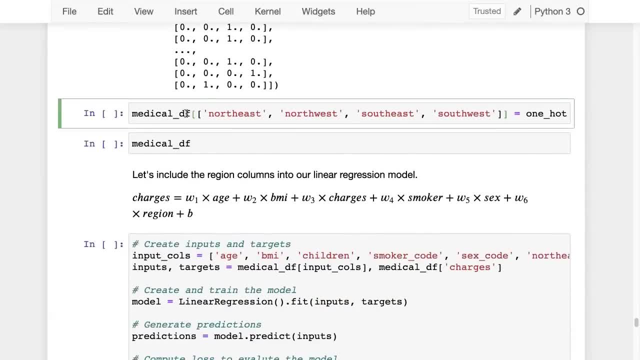 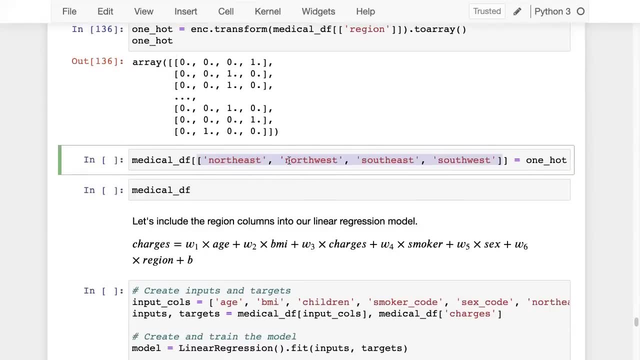 And then we can insert it back into the data frame by saying that in medical DF we want to create four new columns. So still remember, it's not part of the data frame yet. So in medical DF we want to create four more columns and we want to give it this data, one hot. 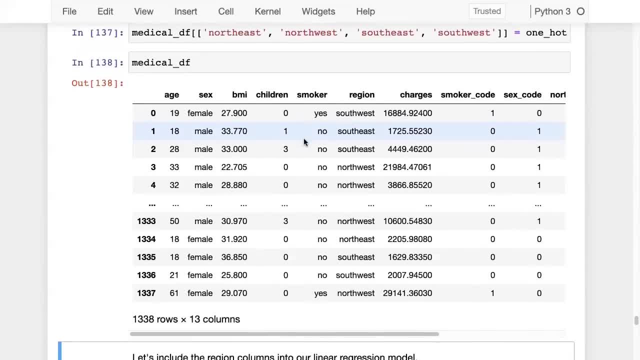 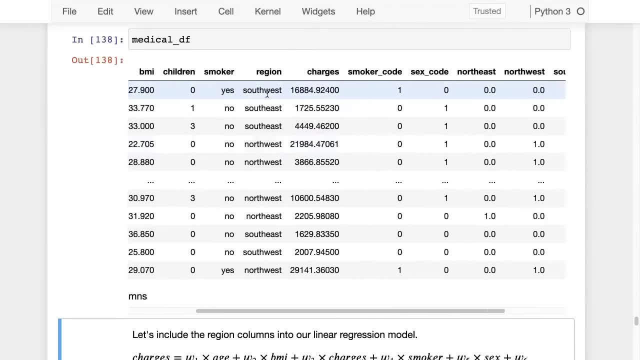 Okay, So here, after doing all of that- and you don't need to actually remember any of that, You can always look that up- but after doing all of that, what we've been able to achieve is: we take the region column: Southwest, Southeast, Northwest. 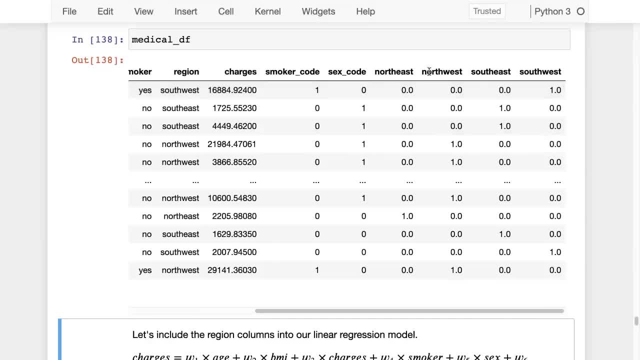 Northeast and we have replaced them with these four columns: Northeast, Northwest, Southeast, Southwest. I've still kept these around. I've not removed these- just so that we can see and make sure things are working properly. And now we can include region into our model as well. 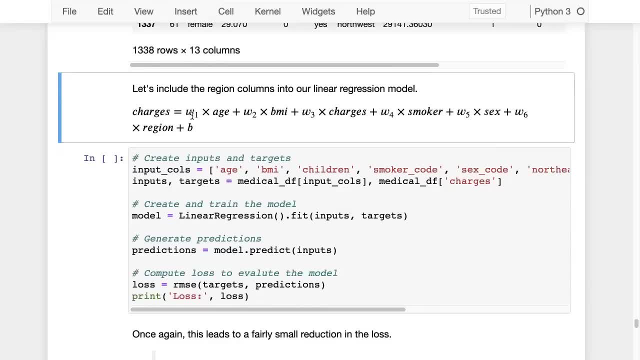 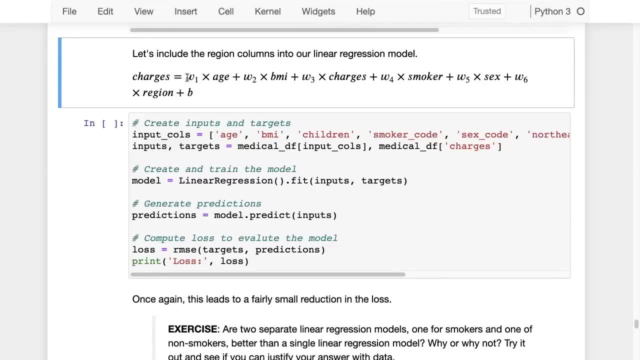 So we have w one times age plus w two times BMI, plus w three times charges, plus w four times smoker, w five times sex, w six times region plus B. So the idea here is: once you understand linear regression with one variable and you 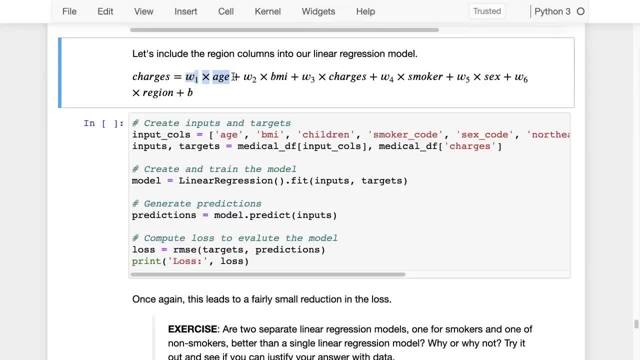 Really understand it. well, if you internalize how it works, then all of this is really. it's a very simple extension. You don't even have to change any of the code. but all you want to understand is that when you're working with one variable, you're trying to fit a line and you start out with a random line and you move the line around. 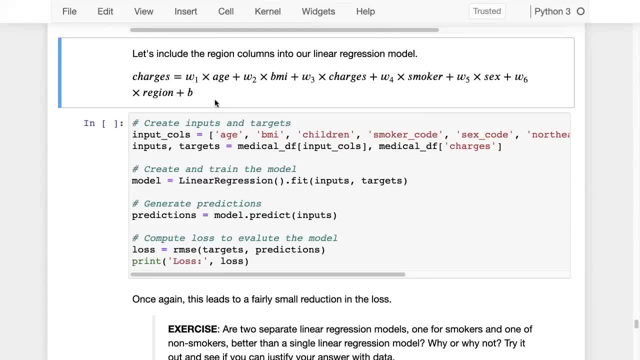 You use the loss function to find out how bad the line is and you then use an optimizer to slowly improve the line and move the line around till it fits the data to the best extent possible, which is to minimize The loss right. 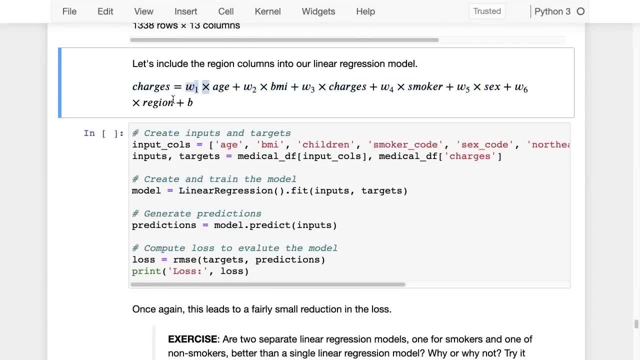 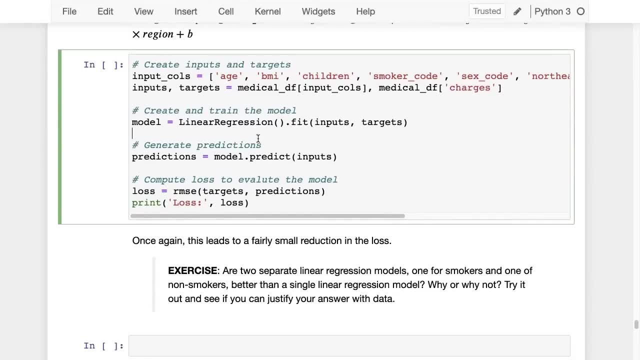 And then you simply have to extend it mathematically into a bunch of other, into a bunch of other dimensions. So now we're no longer dealing with one feature, We're dealing with six, but the code is exactly the same. So there you go. 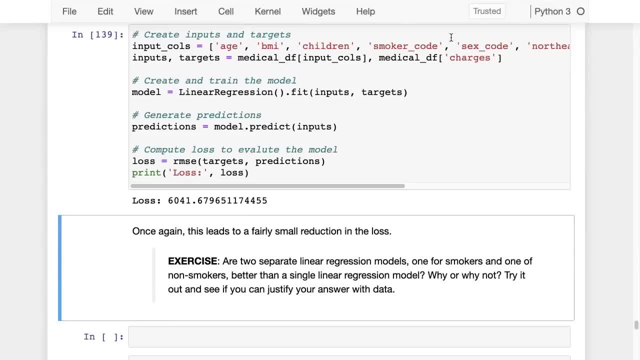 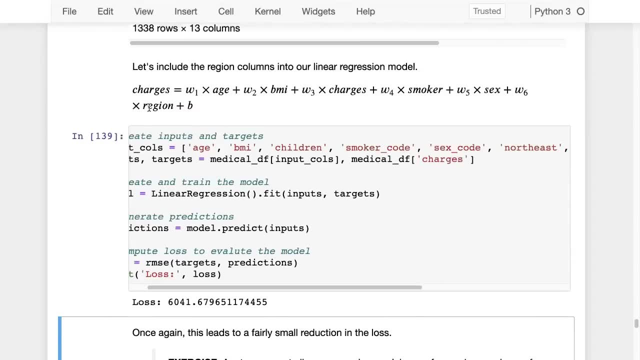 Now we have the inputs, all six. Oh, that's a lot of columns actually. age BMI: children's smoker code. Well, to be honest, this is not correct. Exactly This is. there should be like a w six, w seven, w eight, w. 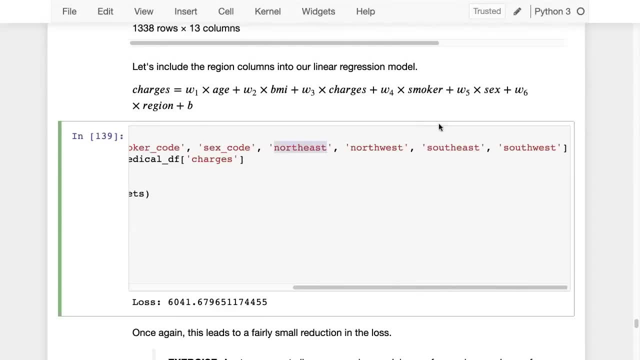 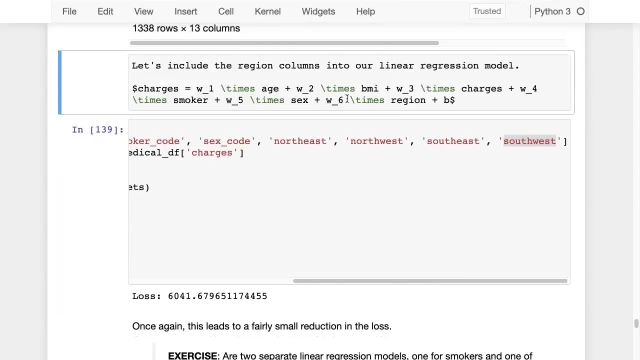 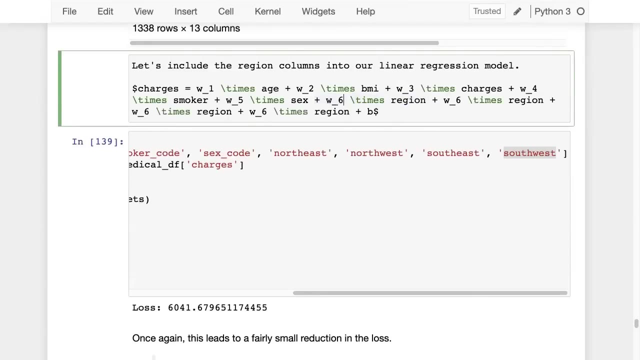 No, Nine, right. So w six times Northeast, w seven times Northwest, w eight times Southeast, w nine times Southwest. So there are four weights here. So I should actually correct This, should probably take that and then put that here and let's make that w six times, and Northeast will take the value zero or one, and then North Northwest will take the value zero or one, and then 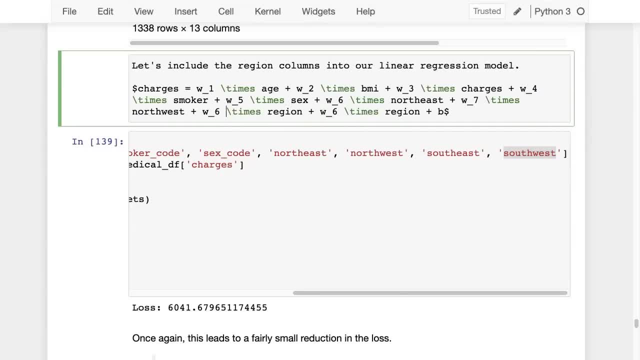 Southeast will take the value zero and one, So which is w seven and you have Southeast, And finally you have w eight applied to Southwest, or sorry, w eight and w nine. So for every region we're actually applying a different weight altogether. 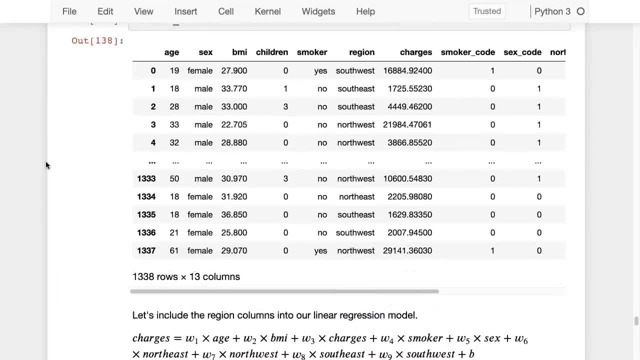 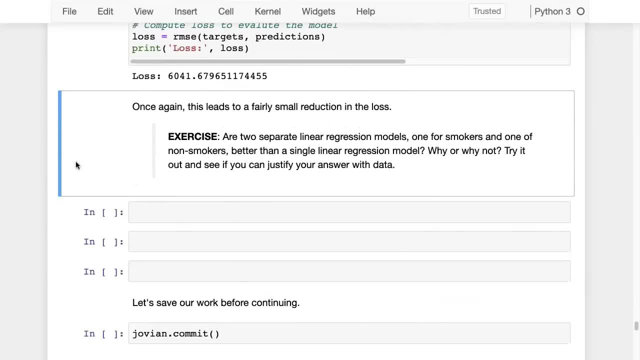 And there you go. Now The loss reduces slightly more to 6 0 4 1.. Where did we have it earlier? Let's see 6 0 5, 6, 6 0 4 1.. So about a $10 decrease, and you can already see that a lot of these other factors are not really helping. It seems like age and children, and maybe just age and a smoker. Those were the two biggest factors, and the rest of them don't really matter. Maybe they give you a 1% difference, but not so much. Now here's an exercise for you. 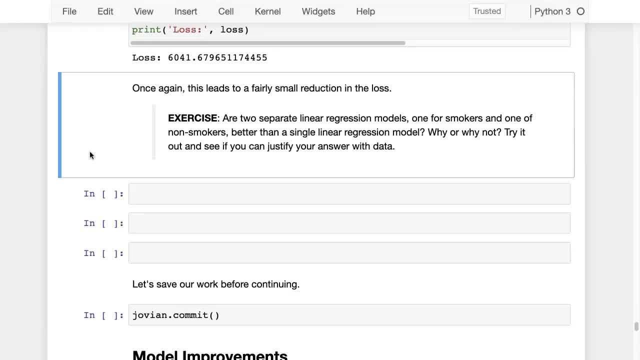 To try and figure out if one linear regression model actually makes sense for this entire data, because, as we already saw, just with the distribution of age, this data is not linear. There is a trend, but it's not linear in any sense. 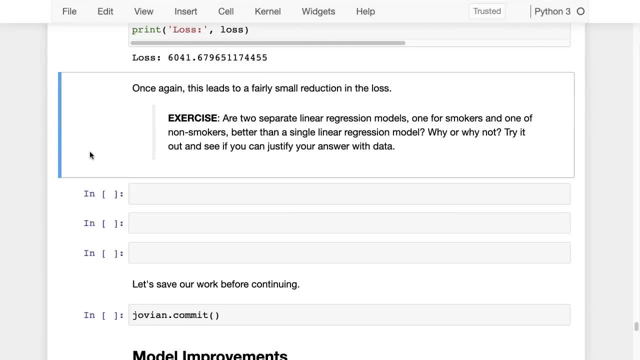 At the very least, if we want to have some sort of a linear relationship, we should set, we should, we should take into consideration the smoker column and the way we have taken into consideration right now the smoker column is by giving a weight to whether this person is smoker or not. 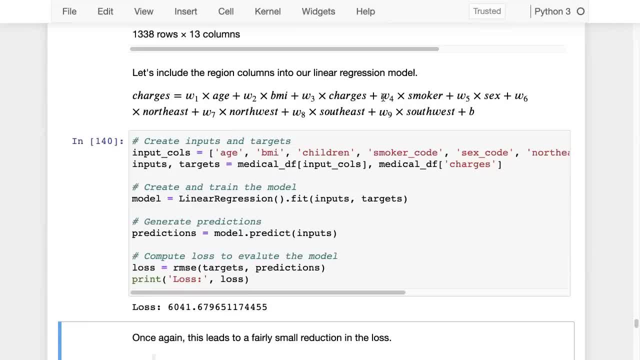 So we are kind of adding a smoker penalty here, that if smoker is one, then this weight gets added to the charges. If smoker is zero, this weight does not get added to the charges. but based on whether the person is a smoker or not, we are not really changing any of the other weights. 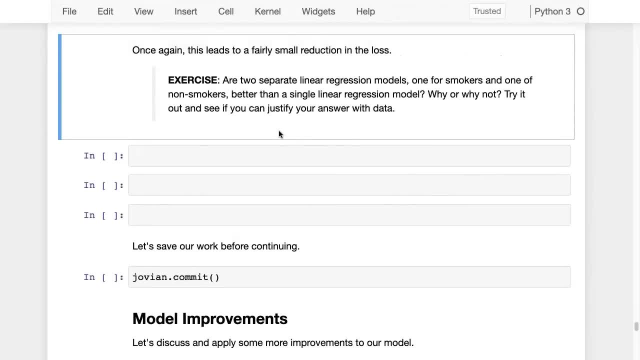 So here's what one thing you can try out: are two separate linear regression models, one for smokers and one for non-smokers, better than once in single linear regression model? And what does better mean? I let you think about that. So try it. try creating two separate linear regression models and use all the other parameters with normal weights. 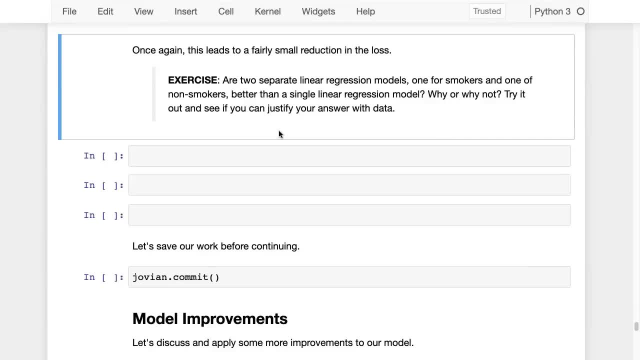 Just include smokers or just exclude smokers and create two separate models, one for smokers, one for non-smokers- and see if the losses for each of those models are lower on average. Let's say the losses for both those models are in the range of 3000 or 4,000.. 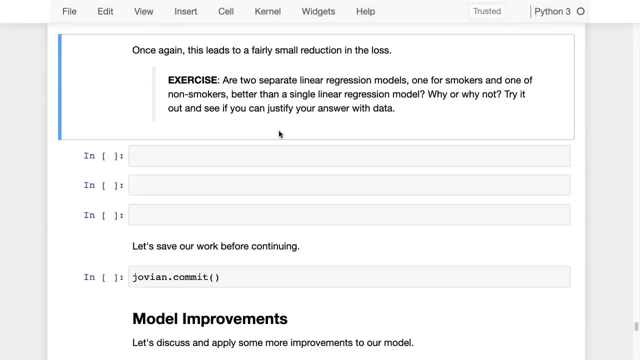 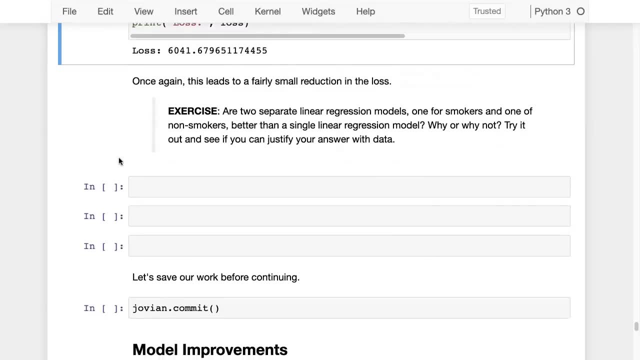 So that means you are better off using two models rather than using one linear regression model, And that's a decision that you will have to make as a data scientist. Should I be using one linear regression model? Does that make sense? Or maybe, based on whether these people are smokers or not, you need to have different linear regression models because the slopes of the lines are different. 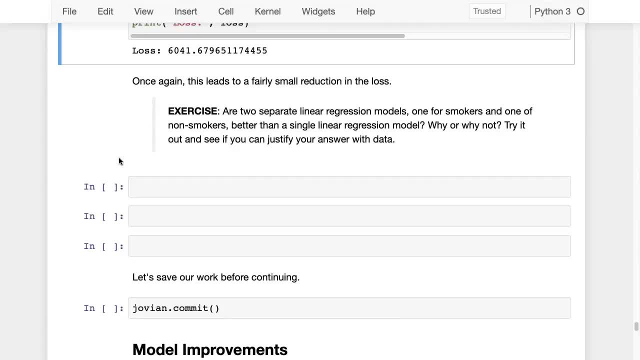 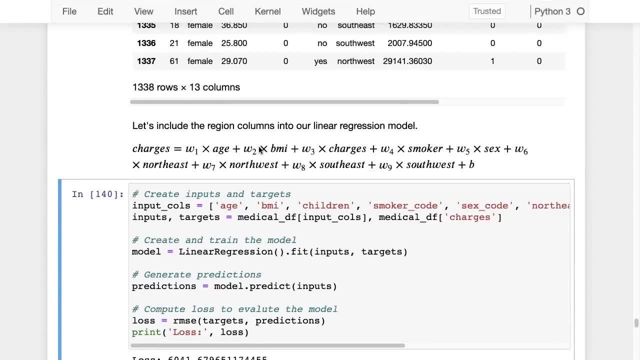 We know that, for example, BMI makes a big difference for smokers, but does not make a big difference for non-smokers. So right now we have imposed a single weight on BMI, but ideally the weight applied to BMI should really depend on whether the person is a smoker or not. 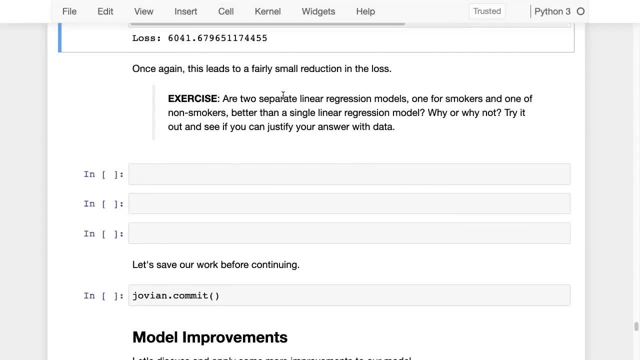 So all these factors have to be taken into consideration. Sometimes, two linear regression models based on our understanding of the data may be better than one, And this also kind of leads into something that we will cover in the coming weeks, which is about decision trees. 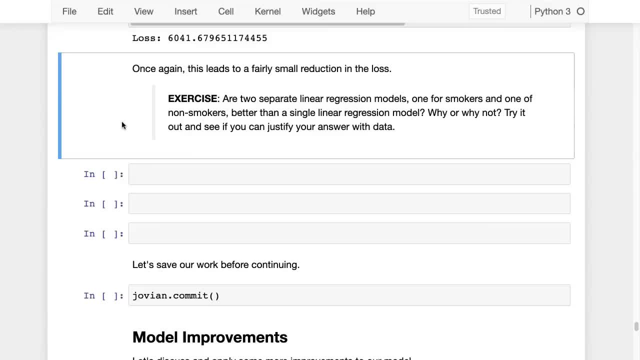 Sometimes you don't want to make a calculation just using just weights. Sometimes you want to use decisions. You want to see whether a person is a smoker or not, and then maybe you want to check the region- which region they're in- and then maybe you want to check something else. 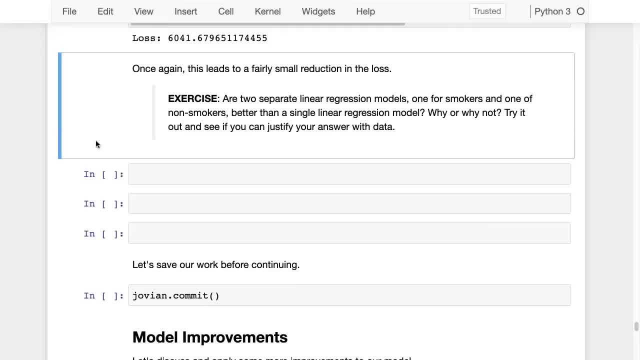 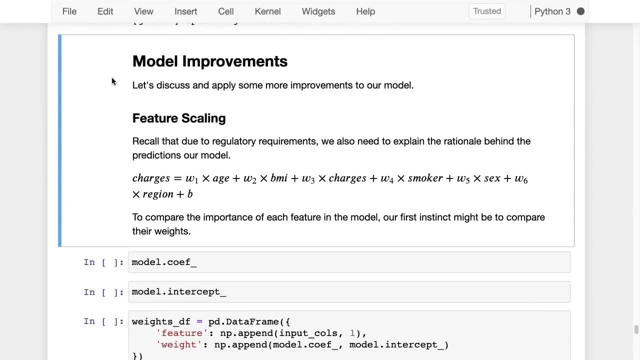 And then maybe you want to use some kind of an averaging technique. So we'll see how to mix some of these models as well as we go. So a couple of model improvements, And again there is some code involved here. I will not go too deep into the code. 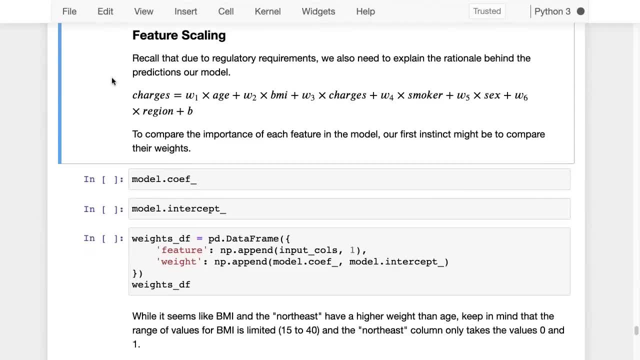 Now we are getting to the point where you should be able to read code yourself and figure out what it is doing. So I'm going to tell you what the idea here is, what we are going to do here, And then you need to go and figure out- where in the study hours or whenever you have the time- what this code means. 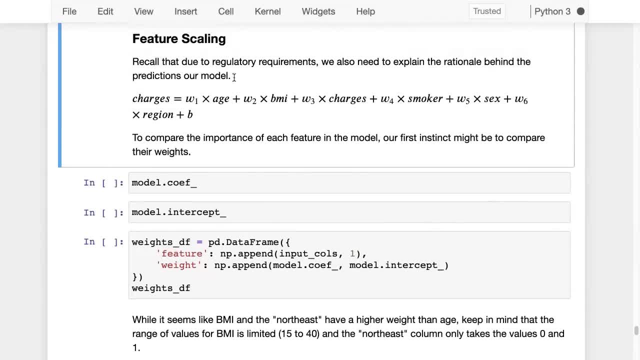 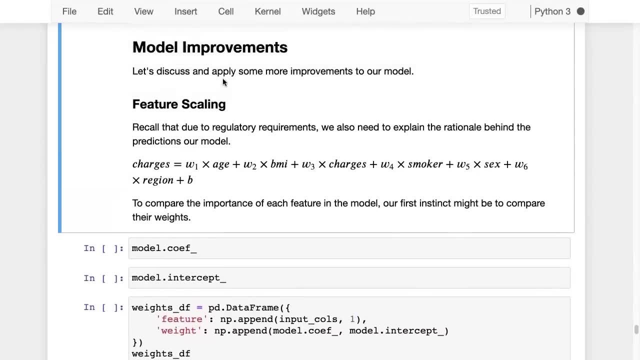 And it's simple code, not too difficult. So recall that, due to some regulatory requirements in Healthcare, we also need to explain the rationale behind the predictions on our model. So when we have a prediction, here's a model, right? Okay? 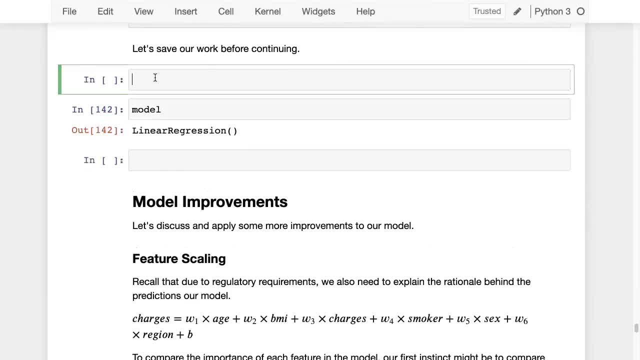 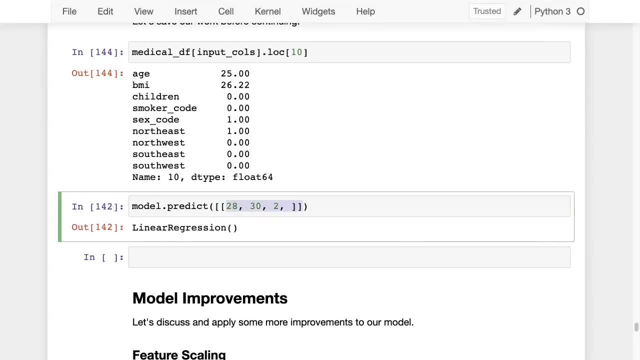 Now somebody walks in and they have a certain profile. So these are the input columns for that We look at in our model and let's try to create a sample input. So we take a person of age 28,, a new, a new applicant that has come in. 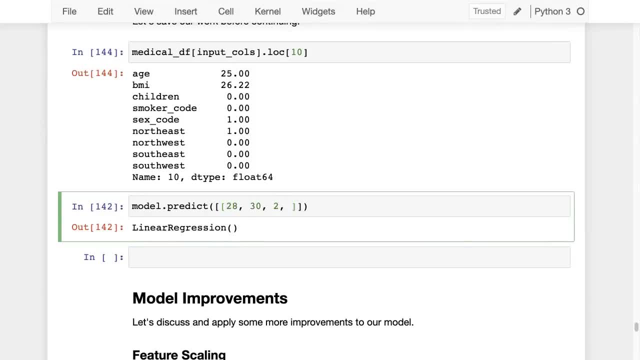 Maybe their BMI is 30. Maybe they have two children, Maybe they are a smoker, So they are a smoker, Code is one. Then they are female, So this is zero, and they belong to the Northwest region. So this is zero, one and zero and zero. 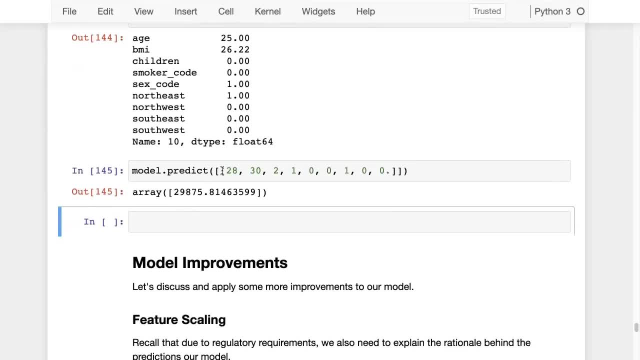 Okay, Now I'm going to predict. So we give this data, this one row of data, into our model and our model predicts that for this new applicant was coming, The estimated medical charges are to 29,875.. And then, using this, we charge a certain premium to the person. 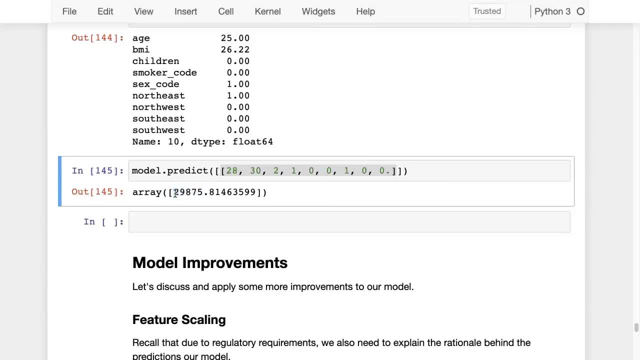 We also look at other Factors, but this is one of the major factors we look at. So now this person comes back to us and says: Hey, I would like to understand why you have quoted me this insurance premium. And then you tell them that, Hey, we predicted that your medical charges would be around $29,000. 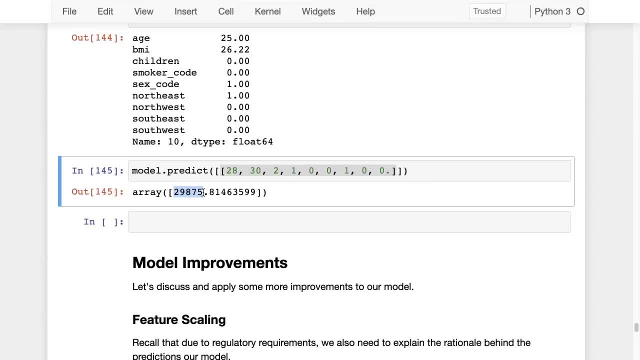 And then they would turn back and say: okay, on what basis are you saying that my medical charges are going to be 28,, $29,000.. And then you would say: so, my model, we created a model. We have a data scientist. 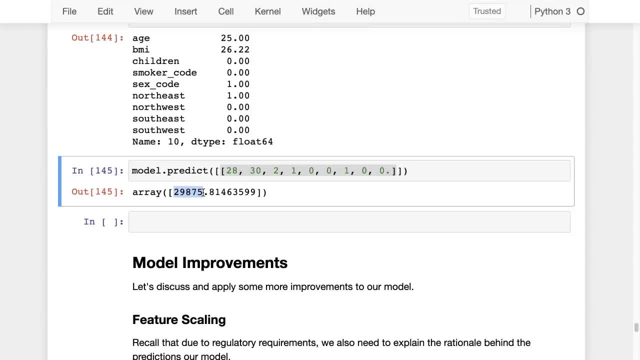 They created this model and the model says 29,000.. And then they say, yeah, but please tell me why it is 29,000. And that's a fair question, because remember the issues with correlation, causation, et cetera. we don't know what issues you had in your data. 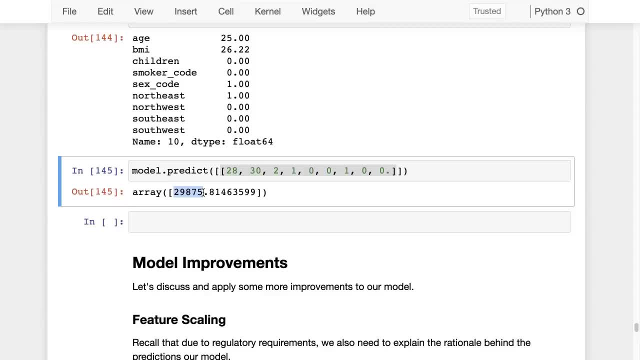 So you can't hide behind your model and say that the model says so. that's why we're charging you that money. You should be able to explain why your model gives a certain outcome. Now, fortunately, in the case of linear regression, that is fairly straightforward. 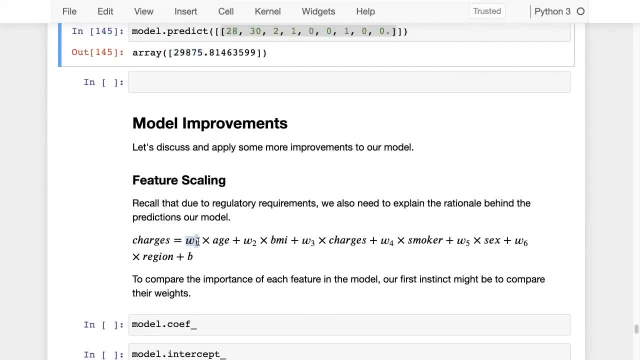 You can see here that we know that our model is applying some weight to the age, It is applying some weight to the BMI, It is applying some weight to the charges, some weight to the smoker, some weight to the, some way to sex, some way to region, some way to, and then it has some intercept right. 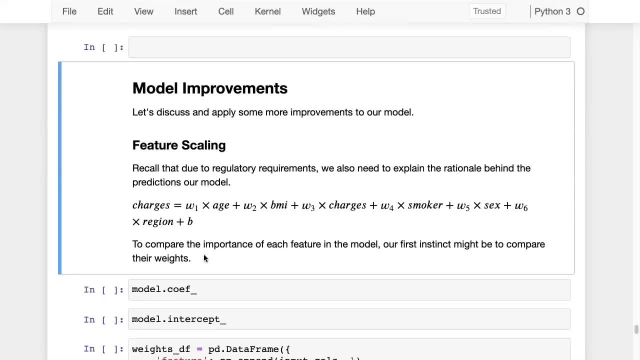 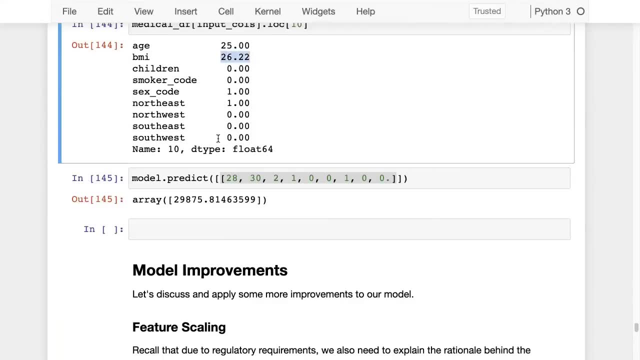 So some baseline, So to compare the importance of each feature. if you have to tell them that, Hey, we're charged, we're quoting this value because you have a certain BMI, And then we need to tell that BMI has a certain weight in our model, right? 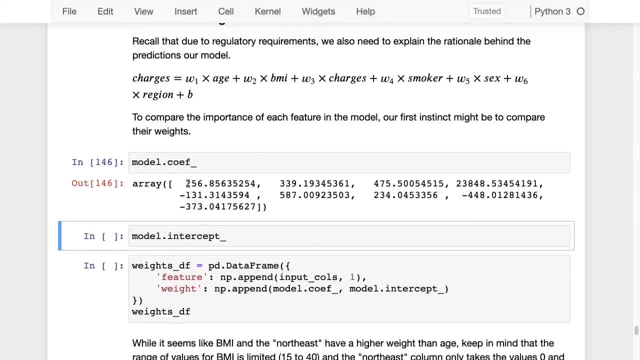 So we go here and we can check the coefficients of our model. The coefficients of our model are: The coefficients of our model are two, 56, three, 39, four, 75. So these are the weights applied to the model. Okay. 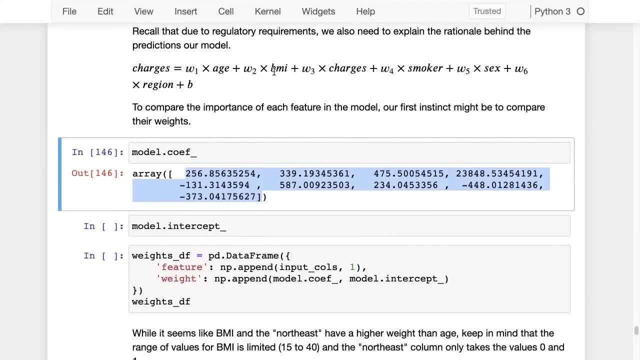 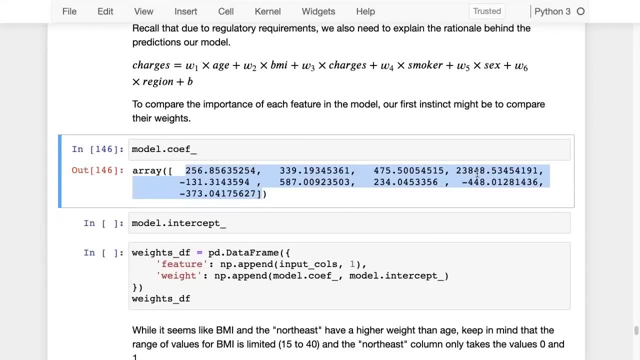 Now, based on these weights, if we compare, w one is for age, w two is for BMI, w three is for charges, w four is for smoker. So you might be tempted to say at this point that look we, we apply a very highway to smokers and $23,000 of your like $20,000. 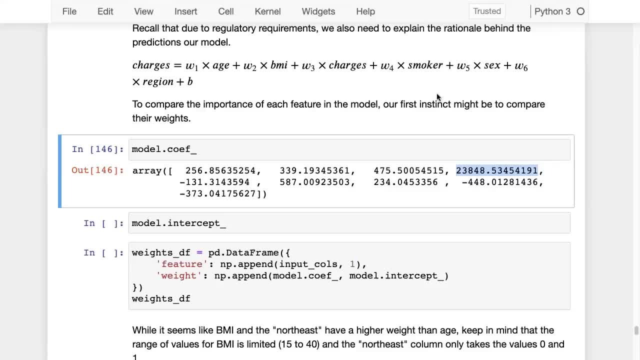 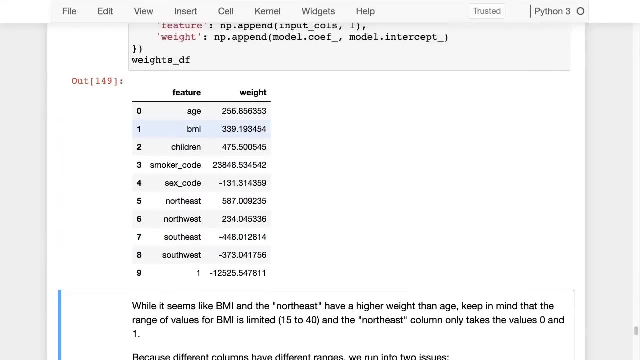 We've accounted for Simply because you're a smoker, right, And that could be fine in certain cases in smoker, because smoker is a simple plus or minus column, a simple zero or one column. It makes sense. But if you notice the weights carefully and to help you notice it carefully, I've actually put them into this data frame. 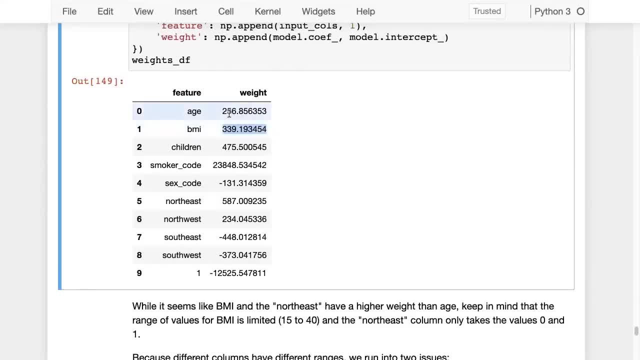 If you notice the weight carefully, it seems like BMI has a higher weight than age. BMI has a weight three, 39,, while age has a weight two, 56, and children have the weight four, 75. So this goes completely Opposite to what we understand. 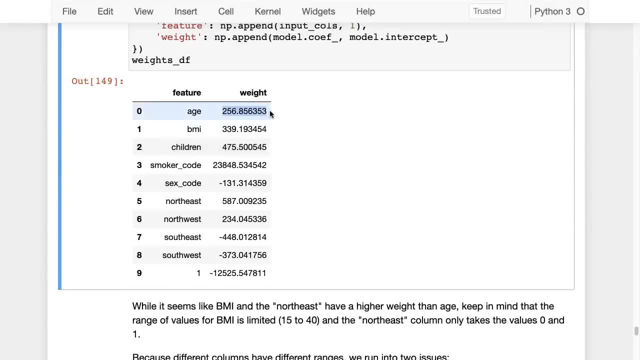 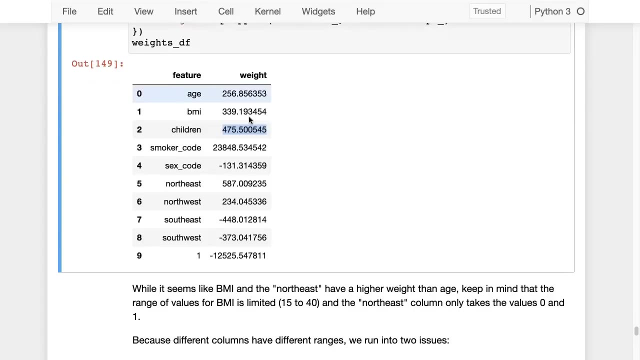 We understand that age is the age is one of the most important factors. We saw that for non-smokers at least, BMI has no bearing and the children again we saw had has no bearing. So what's going on here? Our models results seem to be completely out of sync with the weights that it is assigning to the different features. 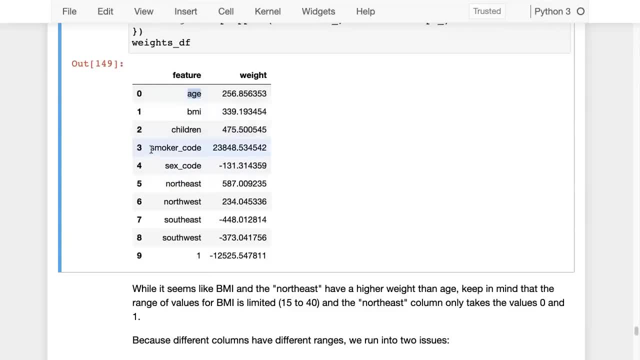 We, we felt that age and smoker to smoker definitely has a high weight, no doubt, but we felt that age has a far more Important impact than BMI, children, sex code, et cetera. but it seems like even Southwest, Southeast region has minus four, 48.. 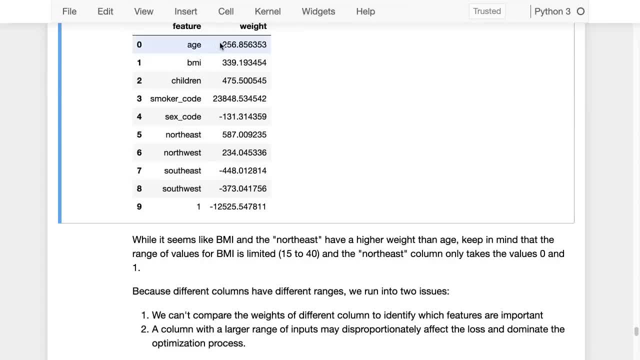 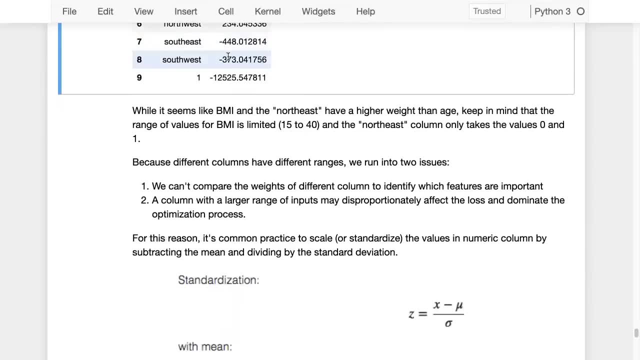 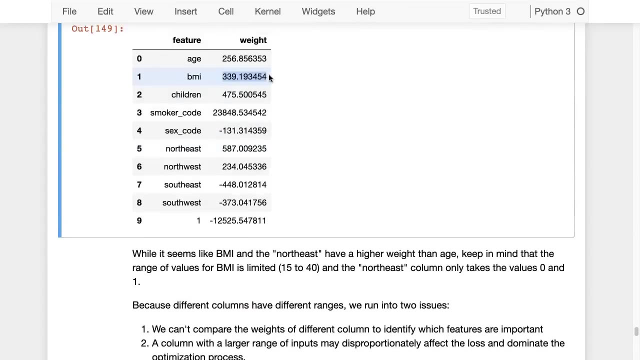 So it has a negative correlation. that is twice as high as age. So what's going on here? What's going on is that the range of values for BMI is limited. BMI is going to be limited from 15 to 40.. BMI is never going to go beyond 40.. 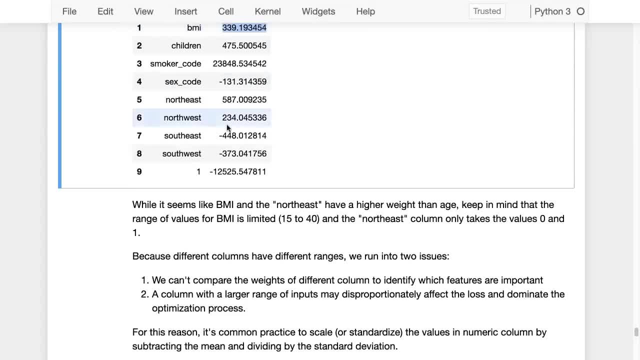 And in fact in most cases it's going to be around 30, the North East column is only going to take The values zero or one. That means the maximum change that the Northeast column can compute and then can create in the final output of charges is $500. 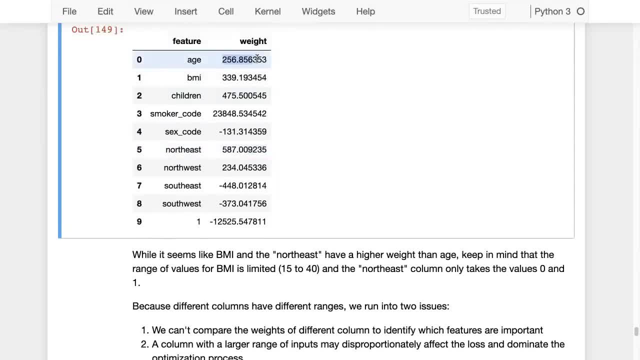 Not more than that. On the other hand, the age: even though two, 56 is the weight for it age can go up to 60. So it can create two 56 times 60. What's that? Two 56 times 60.? 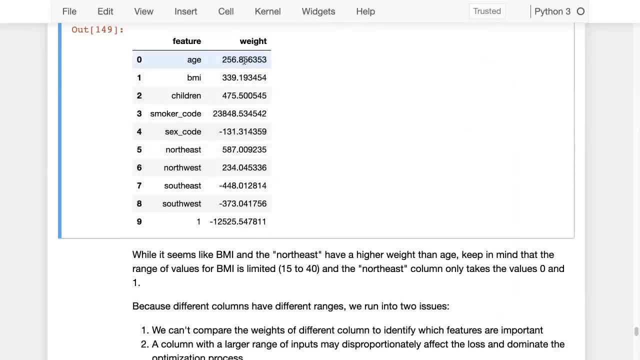 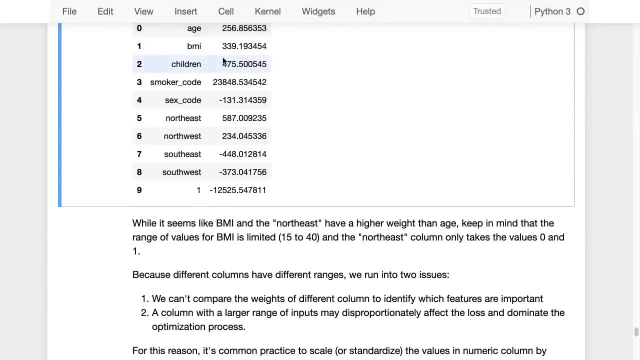 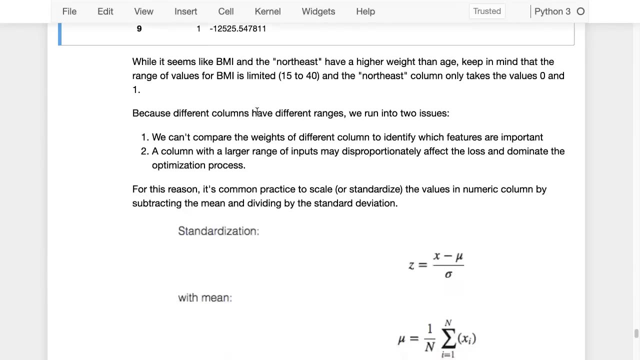 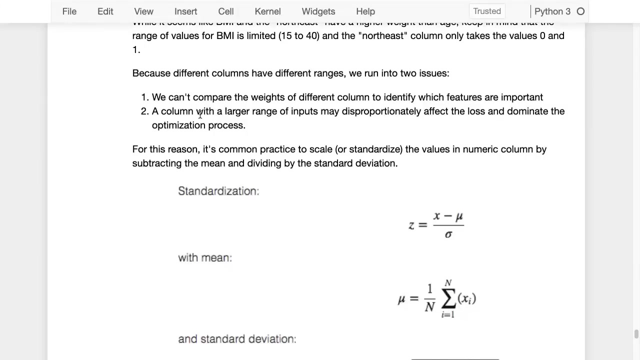 It can create a difference of $21,000, right? So the weights do not Accurately represent which features are important, because the ranges of the different features are different. That's one issue, And another issue that happens not so much in linear regression but in in in later data sets we'll see that sometimes when one column has a very large range of inputs- like age has a very large range of 15 to 60. 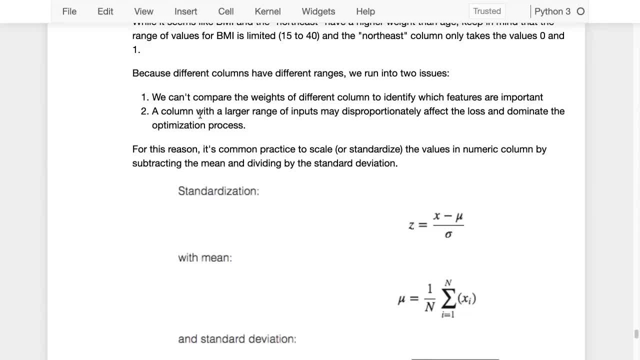 And one column has a very low range of inputs, Like region, can only go zero to one. So then, when you are calculating the loss and when you're performing Any optimizations, that large number disproportionately affects the optimization process because ultimately your number is. your model is simply looking at a single number: the loss. and the loss is computed using all of these inputs and outputs and weights and everything. 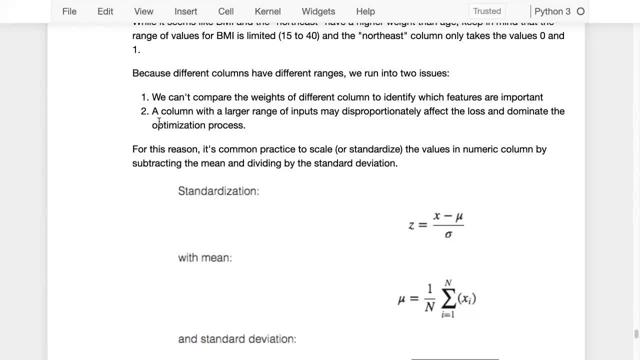 And if some column has a very large inputs or very large outputs- definitely very large inputs- then yeah, if some column has very large inputs, then it will disproportionately come contribute to the loss. So most of our effort will be Spent just optimizing for that one single column. 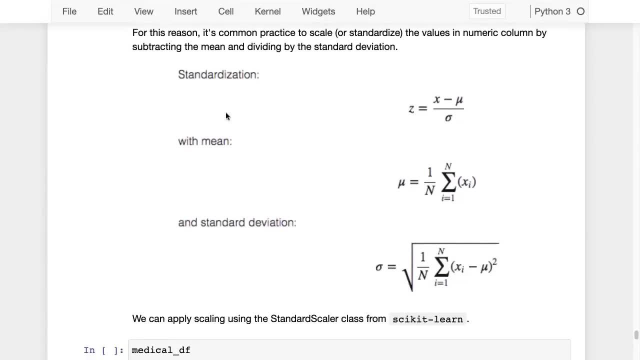 So that's where we perform a certain thing called standardization. We take the values in every column. from the value We subtract the mean of the column and then we divide by the standard deviation of the column. Okay, What does that do? 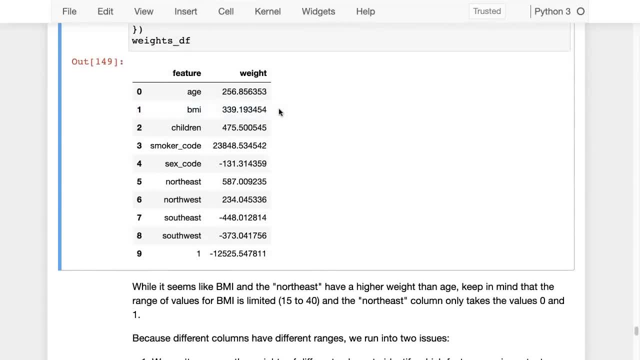 For example, let's say BMI. BMI goes in the range, or BMI varies from the range of 15 to 40. after applying the standardization, we subtract the mean, Which means we subtract 30 from the BMI, and then we divide by the standard deviation. 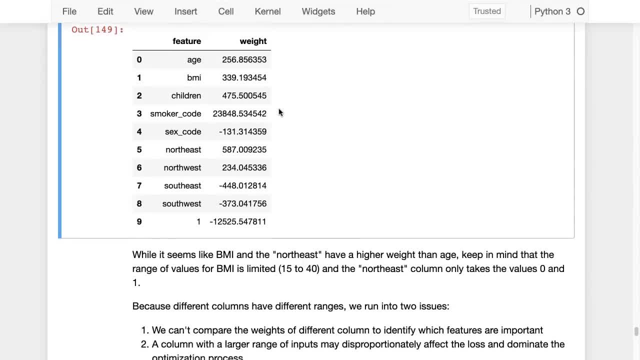 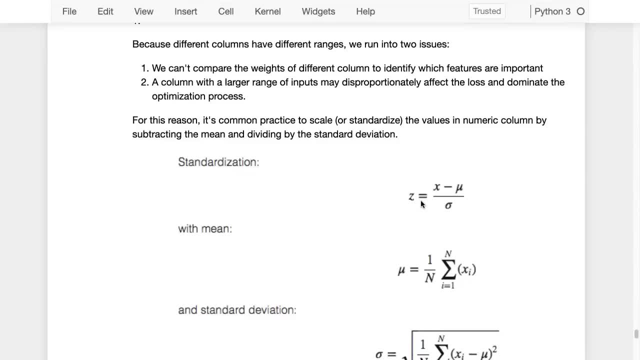 The standard deviation is around six. Let's say, after applying this standardization, the values become centered around zero. So you have the value zero and then you have BMI centered around zero and they are also scaled down so that it becomes a normal distribution with standard deviation one and mean of zero. 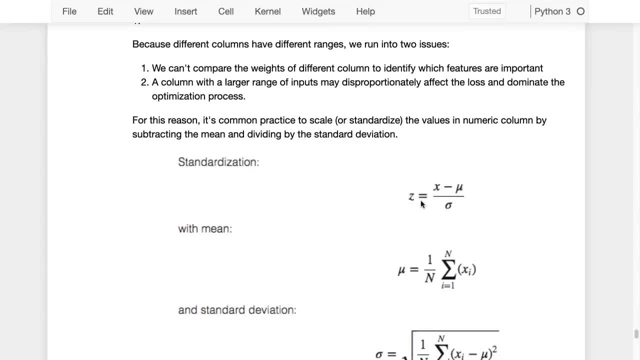 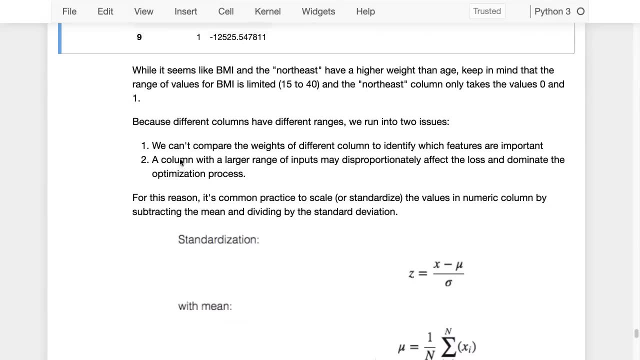 So the idea is we scale down all the values to small numbers that are in the range of one to minus one or two to minus two, And then their mean is also zero, And we do that for every column. So what we do is we standardize every column into the zero to one range, only for the numeric columns. 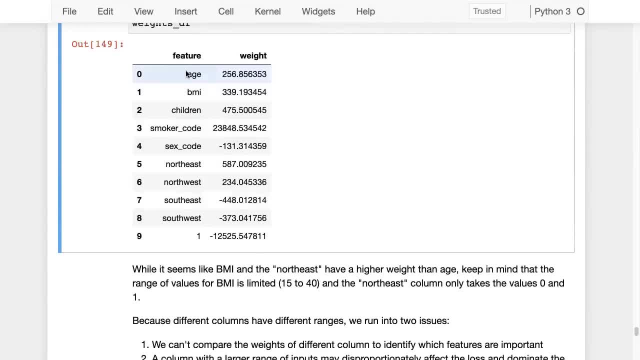 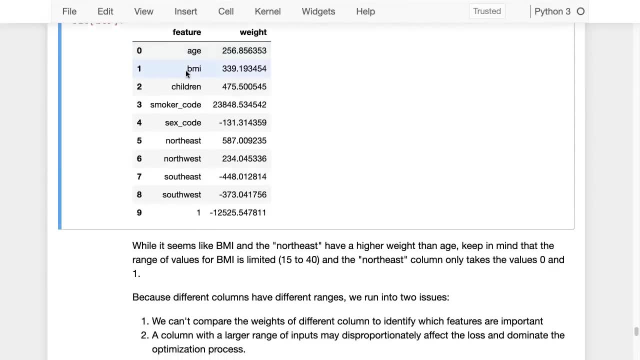 The categoricals are already like a zero to one, So we standardize the. the numeric columns in the minus one to one range means zero, standard deviation one, And then the weights will make a lot more sense. So here's how you do it. 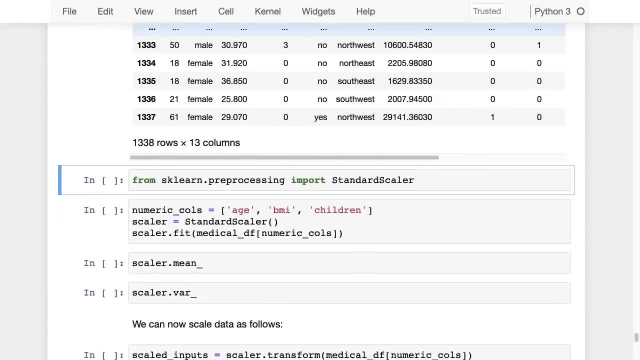 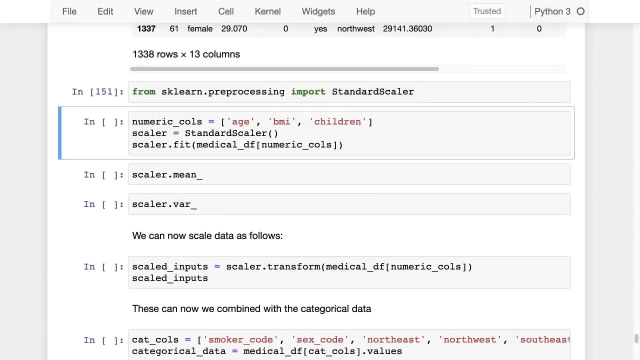 I'll just show you quickly the way to do. it is again, the way to really do it is to just look up Online. Hey, how do I perform scaling of features in a scale on? So I'm just going to import standard scale and we take the numeric columns: age, BMI, children. 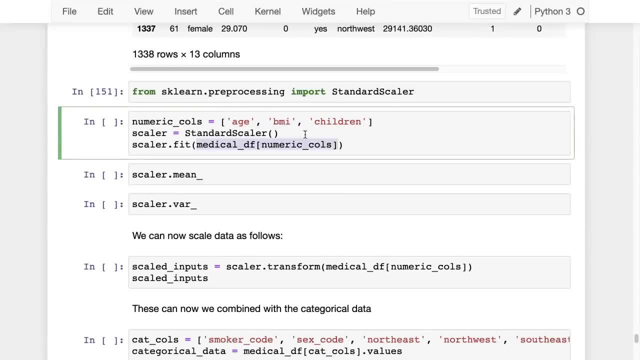 We get the numeric data from the scaler. Uh, we get the numeric data from the data frame- medical DF numeric columns- and we pass that into scalar. So we call scalar dot fit. All it does is it computes the mean and the variance for each of the numeric columns. 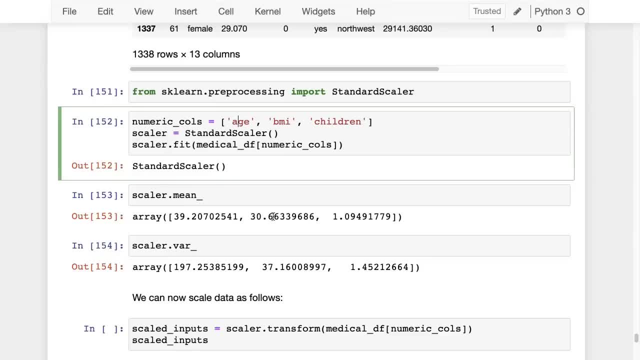 So it turns out that the mean for age is 39. And the mean for BMI is 30. And the mean for children is one. It turns out that the variant variance in ages one 97 variance is square of the standard deviation. 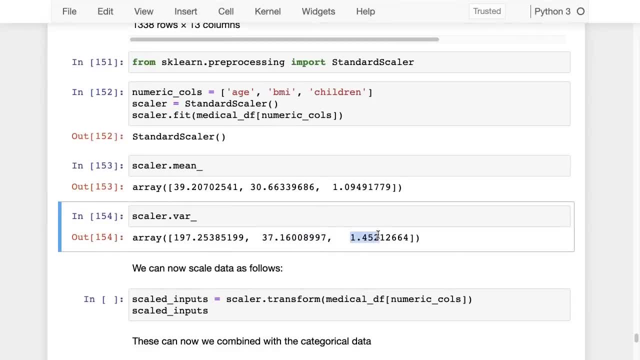 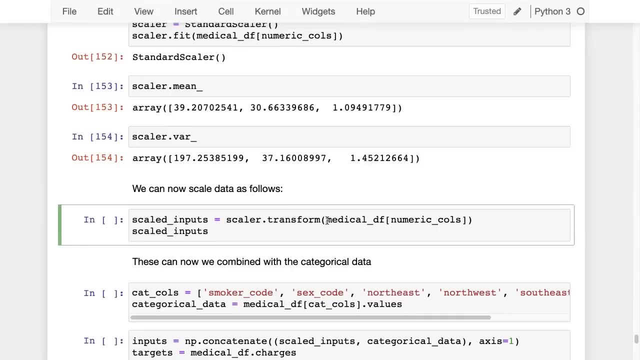 The variance in BMI is far less and the variance in children is even lesser. So now we can scale the data. So what happens now? we call scalar dot transform, and then we give it the data that we want to transform. So here's the data that we want to transform, which is medical DF. 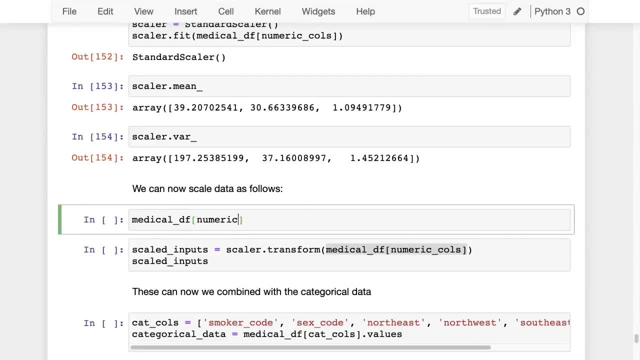 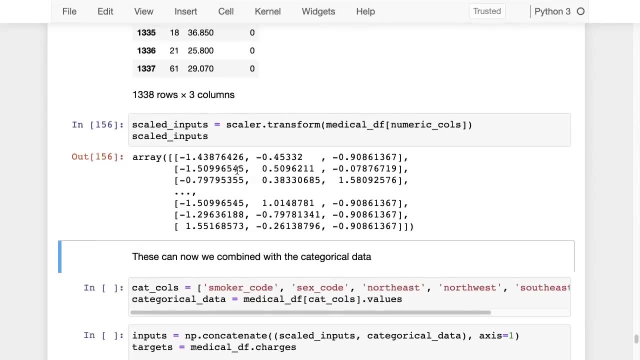 So we call that the value of the data, which is the number of numeric calls. This is the data that we want to transform- each BMI and children- And once we transform it, this is what the values will become. So they will go between minus one and one. 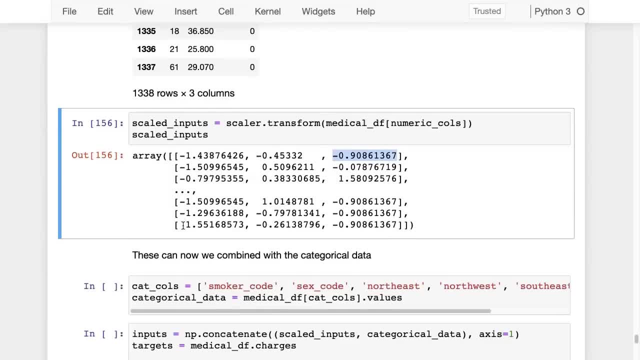 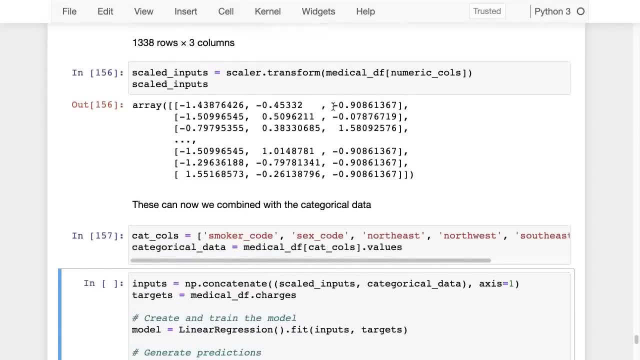 You see, here you can see that this is transformed to something between zero and one. This is transformed to something negative. So these values all change between minus one and one, And then we can take the categorical data And we can put it together. 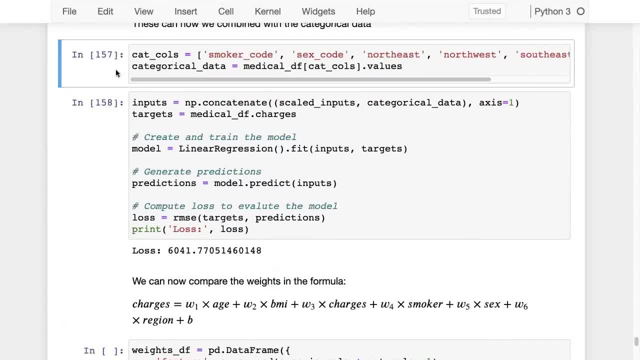 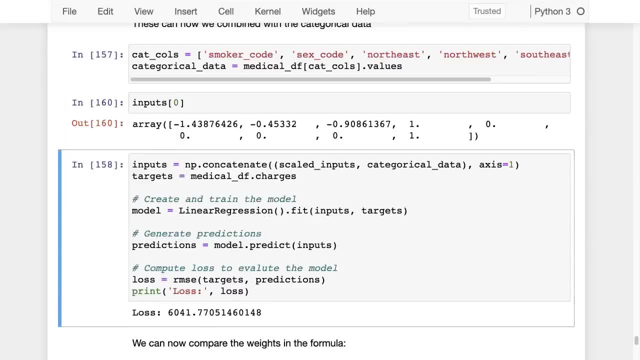 So we take Three rows of numerical data, We take all the categorical data and we put them all together and it looks something like this: So these three rows let me just take show you a couple of one row of data. So these three come from here. 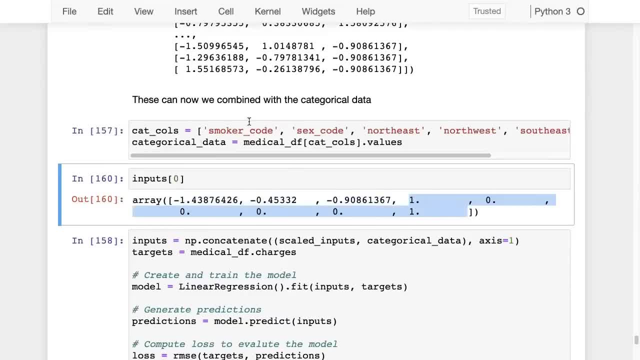 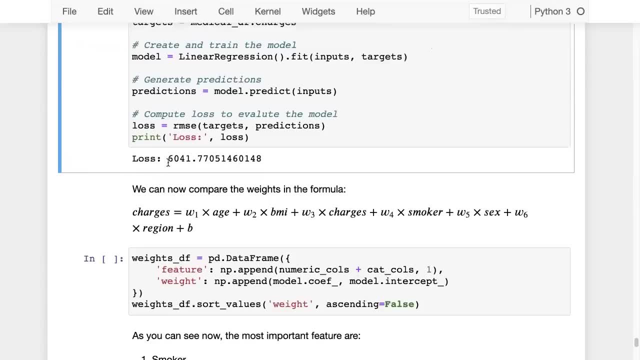 And then these three come from the categorical one: hot encoding and the binary encoding, et cetera. All right, And then we train the model So we get the same loss. It is in this case. it does not really affect the loss in linear regression. 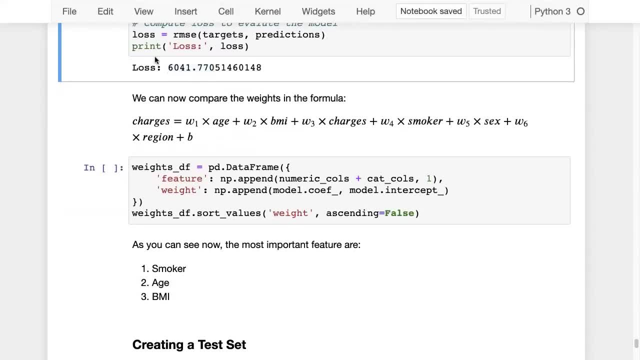 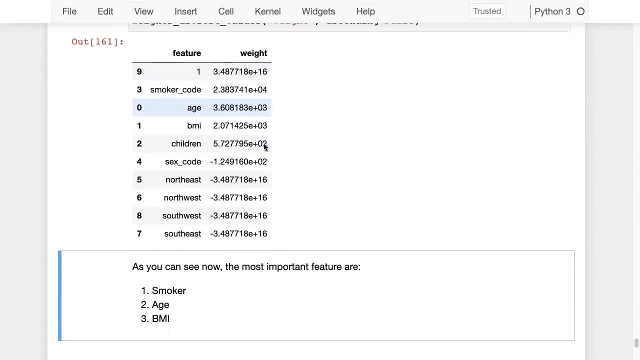 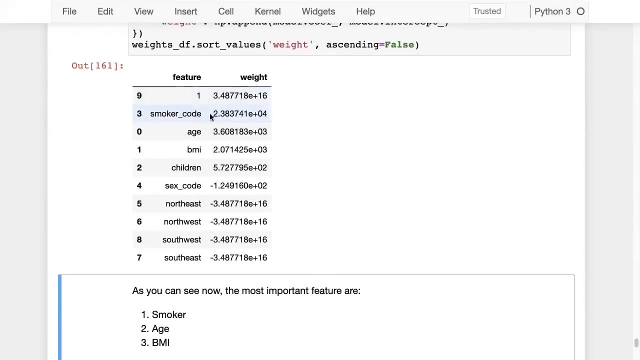 That's the scaling does not affect the loss. Okay, But the difference now is that when you look at the weight for every feature, you will see that the weights for the different features now make a lot more sense. So it seems like the weight for smoker. the weight for smoker is 2.3 into 10 to the power of four, which means 23,000, the weight for age is 3,600. 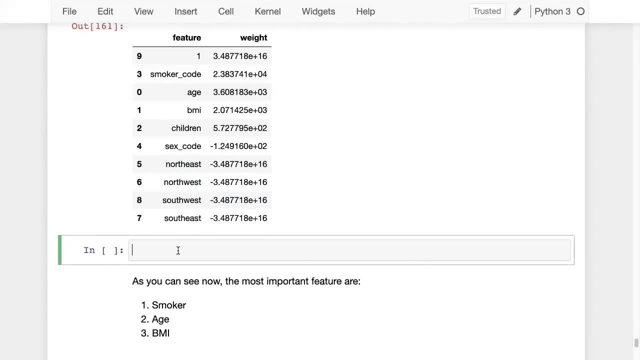 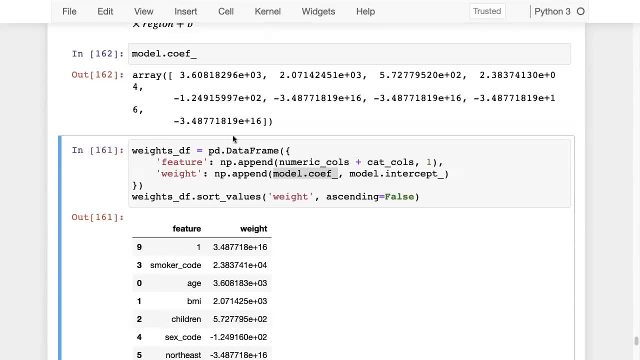 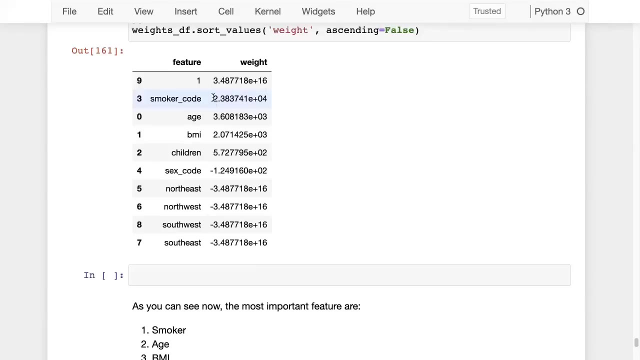 And I guess this is probably not the best way to print it. So let me just, let's just put this: Okay, Modelco F and. okay, I think we'll just have to interpret them here. So the weight for smoker is two, three, eight, three, 2.3 into 10 to the power of four, which is 23,000. 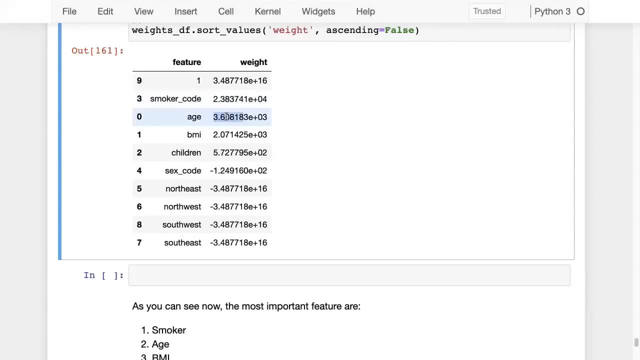 The weight for age is 3.6 into 10 to the power of three, which is 3,600.. The weight for BMI is 2.07, one into 10 to the power of three, which is 2000.. 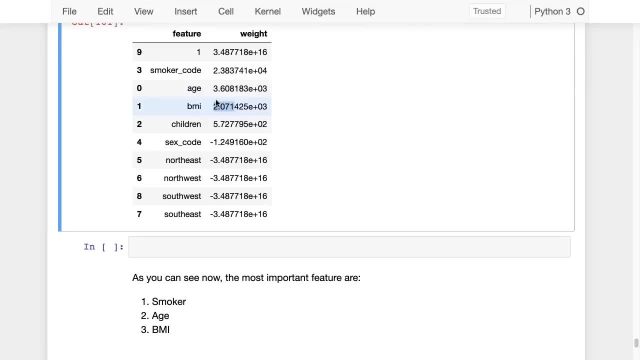 So now you can start to see that we have different levels of weights. and now you, You can tell the person, or you can, you can disclose that in our models, smoking has a very high weight of 23,000.. So it has contributed 23,000 to the calculation. 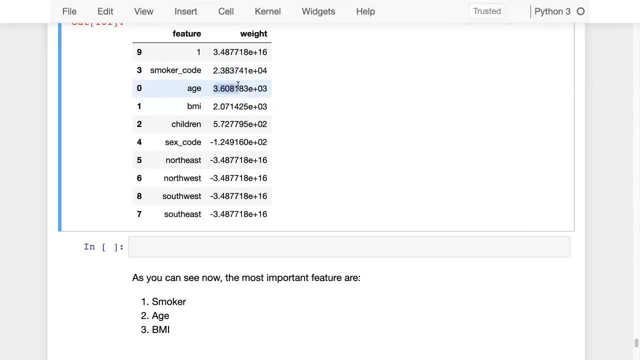 The age has a factor of 3,600.. So we add $3,600 for every year that you have been alive, based on your BMI. for every BMI point, we add $2,000 to your X medical expenses for every child you have. 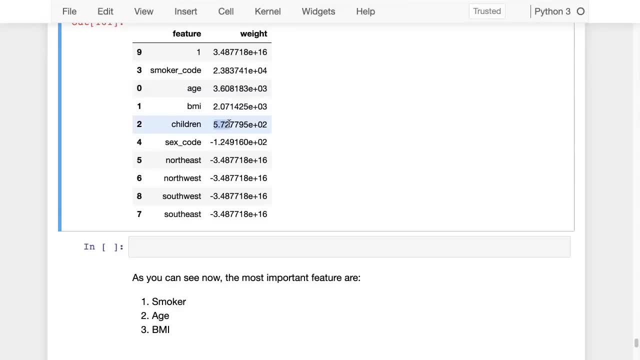 It seems like this is 500.. So for every child we have we add $572.. Then we have minus 1.249.. So it seems like for sex it's the inverse correlation. So we're actually subtracting some money. 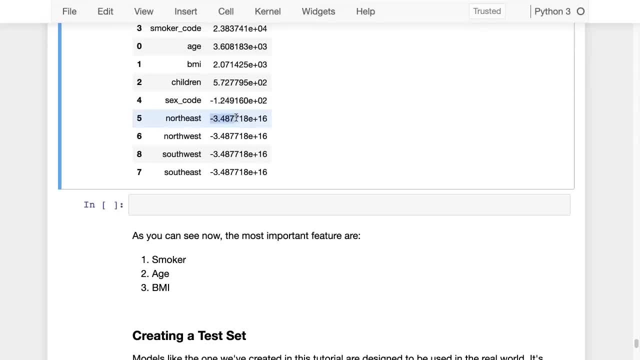 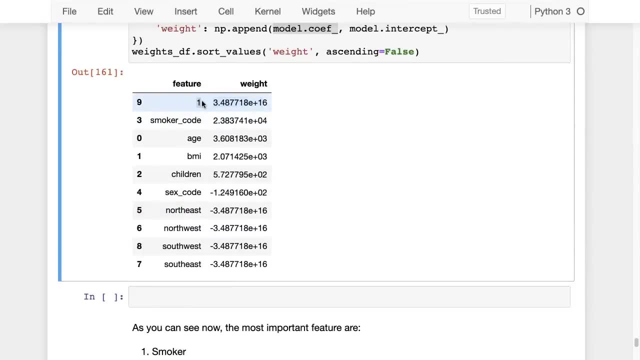 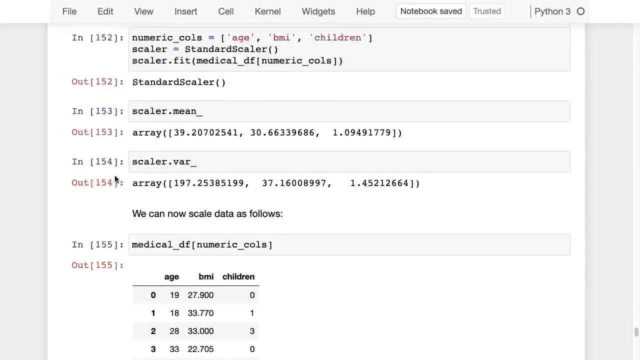 If you're a male, then, depending on whether you're from a certain region, we apply a certain correction factor for a region, And one of the biggest factors is the bias itself. So one simply represents the intercept. All right, Now one thing that you will have to do is, when somebody comes to you, let's say: let's go back to this person here. 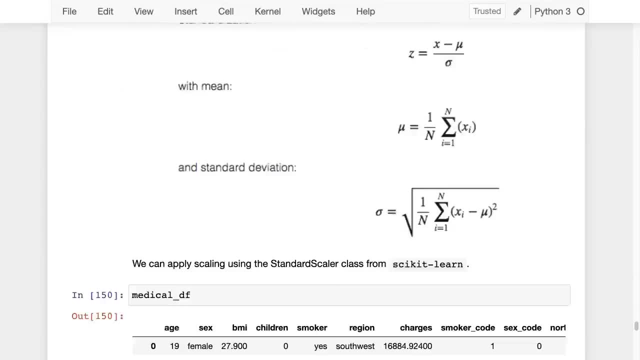 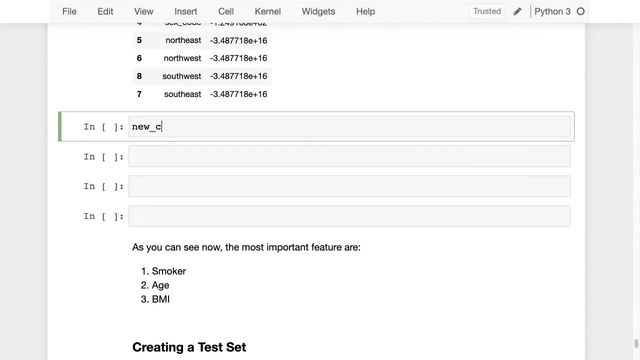 Yeah, So when a new Person comes to you, you will then have to scale these values before you can put them into the model. So let's see, let's get the new customers and we have just one customer here. The first thing we want to do is we want to do scaler dot, scale new customers and from the new customers. we are really only interested in scaling these columns. 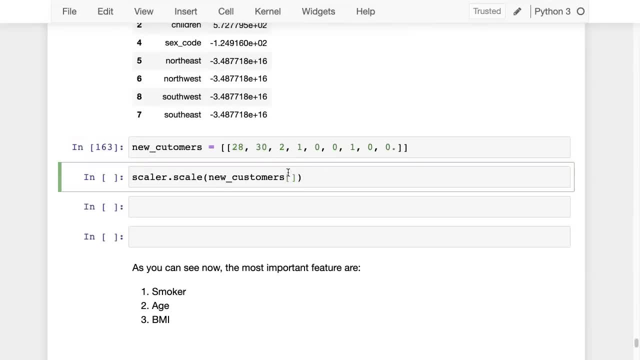 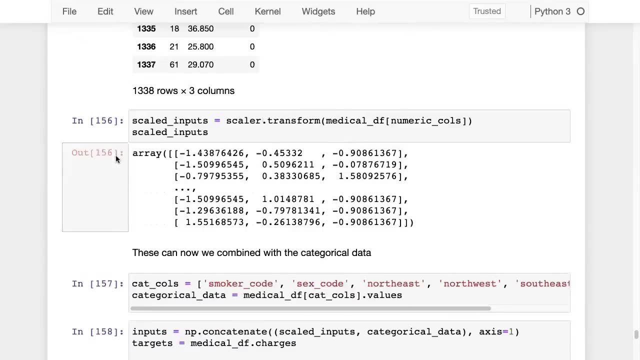 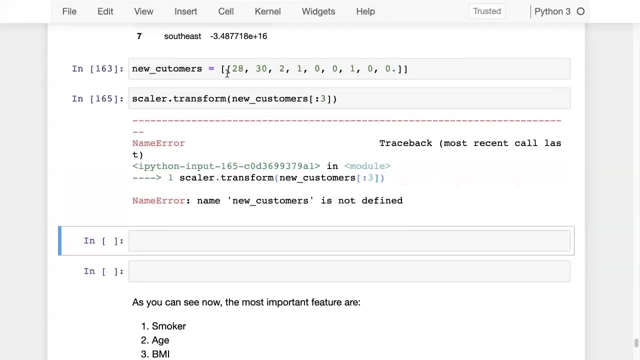 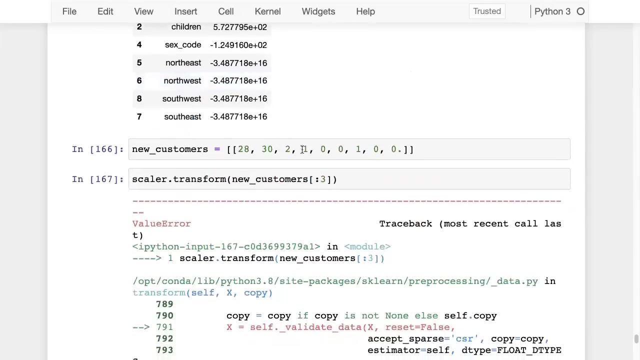 The rest, we don't really need to scale, So I'm just going to Take these three here. What's that called? Yeah, Transform- Sorry, Transform is the word Yup. Okay, Let's just simplify this and directly put these values in 2832.. 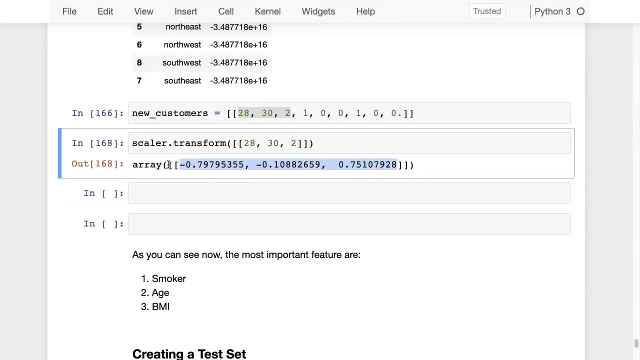 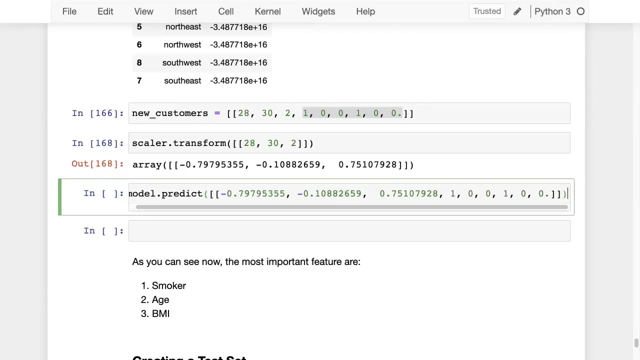 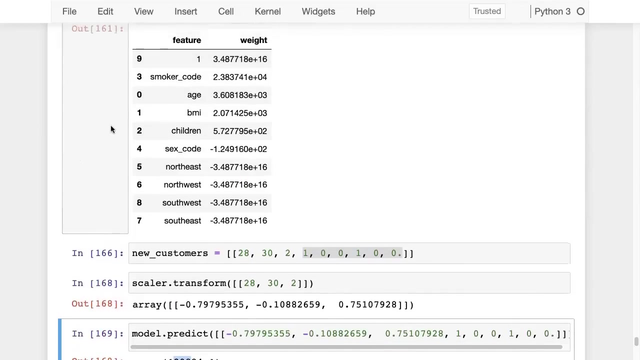 Yup. So you need to scale the numeric values to, anyway, 32.. And then you can simply copy over the actual categorical values- Here we have them- And then you can just call a model, dot, predict, And now you can see here that we have the result 29,824,. but now we have a very clear description of why we've applied 29,824, roughly speaking. 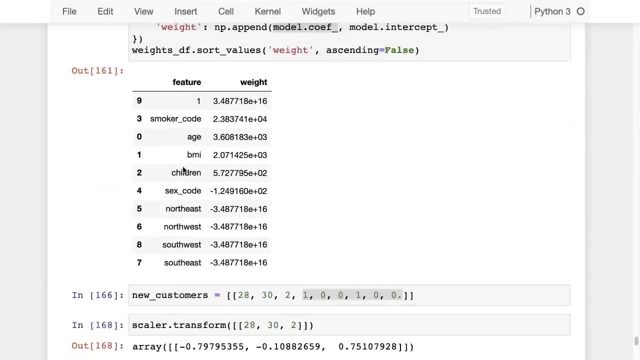 So yeah, that's how you interpret a linear regression model. What I said earlier was about age. adding $3,600 is not completely true because we have scaled the age, but you can give them a relative explanation that the most important factor is smoking. Then you have age, then we have BMI. 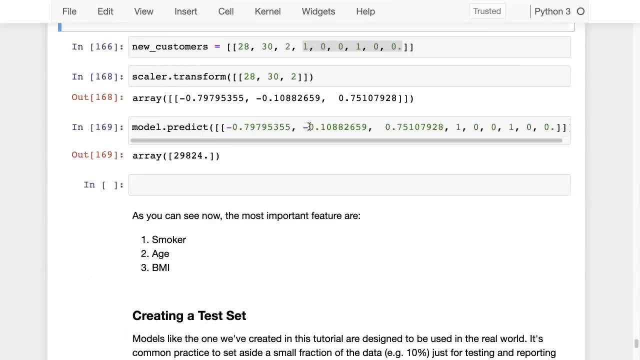 and these, these are the weightages that apply in your case. So in your case, the fact age factor is 0.1 or negative 0.1, and the BMI factor is 0.75, and so on. So this is age, I believe, and this is. 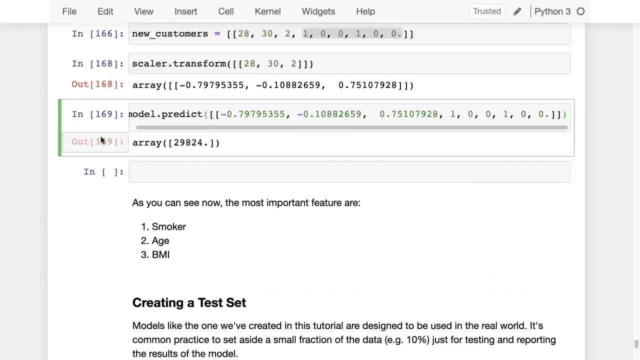 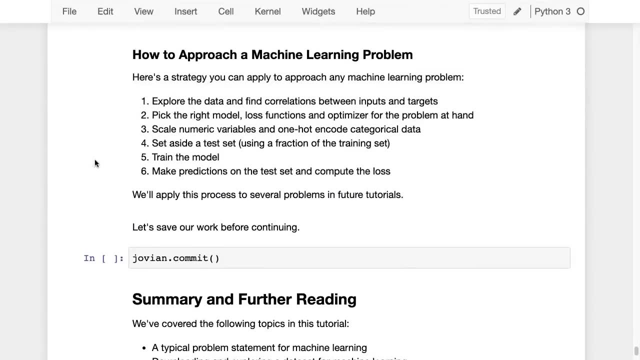 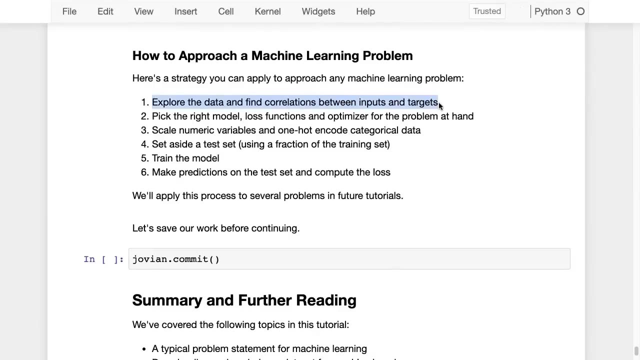 BMI. So that's how you scale the data. Okay, And I guess we're going to end here today. So just a quick summary of how you approach a machine learning problem. First step is to explore the data and find different correlations between inputs and targets. Understand what leads to. 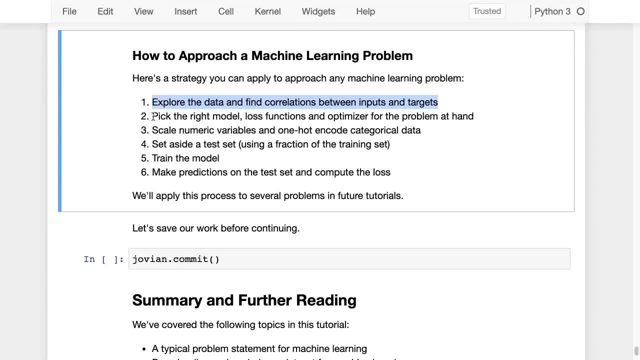 a machine learning problem, And then you can find out what leads to a machine learning problem, And then you can find out what leads to a certain target, maybe even go back and do some research whether there is a cause effect relationship or is there just a correlation And is it possible? 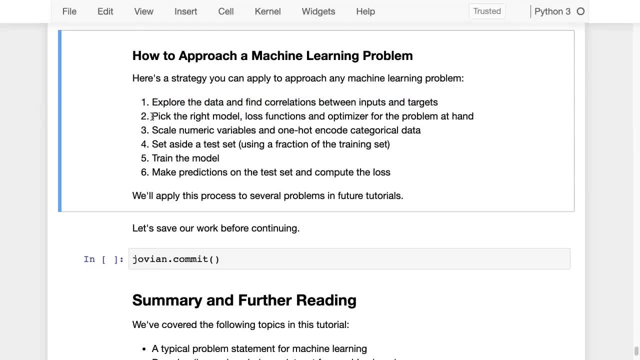 that the correlation may just go away, Or is it possible that the correlation is unfair in any way? For example, sure, Maybe you should not be using race as a factor in computing insurance, right? So that's something you should be conscious of as a data scientist. Then you pick the right. 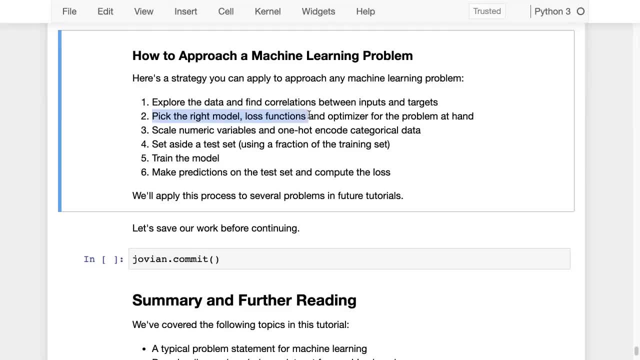 model. In this case, we pick linear regression. You pick the light loss functions- In this case we picked root, mean squared error- and you pick the right optimizer. In this case, we pick least squares. And all of these three are captured in the linear regression class from. 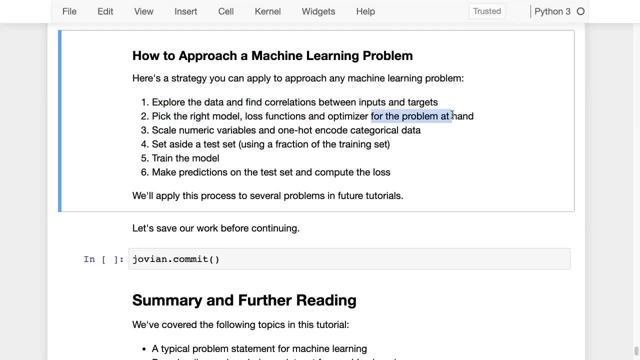 scikit-learn. So for different problems you have to pick different models. Sometimes you have to pick decision trees, Sometimes you have to pick neural networks or something else. Then you scale the numeric variables and a one hot. you scale the numeric variables so that they all have a mean of. 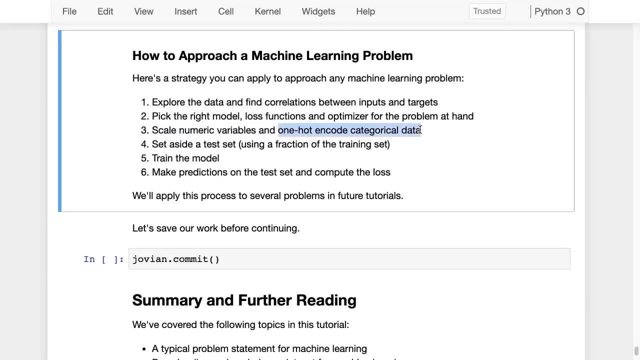 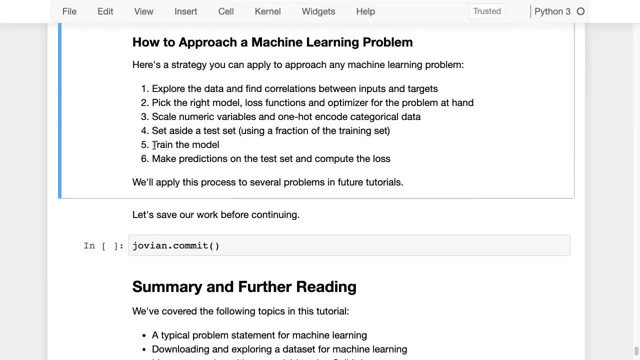 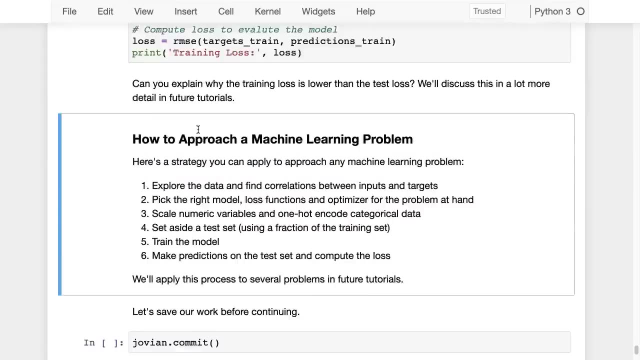 zero standard deviation of one. You perform one hot encoding for categorical data- And this is not something we covered today, but this is something that we will cover next time- about setting aside a test set. Then you train a model, Then you make predictions and compute the laws. Now, we didn't do this today, but one thing you should do is you. 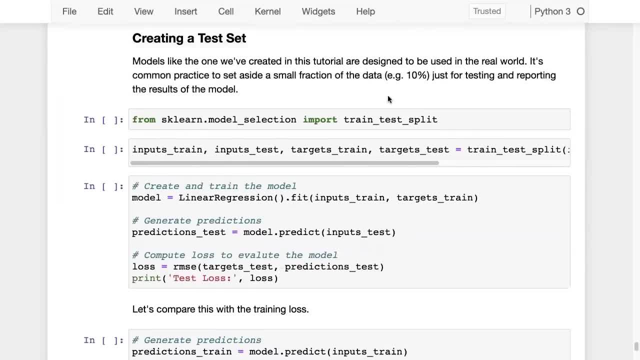 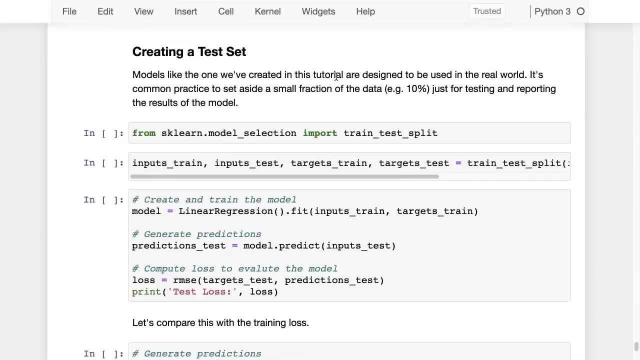 should actually set aside 10% of your data, a small fraction of your data, just for testing and reporting the results of your model, because the model, like the ones we have created today, are designed to be used in the real world, not only on the data that we trained them on. So what people? 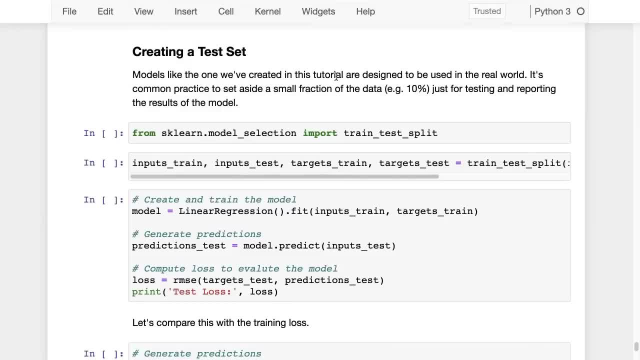 typically do is when they get some data from, let's say, a product manager or some somebody whoever has given us the insurance data, we take 10% of the data and then we set it aside forever. Then we do all our modeling and everything. Let's say we build. 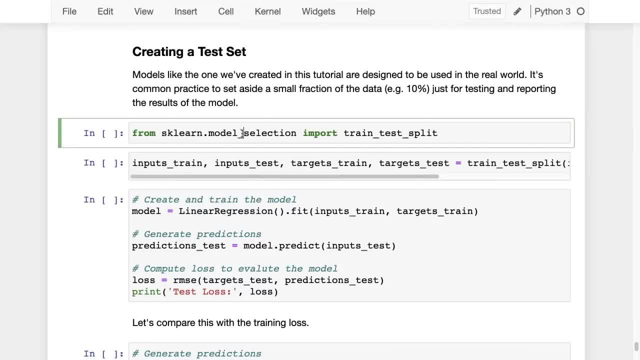 a linear regression model on 90% of the data And then, when we report the loss, when we actually report the metrics, that, Hey, I have built this model and this is the result it gives And this is the kind of loss that I've been able to achieve, or this is the kind of error that my model has. 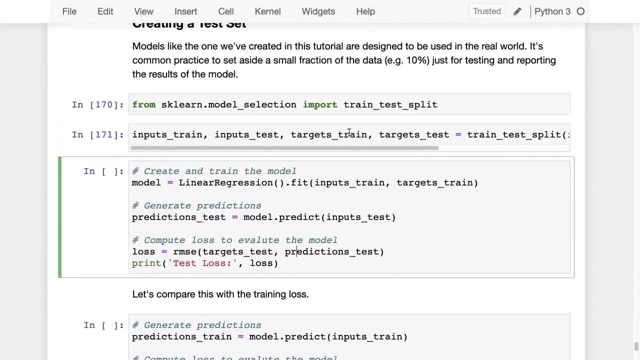 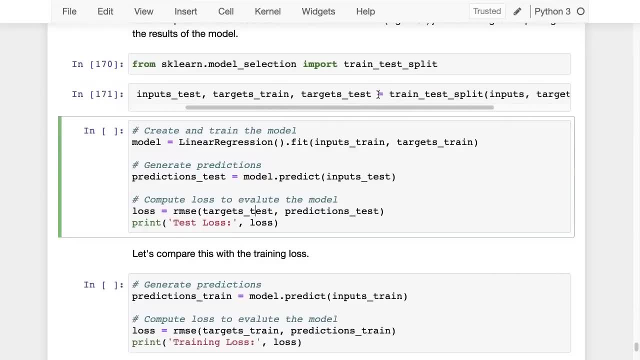 You should be then reporting that error On the test data, which means on the 10% of the data which you set aside at the beginning and did not use for training, And you can do this in scikit-learn using this train test split. 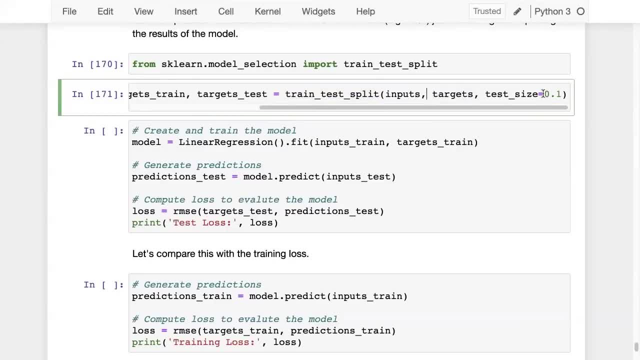 So what that does is it takes some inputs, It takes some targets, It takes a 0.1, like a fraction, and it gives you a bunch of 90% of the data which you can use for training, which is input strain, and 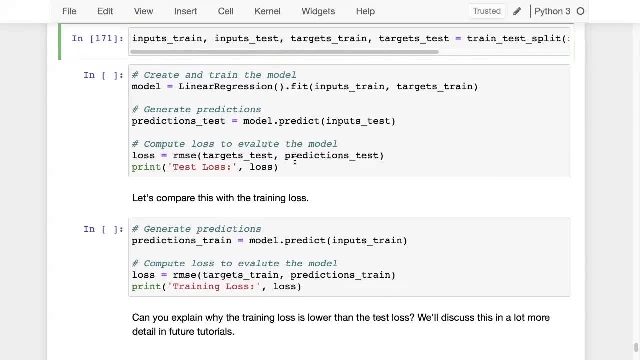 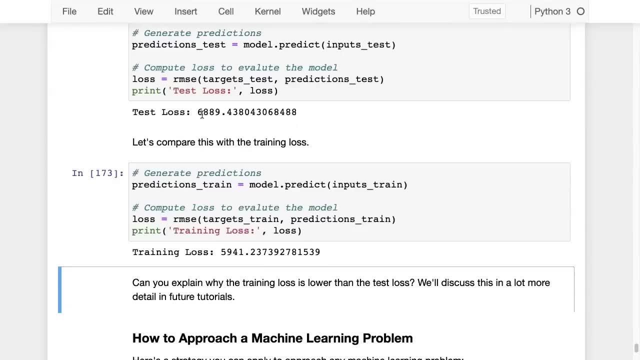 target strain and then 10% of the data which you can use for testing. Okay, And we'll talk about this in a lot more detail the next time. Okay, But what you will notice is that the score on your test set, or the loss on your test set, is: 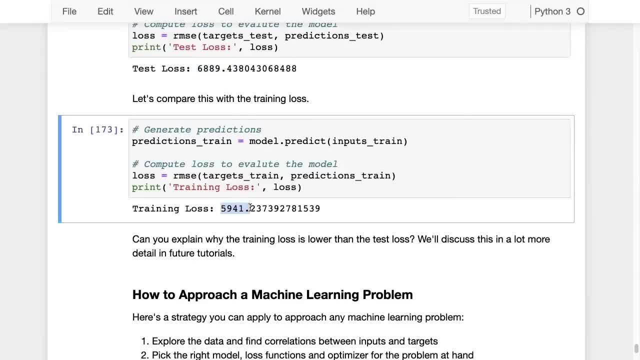 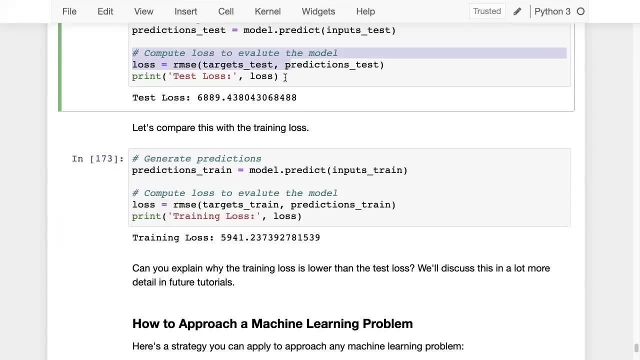 going to be always higher than the loss on your training set because your model has not seen these examples. So model is bad, is worse at predicting examples that it has not seen, And this is again true A lot of machine learning models when you put them out into the real world. 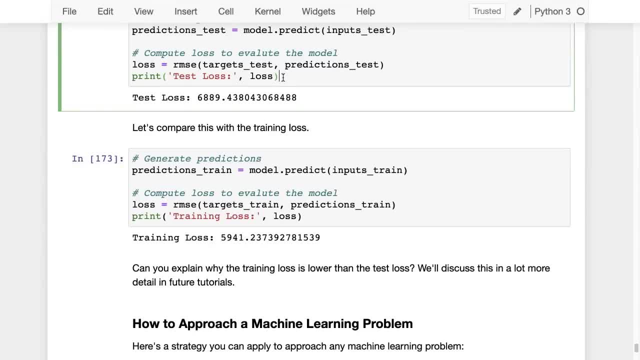 they perform worse. even though you may get a really, you get like a 98% accuracy when you're training the model, but when you put it out it's less than 30%. So we will talk about a lot of techniques in this course on how to counter that. this is called. 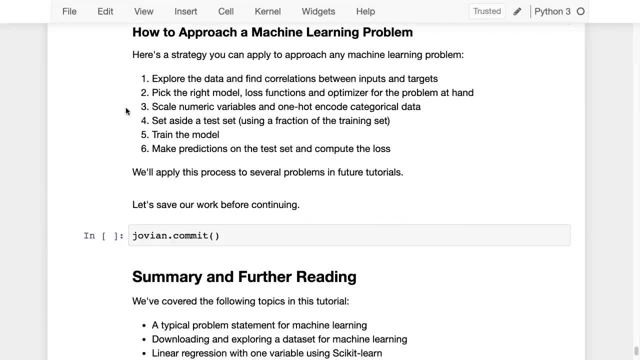 overfitting And we'll talk in a lot of detail about that, right. So the right strategy is to set aside a test set before you train a model and then train the model and then make predictions and compute the laws and report the results on your test set, And we will apply this process over and. 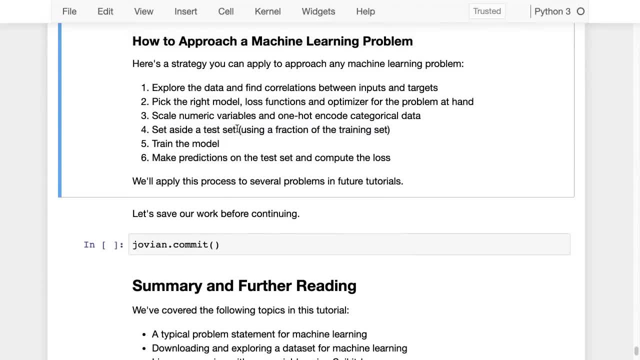 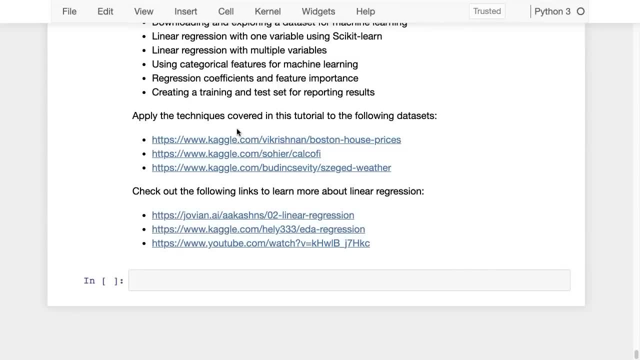 over to several problems with different kinds of models. So that's all we have for today. What you should do really is just run the notebook, try and understand every line. Of course, we've tried to work through it step by step And, if you can understand linear regression, 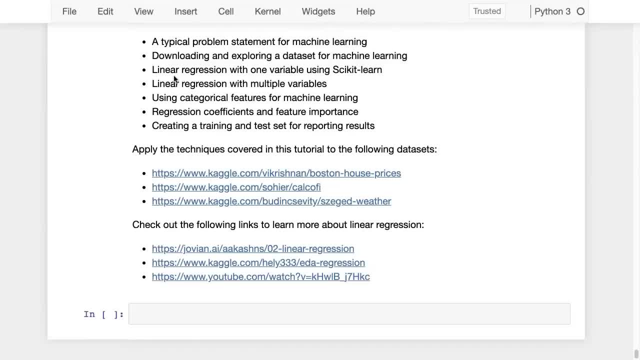 with one variable, then you should be able to understand linear regression with any number of variables And you should be able to understand any machine learning model going forward. Remember that picture about inputs going into a model coming out as predictions. compare them with the 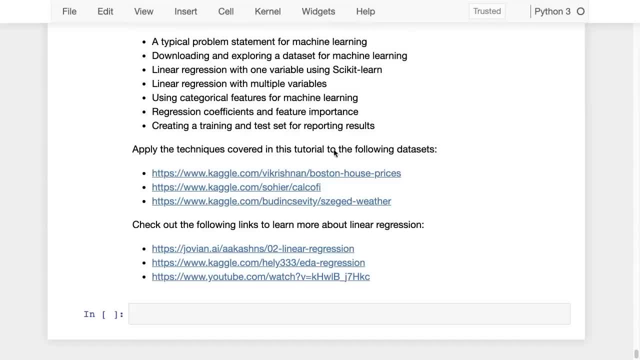 targets using a loss function and then use an optimizer to improve the model. That's all machine learning is. but getting that, the getting that kind of a workflow, internalizing that workflow, is what you need to try and figure out, whether it is by working through this notebook. 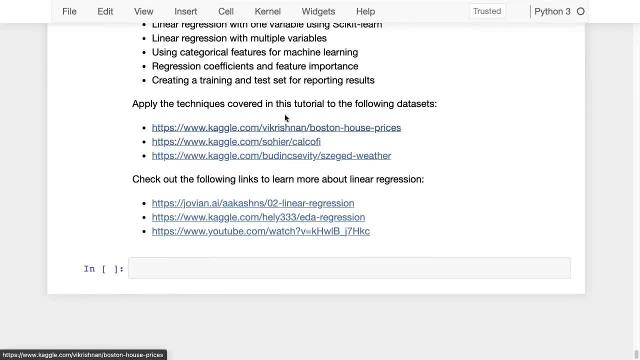 again watching this lecture, again applying it to a few examples or maybe looking at some external references, But once you get that, machine learning becomes really simple. Okay, So here are some other, some resources for you to check out and some other data sets that you can apply. this 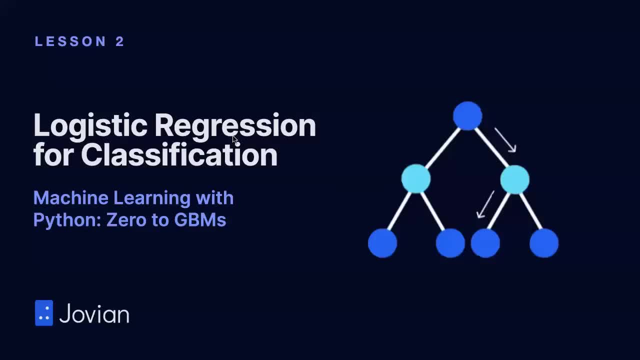 technique to Next week we will look at lesson two, logistic regression for classification. This is machine learning with Python zero, two GBMs. Thank you and goodbye.